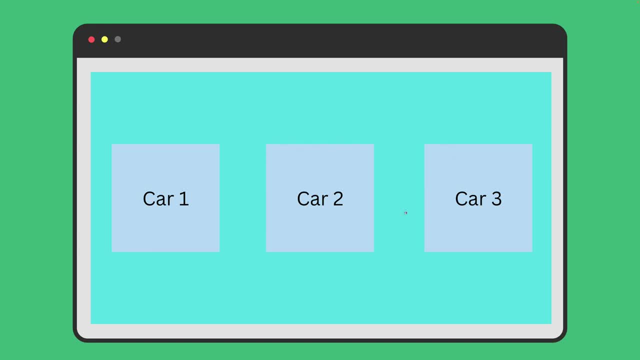 to want to do is add multiple different pages on your website. So maybe for the home page you have this display right over here, but maybe you want to add a nav bar where you know a user can actually click on this about right over here and it shows them a different page that kind of talks about the 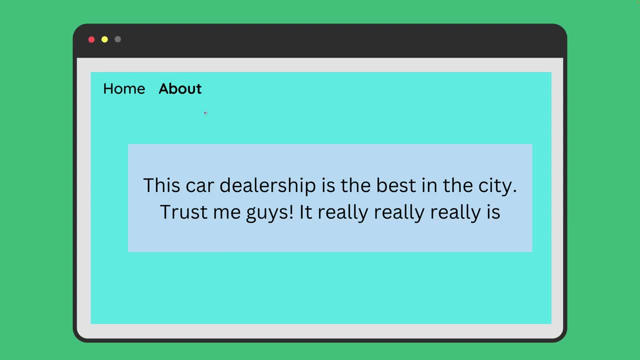 dealership. Nonetheless, what you want to do here is you want to add multiple different pages within your view application, and that is that is exactly what view routing is for. You're going to add these pages and you're going to define all of the routing rules to take you to the different pages that you. 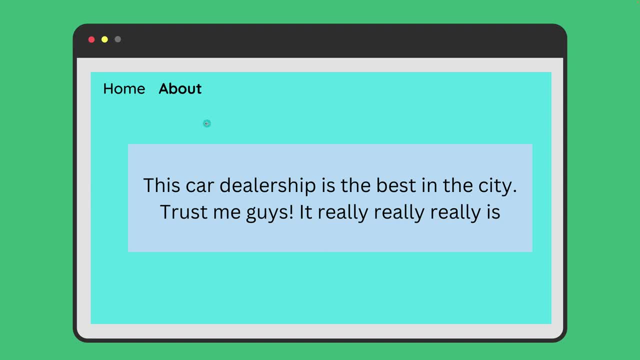 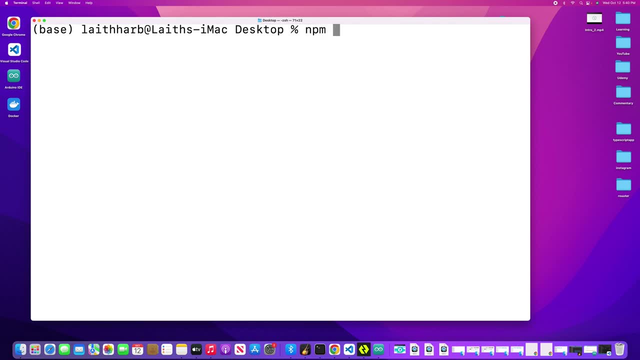 want. So, nonetheless, let's actually go ahead and quickly create a view application and we're going to go ahead and start working with view routing. So let's open up our terminal and we're going to do a npm init and then we're going to view, at latest, just to create a. 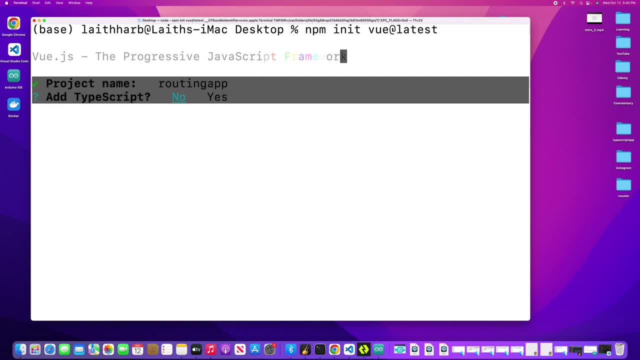 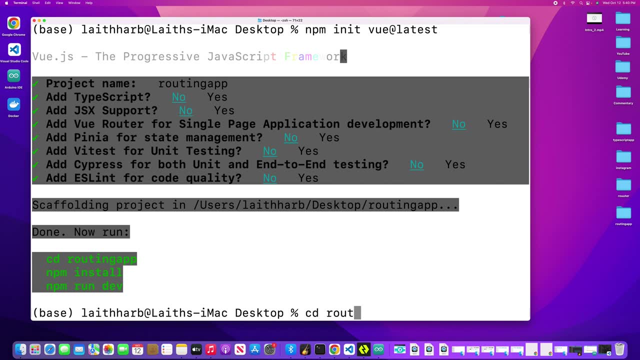 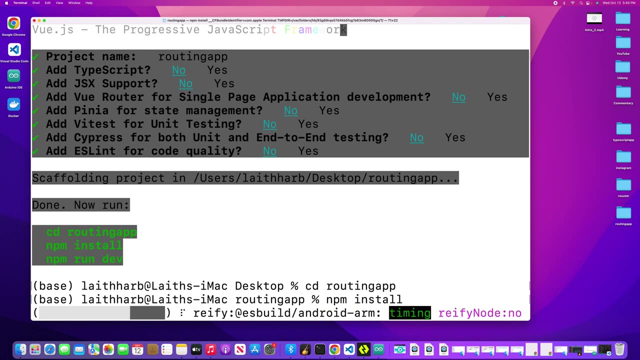 brand new view application and I'm going to call this routing app and I'm going to say no for all of the options. I'm going to say no for everything, and then I'm going to move into the routing app and I'm going to do an npm install to install all of the dependencies. Now, as this installs, 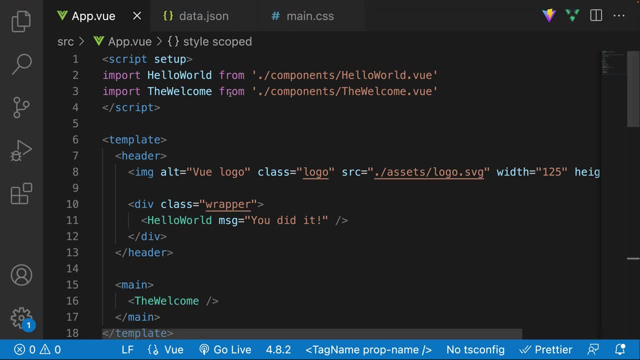 what we're going to do is we're going to go ahead and open this up in VS code. So, as you can see, I actually already have it up in VS code, but you go ahead, open it up in whatever text editor that you want. and before we actually dive deep into this, let's go ahead and just do a little bit of cleanup. 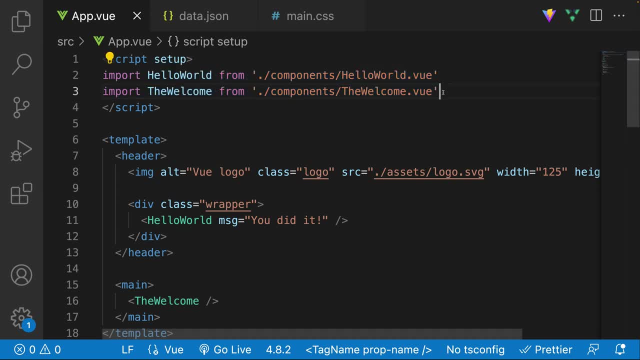 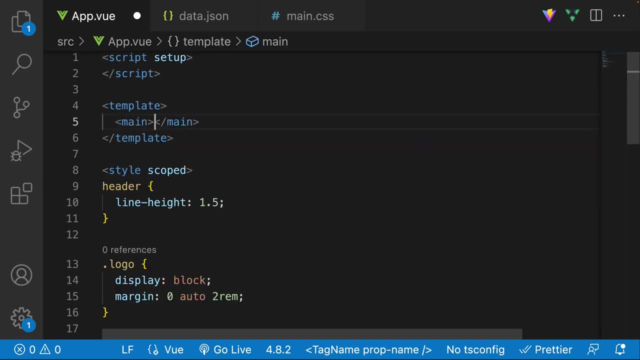 So I'm going to go to the appview file and in that file I'm going to remove everything over here inside of the script tag. I'm going to also remove everything inside of the template. I'm just going to have an empty main tag and also everything inside of the template. So I'm going to go ahead and 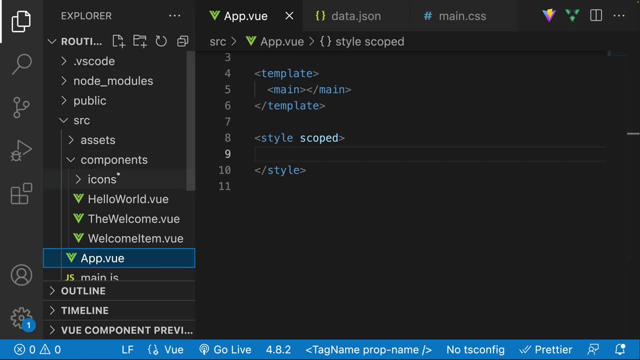 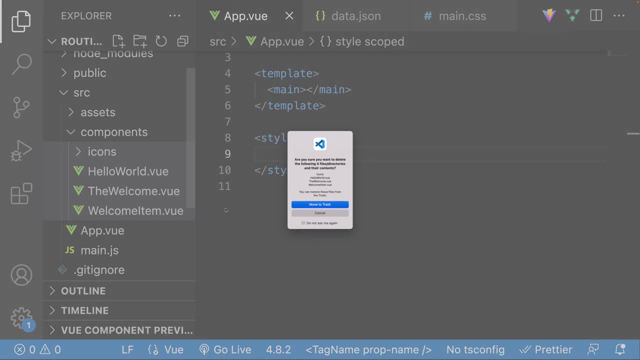 have the styles, let's go ahead and remove it. and also, what we're going to do is we're going to go to the components directory and literally everything in the components directory, just go ahead and delete it. So we're going to go ahead and remove that all together. and lastly, the last little: 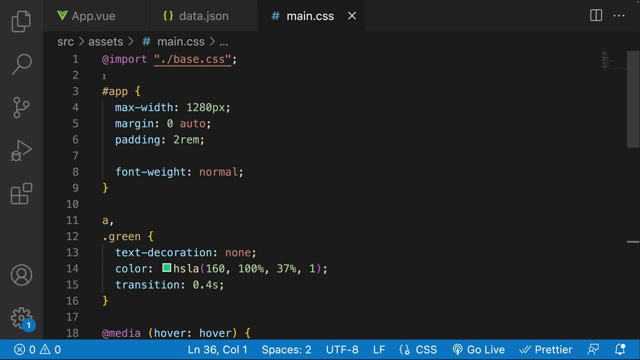 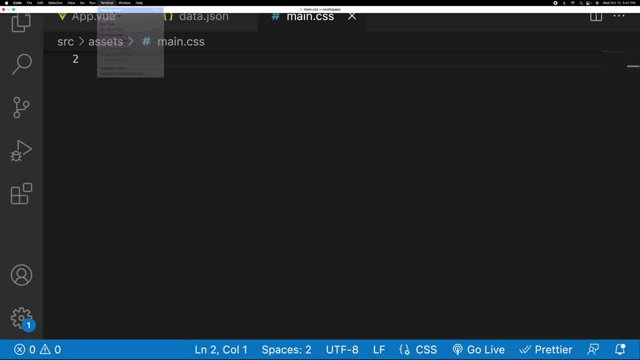 cleanup that I want to do is, in the maincss, everything below this import. just remove it. All right, so cool, everything is done. So now let's go ahead and start up our application. The npm install should be done, So we're going to do an. 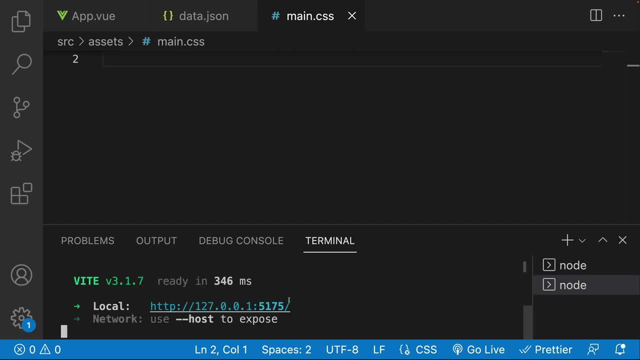 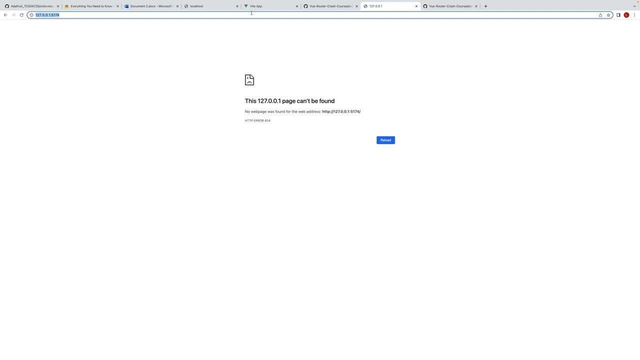 npm run dev to start up our application. and my app is running on localhost 5175.. Yours is probably different, it's probably on 73. But nonetheless, if I were to open this up and I did all my cleanup correctly, you should see a blank application. Okay, so this is looking pretty. 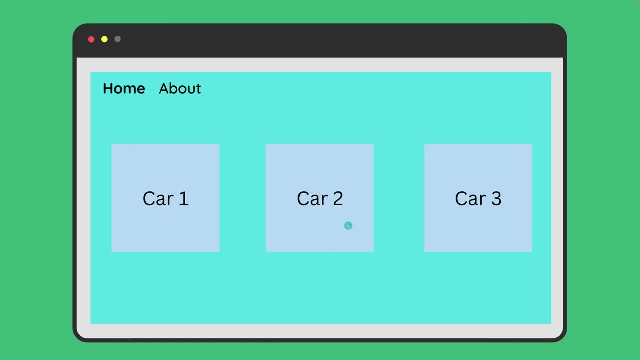 good. So let's go ahead and actually create a scenario that looks a little something like this, where we have our home page and, as soon as we hit our view application, we are all of the different cars that we have. Now, in order to do this, we're going to need to have: 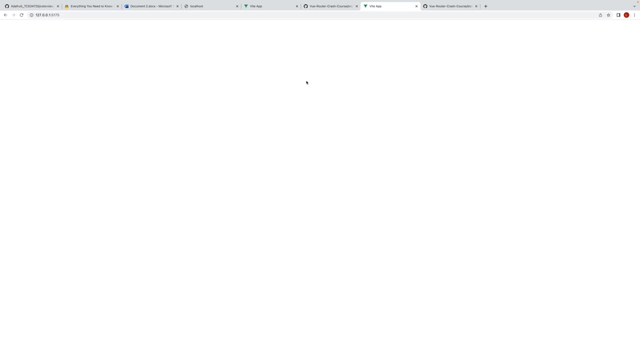 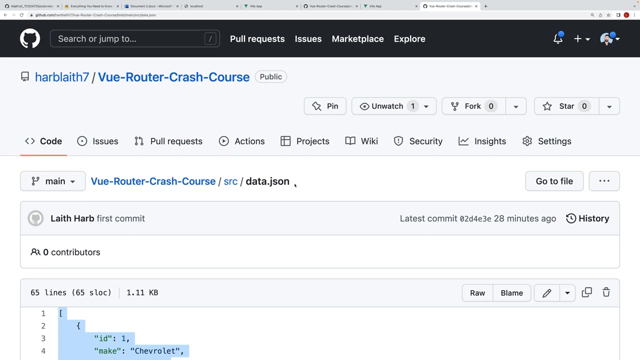 some data for our cars. So, instead of us just writing this up manually- because it doesn't really have anything to do with view routing- what I'm going to do is I'm going to link my github repository inside of this video and, specifically, you're going to go to the source. 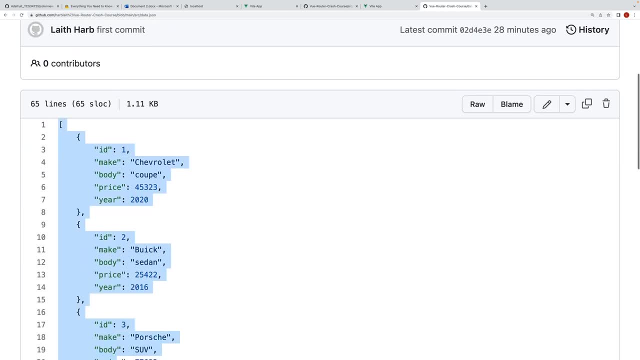 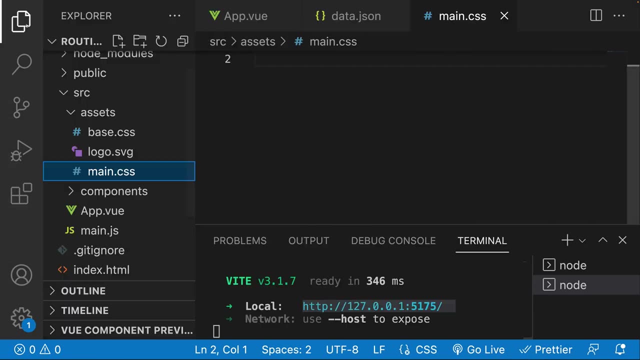 and then the datajson. and what you're going to do is you're just going to copy this json blob of all of these different cars. So go ahead and copy that. and then what you're going to do is you're going to go to your source. 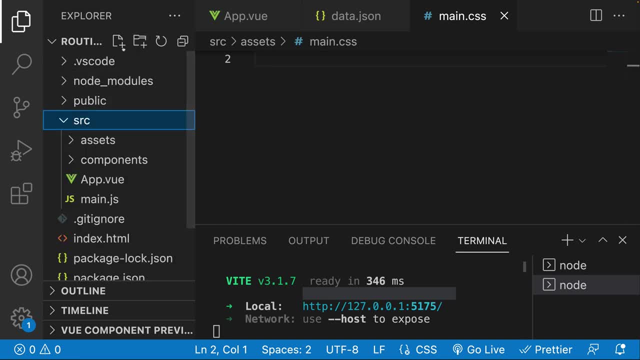 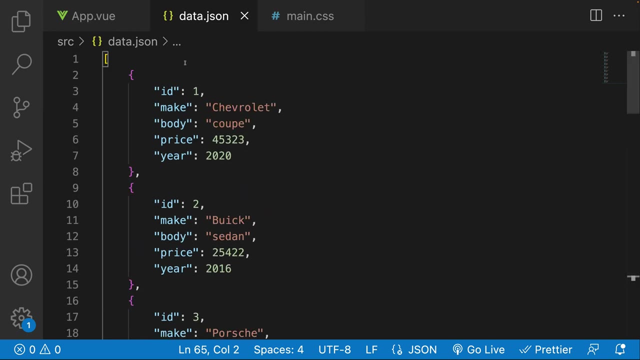 directory and then, inside of your source directory, you're going to create a datajson file and then in here you're going to add that: cars data. Okay, so that is looking pretty good. Let's just clean all this up. Okay, so, this is awesome. So now what I'm going to do is I'm going to utilize this data. 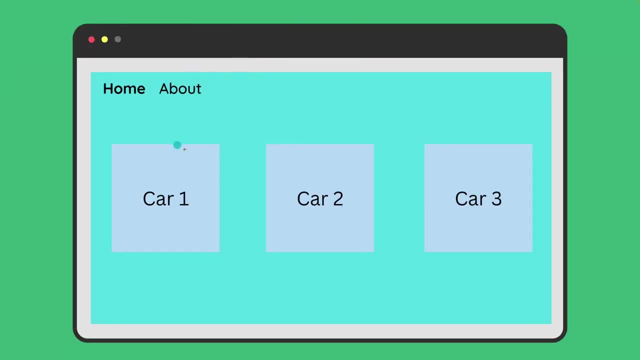 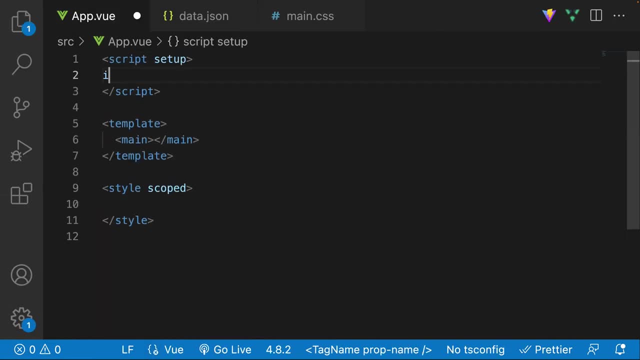 to create again a page that looks a little something like this: So over here, what we're going to do is we're going to go to our appview and let's go ahead and actually import in our cars. So we're going to say import cars. maybe we can call this cars. 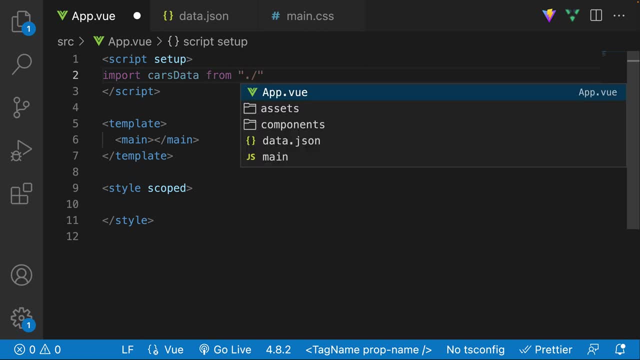 data and we're going to say from, and then over here we're going to say datajson. Now, later on in this course, what we're going to do is we're actually going to start manipulating and kind of filtering through all of the different cars. So the best thing that we can actually do is instead. 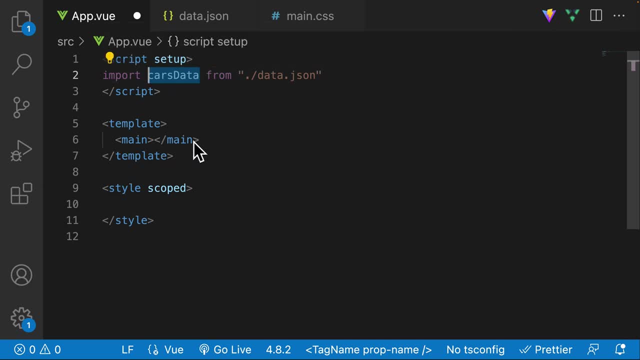 of just using this as an import and iterating over the github repository, we're going to do is we're going to import the cars data within our html. I want to actually store it as a piece of state, So let's go also import ref from. we're going to import ref from view and we're going to say: 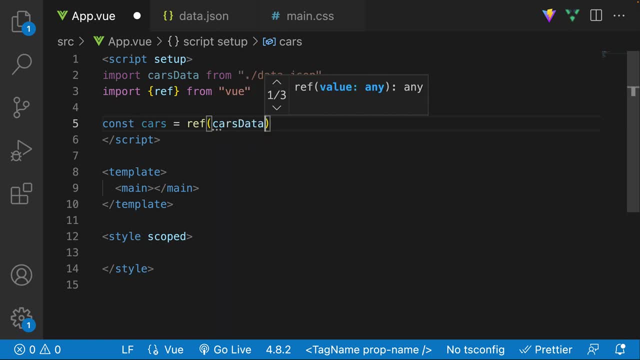 const cars is equal to ref. We're going to say cars data, like so. So that's going to ensure that if we ever update the cars data, our html template is going to re-render and it's going to be inside of the UI. So now what we're going to do, very simply, is just well, create our little app. 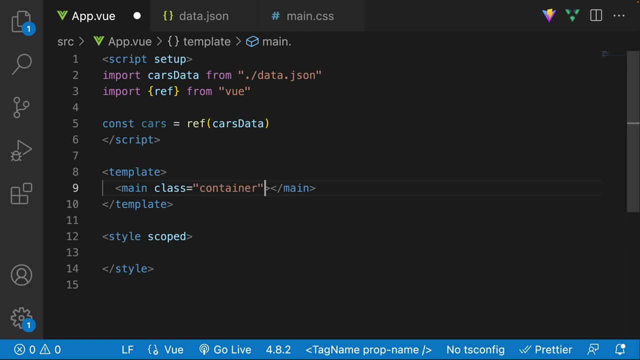 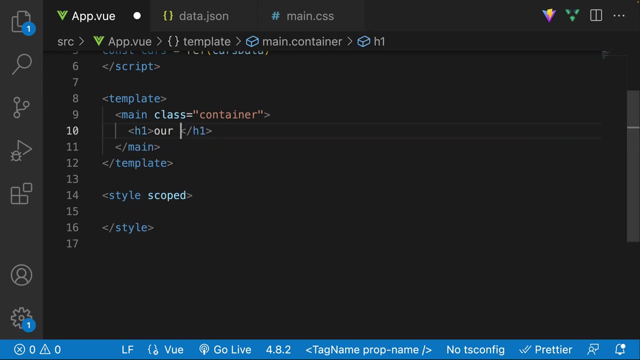 So I'm going to go here to the main. I'm going to give this a class of container and then within this, let's just create an h1.. We're going to say our cars like so, So we're going to have an h1 that. 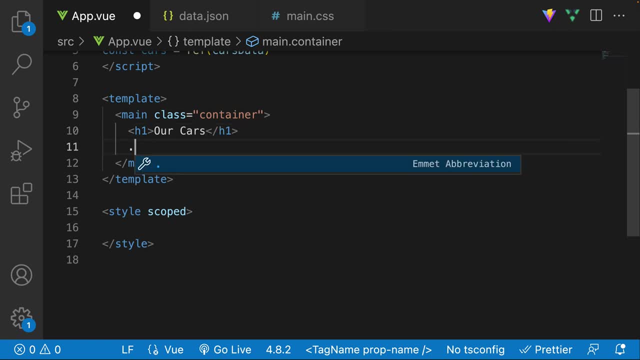 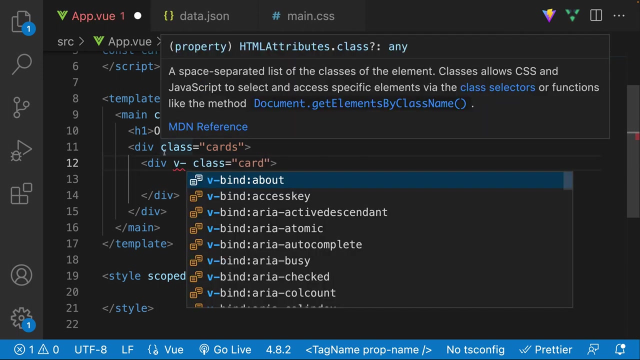 says our cars, and then we are going to have a div that's going to have the a class of cars, And then over here we're going to have another div that's going to have a class of card plural or sorry, not plural- singular, And then over here, this is where we're going to add our v4 directive. So 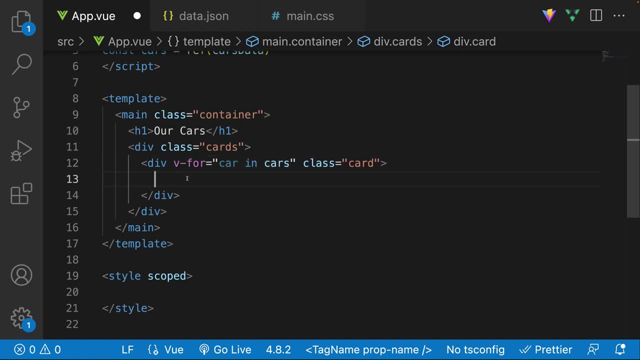 we're going to say v4 car in cars, and then what we're going to do is we're going to go ahead and have an h1 here and we're going to say car and we want to specify the make of the car. So over here. 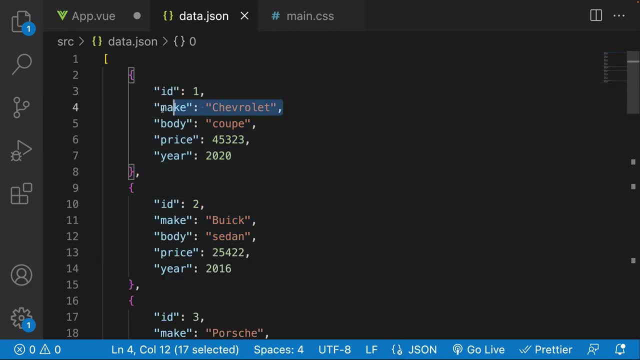 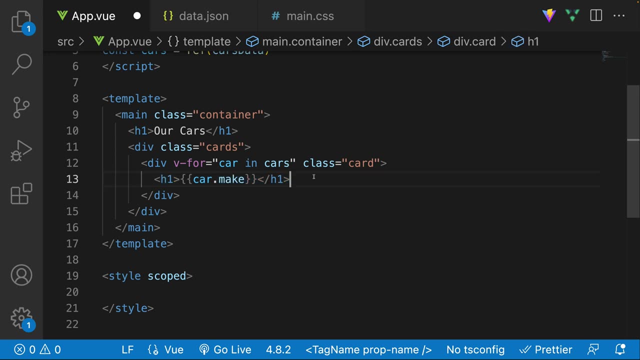 let's just look at the data that we have. So we have an id, we have the make, we have the body, we have the year. So inside of the card itself, we want to tell them what the make is. And let's say, we also want to tell them what the price is. So we're going to say over here, dollar sign, and then 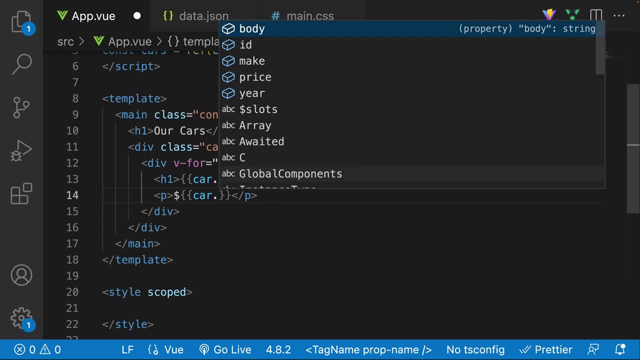 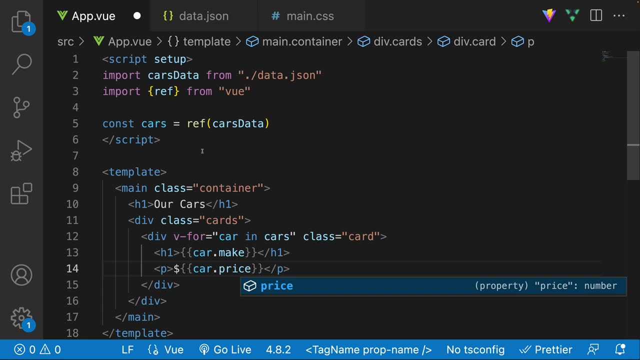 we're going to say car dot price. So this is well very basic stuff. I do expect you to be relatively familiar with this. If you're kind of uncomfortable and you don't really understand what's going on, I highly suggest watching you know view three tutorial video and then come right back to this. 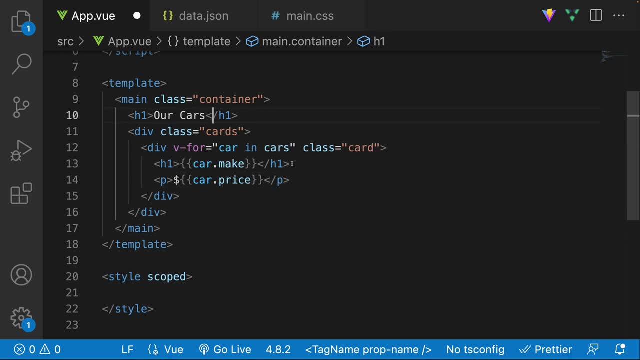 one, Okay. so this, I hope, again makes a little bit of sense. So let's go ahead, and let's go ahead, and over here let's also add our key and we're going to say car dot id, Okay. so this is looking a okay. 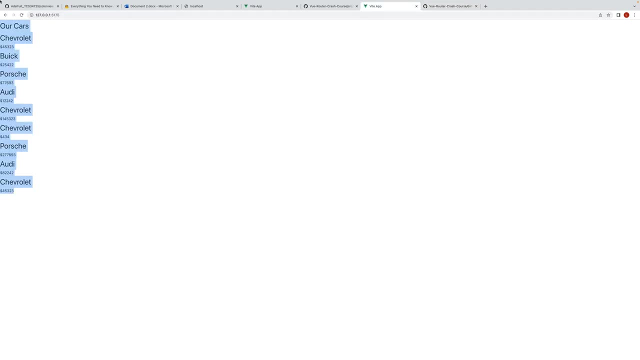 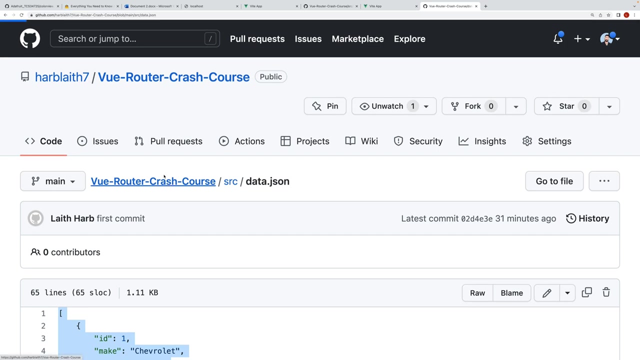 So now, if we were to go to our app here, well, this is what we see. It's kind of ugly, right? So what I'm going to do is we're going to have to add a little bit of styles instead of actually styling it ourselves, and, just, you know, wasting time doing that. Let's go to my repository over here and what? 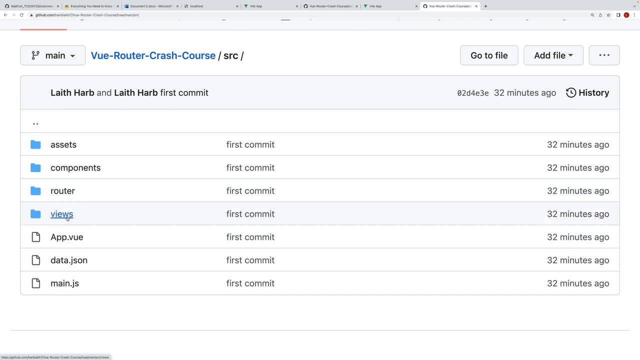 we're going to do is we're going to go to the store and we're going to go to the store and we're going to go to the source. We're going to go to the views and we're going to go to the home view. 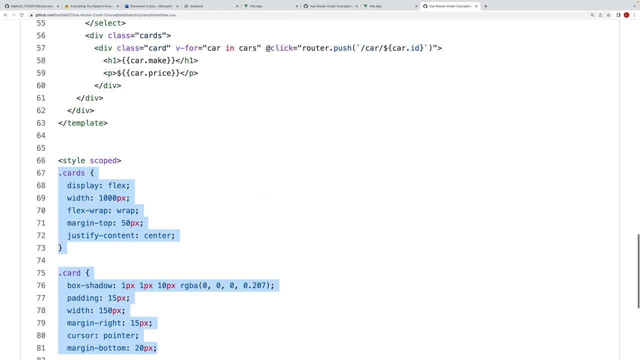 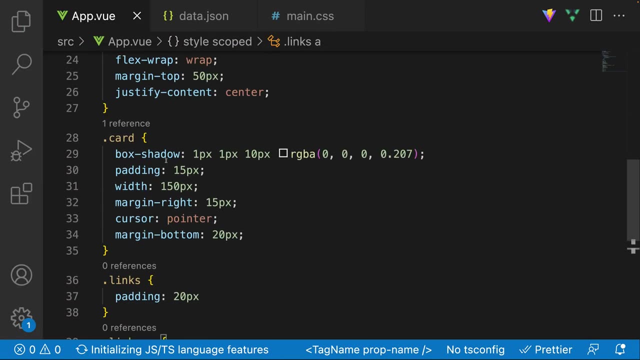 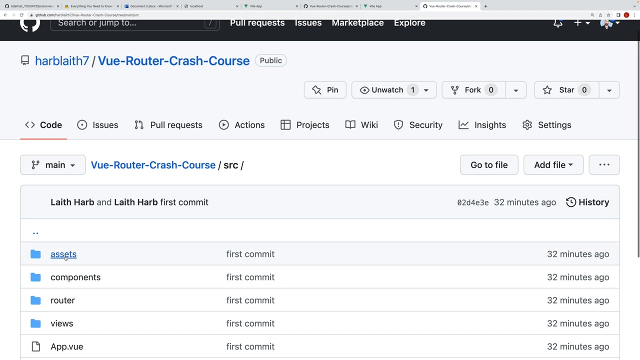 and we're just going to copy all of these styles. So these styles right over here, let's just go ahead and copy them and paste them right here. Now, some of these styles we're not using, but we will use them a little bit later. Another style that we need also need to worry about is inside. 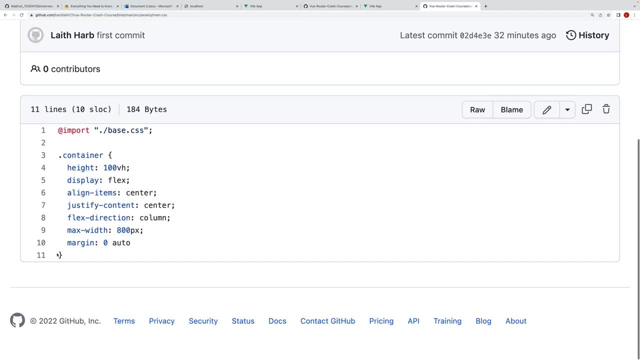 of the assets and then the main dot css. Let's copy this container style and let's also put that inside of the assets. So let's go ahead and copy that and paste them right here. Now, some of these styles we're not using, but we're going to go ahead and copy them inside of our main dot css. So again, 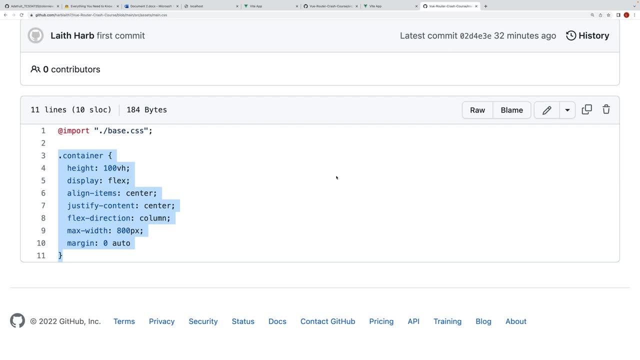 I'll have this repository linked in the description below. You can go ahead and copy these styles as well, because it honestly would have taken us probably like five to seven minutes to style it ourselves, but I don't want to waste time doing that. So now you can see, we have our little. 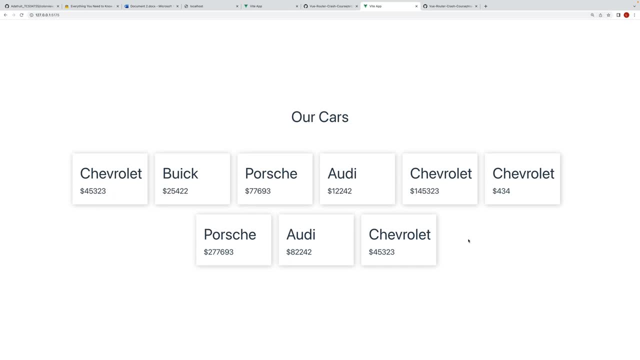 application. Now, obviously it's not beautifully styled and there's no pictures, or there's nothing, but nonetheless, what I'm trying to show you here is now we have multiple different cards that we are rendering, and each- each card- has the make and the style, So we're going to go ahead and copy. 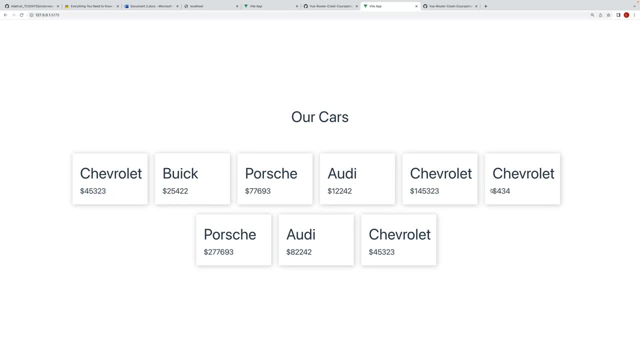 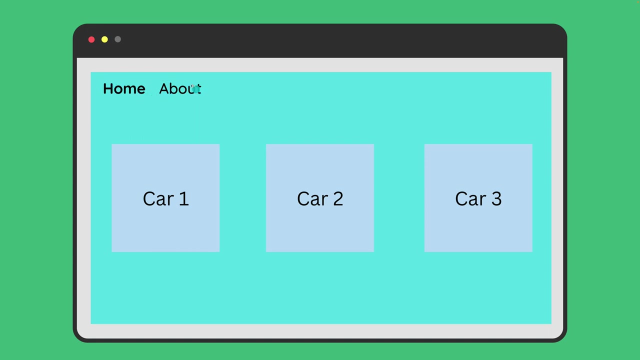 the model part of the template again. So there's our table and we're going to go over here in the animation tips section. so here we go. I'm going to go over here and create a new page. So we're going to go in here and say we want to show a different page and we want to add another page. so 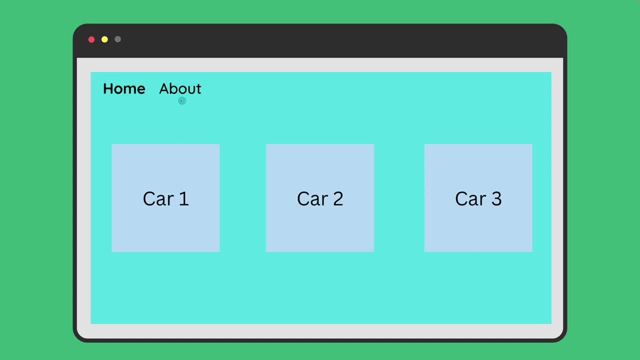 we're going to click on the for page. Now. this page looks pretty good to me. I'm kind of happy with this. but now what I want to do is I want to add another page. I want to add an about page, So rendering maybe another page that has all the information about the about. So to do this, 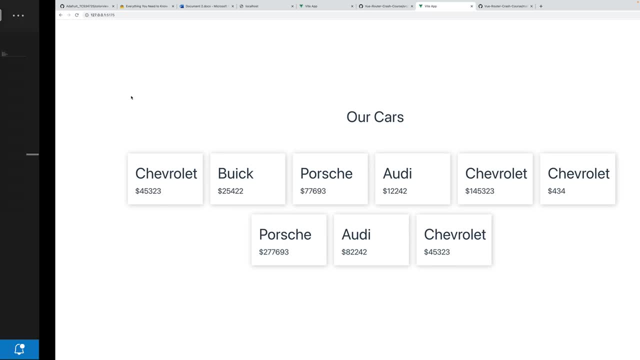 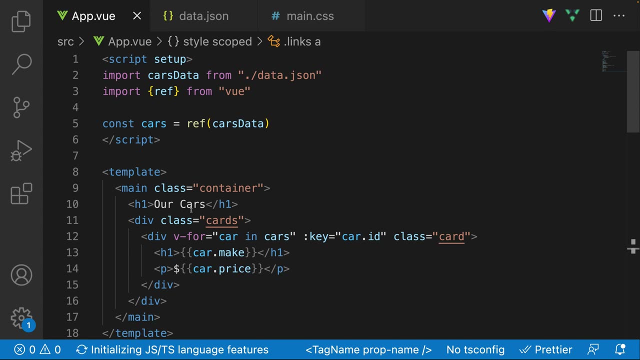 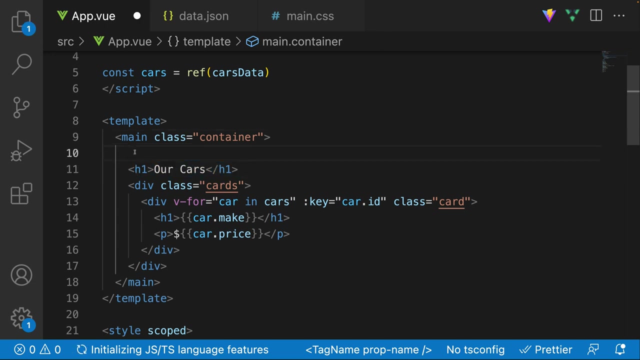 let's first actually go ahead and create our nav bar. So let's go over to here And right over here. this is where we're going to create our navigation bar. So let's create it right above the h1. And right over here again. it's not going to be beautifully styled, we're just going to kind of. 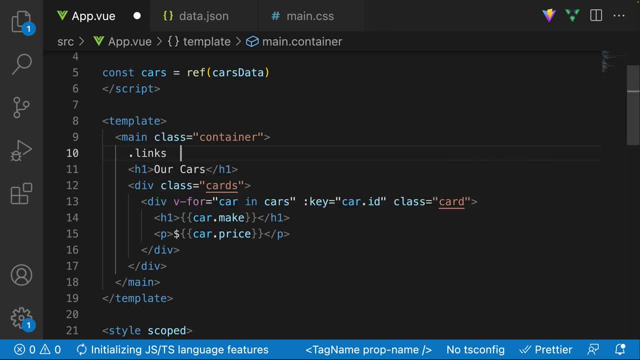 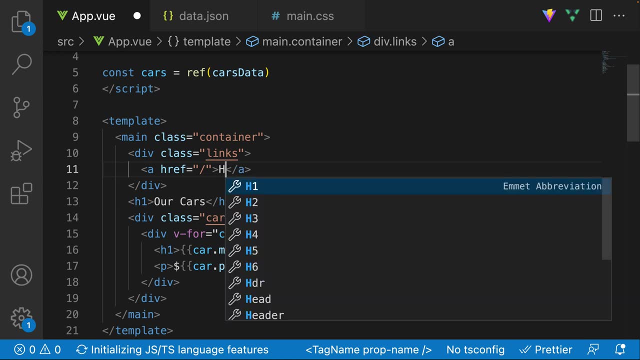 quickly go through this. we're going to create a div called links, And over here we're going to have an anchor tag And the first one is just going to be to the home path, So to slash to the home path. So once you go to local host, this is going to be the home, And then over here we're. 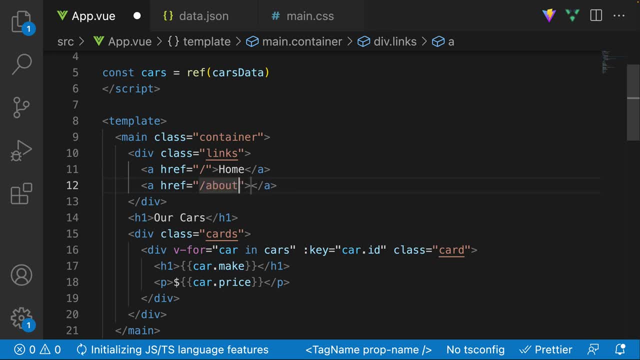 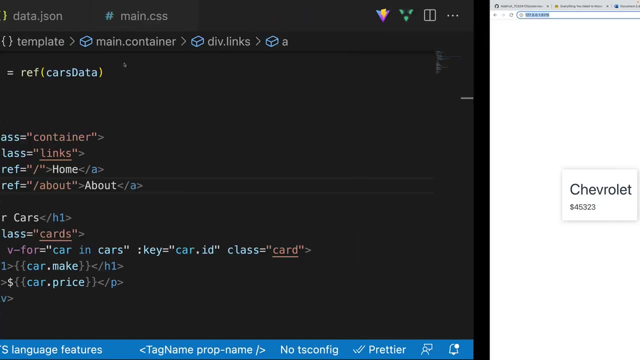 going to have another anchor tag that's going to take us to slash about. So whenever you click on this here, let me go ahead and quickly demo it. Whenever you click on home. I know this is kind of small, But whenever you click on home, this is what we're at. This is the current URL. 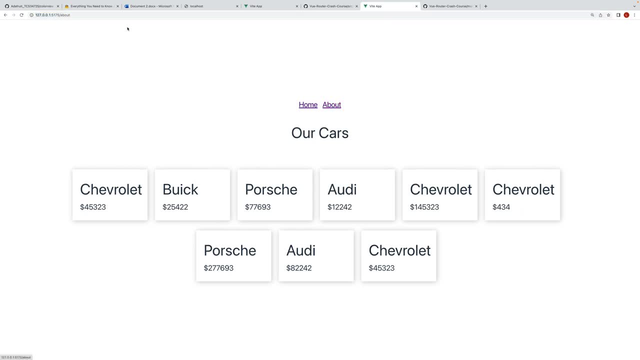 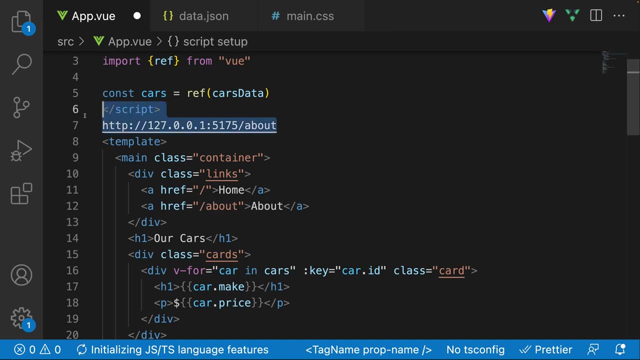 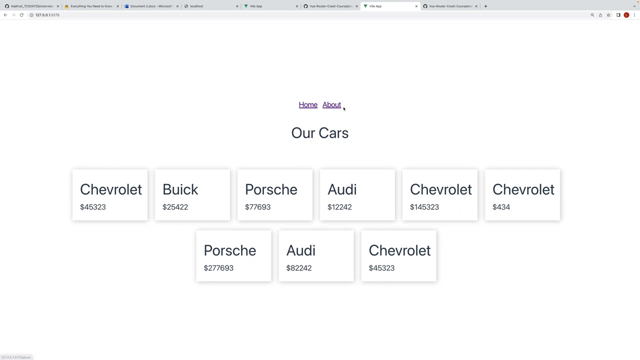 that we're at. However, when I click on about, I'm going to go over here, And you can see here right away I'm on the slash about page, So this is looking pretty good. However, right now, regardless of whether I'm home or about, it doesn't really matter, I'm still rendering the 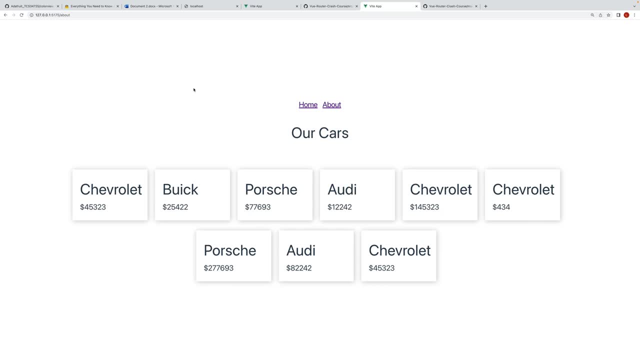 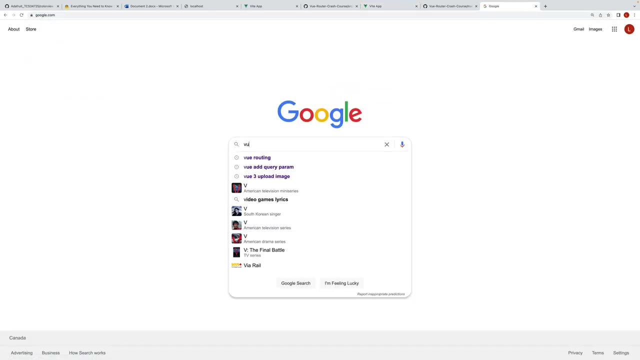 exact same thing. So now, this is where we're going to actually start adding routing in order to start adding pages to our application, And to do this, what we need to do is install a library called view router, So view router. So this is the library, and it's supported by view, And this is the library that we need to. 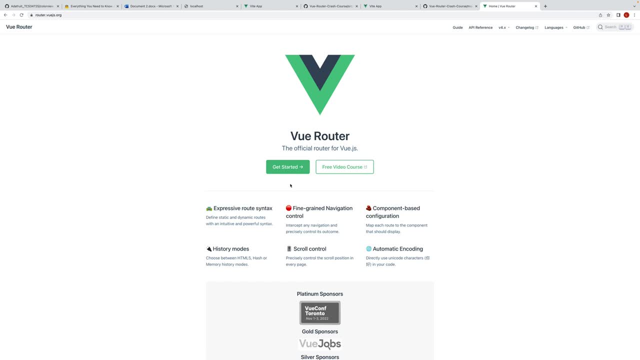 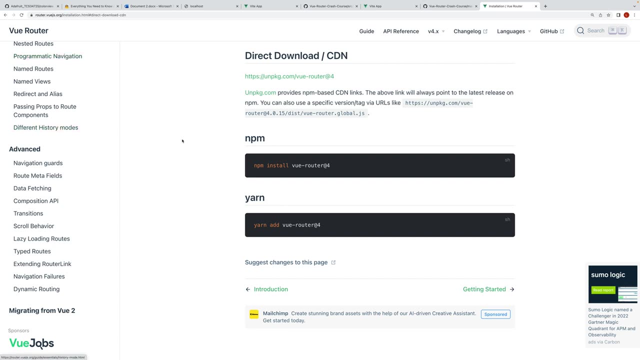 install in order to add routing within our application. you can go to the documentation. the documentation is actually pretty, pretty great. You can see all of the different things that you can do with this library, So it's a very, very popular library. 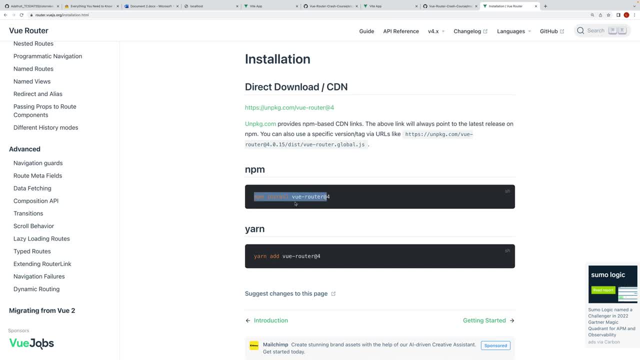 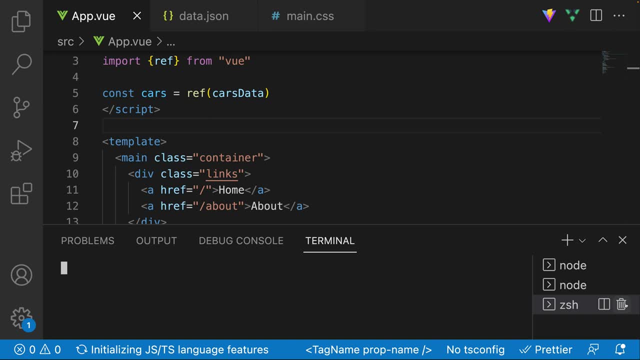 And to install it. what you're going to need is to do an npm install view dash router. So let's go here And we're going to open up a terminal window And let's go here And let's do npm install view. 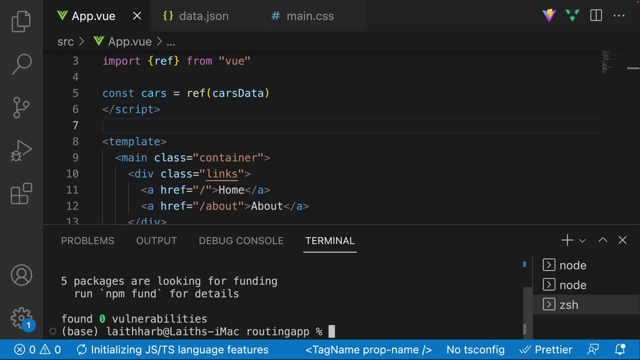 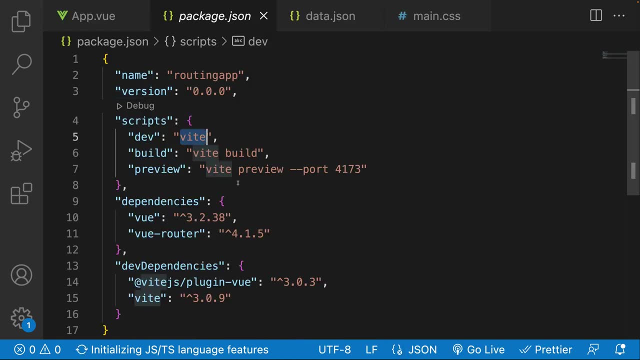 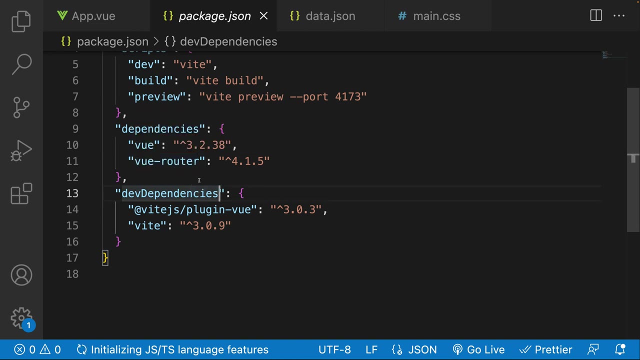 router, like so. So that's just going to install view router into our node modules, And if I were to go to the package dot JSON right away, you can see that we do indeed have view router. Okay, so this is good, we do have the library. But now what we need to do is we need 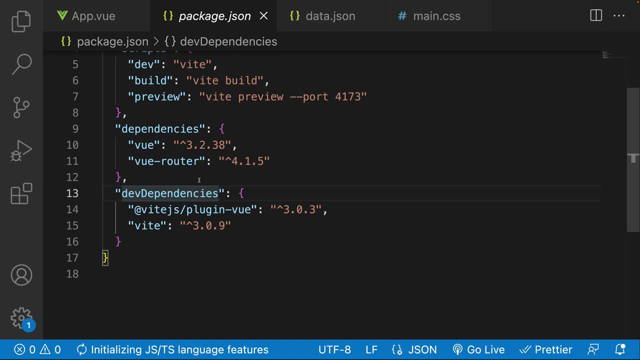 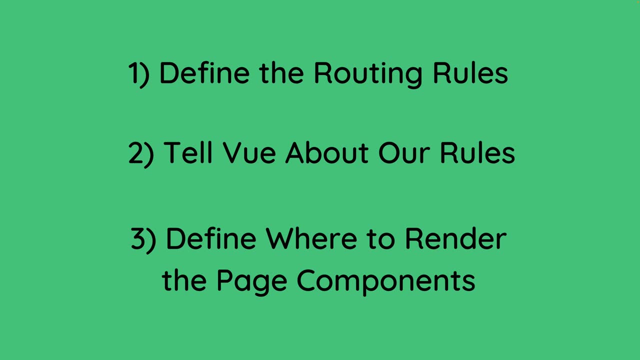 to follow a set of steps in order to actually add routing to our application. So what are these steps? Well, there's three different steps that we need to follow. The first step is to define our routing rules, And I'll talk about that a little bit later, because it's the very 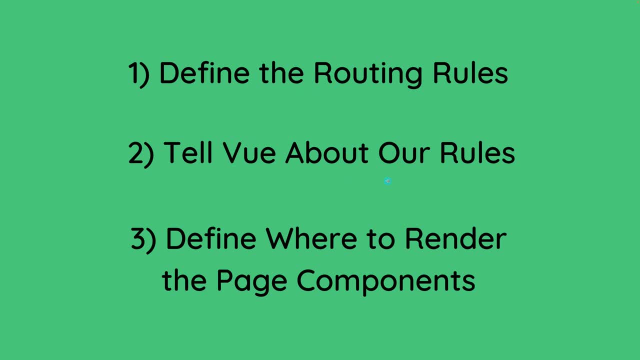 very first step. And then what we need to do is tell you about our rules. So just because we define our rules doesn't mean view knows about them. So we have to tell you about our rules. And then we have to define where to render the page components- And I'll talk about this a little bit later, But for now, 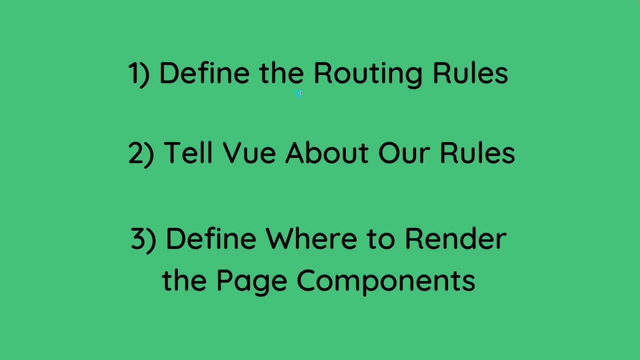 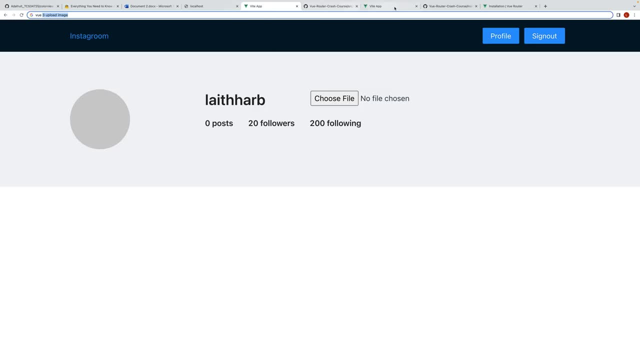 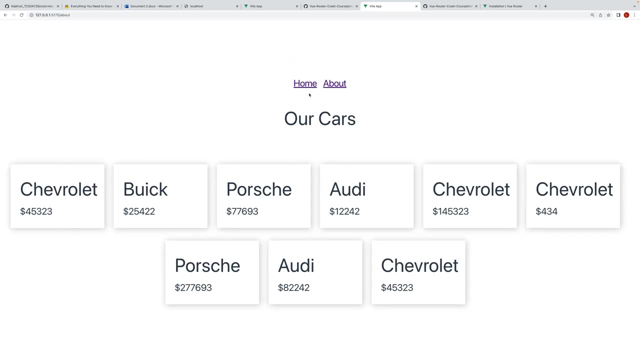 let's go ahead and actually define our routing rules. Now, what do I mean by defining the routing rules? Well, right now, inside of our application, let's go back over here inside of our application, You can see that we have a nav bar that is either going to take us to the slash page. 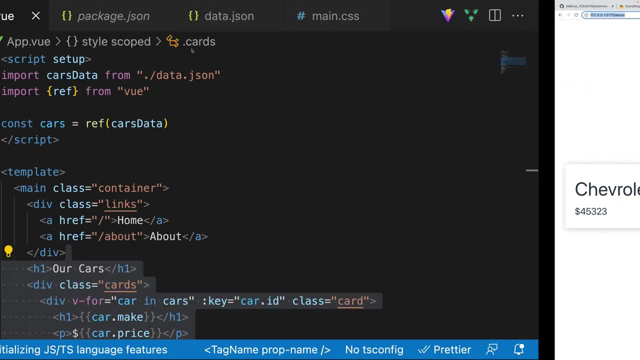 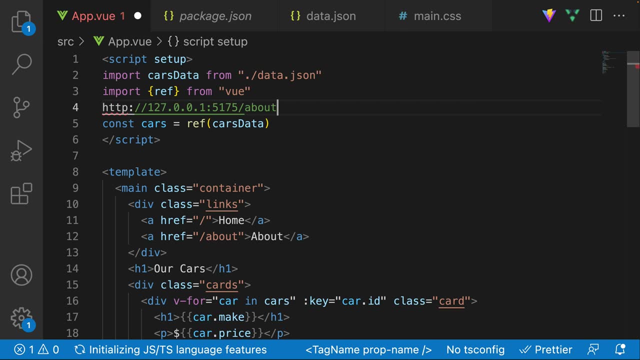 let's just go over here again. So see, they're going to take us. if I were to click on home, it's going to take me to the slash path And then over here, if I were to click on about, is going to. 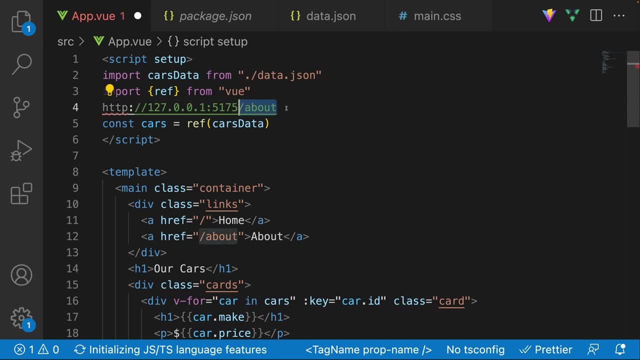 take me to the about path. So what we need to do is we need to tell view, or we need to define exactly what should happen where we, when we are on the slash path, and what should we do. What should happen when we are on the slash about path, Or what should happen if we are on some other. 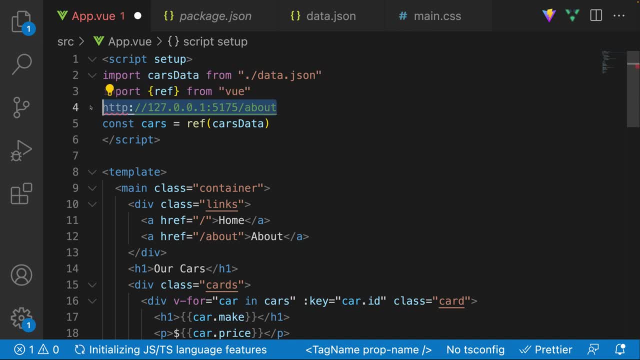 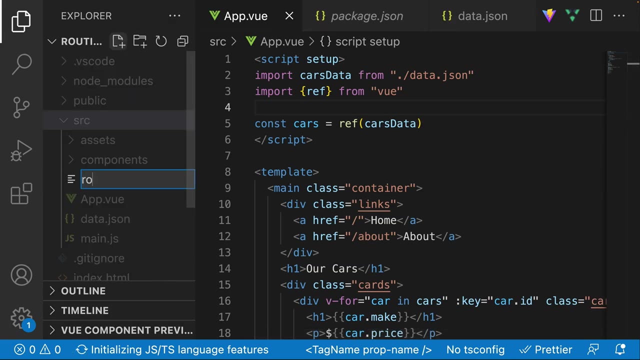 path that we also care about. So those are our rules And we're actually going to define all of those, all of those different rules, inside of a JavaScript file. So typically, the way that it is done is inside of your source directory. you're going to create a router directory, a router. 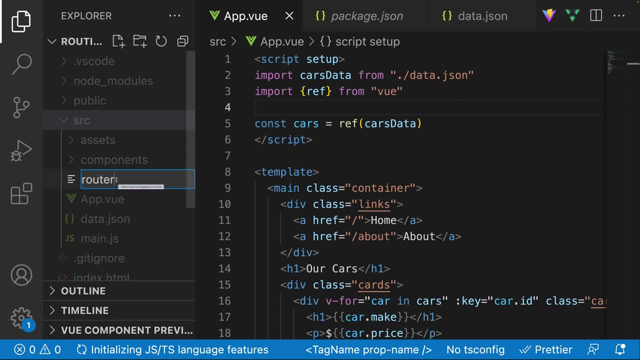 folder. So what I did is actually created a file here. But what I did is I created a file here. but to create a folder within a file, what you can do here is you can say router and then slash, and I'm going to call this index dot j s, And then right in here you can see we have a router directory. 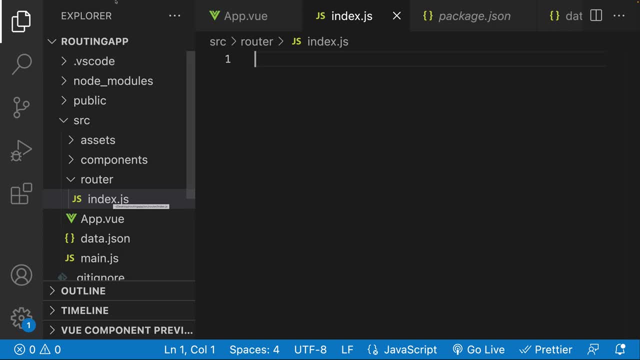 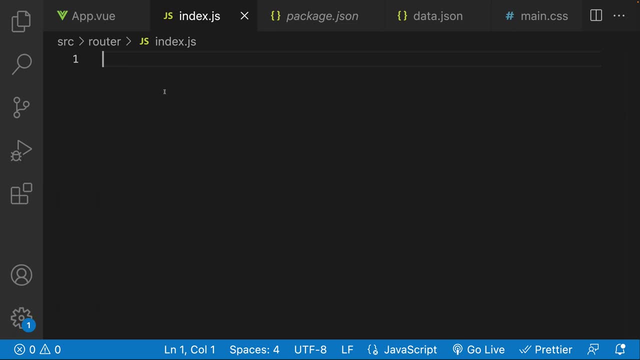 And then within it we have a JavaScript file, And this is where we are going to define all of our different routing rules. So let's go ahead and do that. So to do that, we're going to need to import a few things from that package that we just installed, So we're going to need to. well, 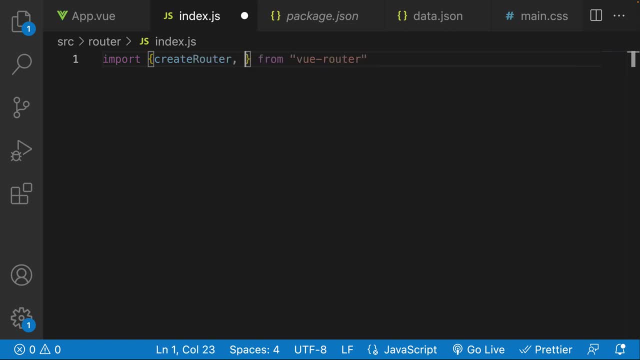 get something called create router, And well, you can probably imagine what this does. And then we need to get another thing called create, And I'm going to say web history. I'll talk about this a little bit later, near the end of the course. For now we'll just kind of ignore it, Okay, so this? 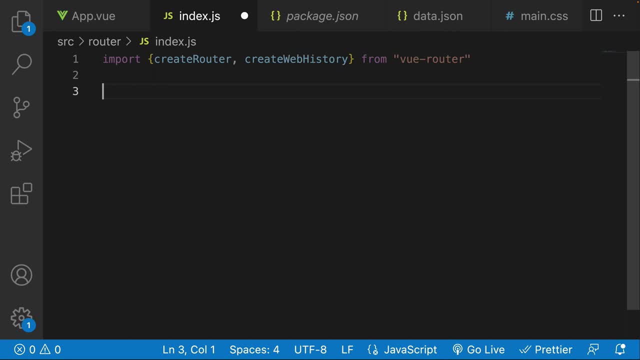 is looking pretty good, And over here, this is where we're actually going to create our routing rules. So we're going to say: const router is equal to create router, And then over here we're going to go ahead and invoke that, And then we're going to say: const router is equal to create router, And 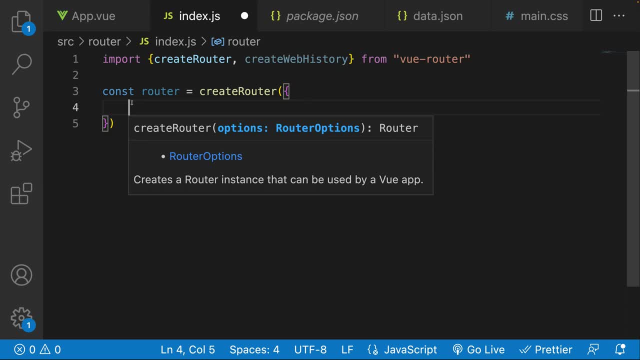 then, over here, we're going to go ahead and invoke that, And then, over here, we're going to go ahead and invoke it, And then we're going to, as a parameter, supply it with a bunch of different options. So the first option we're going to supply is the history. Now, don't worry about this, We'll. 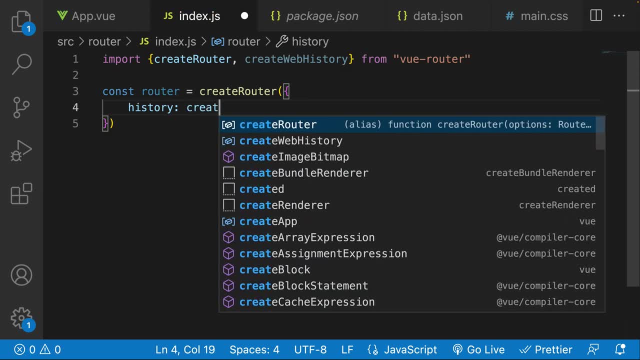 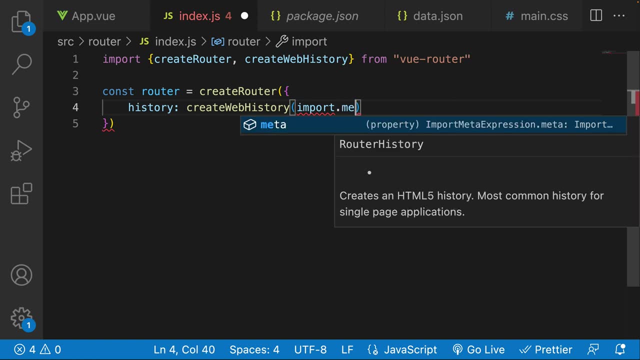 talk about this a little bit later, But this is where we're going to use the create web history. So we're going to say create web history And we're going to go and say import- dot, meta, dot, env, dot, base, underscore, URL. Now this doesn't make much sense to you. do not worry, we'll talk about. 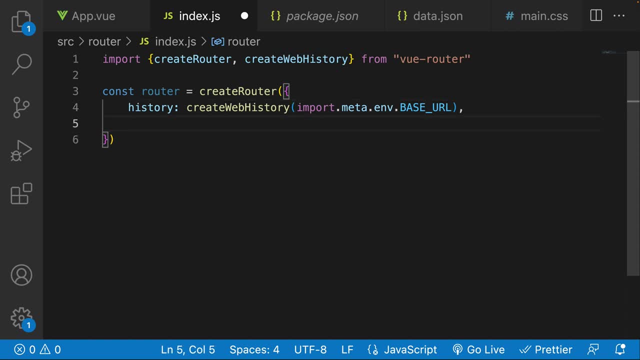 it a little bit later. Now, over here, as the second parameter, we're going to say routes, and this is actually going to be an array, And this is where we define all of those different rules. So over here let's go and let's actually add an object in here Now. 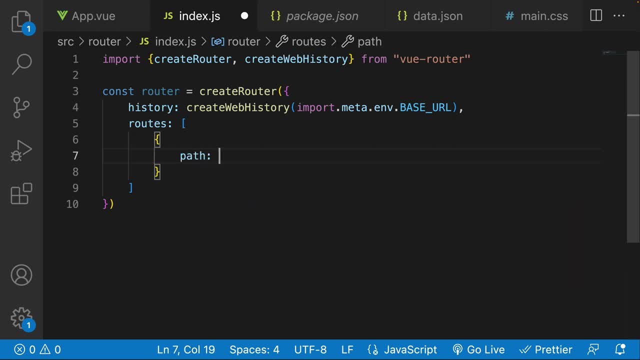 each object is going to take in a parameter called path, And this is the path of the endpoint that we are on. So if we're on the homepage, then it's going to be the slash path. Now let's go ahead and actually give this slash path a name. So let's go ahead and actually give this. 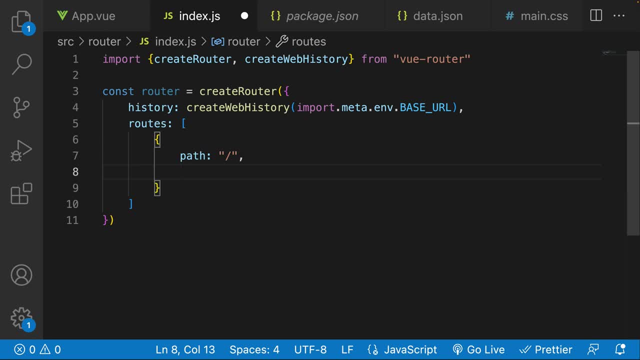 kind of endpoint, or this path, a name, this route a name. I'm going to call this the homepage. Now, over here, what we're going to need to do is define what component we want to render whenever we're on the slash path right over here. So again, let's. let's imagine our website is carscom. 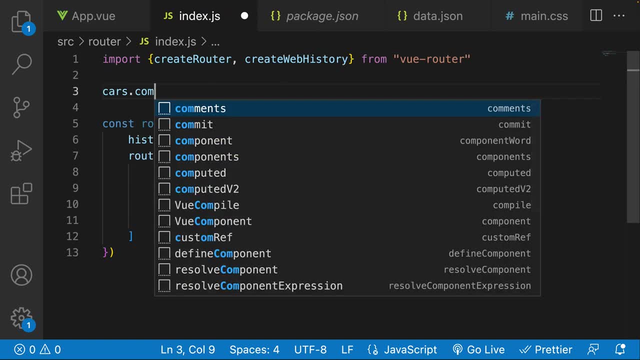 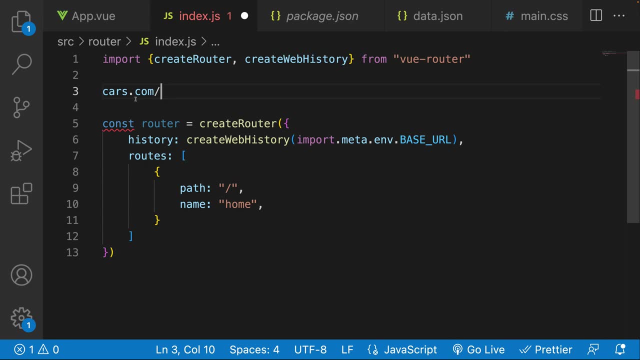 So for carscom, that's what our website is called. If we are on carscom or carscom slash, that's exactly the same thing. I want to render a view component. that's what I want to do. Now, what is the view component that I want to render? Well, I'm going to go ahead and 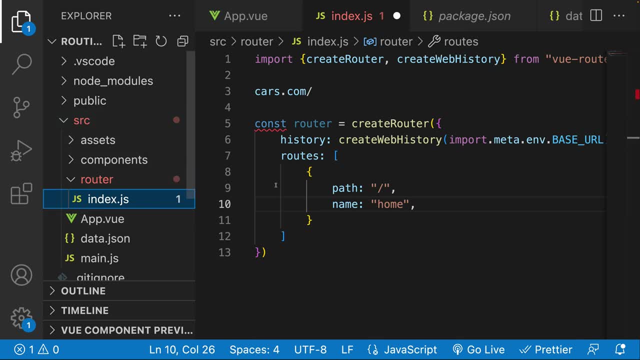 have to actually define it right over here Now. typically these components are called views. So I'm going to go over here, I'm going to say source, I'm going to say views and I'm going to create a home view dot view. 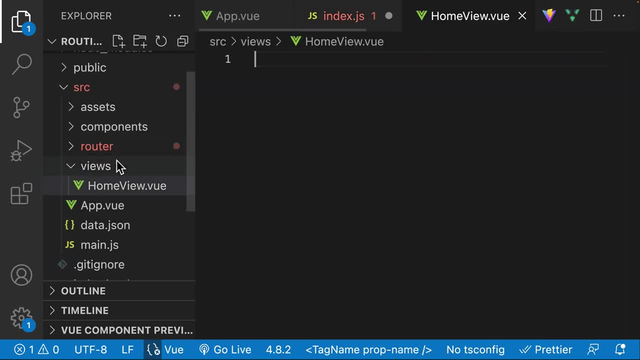 So I'm going to say: home view, dot view. Now, this is just a regular component, but just the convention is to call it views and then home view, dot view. And over here we're just going to create a component And this is the component that we are going to render. 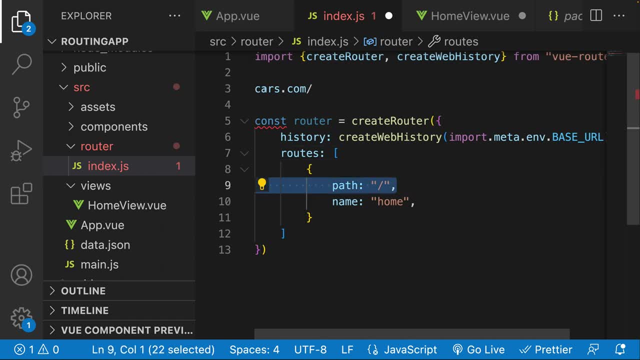 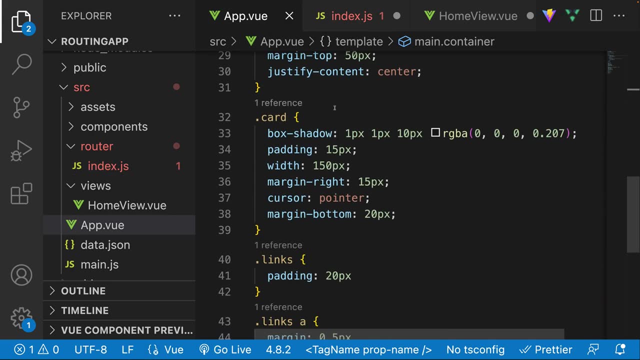 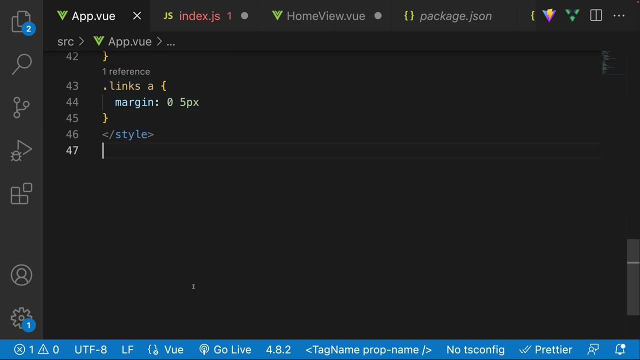 whenever we are on the path slash. So we're on carscom or carscom slash. Okay, so over here let's actually just copy everything we have here inside of this component. So inside the app component, I'm going to copy pretty much everything that we have. I'm just gonna go ahead. 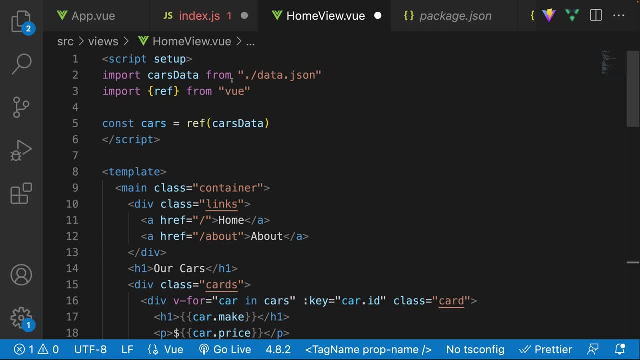 and just copy everything And we're gonna just paste it right here inside of the home view. The data is going to live somewhere else, So it's going to live in dot dot slash data, So the data is going to be a little bit different. And then over here inside of the app component, I'm just gonna 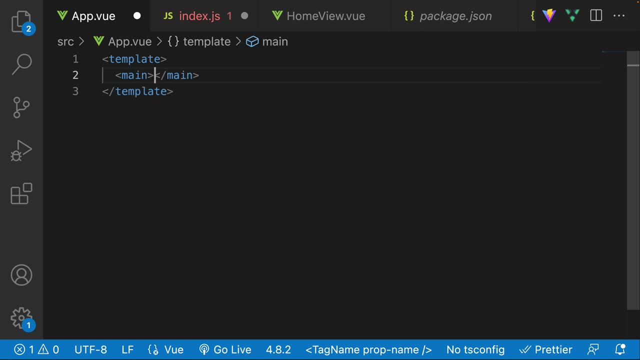 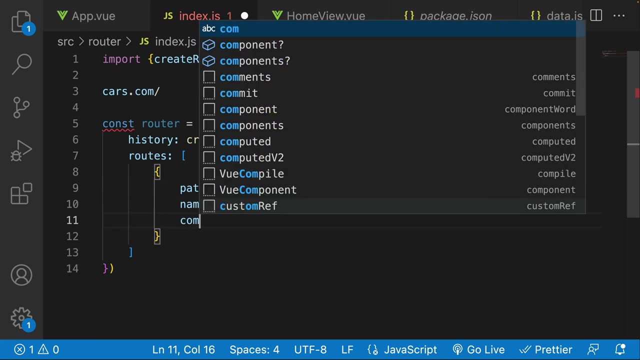 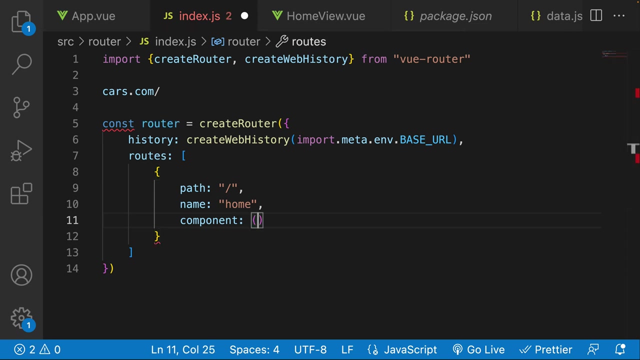 render nothing. honestly, I'm just gonna have a template with a main tag like: so Alright. so now over here inside component, i'm going to say, whenever we're on the path of slash, i want to render the home view component. so what i can actually do is i can call a function that is going to return that component. 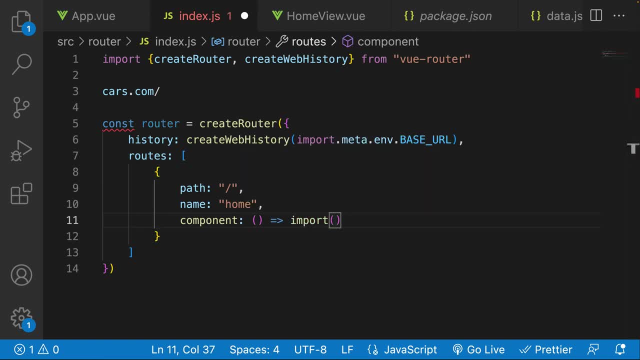 and i can just say very simply: i want to import and i can just specify the path that it's in. so it's over here, inside of the views, and then over here i'm going to say home view, dot view, and what that's going to do is just very simply return that component, this, right over here, this. 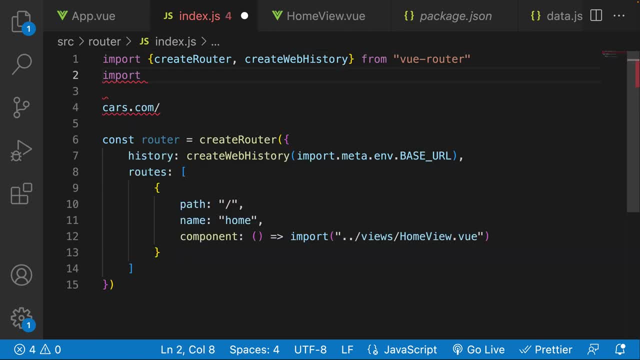 this right here is exactly the same as doing this. so i'm going to say home view and then from, we can just say from views, slash home view, dot view, and then over here we can say home view, like that, and we'll actually go ahead and actually do it this way and we can actually even call it without 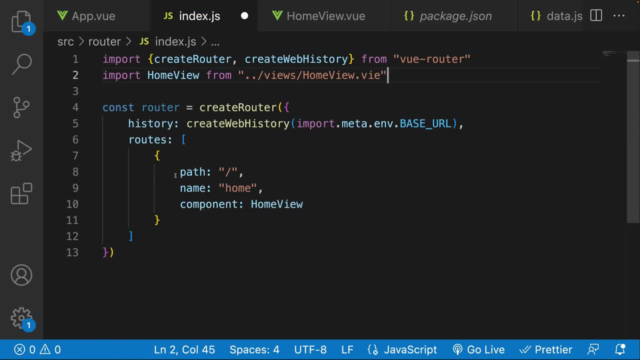 the function itself, because we're just returning it, just because it's just a little bit more complicated. but it's just a little bit more complicated, but it's just a little bit more, little bit more explicit. we're just going to go ahead and do this. so what we're trying to say here 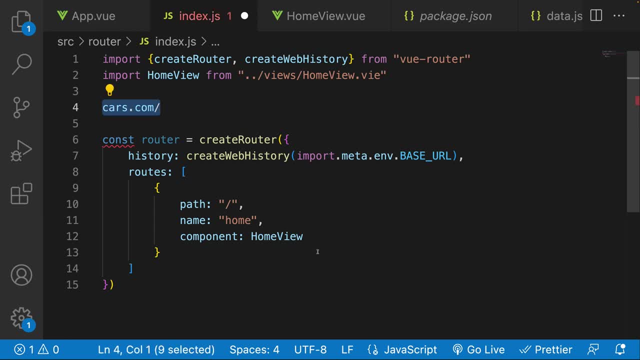 is whenever we're on this path- right over here, the slash path- we're going to render this component. so now what we can do is we can actually add another rule, so whenever we're on the slash about what components do we want to render. so what i can say here is: i can add another object. 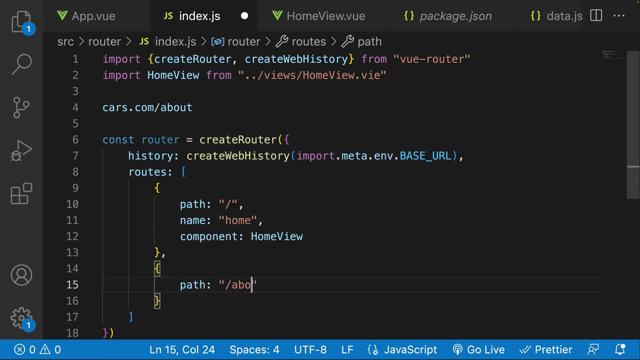 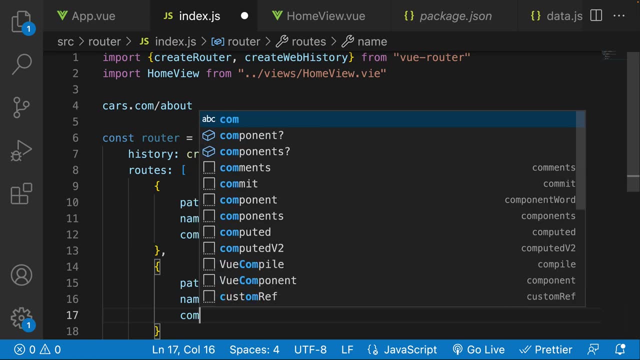 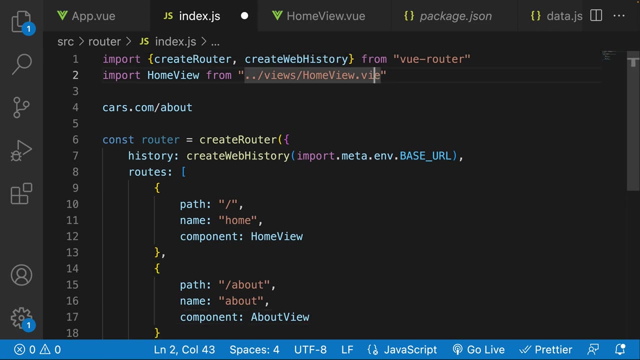 i can specify, okay, the path of slash about, and what i want to do is: let's give this a name of about, and what i want to do is i want to render the- well, i'm going to call this the about view component. now, we didn't create this yet, so let's just go ahead and quickly create it ourselves. 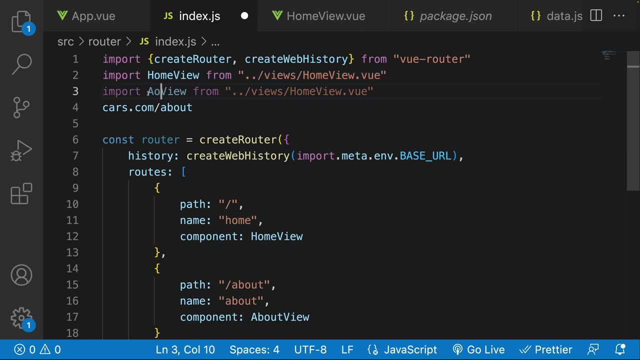 but now let's just first import it. so we're going to say about: about view like so, and then about view like so. i'm going to comment this out for now, and what we're going to do is we're going to create that component, so let's go to our views. 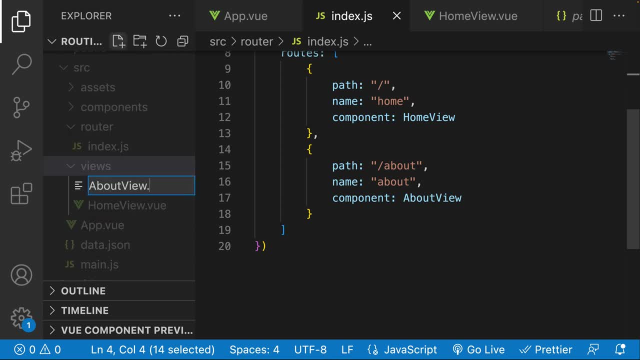 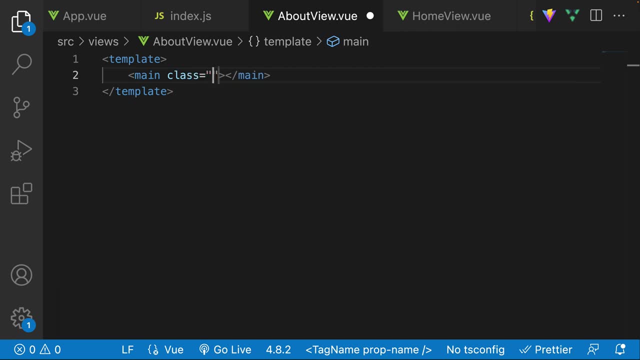 we're going to create that about view, dot, view, and let's go over here. let's create a template, as well as the main, with the class of container, and we are going to very simply for this, let's just add a paragraph with lorem ipsum of, let's say, uh, 30 over here just to get on lorem ipsum, just. 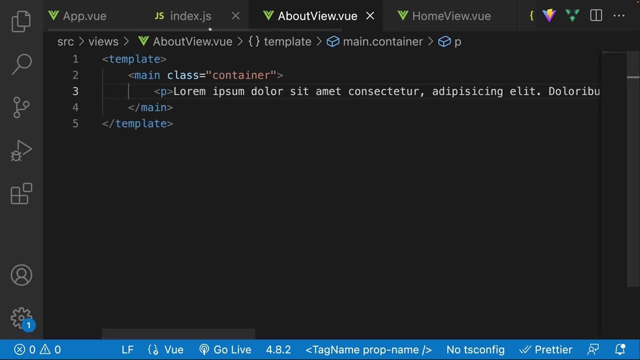 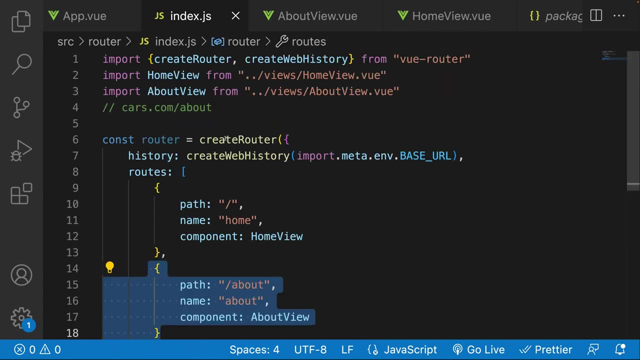 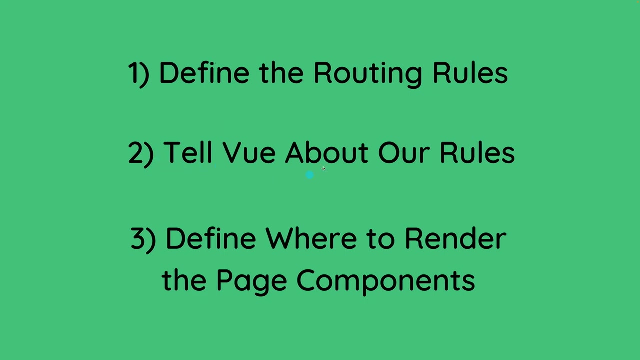 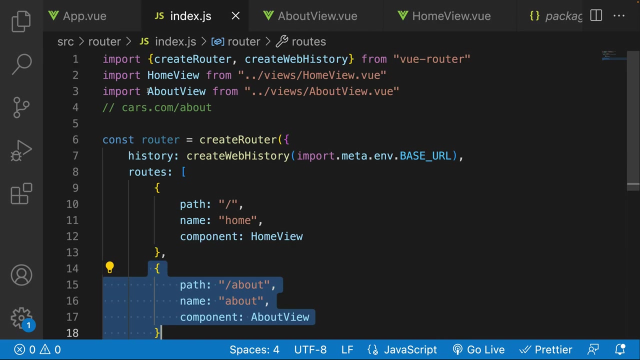 like 30 different texts. so over here now inside of our indexjs, we have defined all of our different rules okay, so this is actually great. this is really good news. so now what we need to do is we need to tell view about our rules. so just because we kind of plop them inside of this file doesn't mean view knows about them, so what? 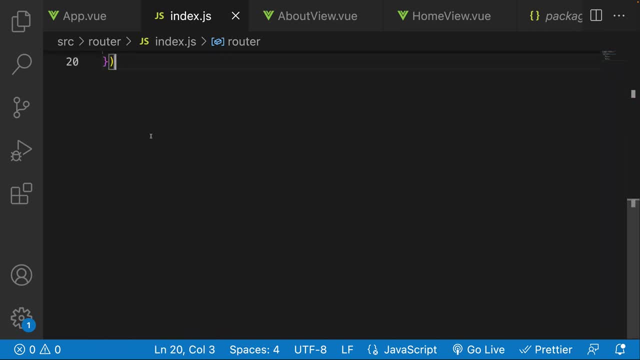 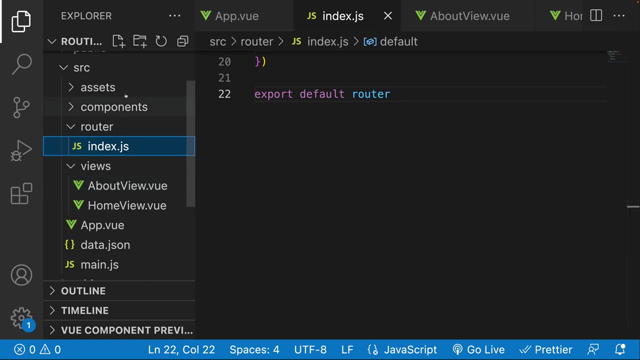 we're going to need to do is actually export this router. so let's go over here at the very bottom we're going to say: export default router to tell view about our rules. we're going to go to the mainjs file, where our view application is actually created. so we're going to say: over here we're going to say mainjs and this: 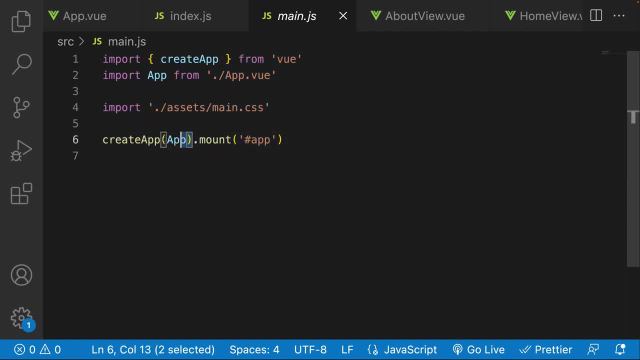 is where our view application is created. so you can see, here we're creating our app and then we're mounting it to this html template that has this id. so, instead of actually doing this, what we're going to do is we're going to cut that out and we're going to say const. 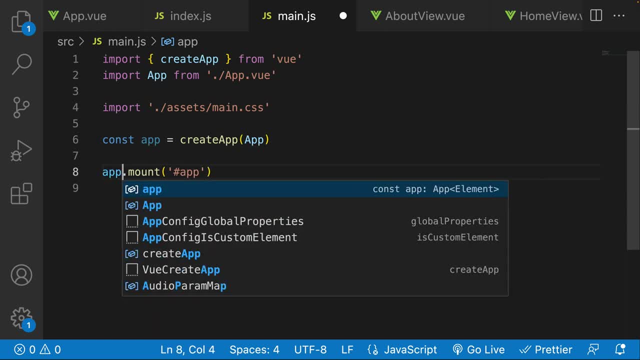 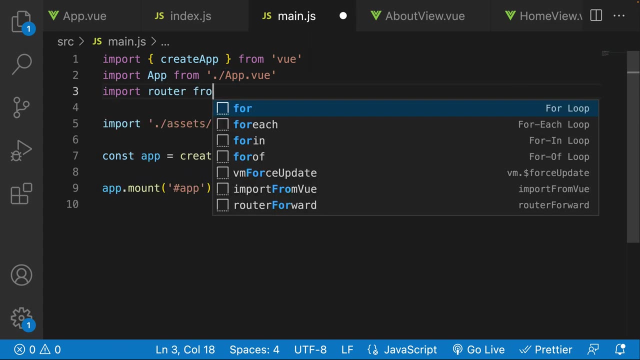 app is equal to create app and we're going to say appmount, like so. now, this is going to allow us to utilize middleware to kind of plug in any different things that we want our view application to be familiar with. now, specifically, we want our application to be familiar with that router that we have just. 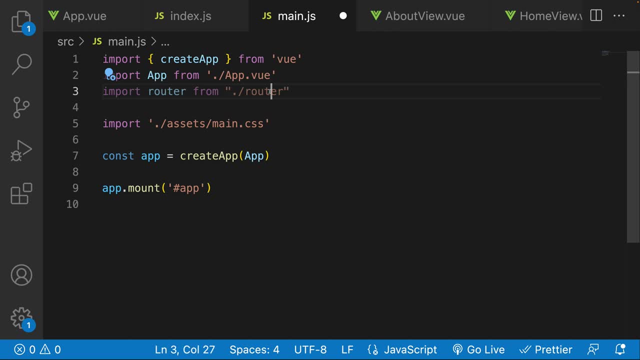 created. so we're going to say here, import router from router, and then we're going to say appuse, and I want you to utilize this router. so if I went out of my window and I went out of my window and I went out of my window and I went out of my 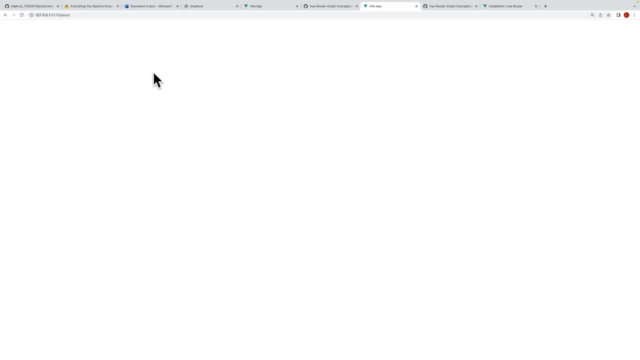 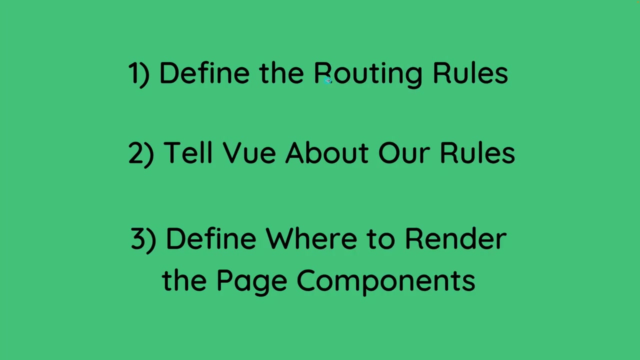 ahead and actually save this. you can actually see that, okay, nothing is erroring out. however, I'm not seeing anything at all, and that's because, okay, we finished this step over here and then we finished step two, but now what we need to do is we need to define where to render the page components. 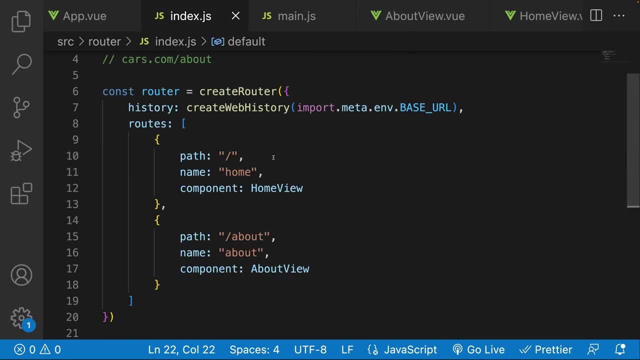 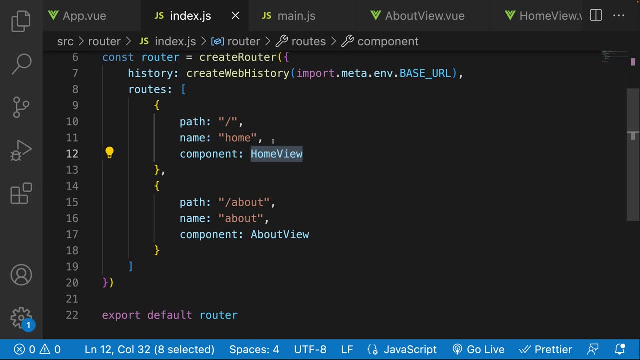 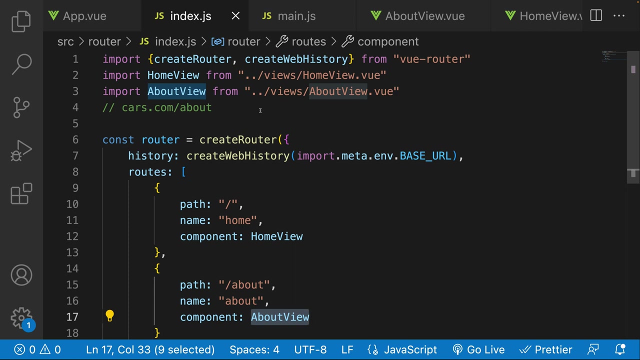 so let's just quickly look at our views again. if we are on the slash path, what's going to end up happening is it's going to render the home view and then over here, if we are on the slash about, it is on the about view. so view actually now knows about this, but it doesn't know where to render. 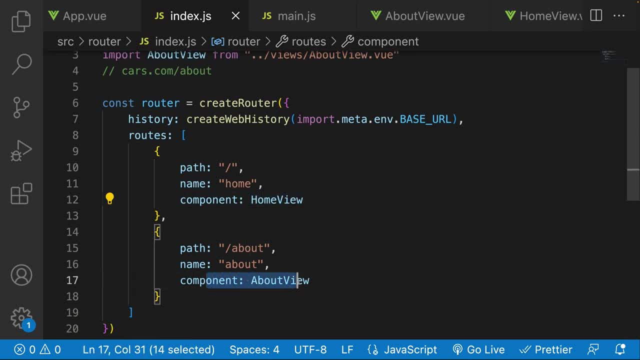 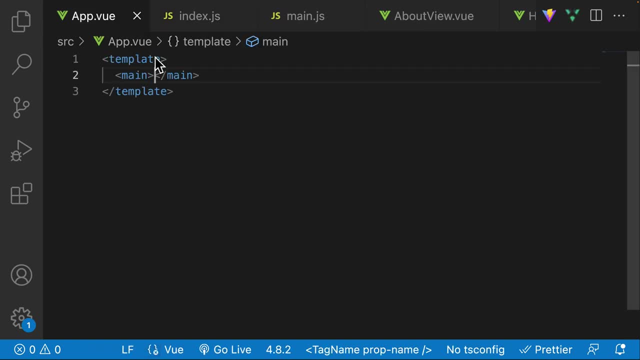 our well, components, these components over here inside of our application, and this is where we actually need to define it. now, what we want to do is we want to actually render it inside of the appview component, because that is our root file, so to define that. hey, this is where we want to render these components, whether it's 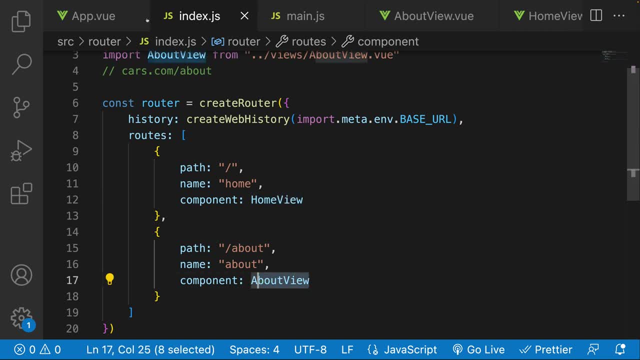 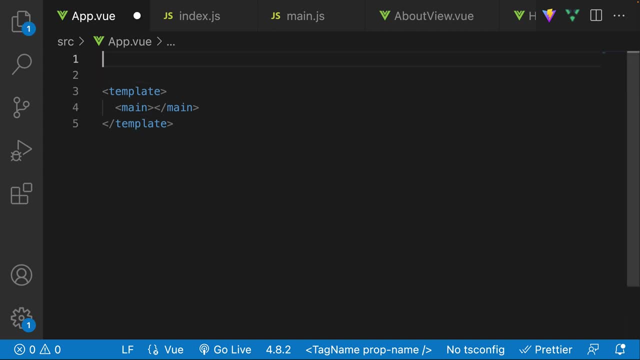 the home view or the about view, depending on which path I'm in. we're going to need to add a little bit of configuration inside of our appview file. so let's go over here and we're going to, we'll do script and setup and we're going to import something from view routers. we're going. 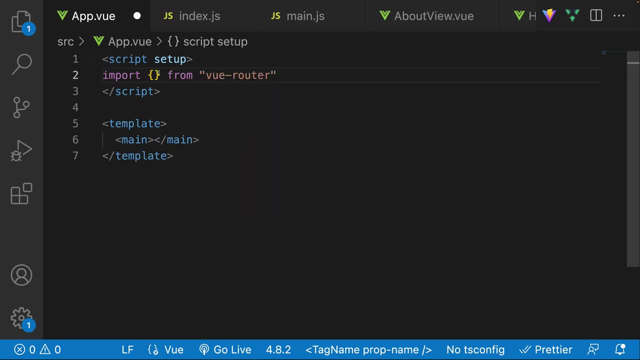 to say from view router. we're going to import a very special component called router link and we're going to go ahead and just render router link within our app. and sorry, not router link, sorry, router view. we're going to go ahead and render this right below or right in between our 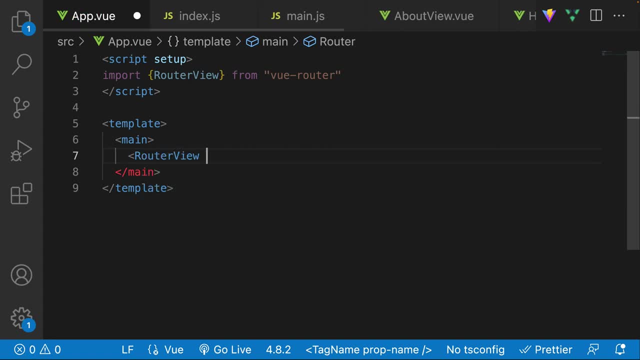 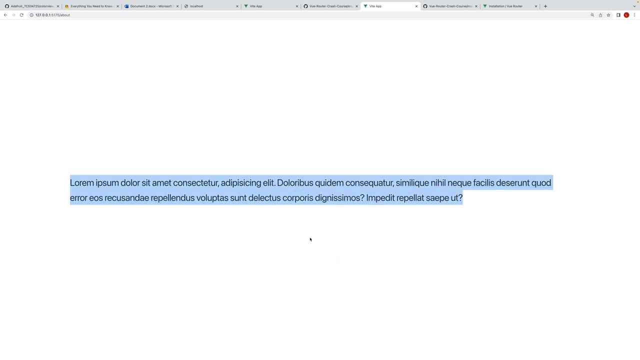 main tags. so we're going to say router view, like so. so now if we actually went to our application, you can see. tada it is indeed working. how wonderful is that? so you can see, our lorem ipsum is actually being displayed because of our appview. 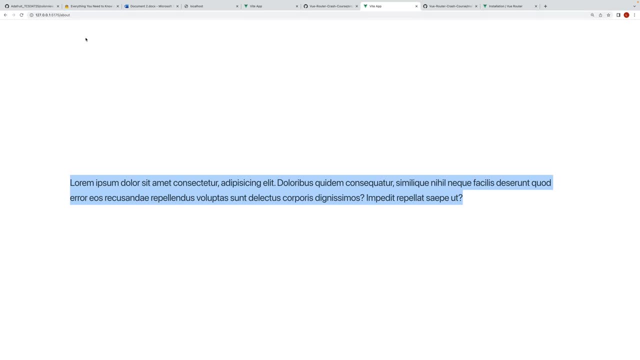 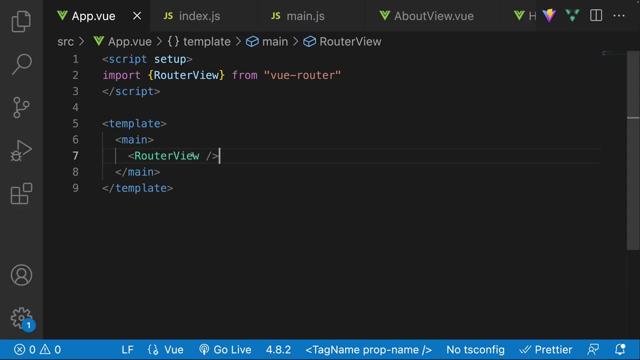 right now we are on the slash about page. now this isn't that beautiful, so let's just go ahead and quickly try to make this just a little bit nicer. I don't really care all too much about the styling, but I just want to make it a little bit nicer. so we're going to say here: h1. we're going to call. 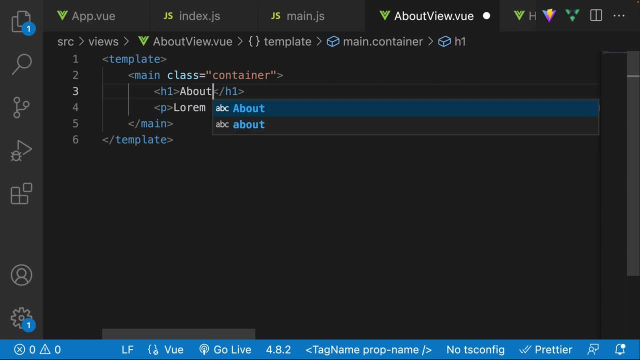 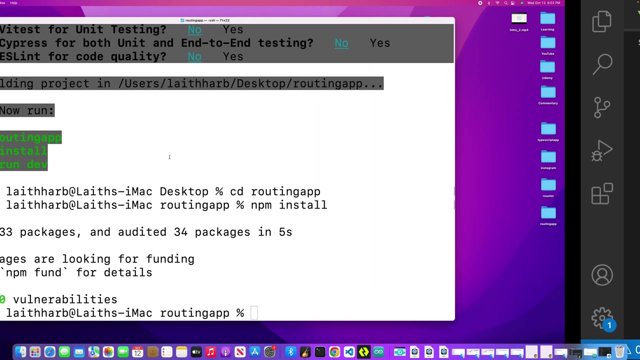 this the about, just so we know that this is indeed the about page. and over here, in the styles we're going to add scoped, we're just going to say the paragraph, we're going to give it a text align of center, all right, so now you can see that this is the about page. 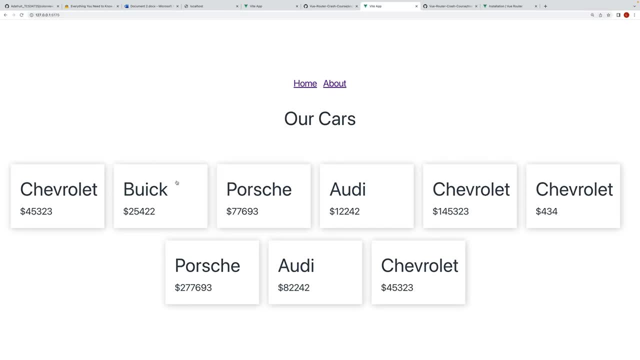 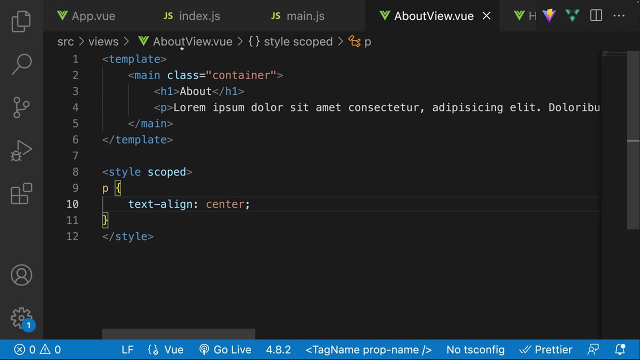 and if I were to go to the slash page, you can see we are now indeed taken to our cars page, so now we can kind of plop back and forth. so what's actually happening here? well, right over here, this router view component is a very special component. what it does is it listens and looks at. 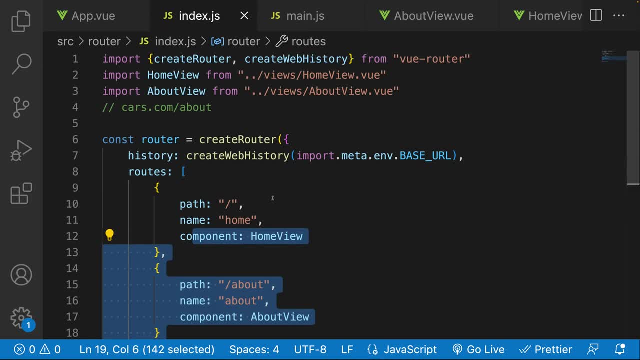 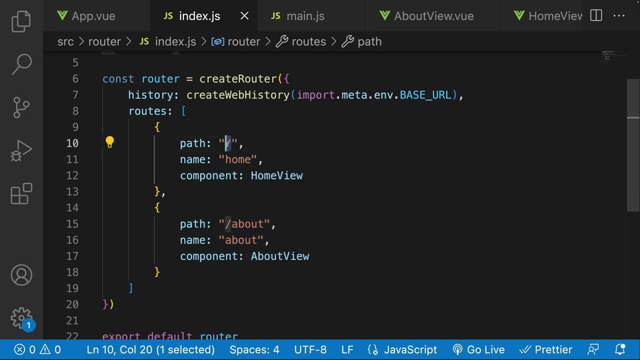 our. well, it looks at our rules and it looks at our rules and it looks at our rules and it looks at our rules that we have defined. and so what it does is it sees: okay, right now we are on the slash component. if we're on the slash component, I am going to kind of change this router view component. 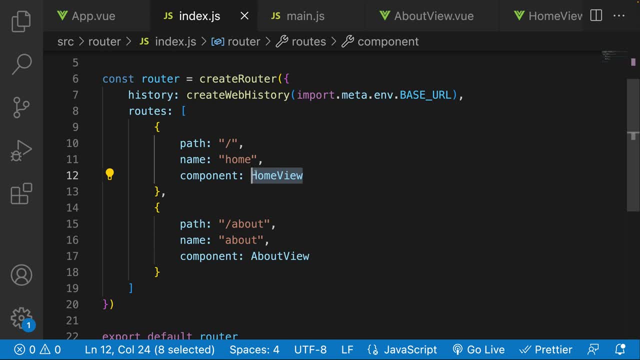 to this home view component. so I'm going to render this home view component and I'm not going to render this about view component. and then if we are to change the path again to slash about, then this router view component knows that and then it removes the home view component and renders. 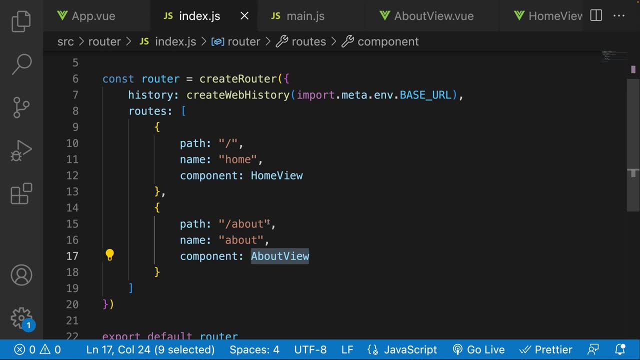 the about view component. so at the end of the day we're just kind of shifting components back and forth, which makes sense because view is a single page application. it is a client-side rendered application. so we're not making html requests and we're not making http requests to get different. 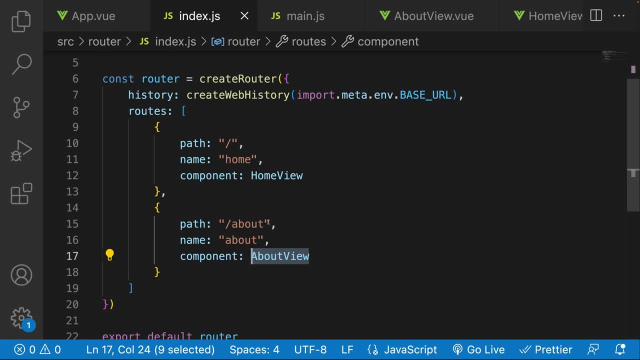 html files. we're just shifting our components back and forth and kind of giving the illusion of having multiple different pages. so that is exactly what we're doing, and that's pretty much all it is that we need to know in order to route our stuff. so this right here is kind of the fundamental knowledge that you need to. 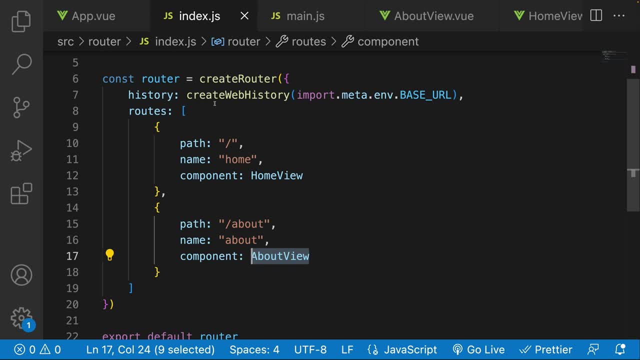 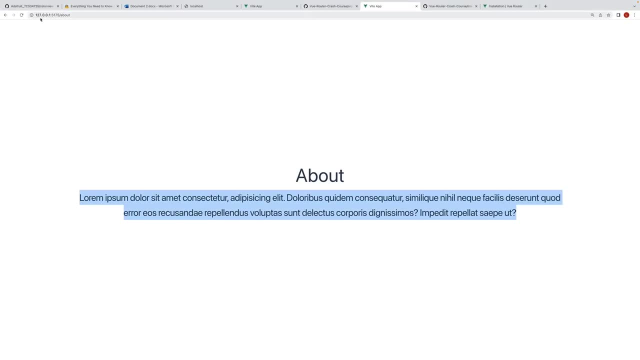 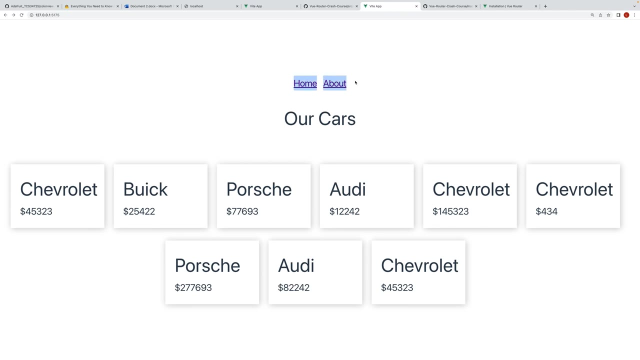 know. everything else is just kind of extra knowledge that you can gain in order to make your application even better and better and more dynamic. now, one thing that I actually want to do before we move on to the next section is I want this right over here, this, this nav bar, to appear. 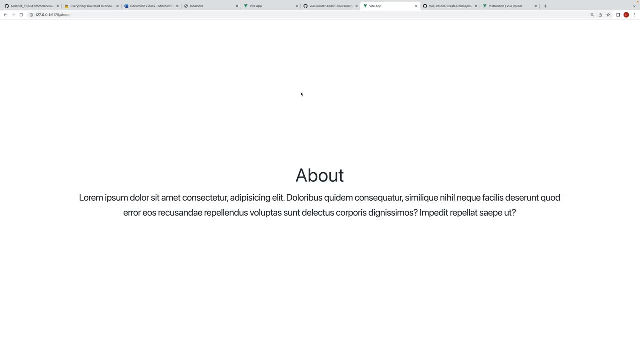 both on the home view as well as the about view. in fact, I kind of want it to appear on every single page so the user can have the ability to navigate to wherever they want, regardless of what page you're on, because right now you can see that I'm on the. 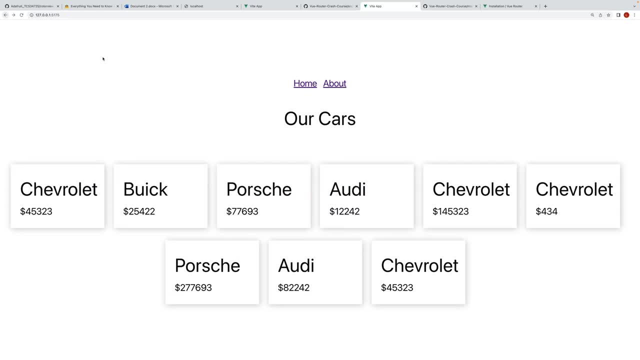 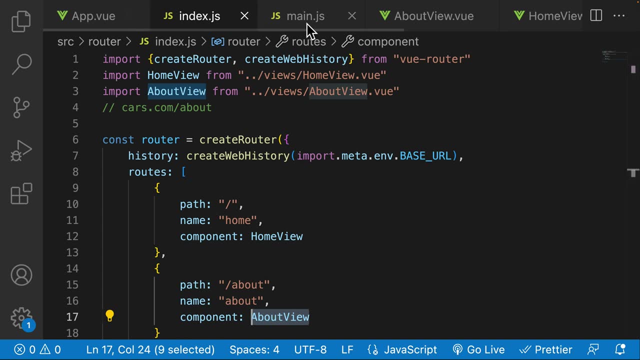 slash about page, there's no real way for me to get back other than to click back or to change the path manually. so that's not a very nice experience. so what we're going to do here is we're going to go to our home view, where our application is being rendered, and we're just going to kind of cut. 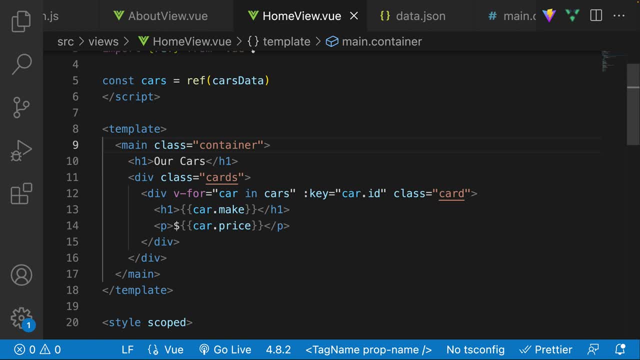 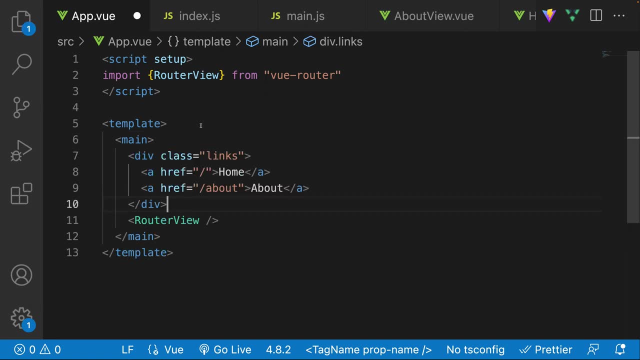 everything out. so we're going to cut these links out. I'm going to go ahead and just save that and I'm going to go and paste it inside of here. so I'm going to paste it right here. so now you can see that it is indeed rendered right here and I can. 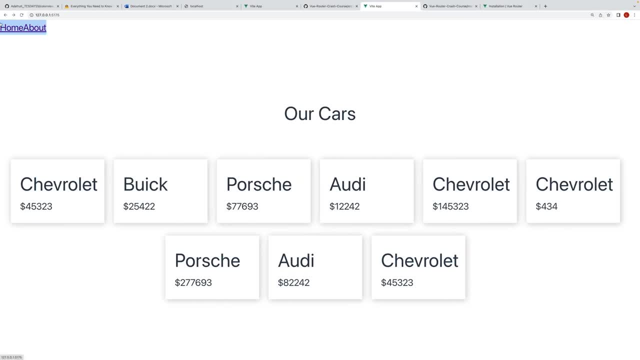 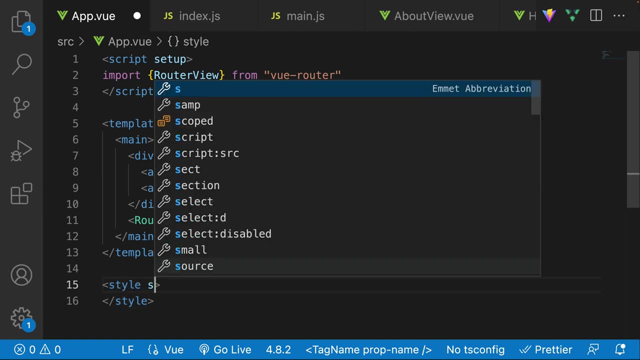 actually put this inside of a container, but let's just say our we like our nav bar right here now. also, what we can do is we can style it as well. so let's add some styles to this. we're going to say scoped, and we can just kind of get these styles. 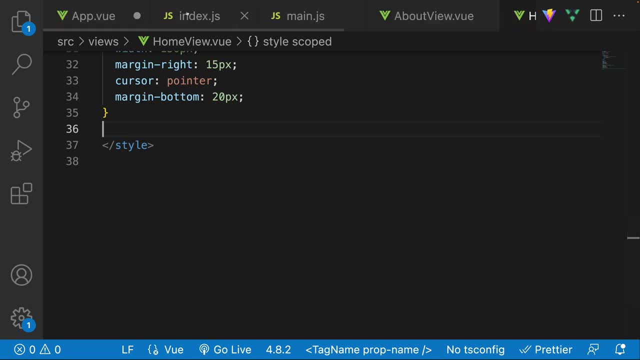 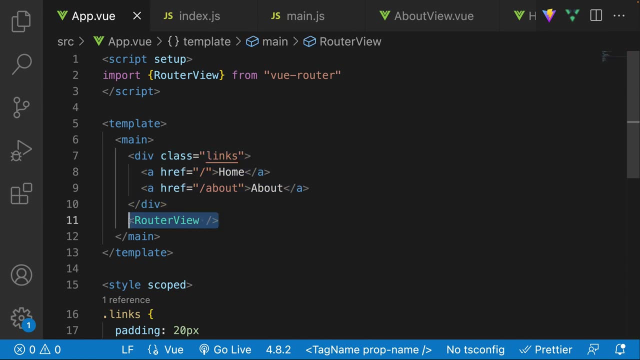 these link styles, cut them out and we can save them right here. so what's going to happen is our app view components is going to render these, and then it's also going to render whatever page that we're on, so that way, we're always going to have our nav bar. so now what we can do is we can move. 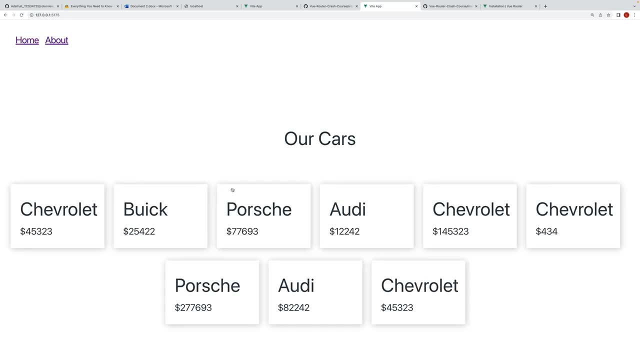 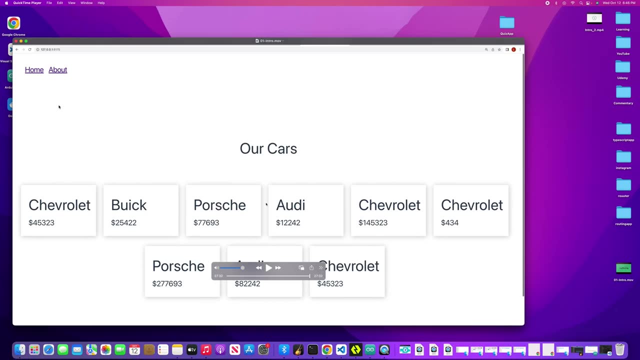 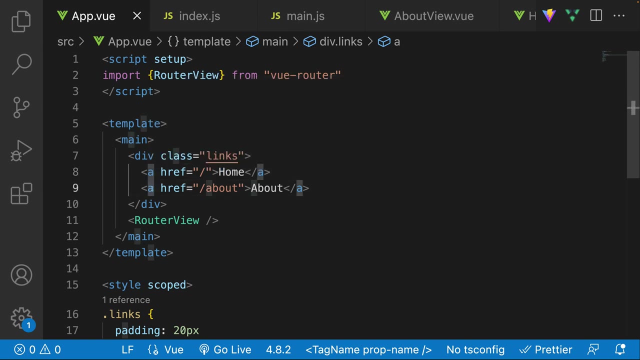 to the about, we can move to the home, we can move to the about and we can move to home. so this is pretty cool. speaking of the nav bar, there is a potential issue with what we have thus far. so right over here. our navbar is using anchor tags, and the issue with anchor tags is that it 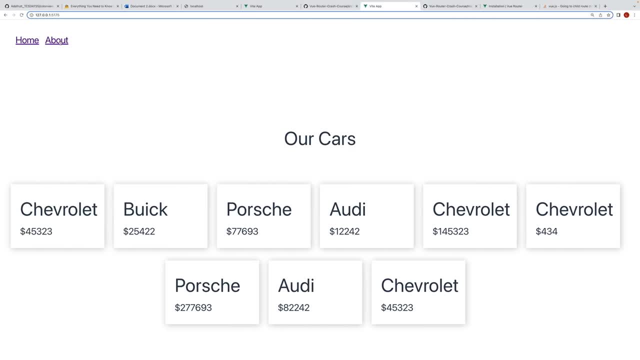 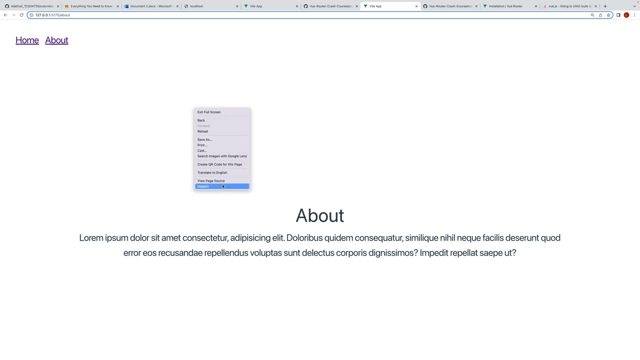 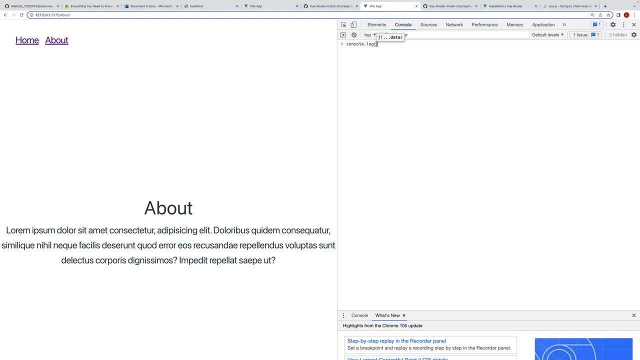 actually reloads our whole application. so, yes, indeed, it does move us to the slash about, but it does reload our app and we can actually to see this in multiple different ways. so over here, let's just say I went ahead and I consolelogged hello, so just say hello and I were to go ahead and just consolelogged this inside of the browser, like we went ahead and I smoothly did and let's see here, add a new function. as you can see, we can go ahead and change this as a mountain as you go and you'll see the app has cleans up the program and anyway, you can see here I've got a number of things on the. 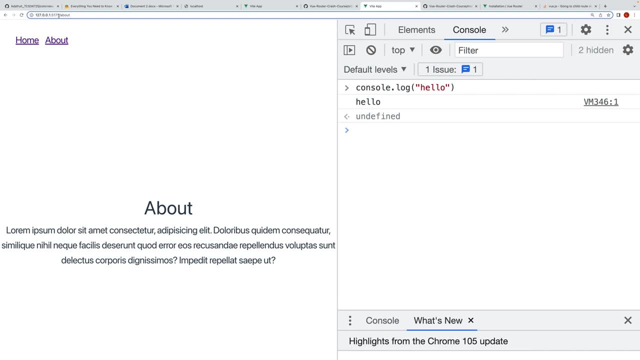 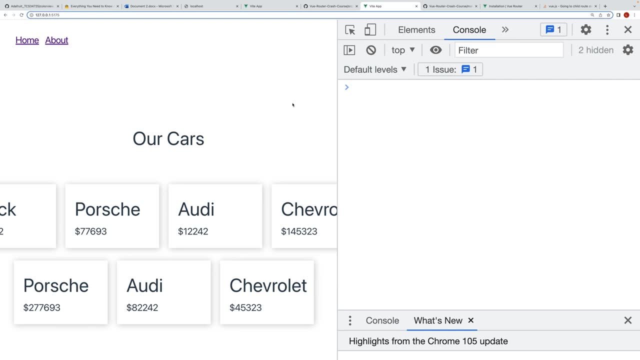 left hand side. that make sense. we have two processes here, and one is newца, to look at it, and the other inside of the console itself. if I were to click on home, you can see that our whole console is now refreshed, because we pretty much reloaded our application. 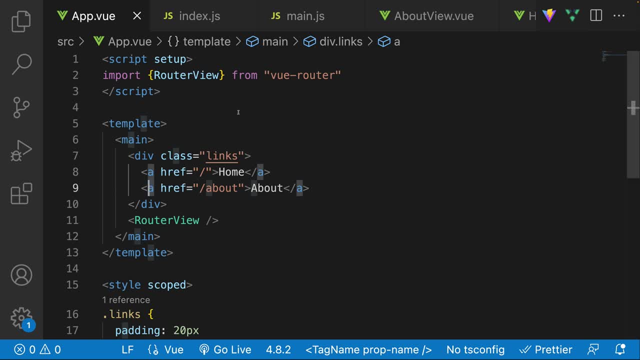 you might be thinking: okay, what's the big deal here? well, the big deal is that our state and other components, other parent components, is going to be refreshed. so, for example, over here, let's go to our app dot view, and I'm just going to go ahead and just add a piece of state, a piece of temporary state. so 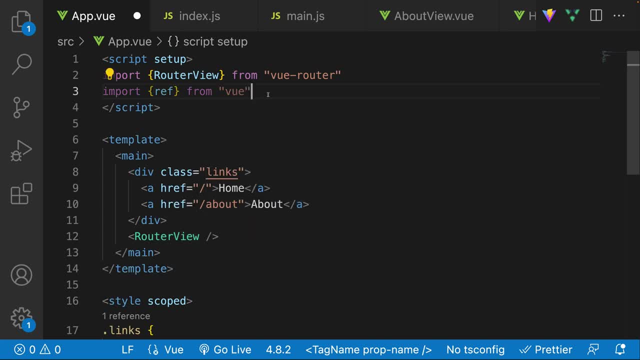 I'm going to import ref from view and let's just add a very simple counter. so we're going to say const counter is equal to, and we're going to initially set this to zero. and let's have a button right over here, click and this is very 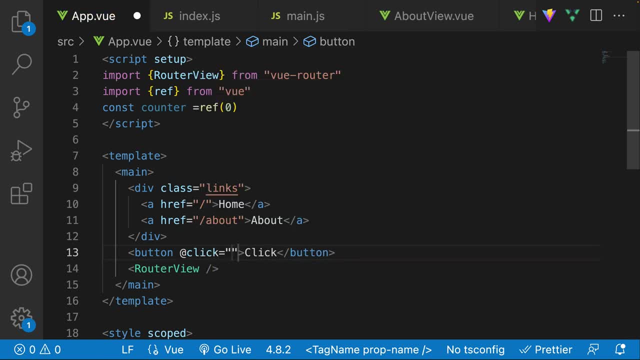 simply just going to add to the counter, so it's just going to say counter plus plus, like so, so and, of course, what we're going to also need to do just to actually see the state. let's add an h1 right over here and h1 tech and let's just say counter, like so. 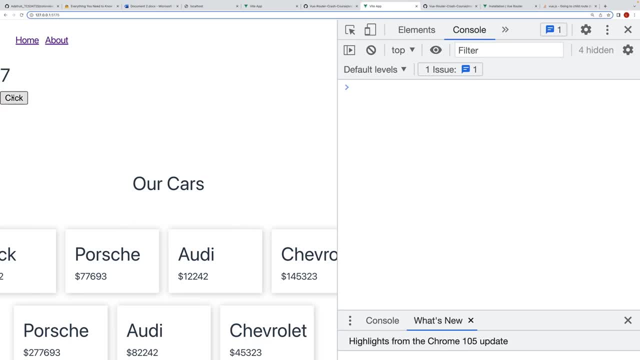 alright, so let's just take a look at that. and if I were to click on this- as you can see, the counter is indeed updating now because our hrefs are refreshing the page- what ends up happening is, when I click on the about, you can see here that now our counter is going back to the default, so regardless. 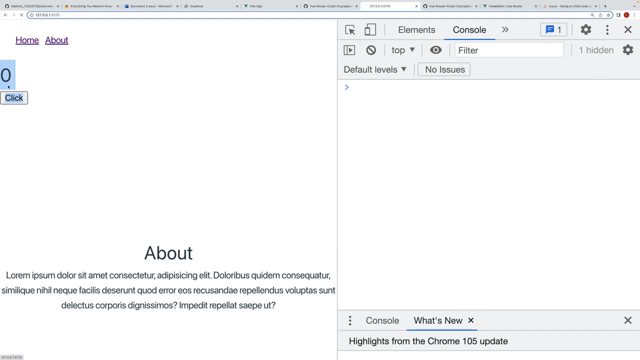 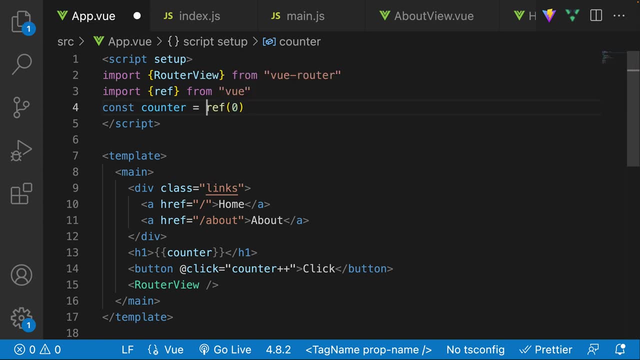 of what it was before, even though it's always there. our application is refreshing the page, and so it's going to go back to the default, which is zero. obviously, this is not what we want. we don't want to have this refresh effect. for one, it doesn't really look all too great, and, of course, number two is it. 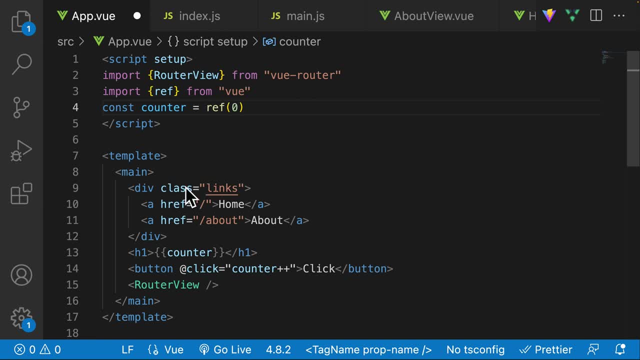 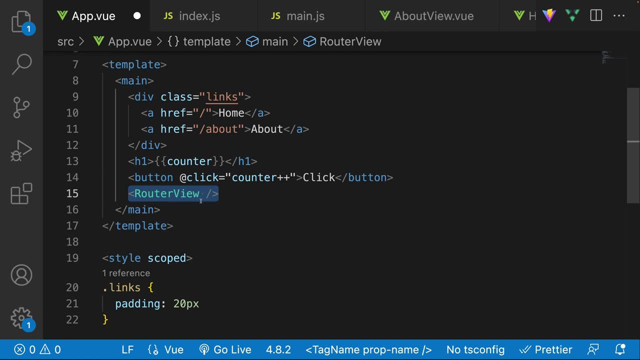 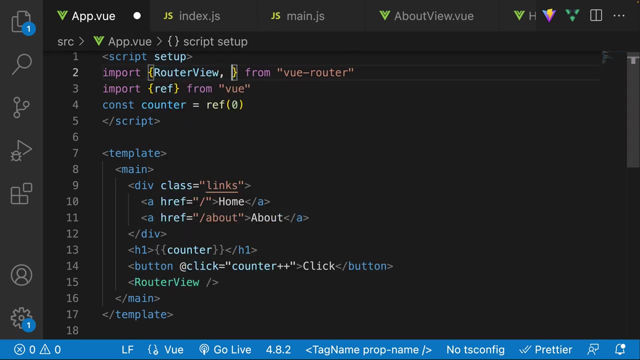 kind of messes up all of our state. so instead, what we wanted to do is to just very simply change the path and just let the router view component figure out what component to render. so we don't want to have that refresh now. when we're going to do that, we're not going to use anchor tags. instead, what we're going to 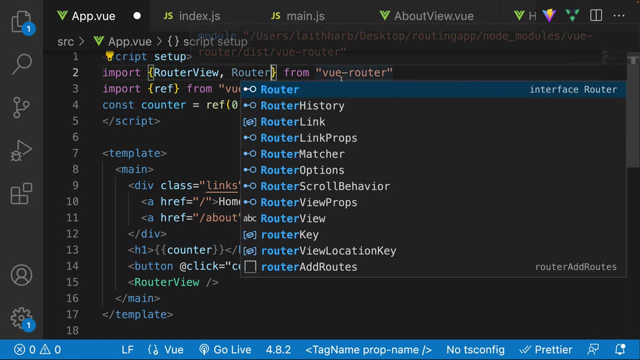 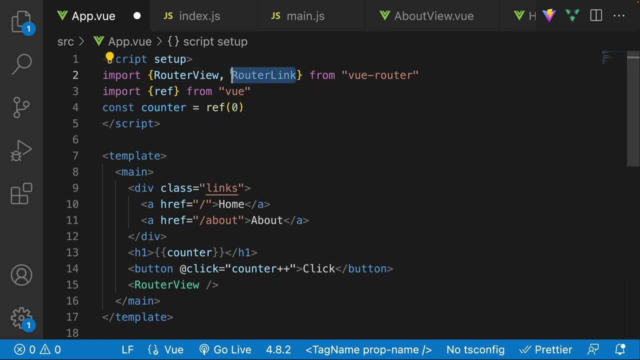 use are another component from the view router library and this is going to be called, well, router link. so, over here, we're going to utilize this instead of hrefs, we're going to go ahead and remove that, and we're going to say, instead of the anchor tags, we're going to remove them, we're going to use router link now. 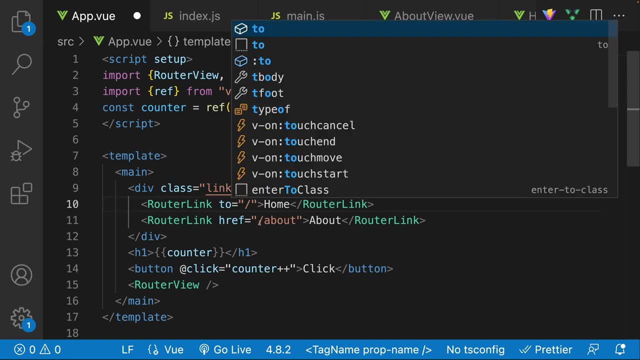 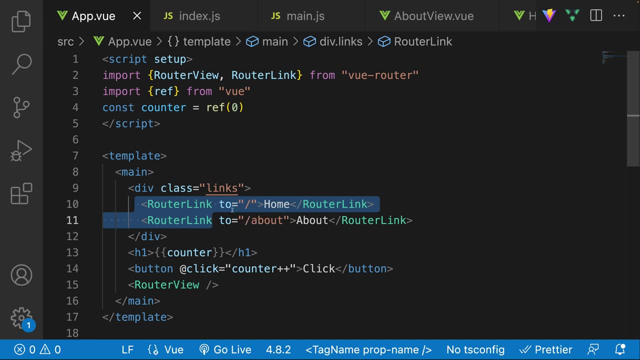 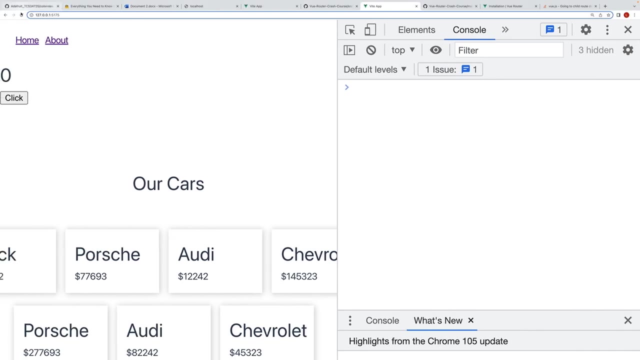 instead of href, what they're going to utilize is a prop called to, and at that point, that's pretty much it. So what this is going to do is change the path of our application, but without actually refreshing our app, so this state should actually persist. so if 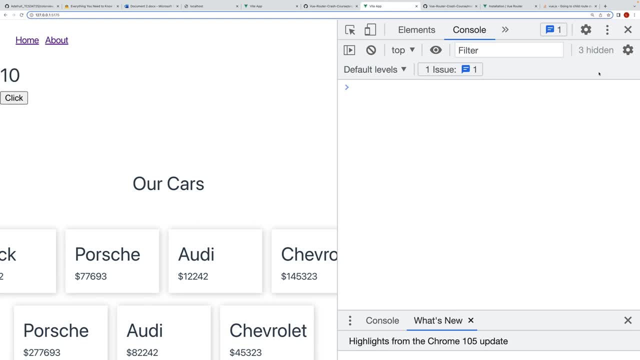 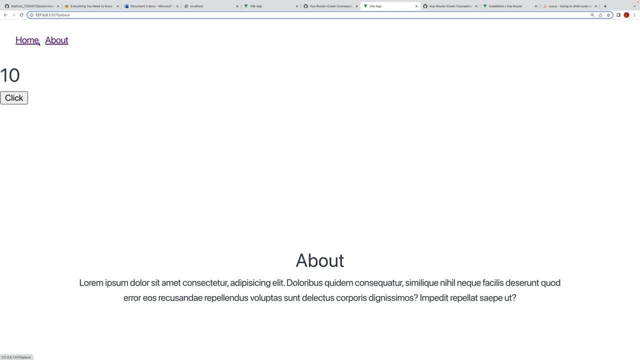 I were to, let's say, add a few things over here, you can even click, just get rid of that for now. and if I were to click on about, you can see here that our state is indeed persisting and you can see that the flow is significantly. 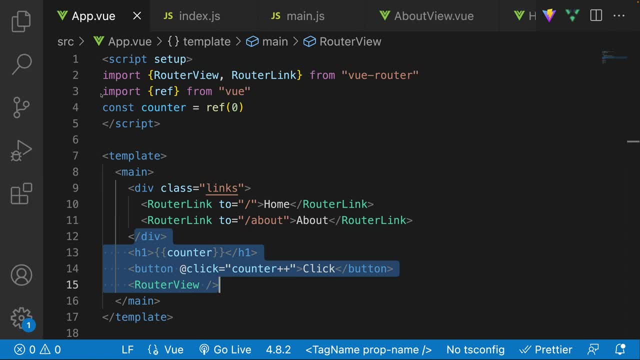 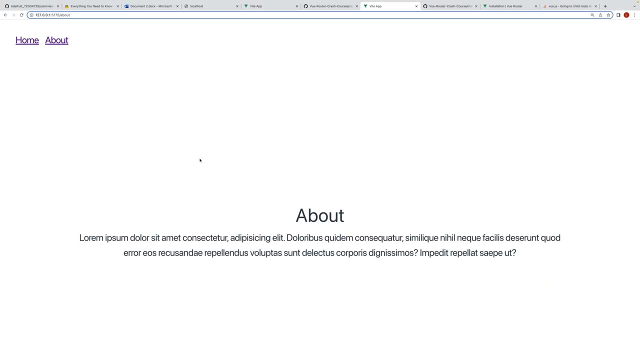 smoother, so it's just a lot nicer. so this is what we're gonna be utilizing to navigate across applications. now let's just quickly just remove this. this is just for demonstration purposes, so let's just go ahead and remove that. okay, looking good, all right. so this is pretty much what we have this far. let's do one. 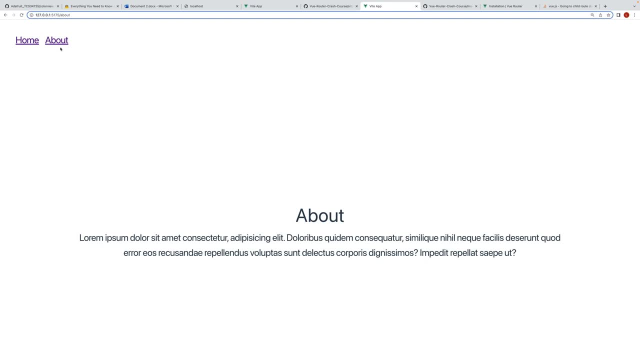 more modification to our navbar. what I want to do is I want to have, you know, different styling depending on the page that we're on. so if we're on the slash about page, maybe I want this to be a little bit bolded, maybe a different color, just so we know how that page looks like. 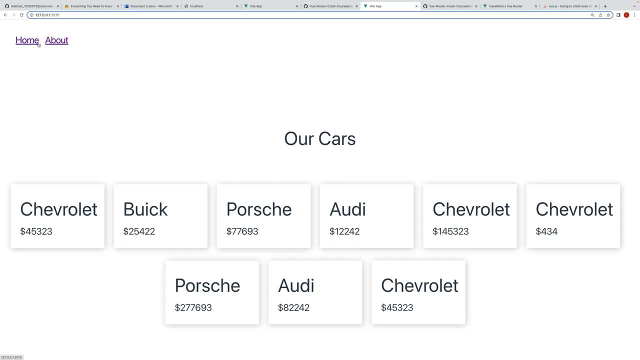 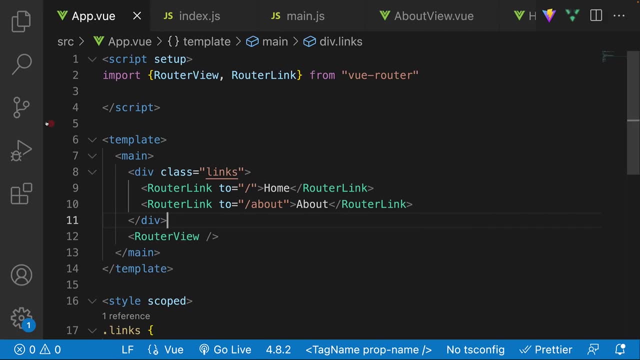 that okay? yes, we are indeed on the slash about page. if we change to the slash home, then i want this one to be bolded and maybe a different color, and then this one back to normal. and it's actually really really easy to do that with the router link component. all we have to do is add the active. 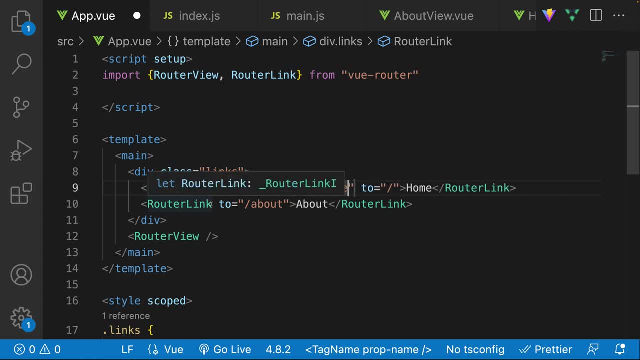 class prop. we're going to give it a class of active. so what this is going to do is okay. if this right over here, if we're on the slash path, the active class is going to apply this class right over here and it's going to apply it to this anchor tag. so, at the end of the day, this is still. 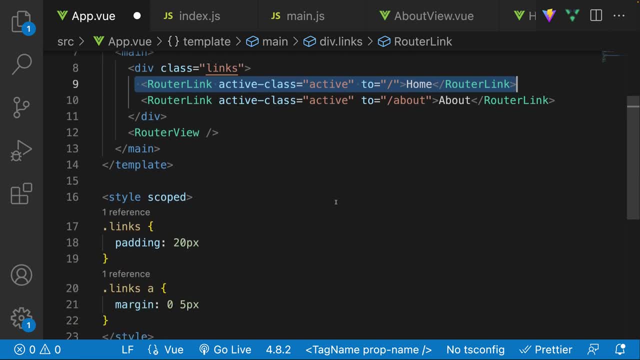 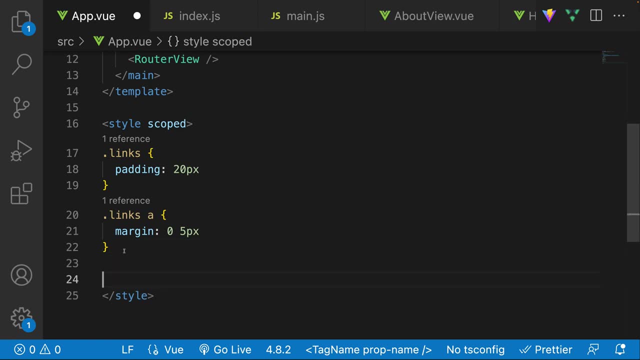 going to be an anchor tag, but this functionality is going to be a little bit different and that is not going to render or is not going to refresh our app. so over here, what we can actually do is just very simply just say dot active and we can just say maybe font. 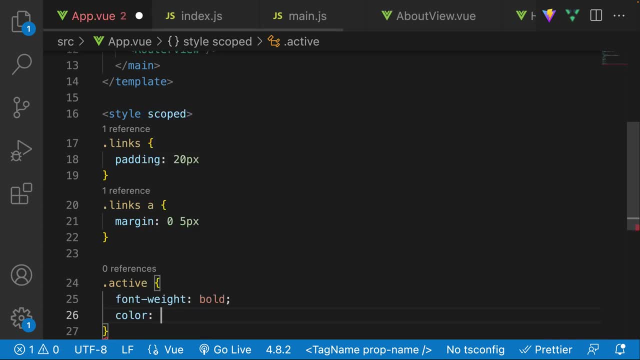 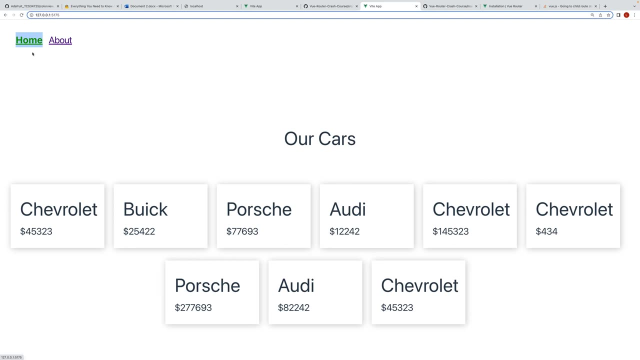 weight bold and maybe we'll just change the color to the green or something, just so we can really see it. so now you can see we're on the home page it's going to apply the active class on to this router link. but when we're on the about you can see here that it applies it to this router. 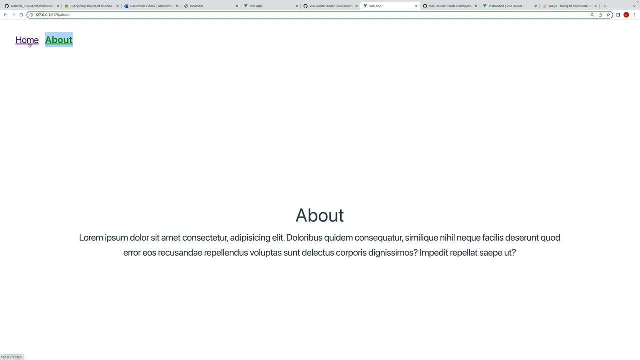 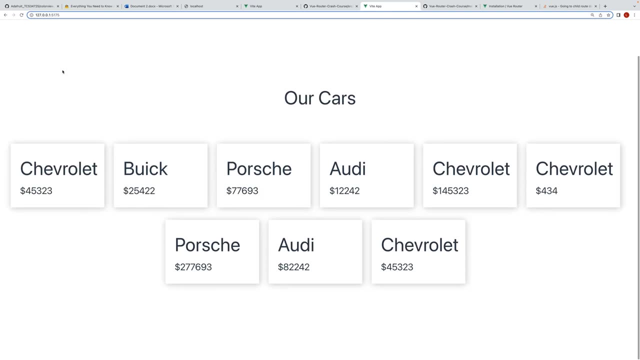 link so you can see we got this really cool and nice effect okay. so this is pretty awesome. i'm really enjoying this. but let's say now what we want to do is we want the to give the user the associated chances to render our app in order and cheer us in now with our ability to render police. 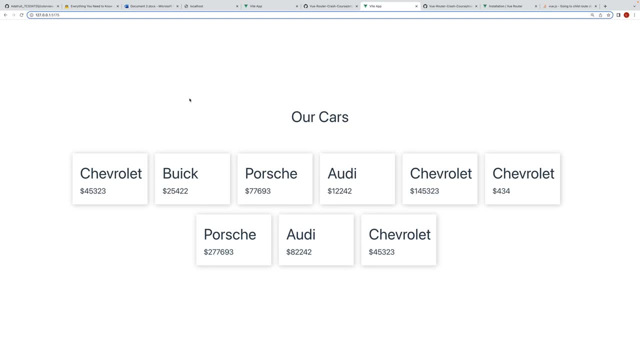 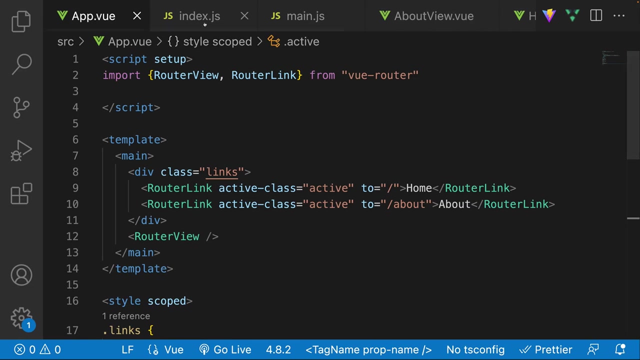 ability to click on a particular card, and then what i want them to do is i want to redirect them into a page that gives them more information about that car, because right now, within the cards, all they can see is the, the car itself, the make of the car, as well as the price. however, we have way. 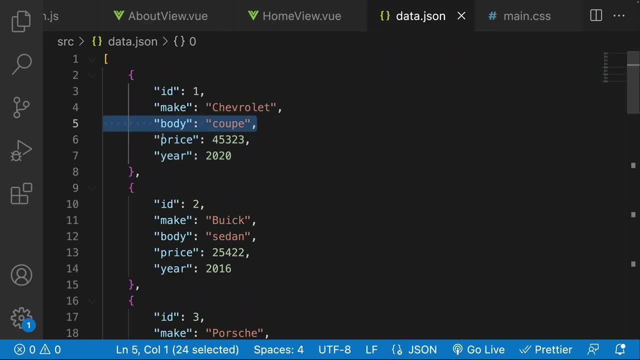 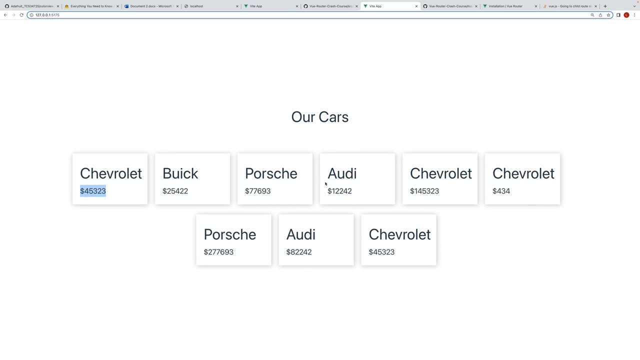 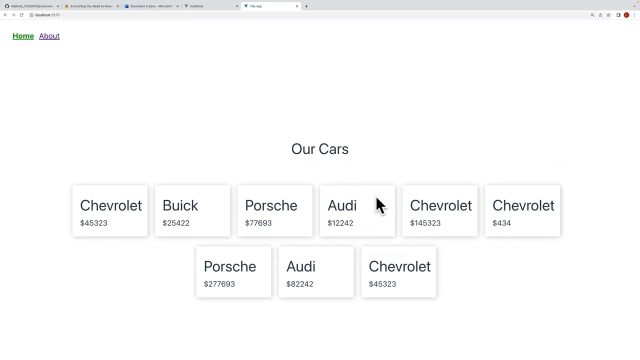 more information inside of our json file. we also have the body of the car, we also have the year of the car. we also want to just show all of this different information within that specific page. so let's actually talk about how we can do that. and this is actually a little bit trickier because 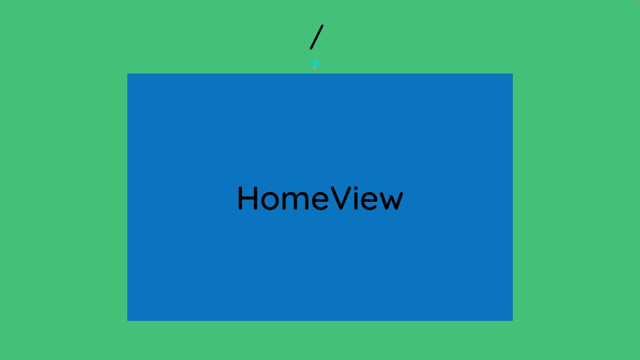 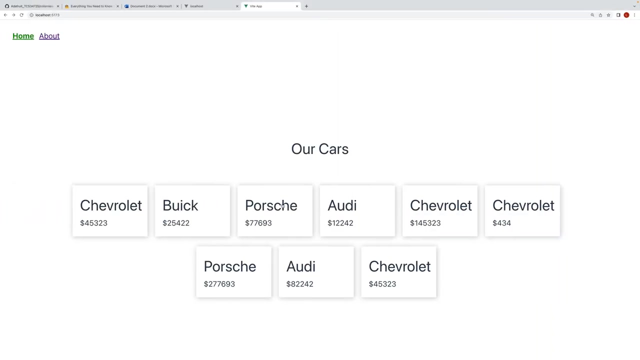 currently this is our outline. when we go to the root route, we have this home view component. when we go to slash about, we have the about view component. but what happens when we go to the audi page? are we going to have an audi view component that's going to show all? 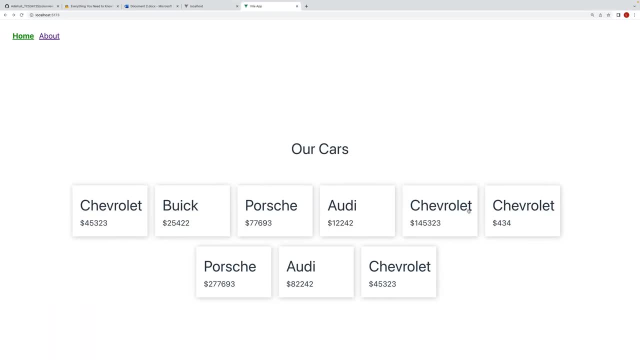 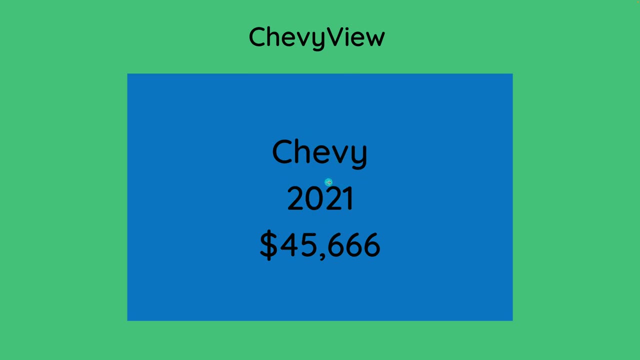 the information for the audi. and what if we go to the chevy page and are we going to have a chevy view component where we're going to have all of the different content for that chevy? so what i'm trying to say is, are we going to have a component for every single card in our application? 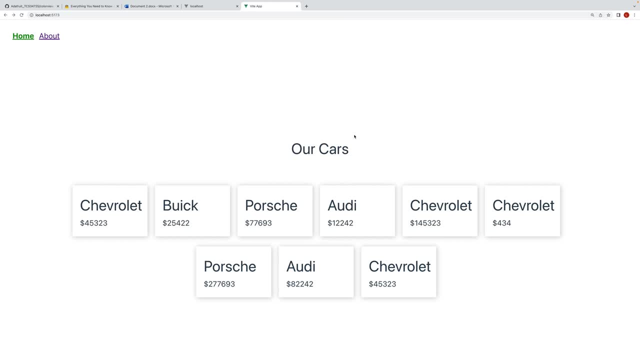 and obviously no, that's not the case, because that will be way too many components. it's just going to be a lot of repetitive code. plus, we're not going to know how many cards we're going to have inside of our application. this could be coming from some sort of 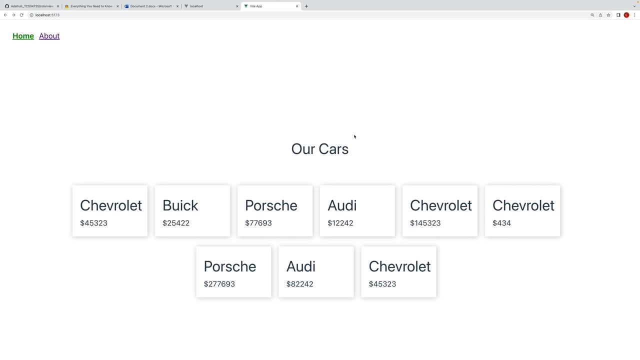 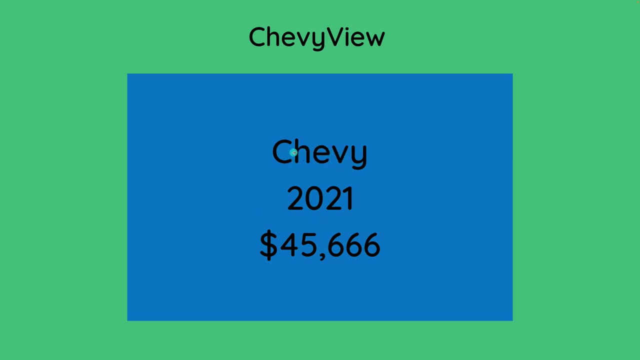 external api and that data could be variable. we could add data to it, we can delete data, we do not know. so instead we have to think of another way. well, let's just take a look at these two right over here. so over here, the overall html structure of both these components, the audi, as well as the. 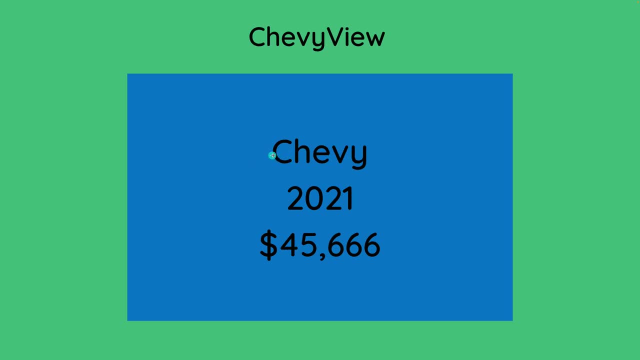 chevy is exactly the same. they both have an h1 that shows this make of the car. then, let's say, these are paragraph tags that show the year of the car as well as the price. so overall, the html structure is exactly the same. all that is different is the data that is within that html structure, so i think it's actually better to create. 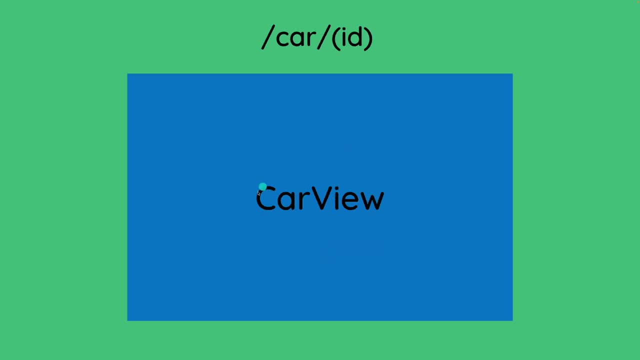 one component instead and we're going to call this component the car view component and it's going to have the path of slash car and then slash that particular car's id. so this right over here is going to be a dynamic path so we can have slash car, slash one, and we're still going to render this component. we're going to have 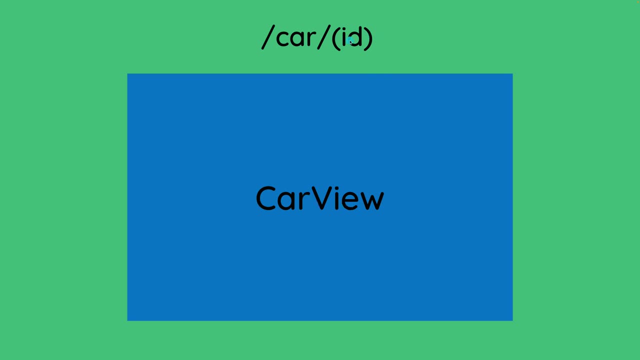 slash car slash two. we're still going to render this component, so it doesn't have to be an exact path. it is going to be dynamic. now, why is this important? well, now the car view can actually access that id over here and once it accesses the id, it can figure out what car data it can go ahead. 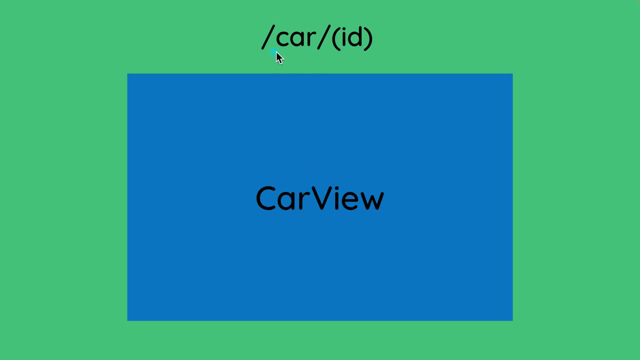 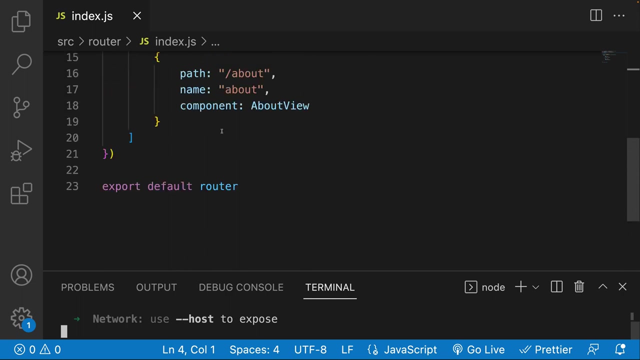 and render. so let's go ahead and actually define this path right over here, inside of our application. so what we're going to need to do here is we're going to need to well define another rule now over here. we're going to define the path and this is where it's just going to be. 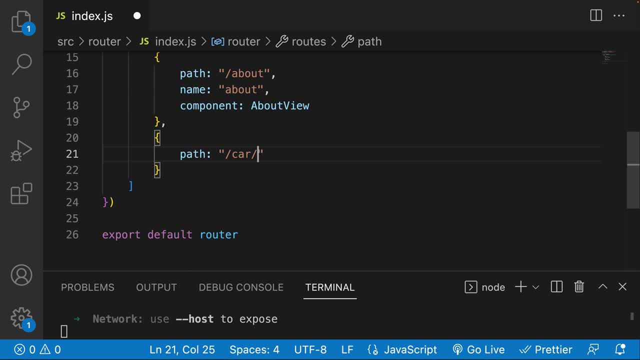 a little bit different. it's going to be slash car and then slash id. but now what we want to do is we want to define this id as being dynamic. so to define something as dynamic, all we have to do is add a colon. so now we say colon id and now this is going to be dynamic. so now, if we go to 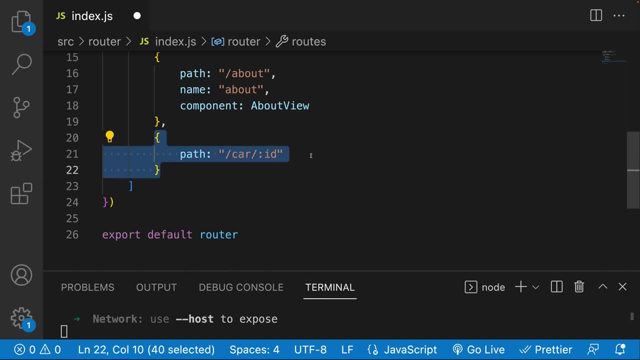 car, slash anything, it is going to match with this rule. so let's go also and just say name of, we'll just say car. and lastly, we're going to say component of, we're going to say car view, like so. so now all it is that we need to do is actually create this car view component, and let me just 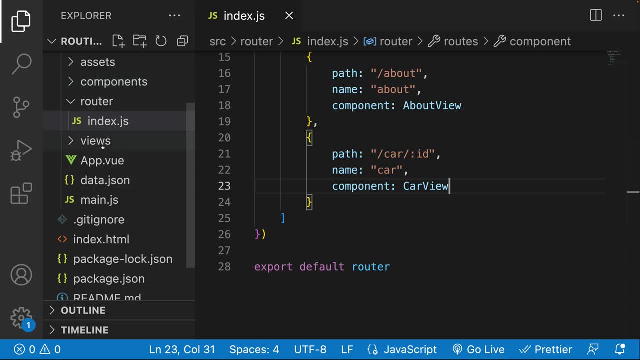 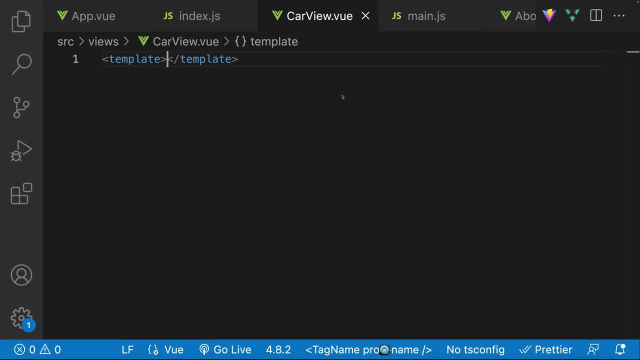 dot view, like so. so let's go ahead and create the template. so i'm going to have a template here. let's also give this a div with a class of container and then over here let's just say h1 and we're going to say the car. now, before we go ahead and actually uh work with this, let's do a. 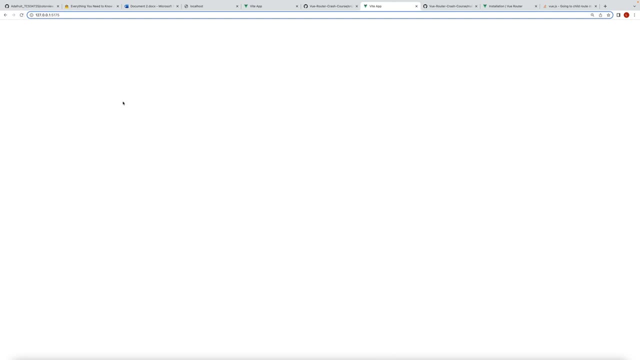 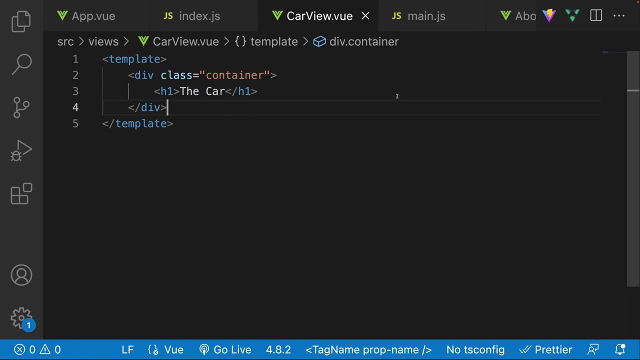 little quick test here, so i'm going to do a quick little refresh, and it seems like something is indeed broken. let's just quickly see why that is. so it says here: car view is not defined. not a problem, let's go over to our indexjs file. 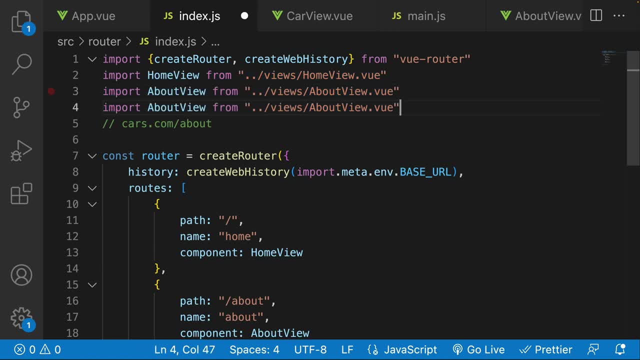 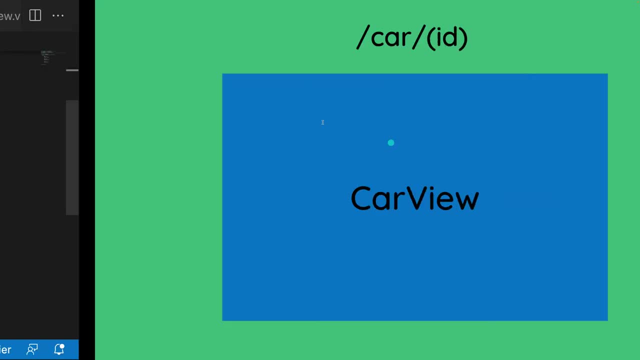 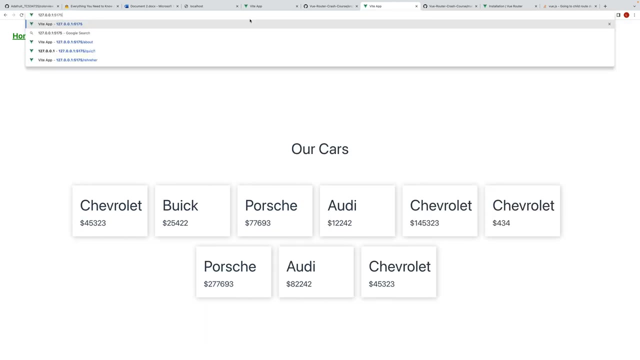 of course we're going to need to import that car view, so we're going to say car view and car view, okay. so nonetheless, now this should theoretically work. so if i were to go to now slash car, slash, whatever, literally anything, i should be able to see this component. 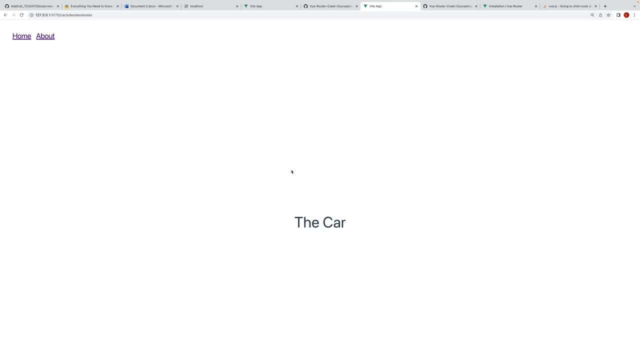 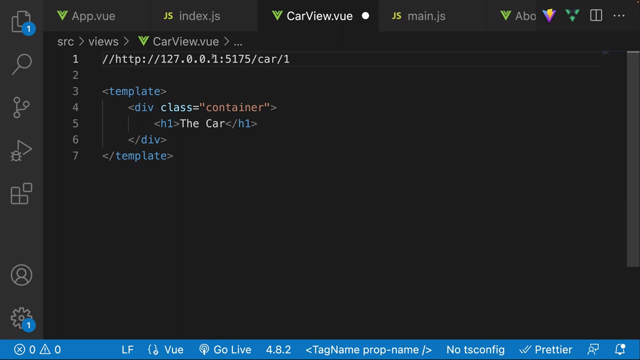 render. okay, so this is looking good. now, what i eventually, of course, want to do is i want to grab this, uh, query right over here this, this kind of path variable. so, again, it could look something like this: so we're going to have something that looks like this. so we're going to. 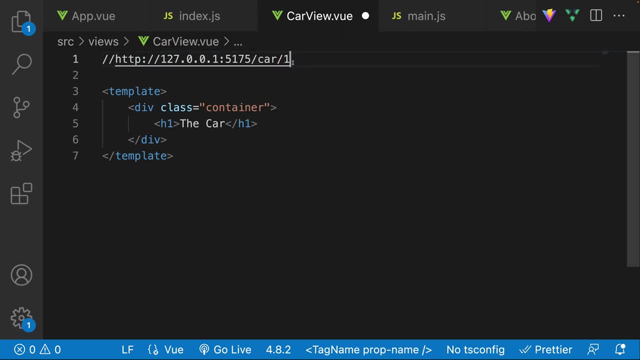 have slash car and then slash one and what we want to do is we want to grab this right over here, this one right over here, so then we can actually find the car with that id. so to do that, let's create a script. so script and we're going to say setup and we're going to import something. 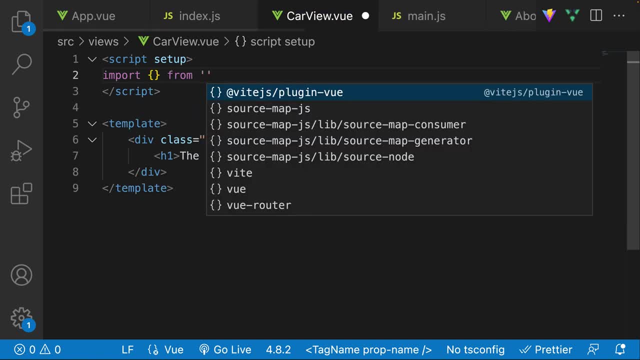 from view router. so this is something that we haven't used before. i'm going to get it from view router and this is going to be a composable, and this composable is going to be called use route, so use route. so over here you can see we have two different composables: use router and 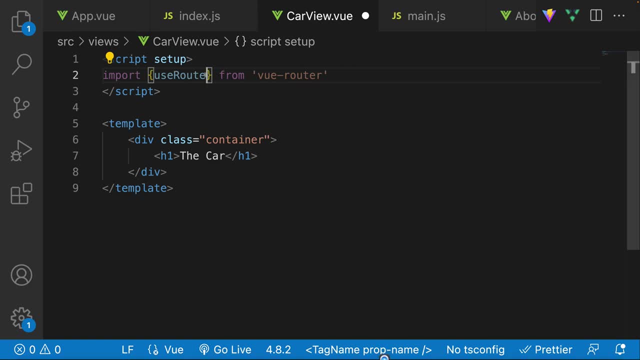 use route. make sure that you're utilizing use route. now what the use route composable allows us to do is just get a bunch of different information that we need about our current route, about our current path. so over here we can just say const route is equal to use route, and we can 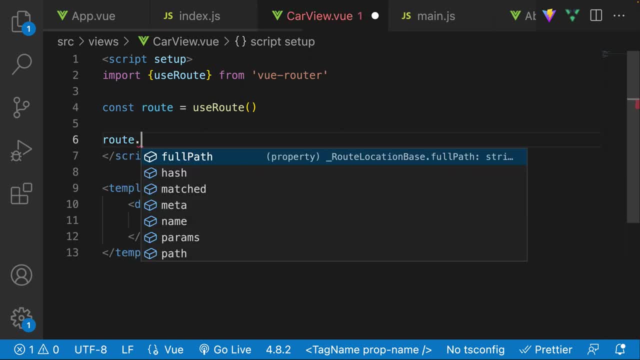 go ahead and invoke it, and now, with this route, i can just say route dot, dot. and you can see here that the there's just a bunch of different things, a bunch of different information that i can get. i can get the name, i can get the path, i can get the params, i can get whatever it is that i want. 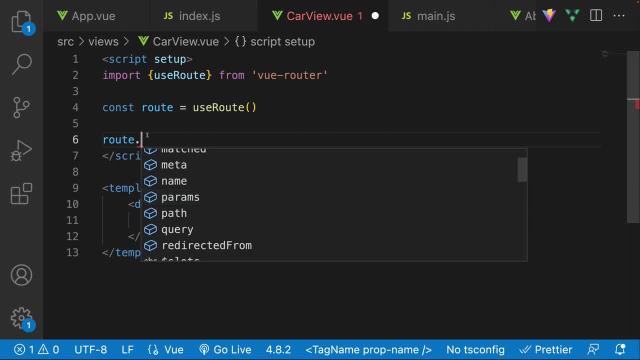 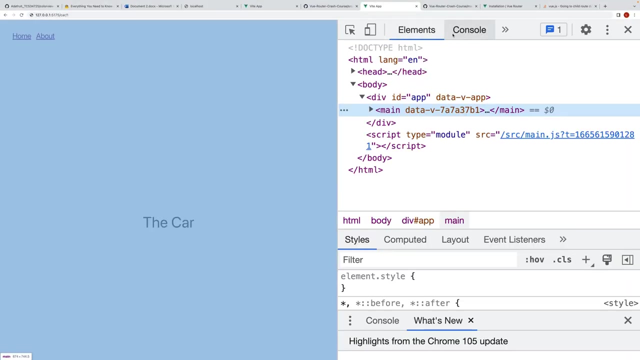 now, specifically, i actually want the params. so let me just go ahead and quickly consolelog the params here, just so we can see what we have here. so i'm going to say route dot params. go ahead and log that and let's just see what we have. so i'm going to say inspect and you can see that this is going. 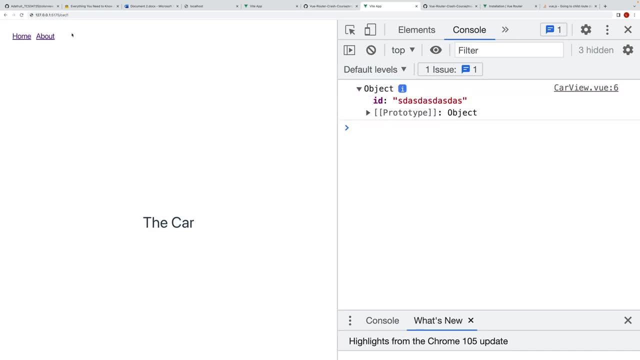 to return an object and if i were to refresh here, let me just quickly refresh- you can see that it gives me an object and you can see that this object has an id of one, which is exactly what we have right over here inside of our param. so let's. 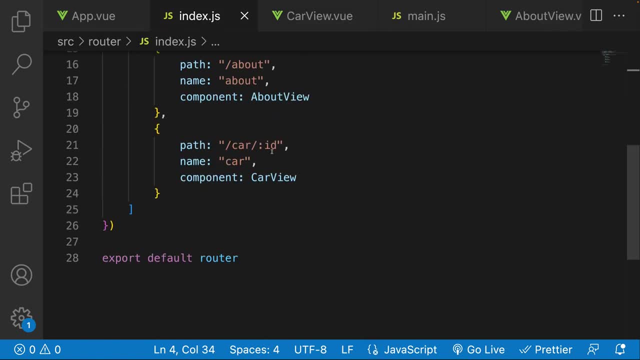 remember in our path what we did in our eroding rules. we said that this right here is going to have the variable name of id and then whatever value it's going to be, it's going to be attached to this. so if i change this, for example, to banana, then it should be banana of one, but of course that. 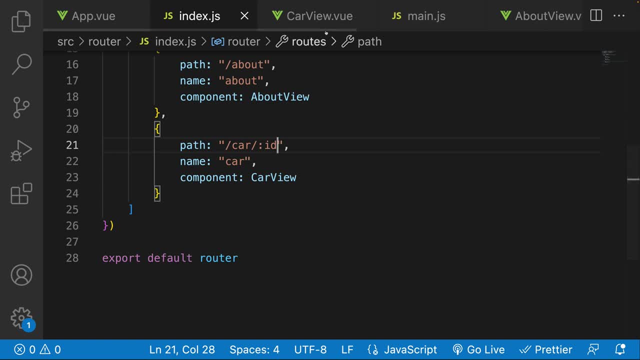 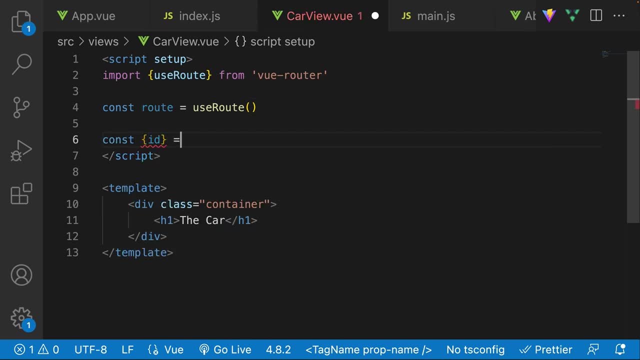 doesn't really make much sense. so let's just say id like so: so now what we can do is we can actually extract this id and we can actually extract this id, and we can actually extract this id and we can utilize it. so let's just say const id. we can just destructure it out dot params. so now we can grab. 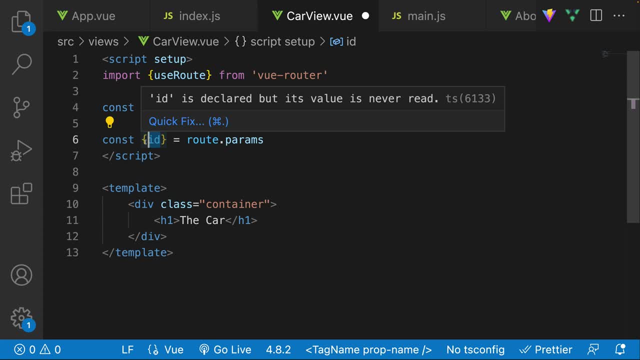 this id and now, once we have this id, we can actually go ahead and utilize this id to figure out what car we want to render. so let's actually go ahead and just create a piece of state here. so we're going to say import and we're going to import from view, we're going to import ref. 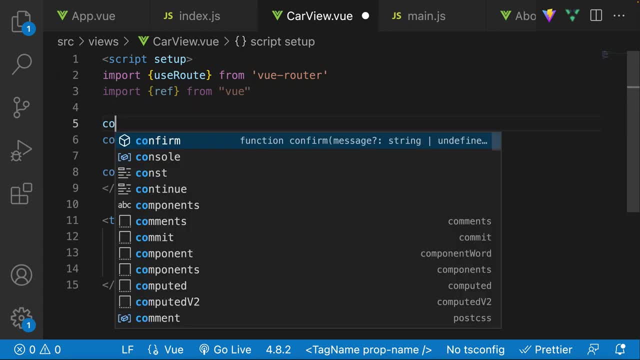 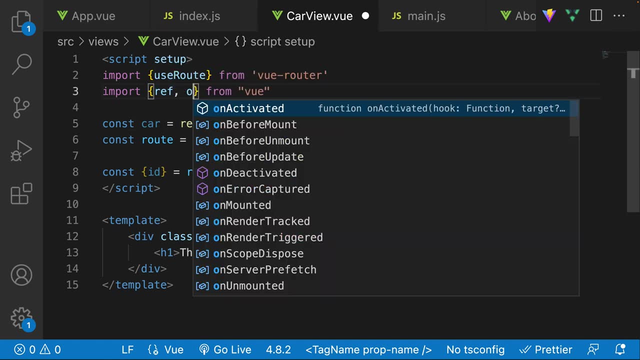 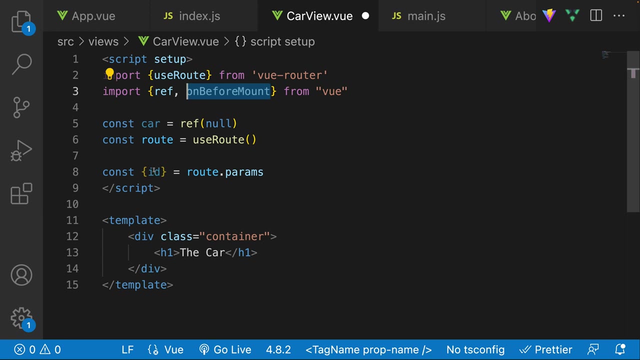 and over here let's just create another piece of state called the car and initially we're going to set it to null and we're going to import something. we're going to import a lifecycle hook on before mount. so before this mounts, let's go ahead and just 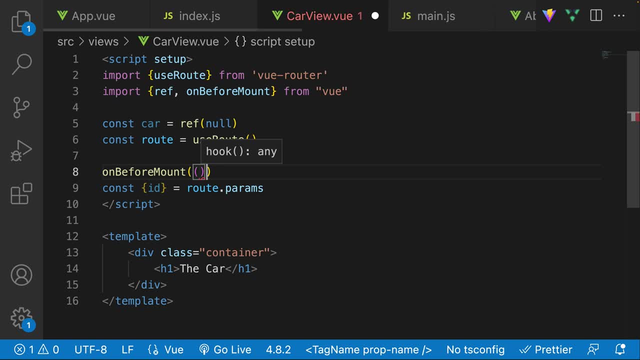 render this. so we're going to go ahead and call this callback over here and, before this mounts, what we want to do is we want to find that specific car. so we're going to say const and let's just say car data, and we're going to say that that is going to be equal to. so let's go ahead and actually import. 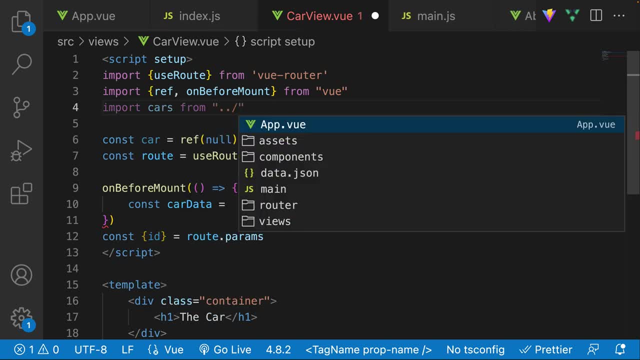 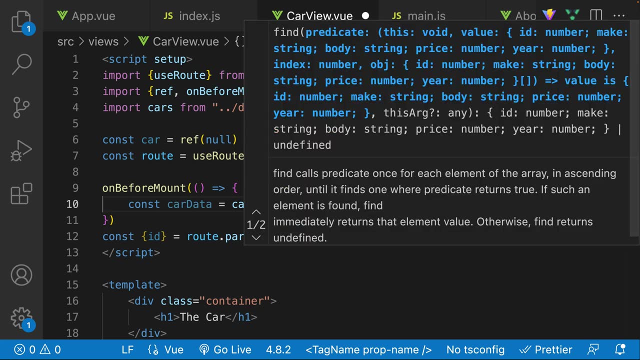 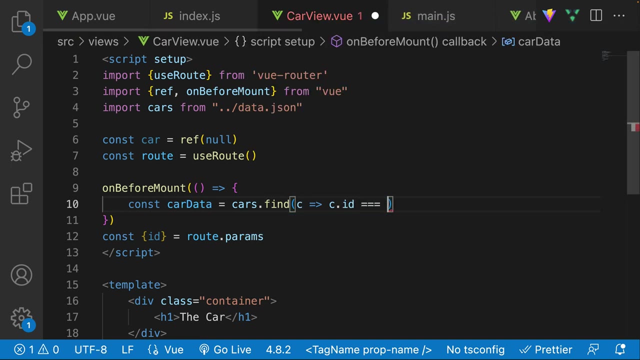 all those cars. so it's going to say cars from the json file. so i'm going to say cars, dot find. and then we're going to say c just stand for car. i'm going to say c, dot, id is equal to, and then we're going to say, uh, what are we going to say here? the id of this param. so let's. 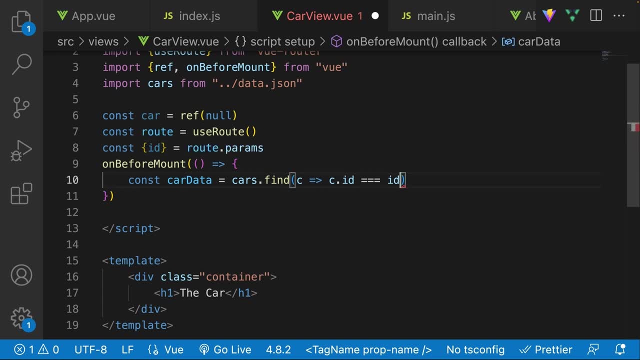 just go over here. let's put this right above we're going to say id, so what we're going to do is we're going to try to find the car that has the id that is the same as the one that we got from our path parameters. now, one thing that i want to note is that if i were to go to the data dot, 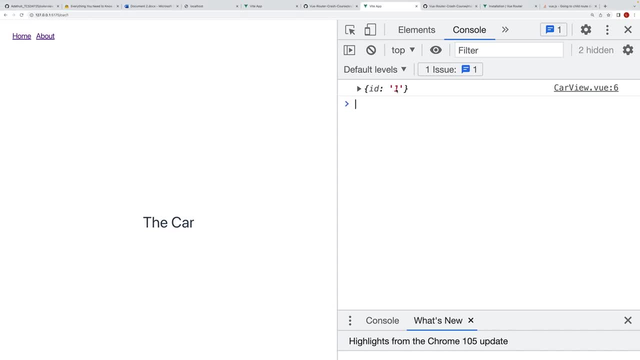 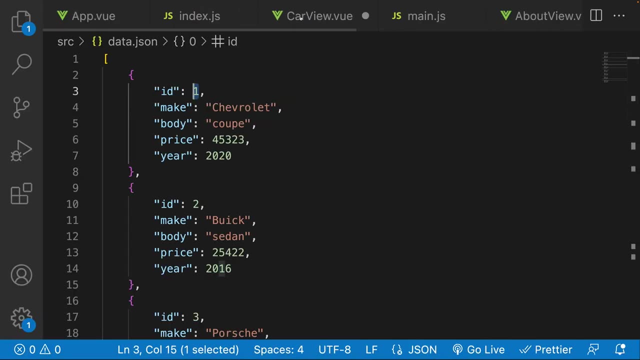 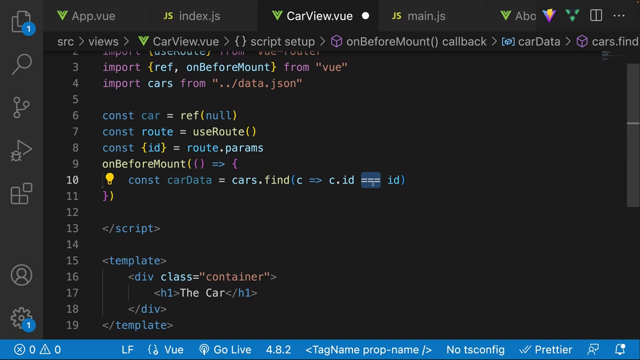 json, you can see that the id is actually a number, whereas over here our id is a string. so we actually have to keep that in mind when we do this kind of comparison. so what we can either do is we can remove the uh, triple, uh equal sign or and just say double equal sign. or what we can do is we can: 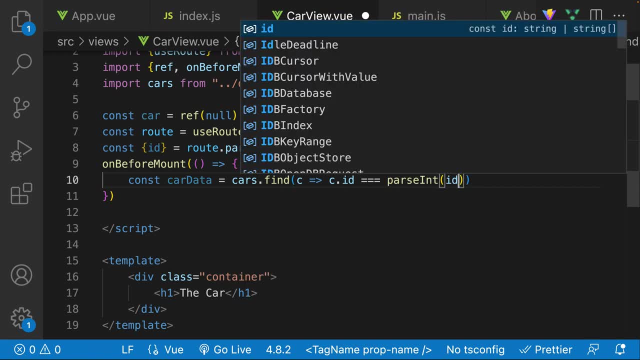 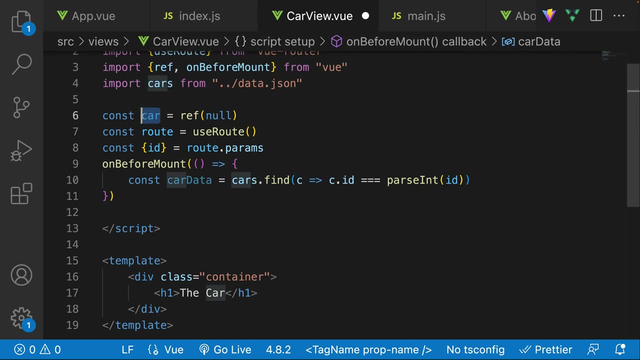 actually parse into this. we can say parse int and we can turn it from a string to an integer, and once we find that, what we can very simply do is change our piece of state. so actually, instead of just creating a new variable, what we can do here is we can just say: car dot value is equal to this. 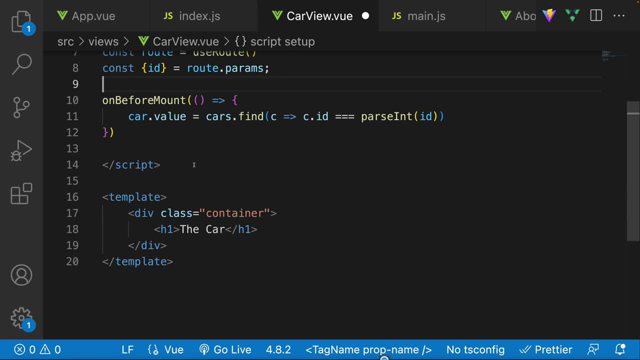 all right, so that will get us the car information and now, once we actually have the car, we can go ahead and actually render it within our app. so i can just say something like the make, and that's going to be car dot make, and i can say paragraph. 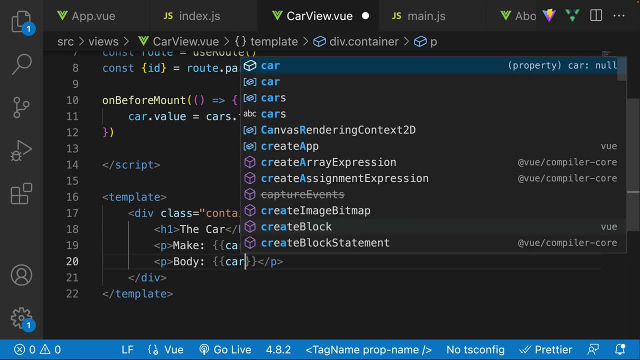 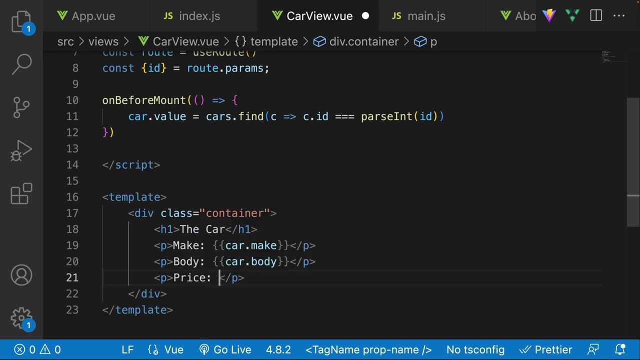 i can say the body, and that is going to be the car dot body, and we can say the price, and then car dot price, like so, and then over here we can say the year, and we can say car dot year and, uh, that's pretty much it. i think that's pretty good for me. 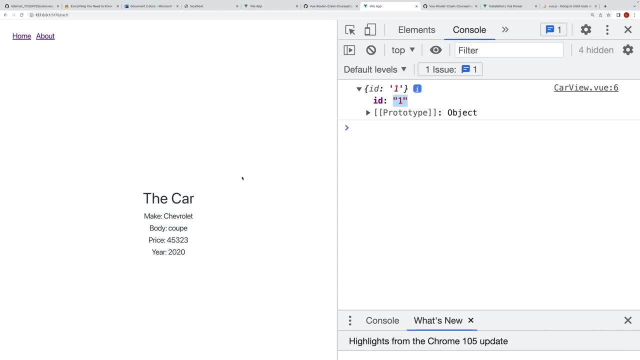 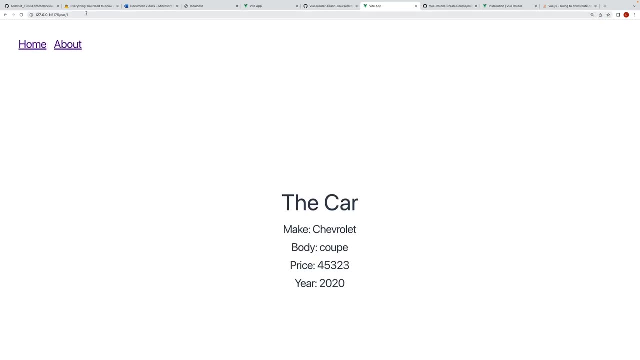 i'm going to change that to a capital. and now if i were to go here, you can see i am indeed actually getting all the information that i want. and if i were to go to slash two right now, you can see, now we're getting information about the buick and you can see, here we're getting now the car dot year. 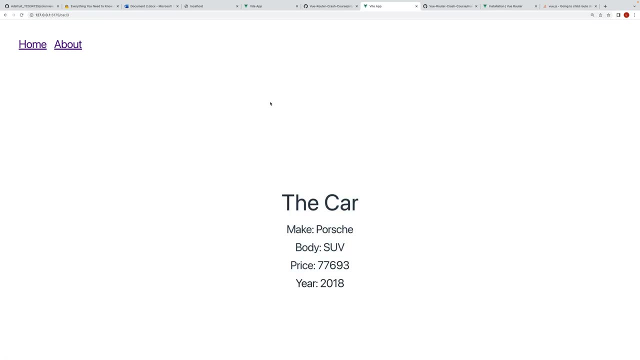 three, which is the porsche. so you can see here that if we're we have multiple different uh- kind of data that we want to render here, however, the html is the the same- we can utilize these dynamic paths. now, one thing i want to do is, of course, i want the ability to click on these cards. 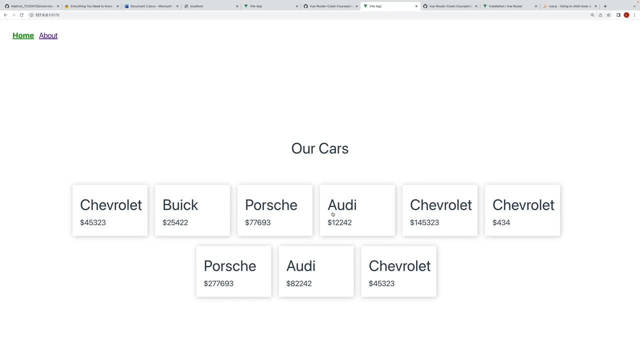 and then i want it to take me to the path that i wanted to. obviously that's what i want. no way the user is going to know that the audi has an id of four or something like that. you know, in a real application the id of this audi might be 1 million 647 you. you really never know. 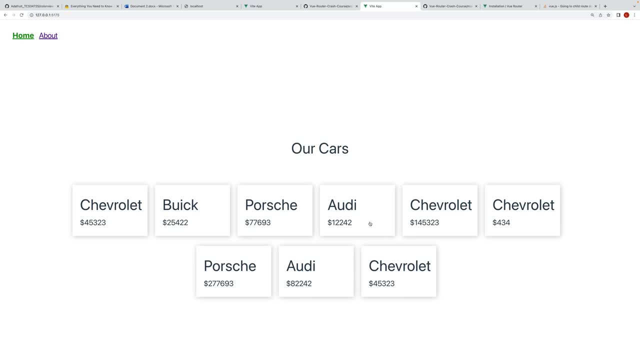 so you want the user to have the ability to click on this card and then it's going to move them to the correct path. now this might seem a little bit simple, but it's actually kind of a little bit tougher than you think, because you might think i can- okay, i can just change this card from being a 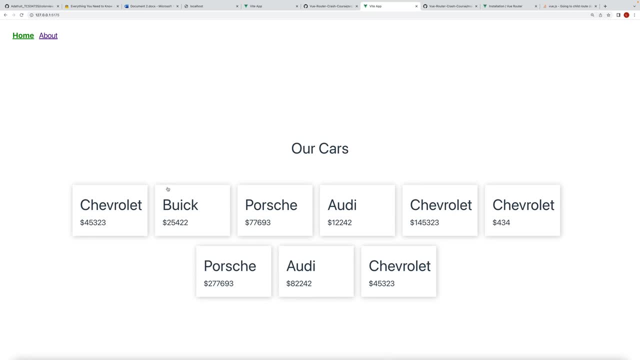 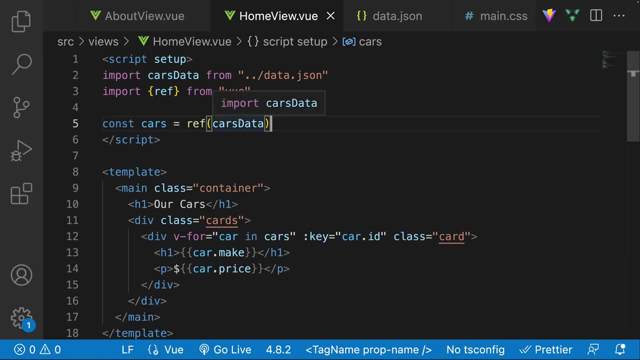 div to just being a router link, and that's what i'm going to do. so i'm going to go ahead, and i'm going to go ahead, and i'm going to go ahead and quickly do that. so let's go to our home view component, and what we're going to do is: 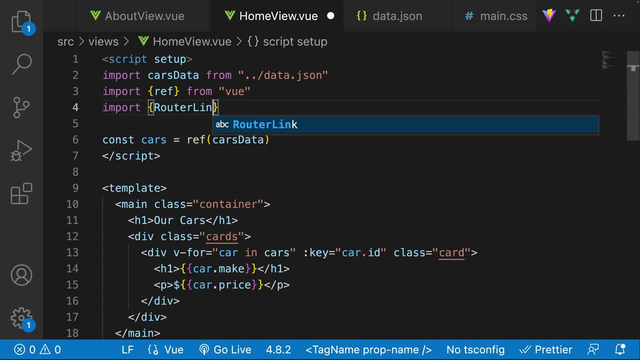 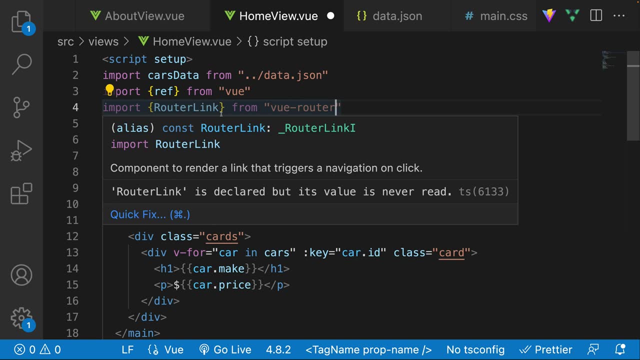 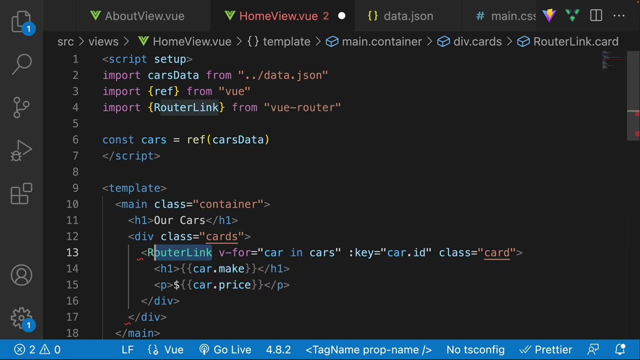 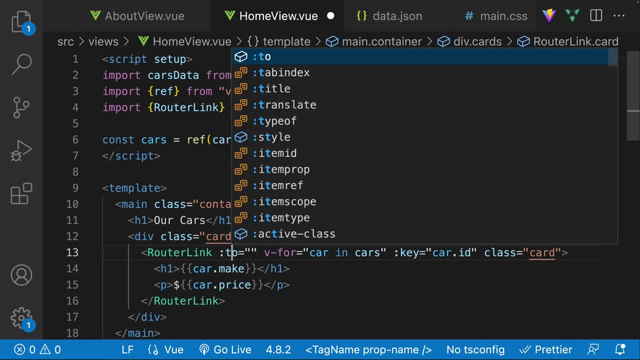 we're going to change this to a router link and then over here we're going to specify a two and let's just make a two, and let's just make a two and let's just make this dynamic. so we're going to add the colon. this dynamic, so we're going to add the colon. 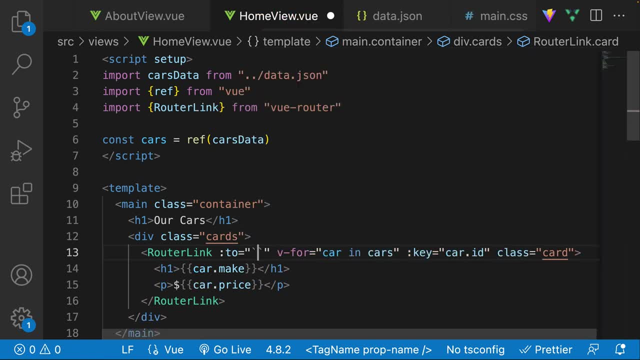 this dynamic. so we're going to add the colon here, we're going to bind it here, we're going to bind it here, we're going to bind it and let's add template literals, and and let's add template literals, and and let's add template literals, and we're going to say, hey, i want you to go. 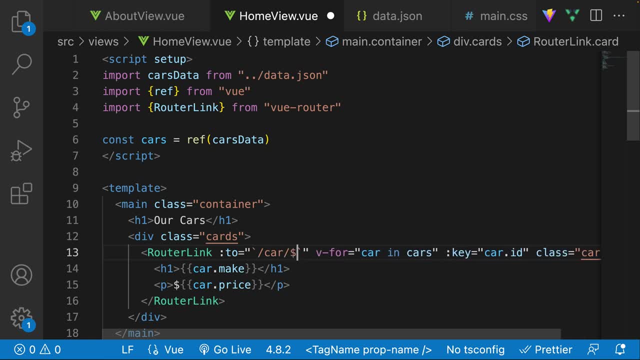 we're going to say, hey, i want you to go. we're going to say, hey, i want you to go to slash car, to slash car, to slash car, and then i want you to go to slash car, and then i want you to go to slash car. 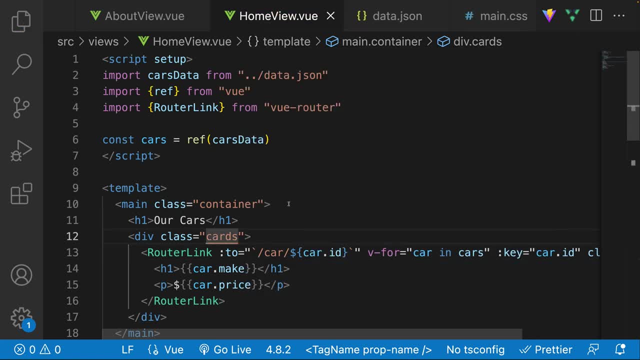 and then i want you to go to slash car and then whatever that car's id so dot, and then whatever that car's id so dot, and then whatever that car's id so dot, carid, carid, carid. and this would actually work in terms of: and this would actually work in terms of and this would actually work in terms of the routing it would 100, the routing it would 100, the routing it would 100 work. so you can see here if i were to work, so you can see here if i were to. 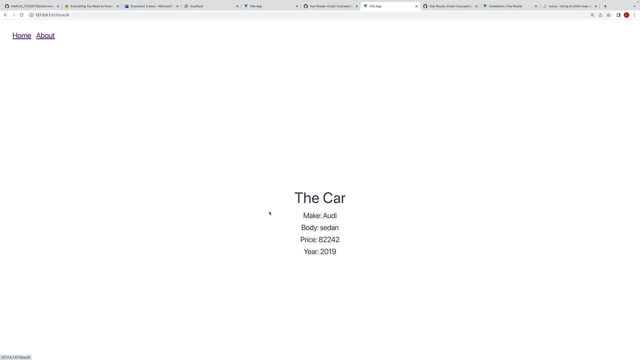 work. so you can see here, if i were to click here, it takes me to the porsche. i click here, it takes me to the porsche. i click here, it takes me to the porsche. i. styling that i don't like personally of styling that i don't like personally of. 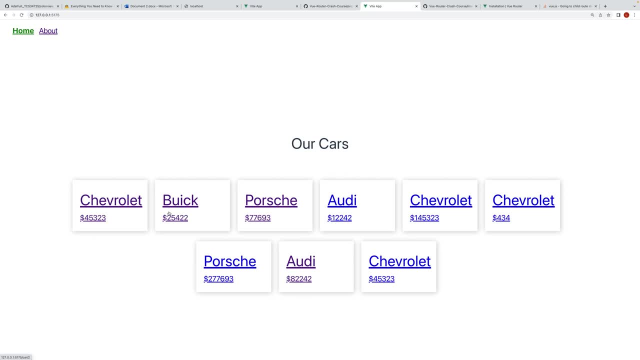 styling that i don't like personally. of course we can go ahead, and manually. course we can go ahead and manually. course we can go ahead and manually remove this styling. however the uh the remove this styling. however, the uh, the remove this styling. however the uh, the anchor tag will always be there and 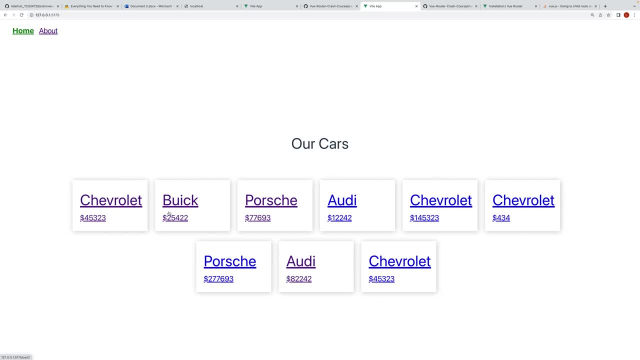 anchor tag will always be there, and anchor tag will always be there, and maybe i want it to be a div, maybe i want it to be a div, maybe i want it to be a div. well, in cases like these, this is where. well, in cases like these, this is where. 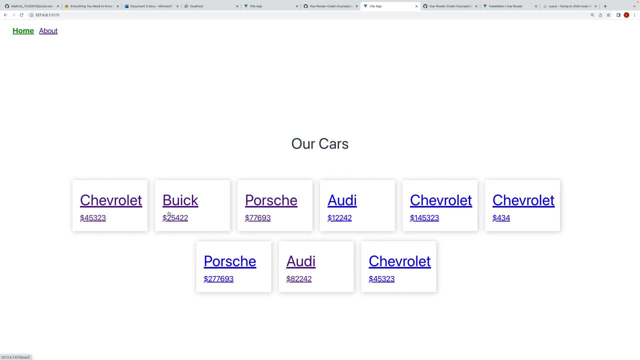 well, in cases like these, this is where it's actually better to programmatically. it's actually better to programmatically. it's actually better to programmatically, through javascript itself, change the path through javascript itself, change the path through javascript itself, change the path. so let's go over here. 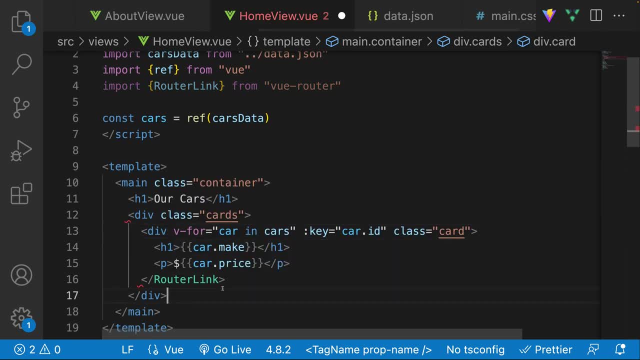 so let's go over here. so let's go over here, and what we're going to do is we're, and what we're going to do is we're, and what we're going to do is we're going to change this back to a div. going to change this back to a div. 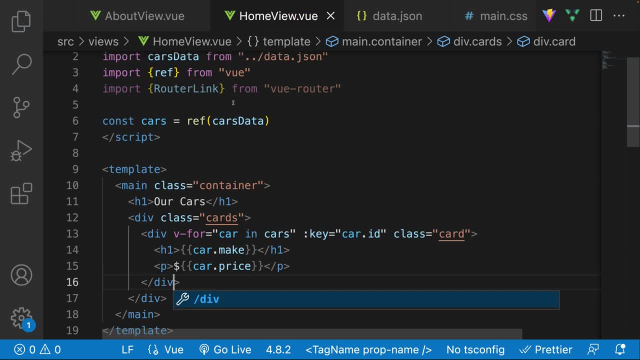 going to change this back to a div and we're going to just programmatically, and we're going to just programmatically and we're going to just programmatically change the path. so we're going to do change the path. so we're going to do change the path. so we're going to do this inside of the script itself. this inside of the script itself, this inside of the script itself. so to do this, we're going to need to. so to do this, we're going to need to. so to do this, we're going to need to import something else from view router. import something else from view router. 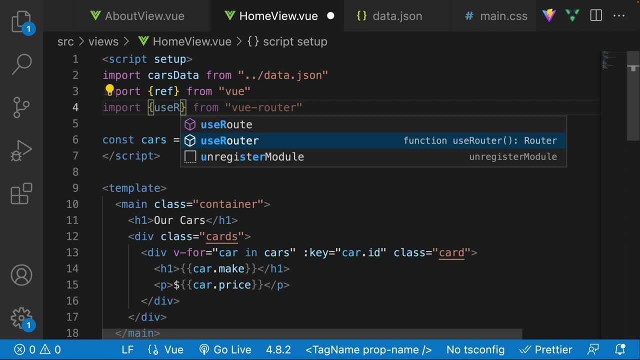 import something else from view router. it's another composable. and this time it's another composable. and this time it's another composable. and this time we're going to import the use. we're going to import the use. we're going to import the use router composable, not the use route. 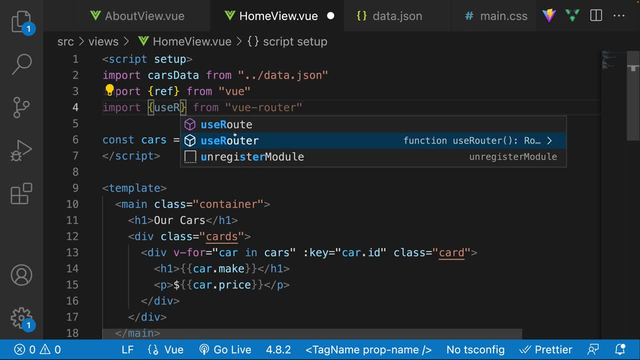 router composable, not the use route. router composable, not the use route composable. composable, composable: the use router, so just a quick little. the use router, so just a quick little. the use router. so just a quick little. definition about these two composables. definition about these two composables. 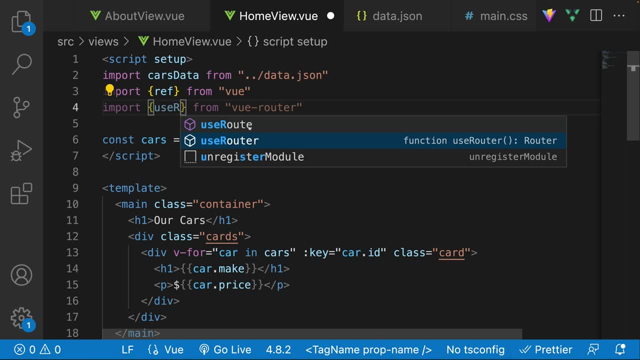 definition about these two composables: the use route composable is a composable. the use route composable is a composable. the use route composable is a composable that we use. that we use. that we use in order to get information about our, in order to get information about our. 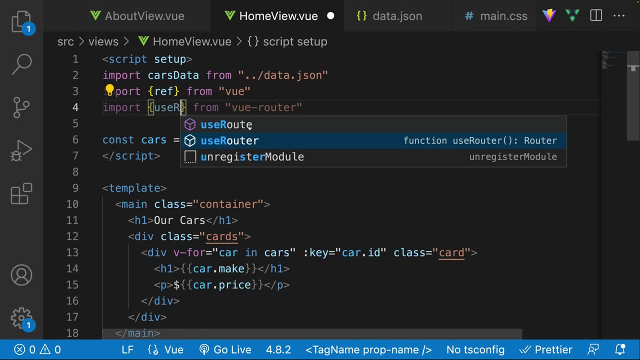 in order to get information about our path. so the query parameters, the path. so the query parameters, the path. so the query parameters, the parameters themselves, the path parameters themselves, the path parameters themselves, the path, whatever information that we want to get, whatever information that we want to get. 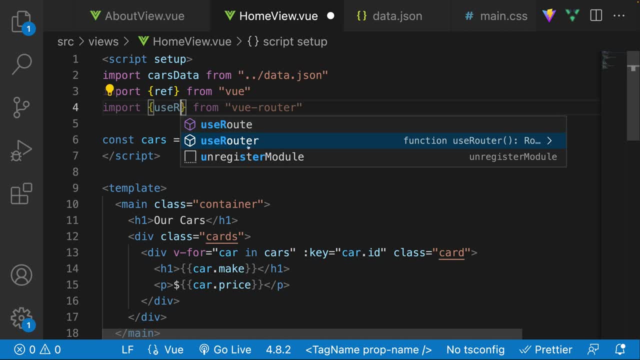 whatever information that we want to get, we're going to get it with the use. we're going to get it with the use. we're going to get it with the use route composable, however, if we want to route composable. however, if we want to route composable, however, if we want to do some functionality to our path, like 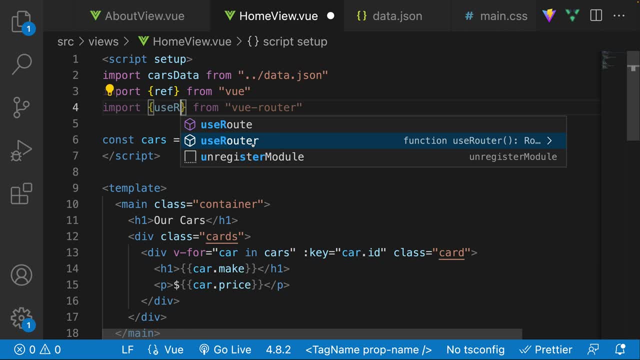 do some functionality to our path, like do some functionality to our path, like change it, or maybe go back to what we change it, or maybe go back to what we change it, or maybe go back to what we had or reset it had or reset it had or reset it. then we're going to use the use router. 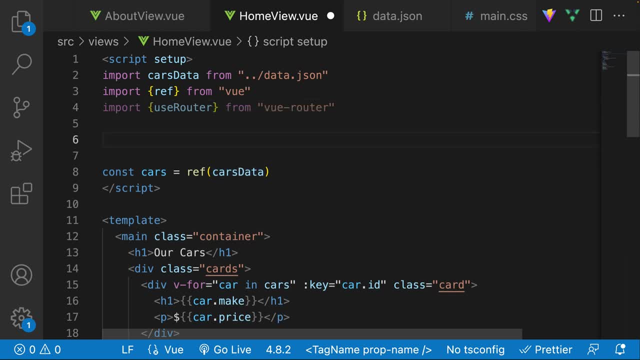 then we're going to use the use router, then we're going to use the use router, composable, so that's kind of the composable, so that's kind of the composable, so that's kind of the difference between difference, between difference between the two. so hopefully that makes sense. 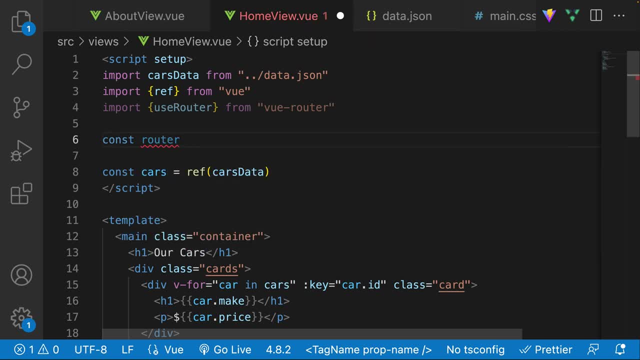 the two, so hopefully that makes sense. the two, so hopefully that makes sense. so, over here, very similarly, we're going so, over here, very similarly, we're going so, over here, very similarly, we're going to say to say: to say, const router is equal to const router is equal to. 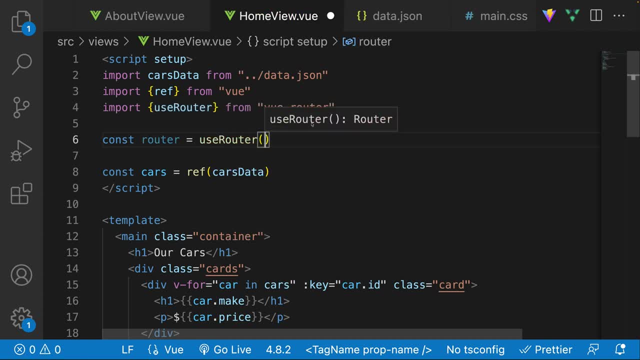 const router is equal to use router. and then what we're very use router, and then what we're very use router, and then what we're very simply going to do, simply going to do. simply going to do- is over here we're going to add a click. 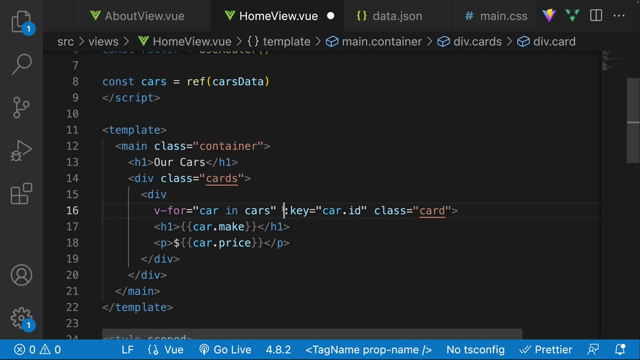 is over here we're going to add a click is over here we're going to add a click handler and let me just kind of handler and let me just kind of handler and let me just kind of multi-line, this, multi-line, this, multi-line, this. so we're going to add a click handler. 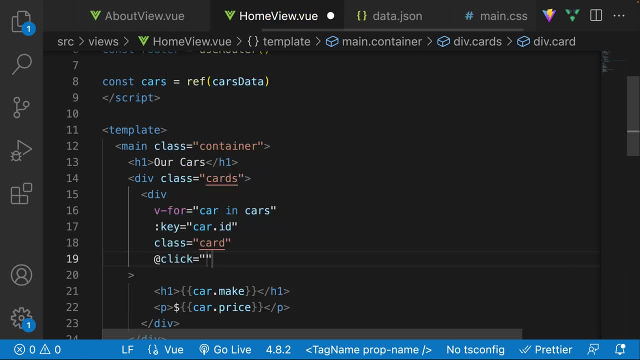 so we're going to add a click handler, so we're going to add a click handler and we're going to say add click and we're going to say add click and we're going to say add click and we're going to say router, and then 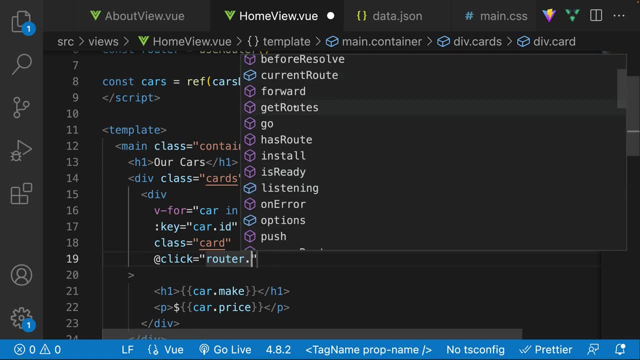 and we're going to say router, and then, and we're going to say router, and then we're going to say dot, and you can see we're going to say dot, and you can see we're going to say dot. and you can see here that there's a bunch of different. 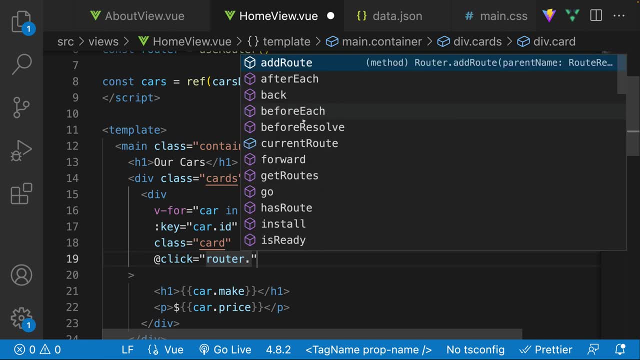 here that there's a bunch of different here, that there's a bunch of different methods that we can do, and all of these methods that we can do and all of these methods that we can do and all of these methods actually update methods, actually update methods, actually update our path. so over here i'm going to say our path. so over here, i'm going to say our path. so over here, i'm going to say routerpush. i'm going to go ahead and routerpush, i'm going to go ahead and routerpush, i'm going to go ahead and invoke it, invoke it. 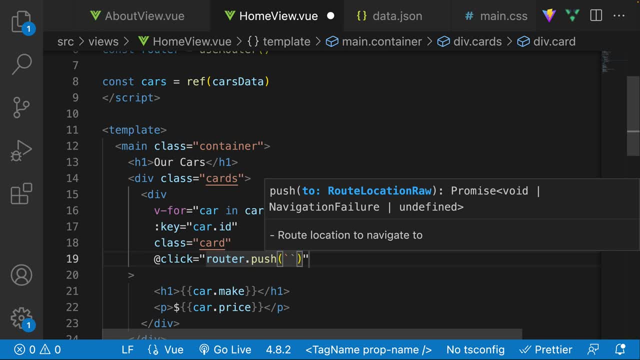 invoke it, and i'm going to push a particular path and i'm going to push a particular path and i'm going to push a particular path. specifically. what i'm going to do, specifically what i'm going to do, specifically what i'm going to do is i'm going to push the slash car. 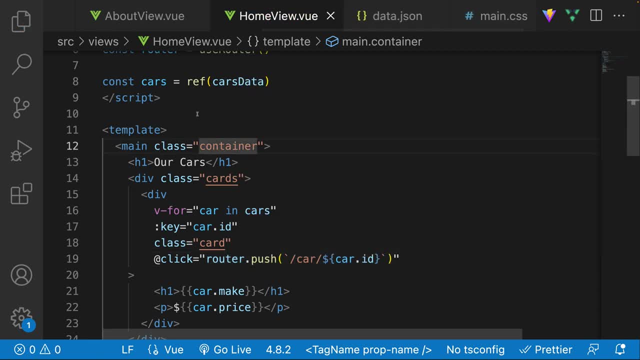 is i'm going to push the slash car, is i'm going to push the slash car and then i'm going to say car, and then i'm going to say car and then i'm going to say car dot id path. so this is how we can. 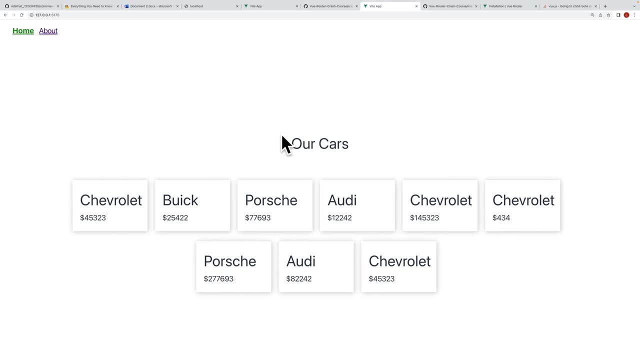 dot id path. so this is how we can dot id path. so this is how we can actually programmatically do it. actually programmatically. do it actually programmatically. do it: instead of changing our uh component to. instead of changing our uh component to, instead of changing our uh component to router link. 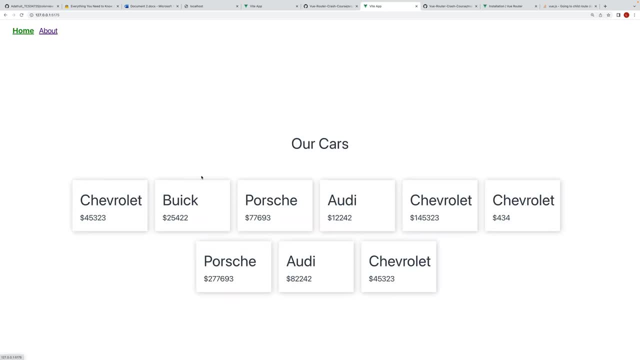 router link. router link. so now you can see that this is still so. now you can see that this is still so. now you can see that this is still working, working, working the exact same way, alrighty, so this is the exact same way, alrighty, so this is. 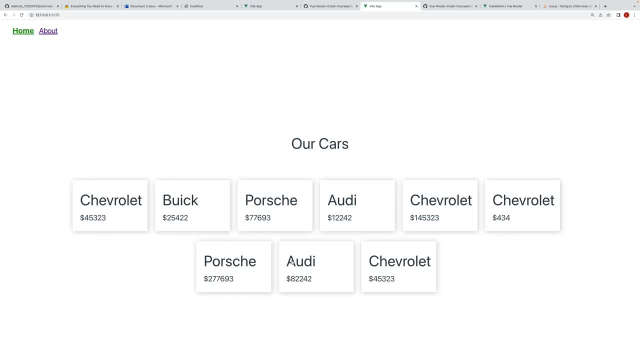 the exact same way. alrighty, so this is looking, looking, looking pretty good. so now we actually learned pretty good. so now we actually learned pretty good. so now we actually learned how to apply these, how to apply these, how to apply these dynamic uh um routes, dynamic uh um routes. 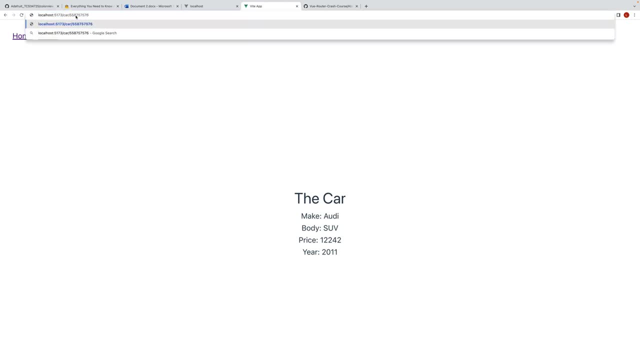 dynamic, uh um routes, i don't know. maybe adds an id here, i don't know, maybe adds an id here. i don't know, maybe adds an id here that doesn't really exist in our database. that doesn't really exist in our database. that doesn't really exist in our database. when we do that, we actually get. 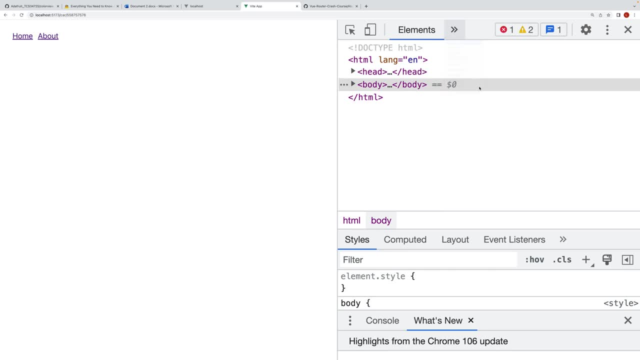 when we do that we actually get. when we do that, we actually get an error. if we were to inspect here we an error. if we were to inspect here we an error. if we were to inspect here, we were to get to go to the console and you 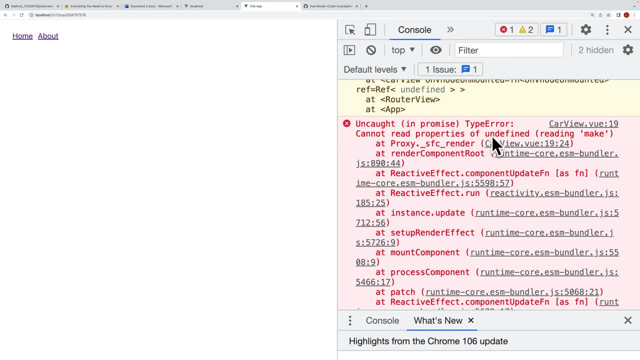 were to get to go to the console and you were to get to go to the console and you can see here that we're getting you know, can see here that we're getting you know, can see here that we're getting you know an error saying that this is undefined. we. 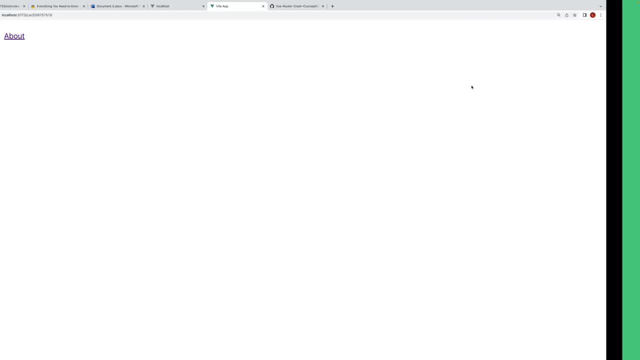 an error saying that this is undefined. we an error saying that this is undefined. we cannot read the makeup undefined kind, cannot read the makeup undefined kind, cannot read the makeup undefined kind of that typical error, of that typical error of that typical error. so what we need to do is we actually need 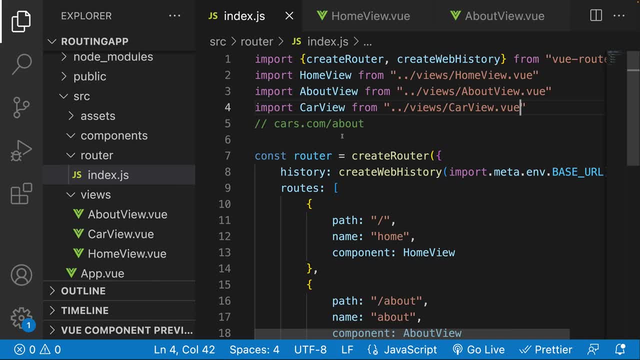 so what we need to do is we actually need. so what we need to do is we actually need to handle when we don't find a to handle, when we don't find a to handle, when we don't find a particular car, and this isn't anything. 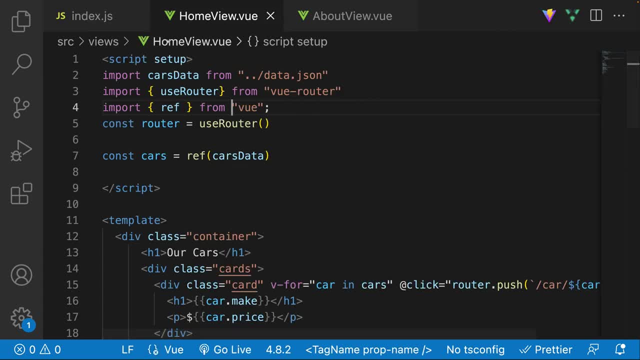 particular car and this isn't anything particular car and this isn't anything view router related. this is just kind of view router related. this is just kind of view router related. this is just kind of viewish itself. so what we can do here, viewish itself, so what we can do here. 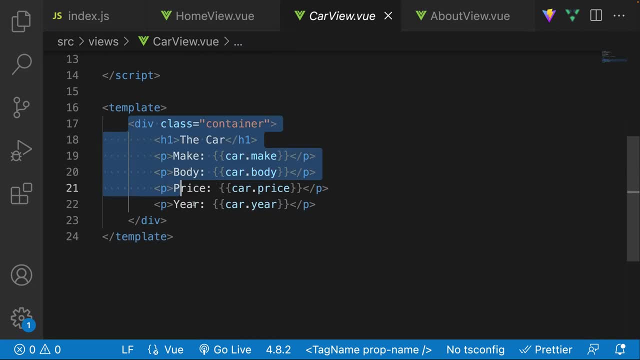 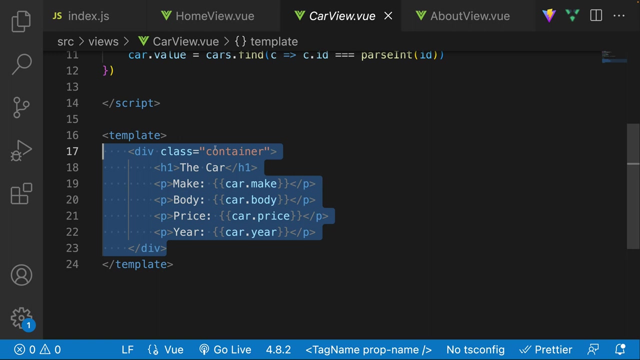 viewish itself. so what we can do here very simply, very simply, very simply is: we can just go over here and we can, is we can just go over here and we can, is we can just go over here and we can do that car. so let's actually go ahead and 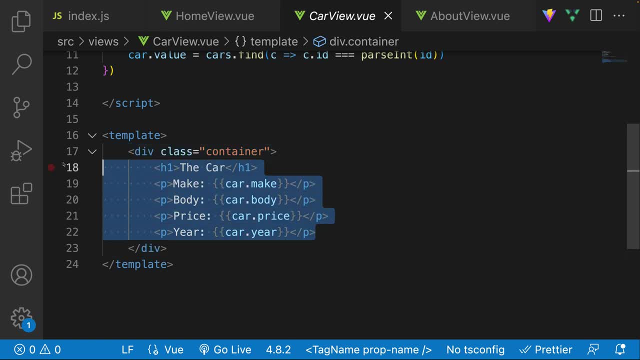 do that car. so let's actually go ahead and do that car. so let's actually go ahead and do that right now. so i'm going to do that right now. so i'm going to do that right now. so i'm going to kind of wrap all of this right now in a div. 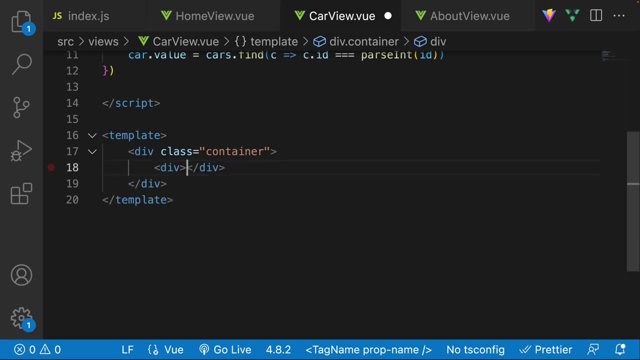 kind of wrap all of this right now in a div, kind of wrap all of this right now in a div itself, itself, itself, and within this div i'm going to go, and within this div i'm going to go, and within this div i'm going to go ahead and paste everything. actually, i 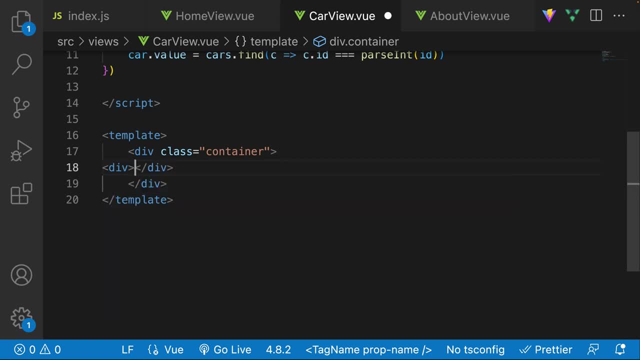 ahead and paste everything. actually, i ahead and paste everything. actually, i accidentally copied- let's go here- and accidentally copied- let's go here and accidentally copied, let's go here. and we're going to wrap it inside of the. we're going to wrap it inside of the. 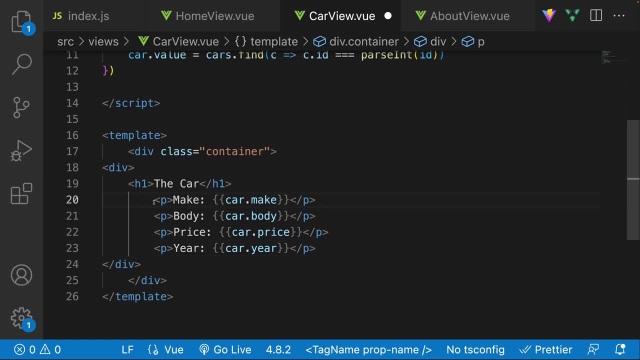 we're going to wrap it inside of the div. we're going to paste everything right, div. we're going to paste everything right, div. we're going to paste everything right in there, in there, in there, and let's just make sure that everything, and let's just make sure that everything. 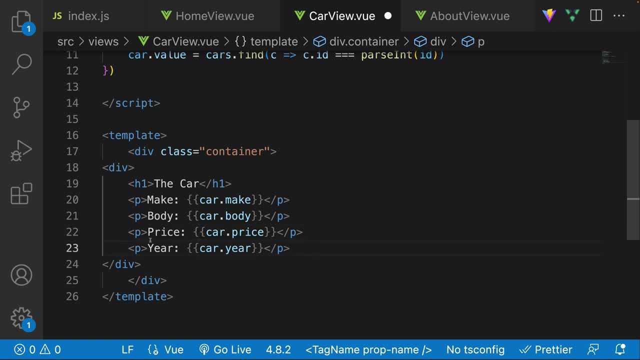 and let's just make sure that everything is nice and tabulated is nice and tabulated is nice and tabulated. and there we go. so now, and there we go, so now and there we go. so now we're going to go ahead and add a v. 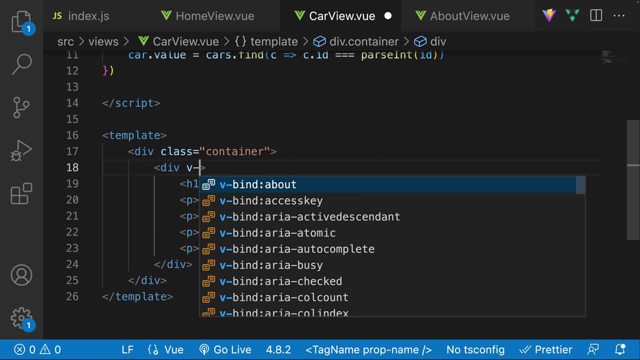 we're going to go ahead and add a v. we're going to go ahead and add a v if directive. to this, we're going to say if directive. to this, we're going to say if directive to this, we're going to say hey v if, hey v if. 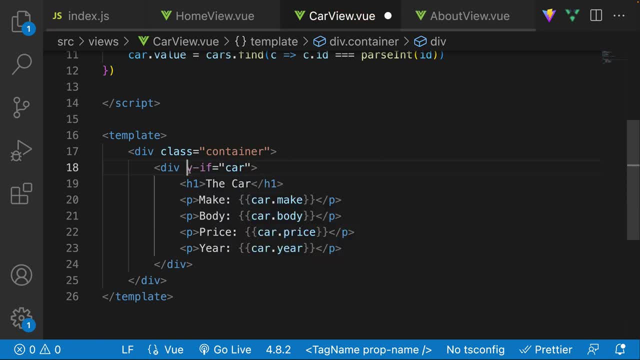 hey v. if so, if you have found this, so if you have found this, so if you have found this, then we're going to say car like so so v. then we're going to say car like so so v. then we're going to say car like so so v of car. then we want to render the car. 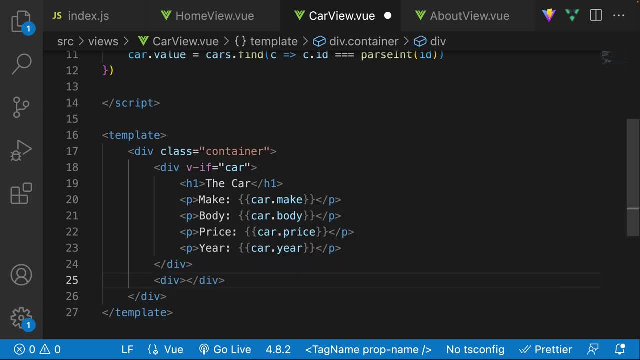 of car, then we want to render the car of car, then we want to render the car, and then, of course, what we're going to, and then, of course, what we're going to, and then, of course, what we're going to have here is a v else directive, and we 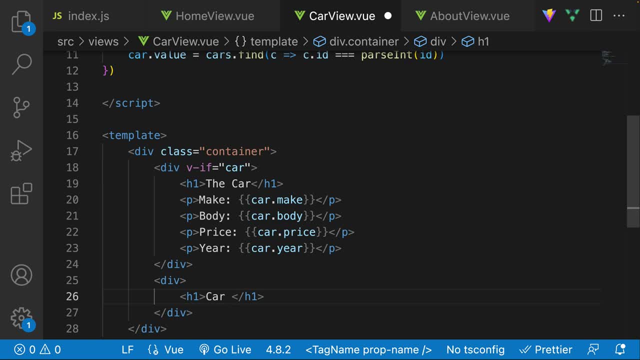 have here is a v else directive and we have here is a v else directive and we can say something like car can say something like car can say something like car not found so, car not found like so, not found so. car not found like so, not found so, car not found like so. and over here we can have a v else. 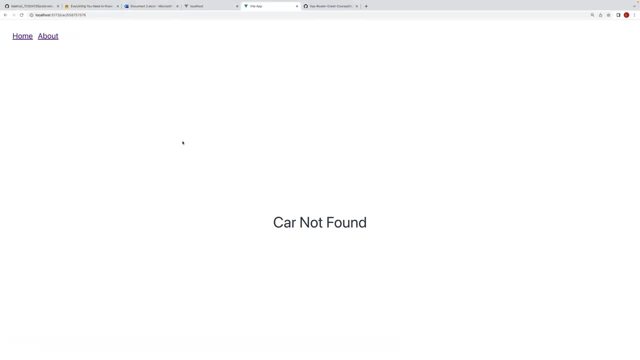 and over here we can have a v else, and over here we can have a v else: directive, directive, directive. so now if we were to go back over here? so now, if we were to go back over here? so now, if we were to go back over here, you can see, this time, instead of getting, 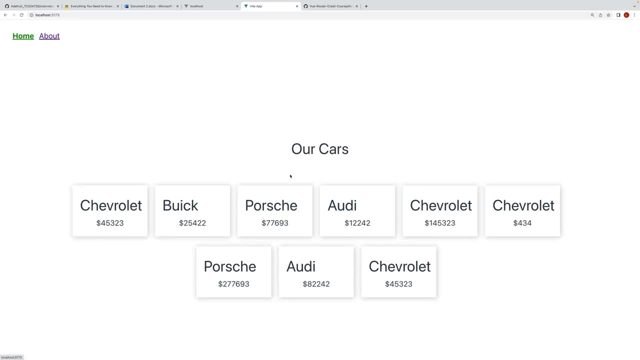 you can see this time instead of getting. you can see this time, instead of getting an error: we're getting a car not found, an error. we're getting a car not found, an error. we're getting a car not found, so the user can just go back home and 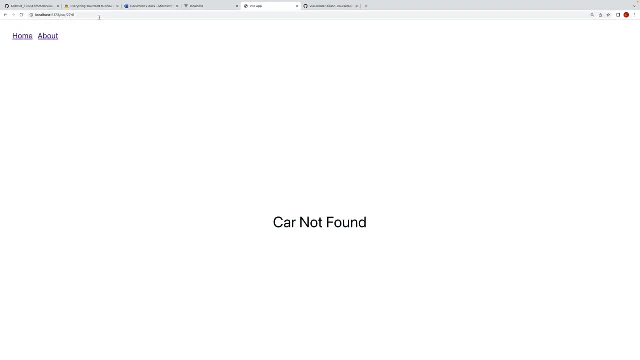 so the user can just go back home, and so the user can just go back home and select a particular car, select a particular car, select a particular car. but this actually presents a little bit, but this actually presents a little bit, but this actually presents a little bit of an issue here. so what if now? 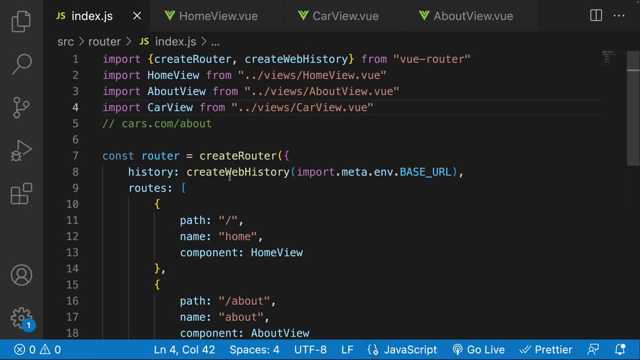 of an issue here. so what if now? of an issue here? so what if now a user follows a path, goes to a path? a user follows a path, goes to a path. a user follows a path that doesn't really exist inside of our. that doesn't really exist inside of our. 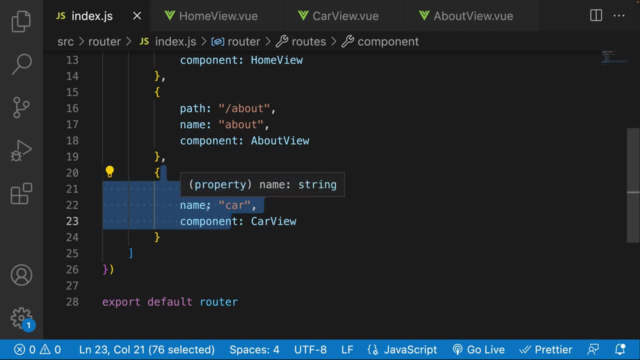 that doesn't really exist inside of our application, so it doesn't really render application. so it doesn't really render application. so it doesn't really render any particular component. what do you any particular component? what do you any particular component? what do you think is going to happen in this case? 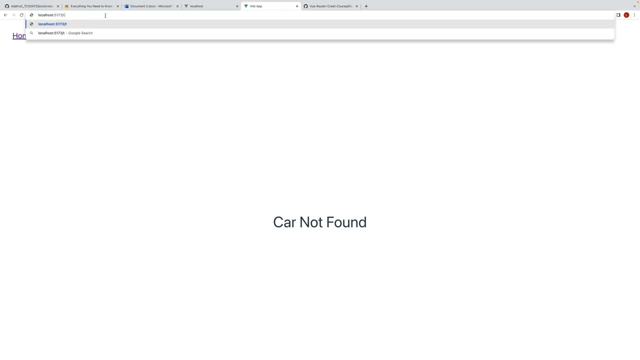 think is going to happen in this case. think is going to happen in this case. well, in this case, what's going to happen? well, in this case, what's going to happen? well, in this case, what's going to happen is it's just going to render nothing. so 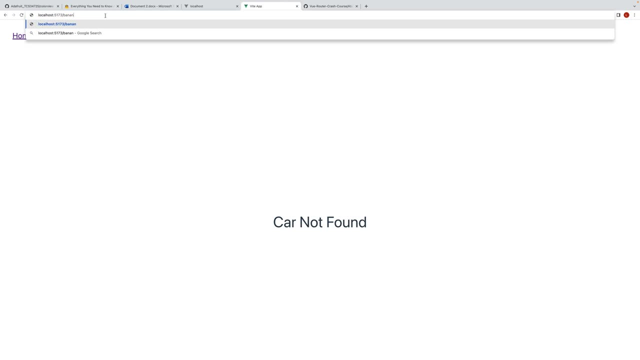 is it's just going to render nothing. so is it's just going to render nothing. so if i go to slash, let's say: if i go to slash, let's say: if i go to slash, let's say banana, banana, banana, oranges, for example, it's just not going. 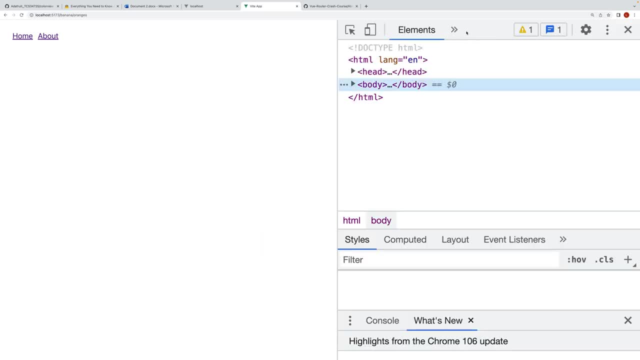 oranges, for example. it's just not going to render any component. so if i were to to render any component, so if i were to to render any component, so if i were to actually inspect this, we're not getting actually inspect this. we're not getting actually inspect this. we're not getting any error, we're just not rendering. 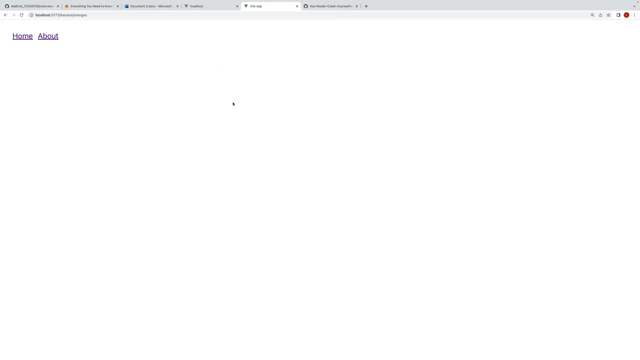 any error. we're just not rendering any error. we're just not rendering anything. so we could go this, this route, anything. so we could go this, this route, anything so we could go this, this route. it's 100, it's 100, it's 100 possible. we could do this, or what we could. 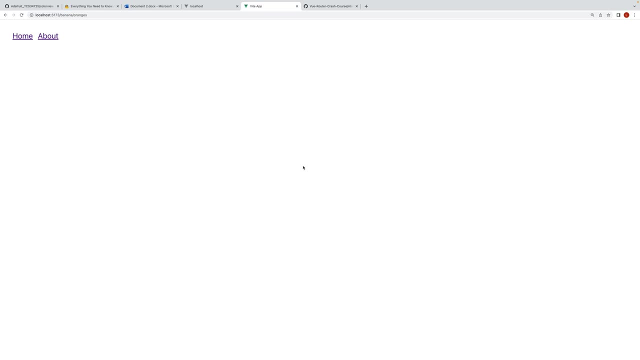 possible we could do this or what we could possible we could do this, or what we could do is show some sort of 404 page. do is show some sort of 404 page. do is show some sort of 404 page telling them: hey, we, we can't find this. 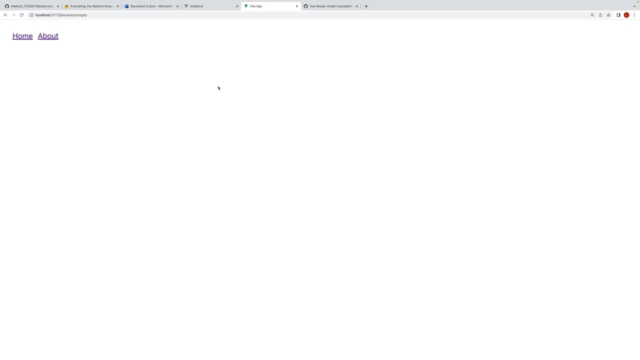 telling them, hey, we, we can't find this. telling them, hey, we, we can't find this, you can't find this page that you are. you can't find this page that you are, you can't find this page that you are looking for. so, to do that what we can, 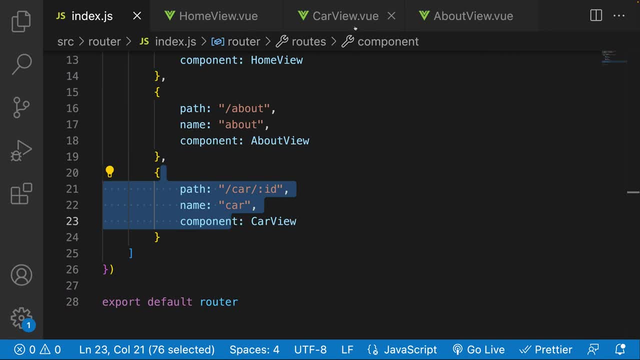 looking for, so to do that, what we can looking for, so to do that. what we can very simply do here is go over to our very simply do here is go over to our very simply do here is go over to our, our rules, and what we're going to do is. 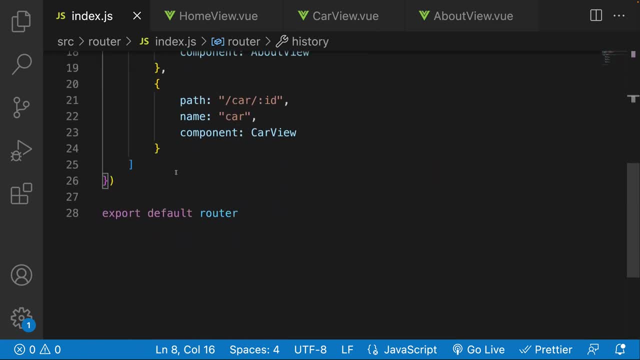 our rules and what we're going to do is our rules. and what we're going to do is we're going to add a catch all route. so we're going to add a catch all route. so we're going to add a catch all route. so right over here, we're going to say: 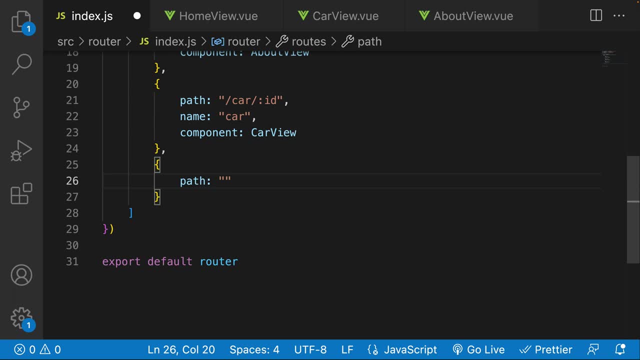 right over here we're going to say: right over here we're going to say: path, path, path, and this is where we're going to use a, and this is where we're going to use a and this is where we're going to use a regular expression. so we're going to say: 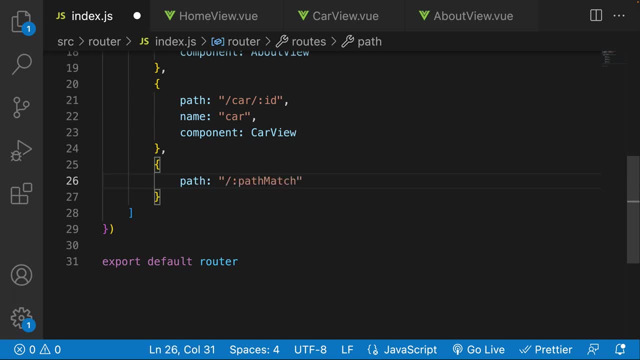 regular expression. so we're going to say regular expression. so we're going to say colon and we're going to say colon, and we're going to say colon and we're going to say path match, we can call this whatever it. path match, we can call this whatever it. 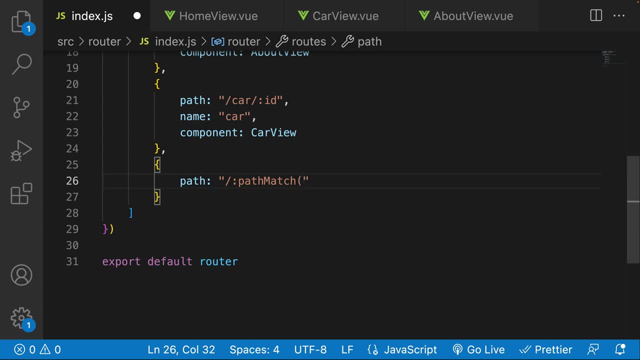 path match. we can call this, whatever it is, that we want. what's important now is is that we want. what's important now is is that we want. what's important now is: we're going to use a regular expression. we're going to use a regular expression. 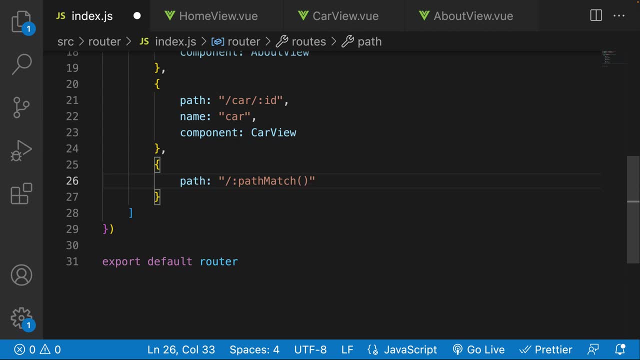 we're going to use a regular expression saying that, hey, i want to catch all. saying that, hey, i want to catch all. saying that, hey, i want to catch all, doesn't really matter what it is i want, doesn't really matter what it is i want, doesn't really matter what it is, i want to catch it all. so we're going to say: 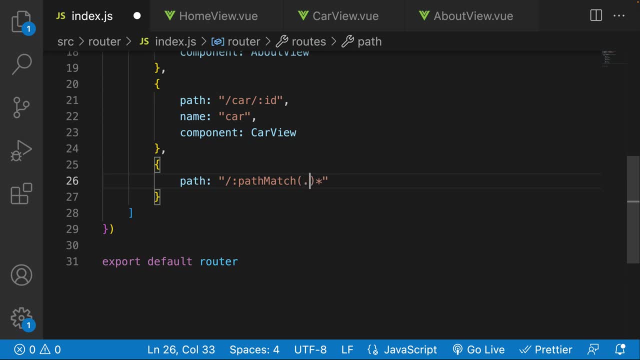 to catch it all. so we're going to say to catch it all. so we're going to say over here, and then we're going to say over here, and then we're going to say over here, and then we're going to say dot star, like so, and that is going to. 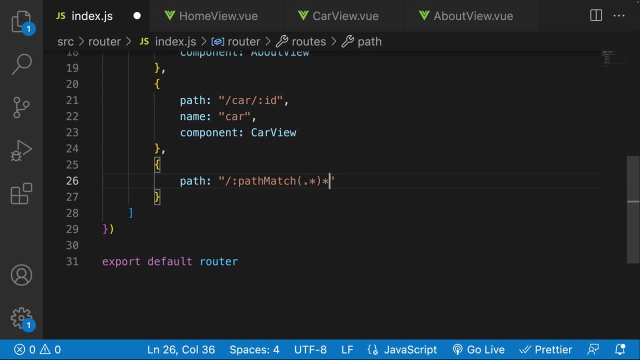 dot star like so, and that is going to dot star like so, and that is going to catch all of the um, all of the ones that catch all of the um, all of the ones that catch all of the um, all of the ones that weren't caught below. so if we were going, weren't caught below. so if we were going weren't caught below, so if we were going to slash about, it's going to go over to slash about, it's going to go over to slash about, it's going to go over here and render this component. but if 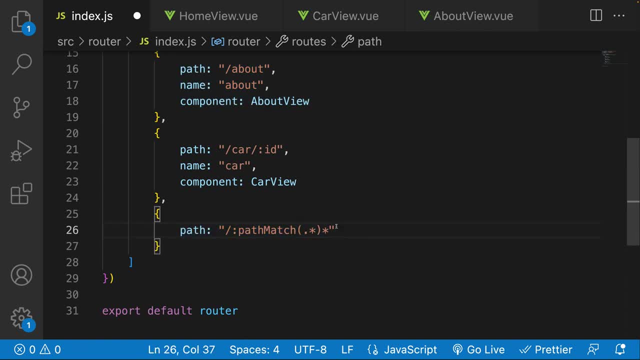 here and render this component. but if here and render this component, but if we're going to slash bananas, then it's we're going to slash bananas, then it's we're going to slash bananas, then it's going to be over here and what we want going to be over here and what we want. 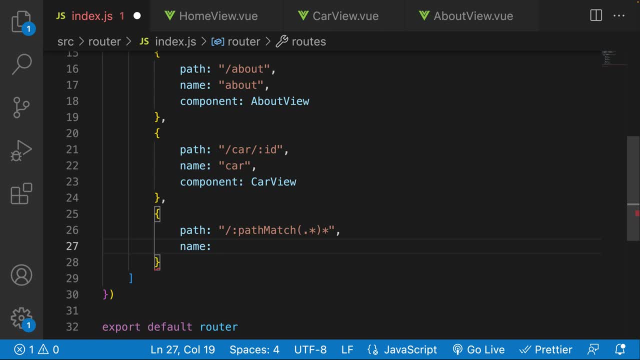 going to be over here and what we want to do here is render a not found page to do here is render a not found page. to do here is render a not found page. so we're going to say so. we're going to say so, we're going to say a name, we're going to call this. 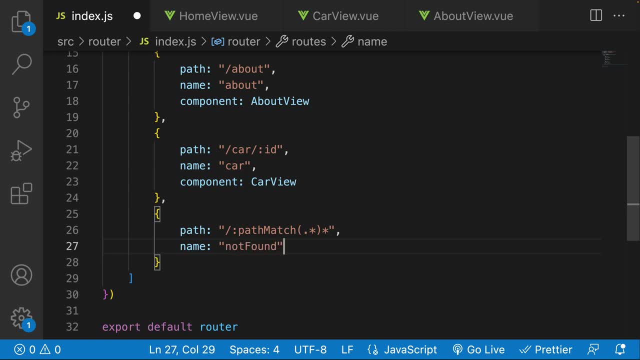 a name. we're going to call this a name. we're going to call this not not, not, not found like so, not found like so, not found like so. and then we're also going to say the, and then we're also going to say the, and then we're also going to say the component. 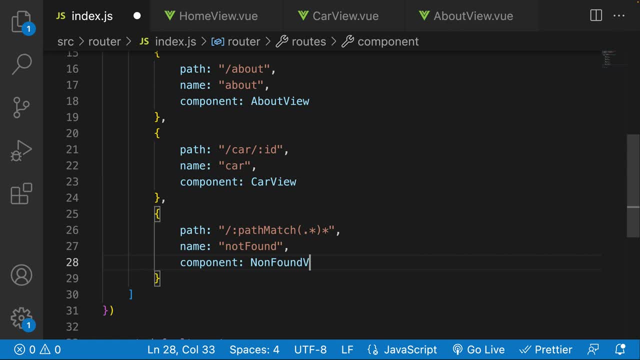 component. component is going to be the is going to be the, not found view component. so let's go. not found view component, so let's go. not found view component. so let's go ahead and import that we haven't really ahead and import that we haven't really. 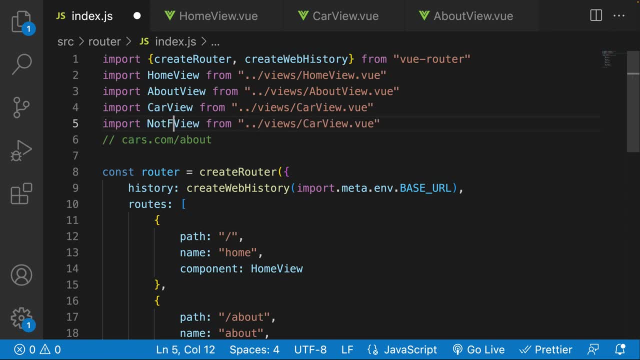 ahead and import that. we haven't really created it. let's just go ahead, created it. let's just go ahead, created it. let's just go ahead and import it, and we'll say not found and import it. and we'll say not found and import it. and we'll say not found. and then 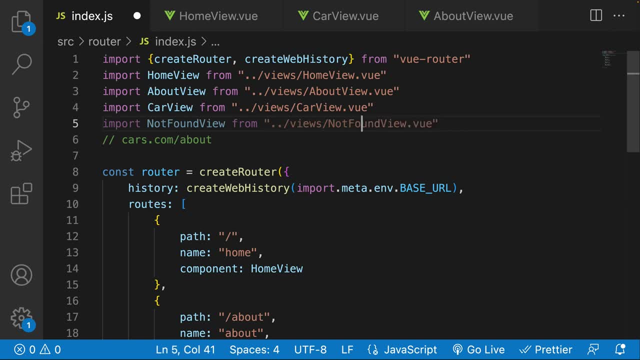 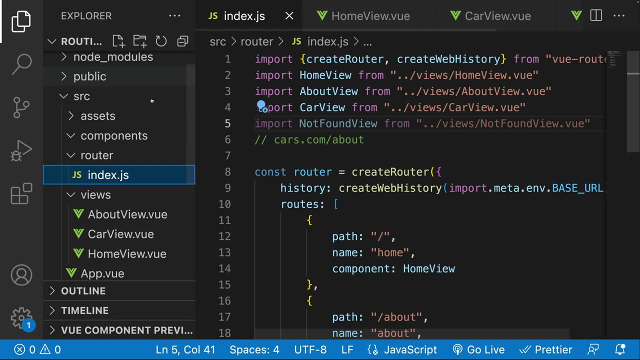 and then, and then, not found, not found, not found, and now we have to actually create this, and now we have to actually create this, and now we have to actually create this component, component, component. so let's go over to our views. so let's go over to our views. 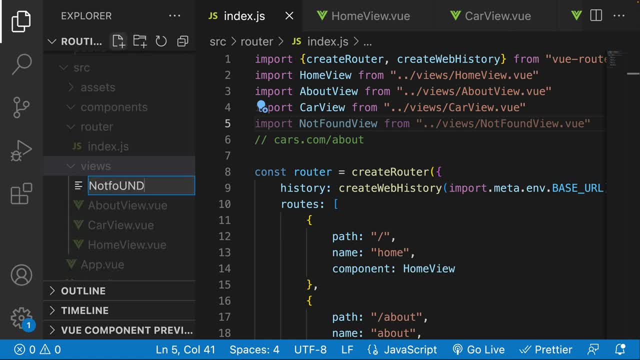 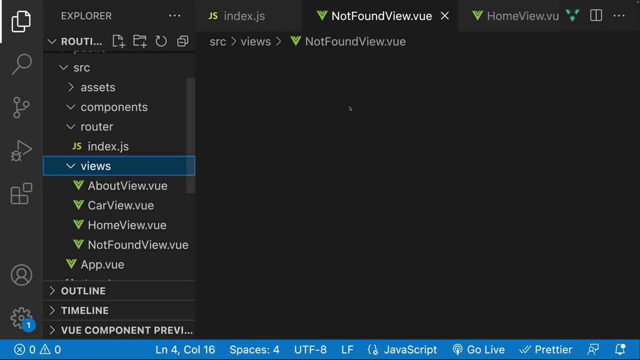 so let's go over to our views. so views, and we're going to say not so views, and we're going to say not so views and we're going to say not view dot view like so all right, so now. view dot view like so all right, so now. 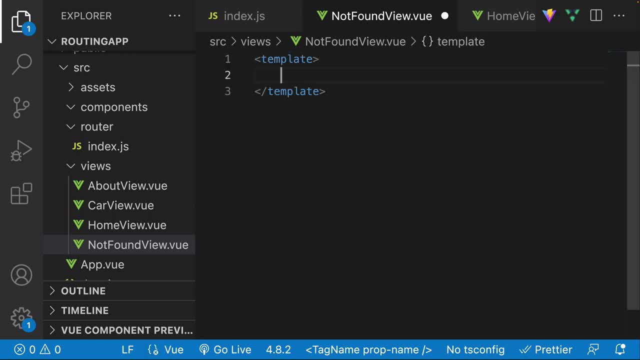 view, dot, view, like. so all right, so now let's just create a very simple uh, not, let's just create a very simple uh, not, let's just create a very simple uh, not found component. so we're going to say found component. so we're going to say: 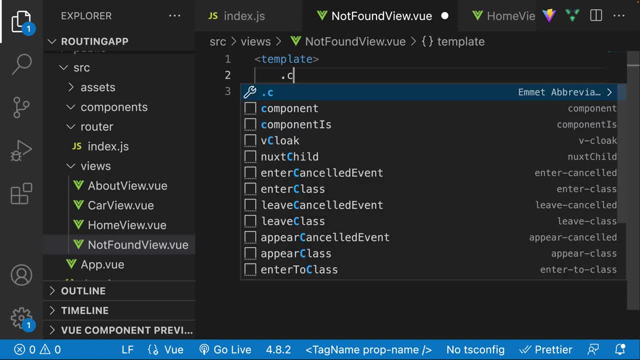 found component. so we're going to say div here. we're going to say div here. we're going to say div. here we're going to say container, container, container, and let me get rid of this and then over. and let me get rid of this and then over. 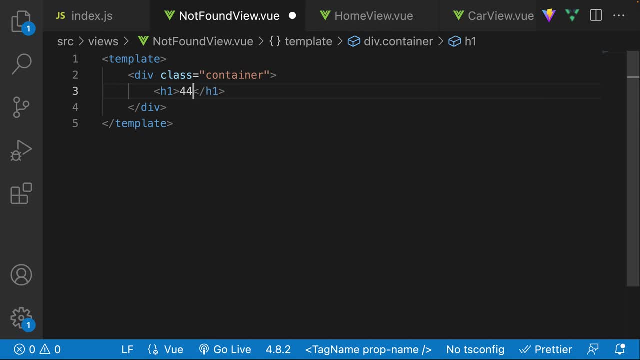 and let me get rid of this. and then over here we're just going to have an h1. here we're just going to have an h1. here we're just going to have an h1. that's going to say 404. that's going to say 404. 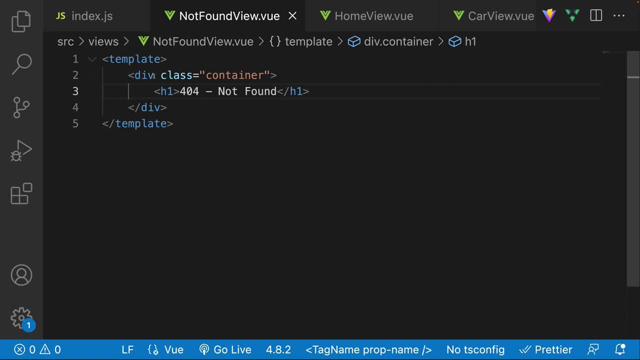 that's going to say 404 and not found like that. okay, so that's. and not found like that. okay, so that's, and not found like that. okay, so that's pretty much. it, pretty much it, pretty much it. so now i'm going to go ahead and refresh. 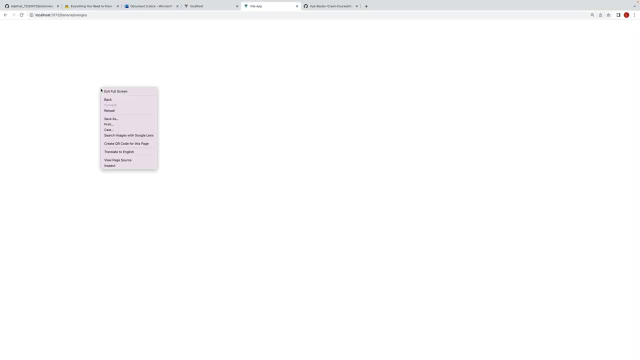 so now i'm going to go ahead and refresh. so now i'm going to go ahead and refresh this, this, this. are we still getting this error? we are. are we still getting this error? we are. are we still getting this error? we are indeed. what's going on? let's inspect. 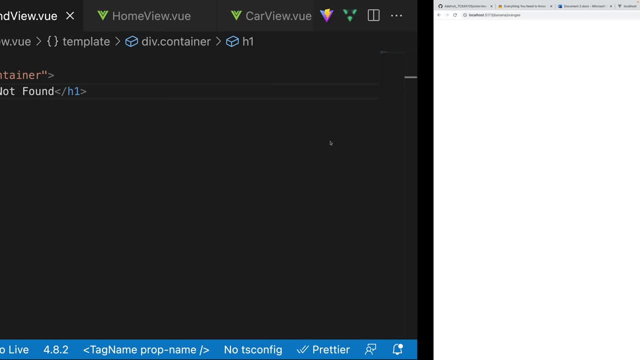 indeed what's going on. let's inspect, indeed what's going on, let's inspect. so we're getting an error saying non. so we're getting an error saying non. so we're getting an error saying non found. i should have called this not found. i should have called this not. 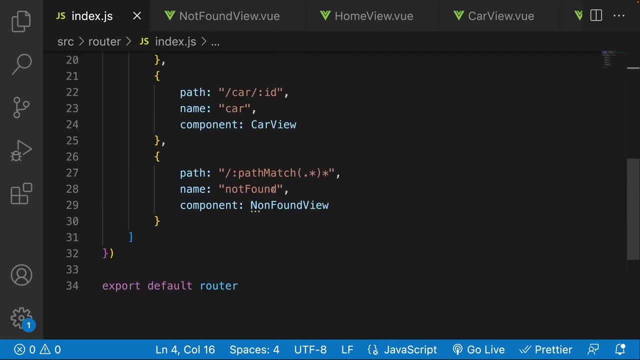 found. i should have called this not found, not non found found, not non found. found, not non found. uh, let's go here and change that to not. uh, let's go here and change that to not. uh, let's go here and change that to not found found. 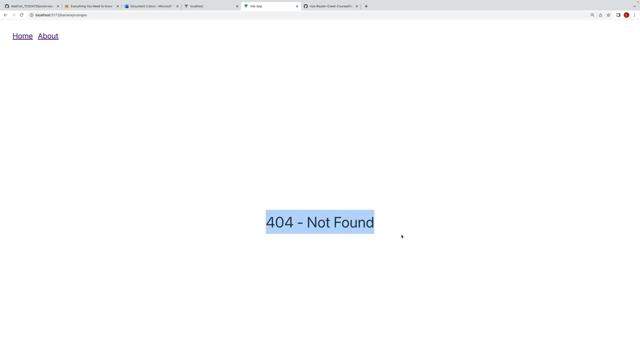 found: all right, there we go. so now you can see: all right, there we go. so now you can see: all right, there we go. so now you can see that anytime we go to a path, that that, anytime we go to a path, that that, anytime we go to a path that doesn't exist, we're rendering the not. 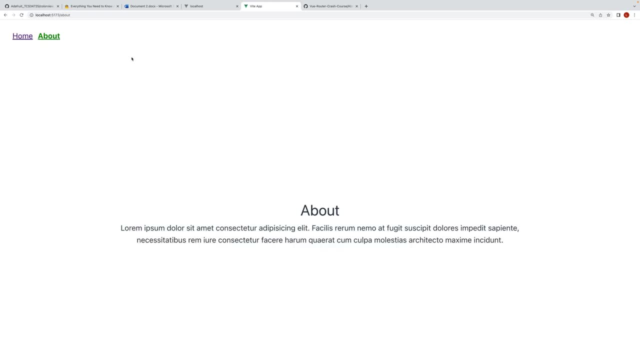 doesn't exist. we're rendering the not doesn't exist. we're rendering the not found. however, if we go home, we render found. however, if we go home, we render found. however, if we go home, we render this, this, this, for on about. we render this for on a. 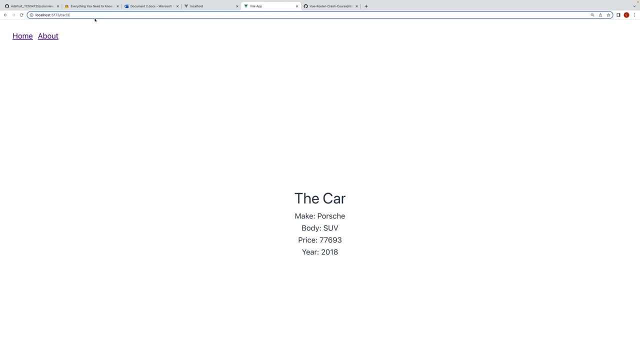 for on about we render this for on a for on about we render this for on a specific path. but let's say we go now for on about we render this for on a specific path. but let's say we go now for on about we render this for on a specific path. but let's say we go now to slash car, slash three. 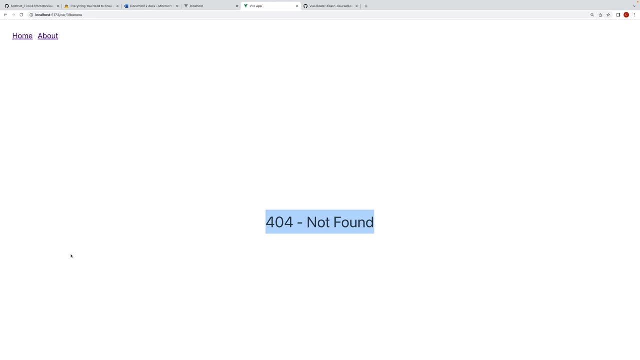 to slash car, slash three. to slash car, slash three. slash banana- that's not a supported path. slash banana, that's not a supported path. slash banana- that's not a supported path. now we have not found it okay. so now we have not found it okay. so now we have not found it okay. so this is terrific, this is great. now let's. 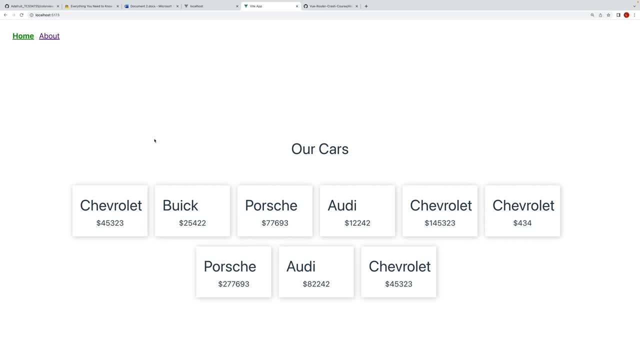 this is terrific, this is great. now let's- this is terrific, this is great. now let's actually start moving on to some of the actually start moving on to some of the actually start moving on to some of the more complicated features of view. more complicated features of view. 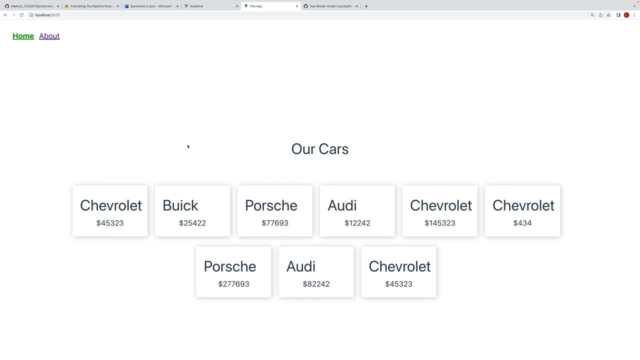 more complicated features of view routing. so let's say that i want the routing. so let's say that i want the routing. so let's say that i want the ability for my users to filter for cars, ability for my users to filter for cars, ability for my users to filter for cars, because right now we have what? how many? 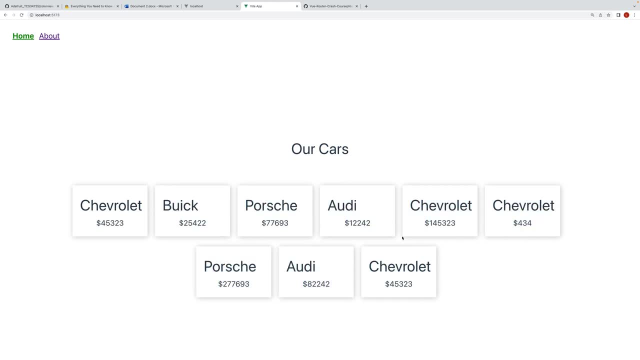 because right now we have what how many? because right now we have what? how many cars. we have six, nine cars, you know cars. we have six, nine cars, you know cars. we have six, nine cars, you know that's just too many cars for the user. that's just too many cars for the user. 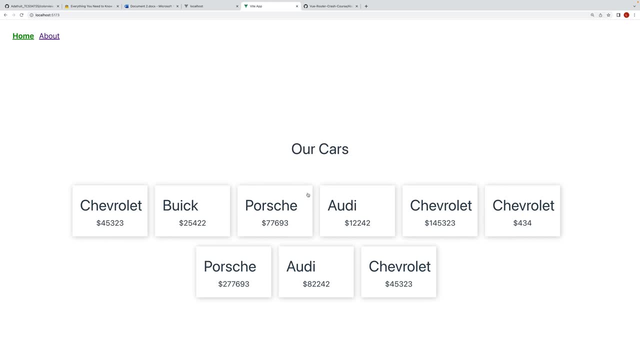 that's just too many cars for the user to look at. we want them to filter based to look at. we want them to filter based to look at. we want them to filter based on what they want. maybe they want a on what they want. maybe they want a. 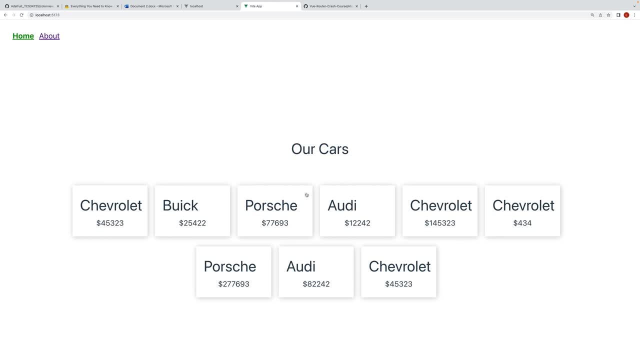 on what they want. maybe they want a specific make. maybe they want you know specific make. maybe they want you know specific make. maybe they want you know to sort their prices. sort the cars based to sort their prices. sort the cars based to sort their prices. sort the cars based on their prices, maybe from highest to 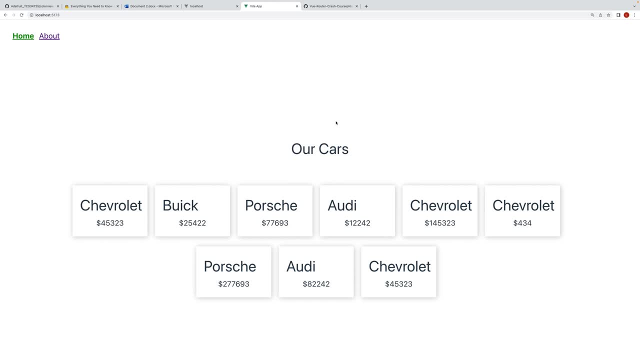 on their prices, maybe from highest to on their prices, maybe from highest to lowest, or from lowest to highest lowest or from lowest to highest- lowest or from lowest to highest. so i want to add that ability and this. so i want to add that ability and this. so i want to add that ability, and this is going to actually present a little. 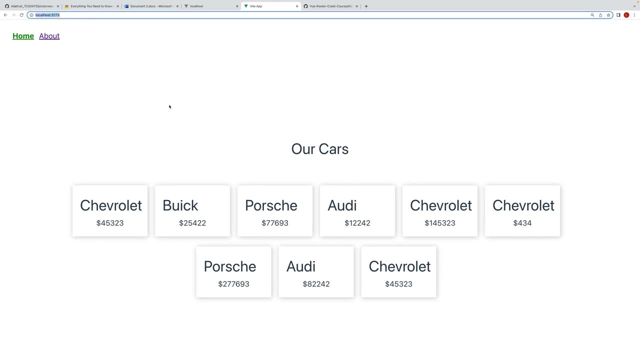 is going to actually present a little, is going to actually present a little bit of a challenge when it comes to the bit of a challenge when it comes to the bit of a challenge when it comes to the routing portion of things, so let's go. routing portion of things, so let's go. 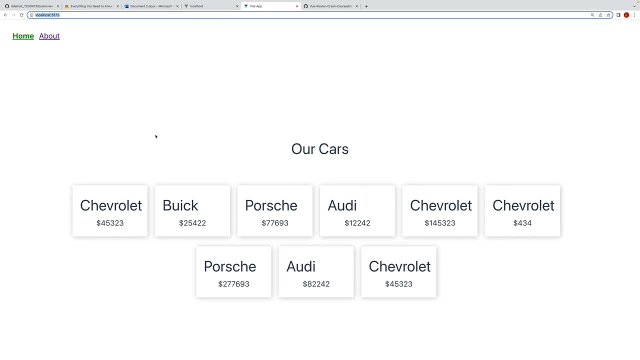 routing portion of things. so let's go ahead and actually implement this right ahead and actually implement this right ahead and actually implement this right about now, about now, about now. so i want to add the ability to go ahead. so i want to add the ability to go ahead. 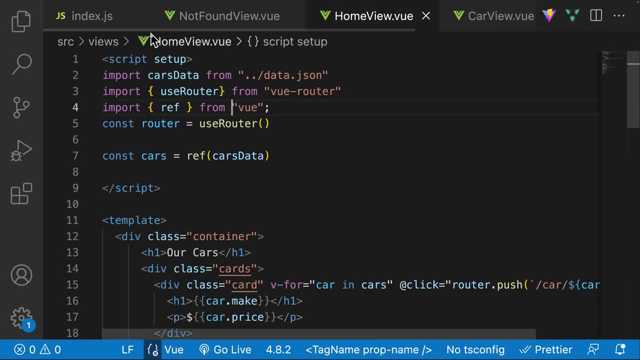 so i want to add the ability to go ahead and uh well, let's say, i want to be able. and uh well, let's say i want to be able, and uh well, let's say i want to be able to kind of filter by a specific make. so to kind of filter by a specific make. so to kind of filter by a specific make. so right now let's just add that. right now let's just add that, right now let's just add that functionality, and then later on we're functionality, and then later on we're. 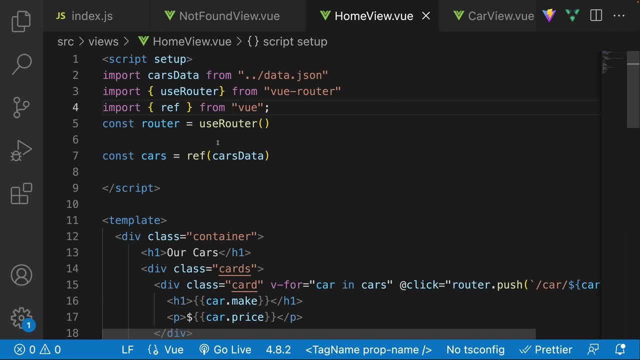 functionality, and then later on, we're going to talk about how we can kind of going to talk about how we can kind of going to talk about how we can kind of incorporate this to our routing, incorporate this to our routing, incorporate this to our routing. so i'm going to go over here and i'm 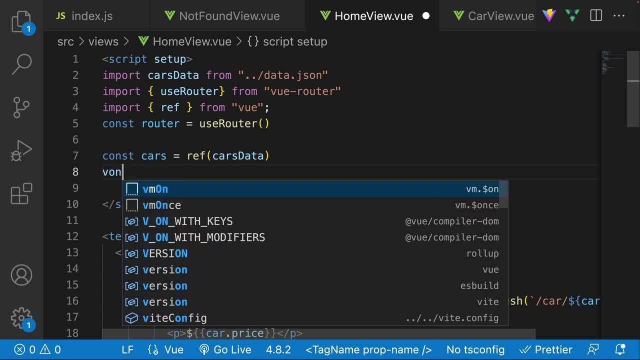 so i'm going to go over here and i'm so i'm going to go over here and i'm going to add a new piece of state and going to add a new piece of state and going to add a new piece of state and i'm going to call this piece of state. 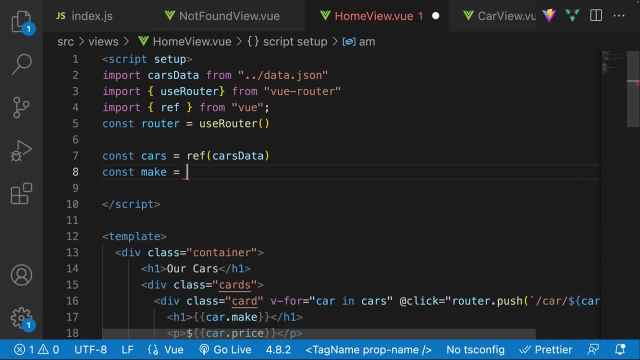 i'm going to call this piece of state. i'm going to call this piece of state make. so i'm going to say const make, make. so i'm going to say const make, make. so i'm going to say const make, and that's going to be equal to ref and 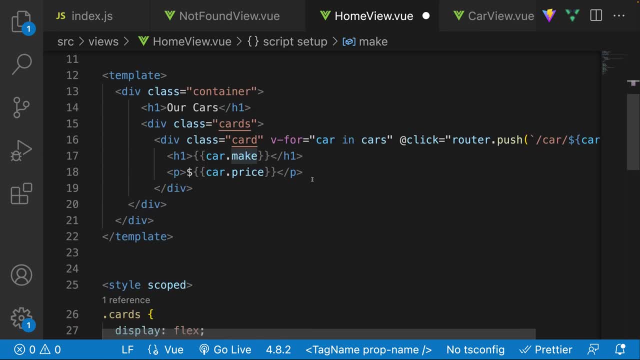 and that's going to be equal to ref, and and that's going to be equal to ref, and initially this is going to be equal to. initially this is going to be equal to. initially this is going to be equal to just something completely empty. just something completely empty. 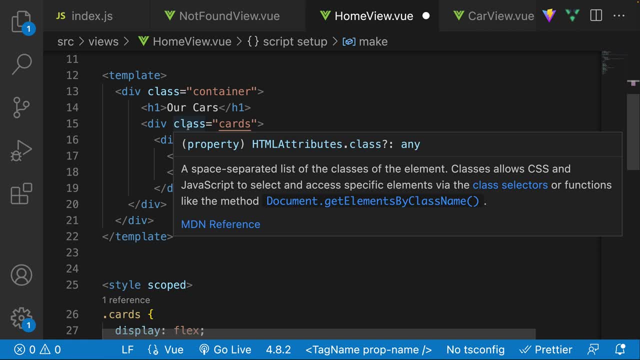 just something completely empty, and then over here inside of our view, and then over here inside of our view, and then over here inside of our view. template. let's go right below here i'm template. let's go right below here, i'm template. let's go right below here i'm going to add. 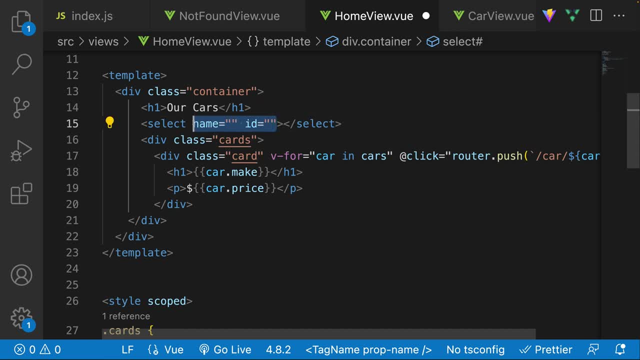 going to add, going to add a select, and let's just get rid of the a select and let's just get rid of the a select and let's just get rid of the name as well as the id- for now we don't name- as well as the id- for now we don't. 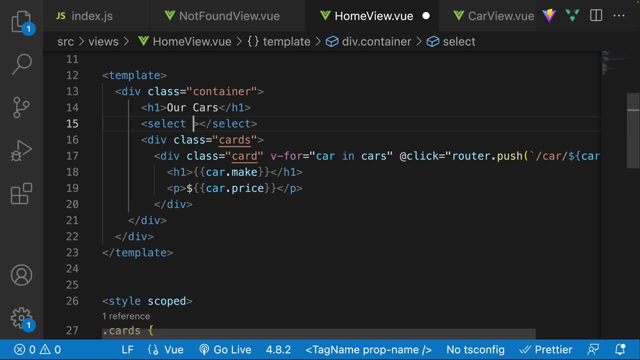 name as well as the id. for now, we don't really care for that, really care for that, really care for that, and what we're going to do is we are, and what we're going to do is we are, and what we're going to do is we are going to. 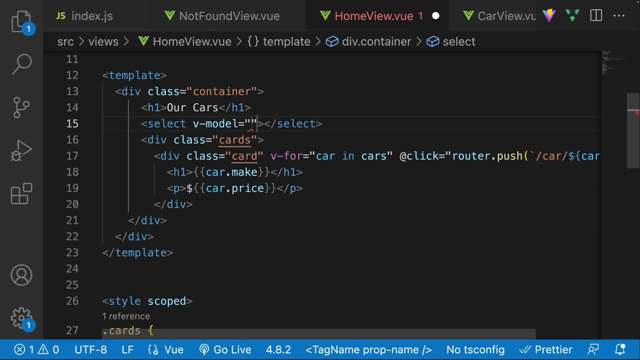 going to going to add a v model and we are going to bind add a v model and we are going to bind add a v model and we are going to bind it to it, to it, to the make itself, all right. so that's the make itself, all right, so that's. 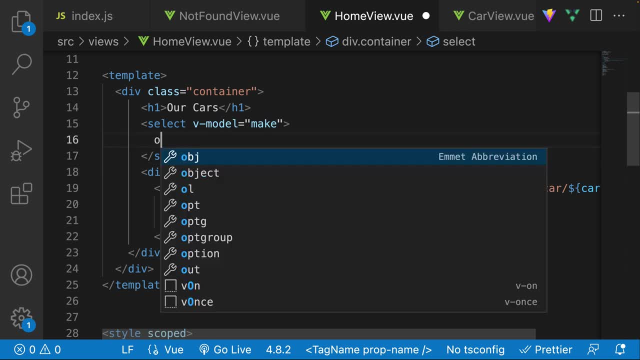 the make itself all right. so that's looking pretty good, looking pretty good, looking pretty good. and then, over here, we're going to have a, and then over here, we're going to have a, and then over here we're going to have a bunch of different options. so let's say: 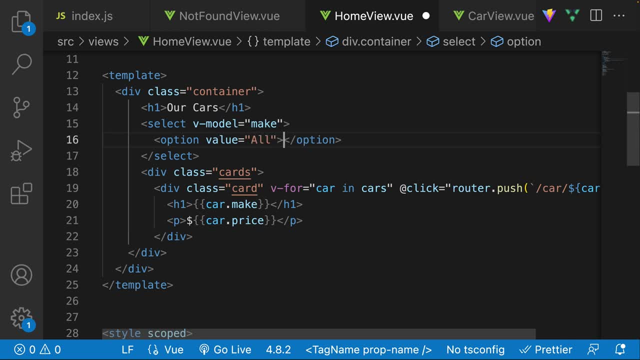 bunch of different options. so let's say bunch of different options. so let's say the first option, the first option, the first option is the all all makes we're going to say is the all all makes. we're going to say is the all all makes. we're going to say all like so. 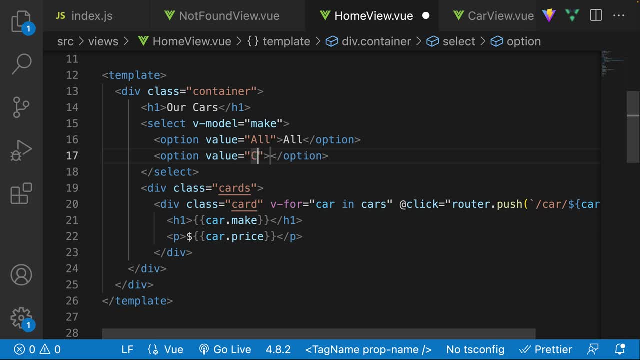 all like so, all like so, and then option of uh, and then option of uh, and then option of uh. let's say the chevy, so let's say we want. let's say the chevy, so let's say we want. let's say the chevy, so let's say we want a chevy chevrolet. 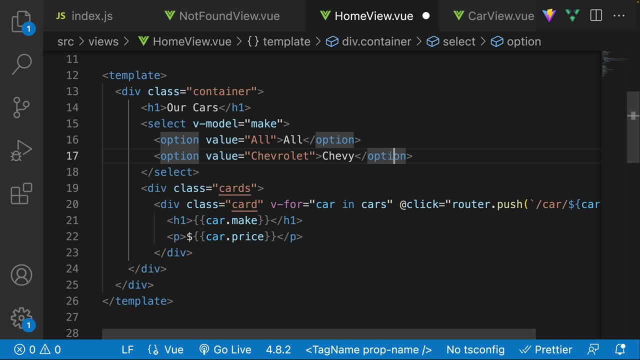 a chevy chevrolet, a chevy chevrolet, and this one also, we'll just, we'll just, and this one also, we'll just, we'll just, and this one also, we'll just, we'll just call it chevy like so, call it chevy like so, call it chevy like so. and then let's say: option another option. 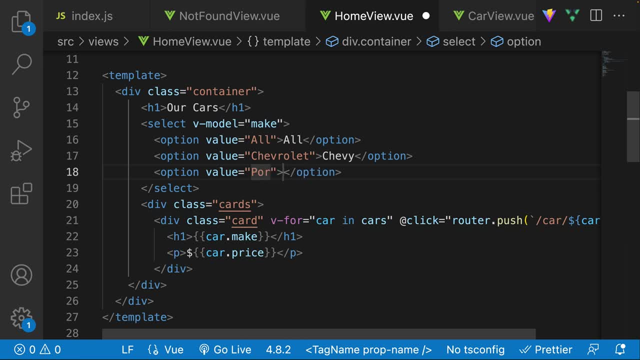 and then let's say option, another option, and then let's say option another option is porsche. so maybe you want to filter is porsche, so maybe you want to filter is porsche, so maybe you want to filter by the porsche, by the porsche. 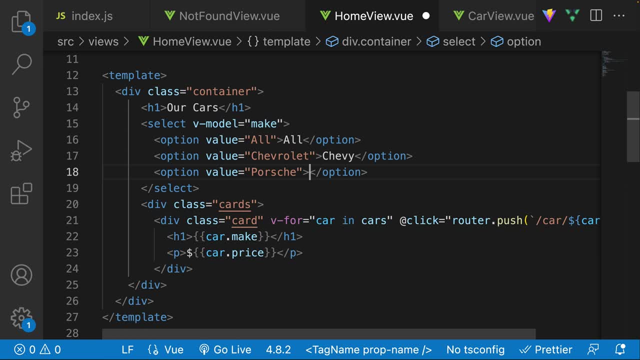 by the porsche, so porsche, so porsche, so porsche. and then over here we're going to call, and then over here we're going to call, and then over here we're going to call this porsche, this porsche, this porsche. and lastly, let's add the option to: 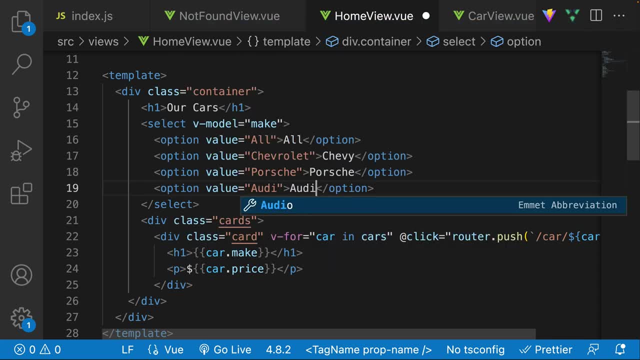 and lastly, let's add the option to: and lastly, let's add the option to: filter by the audi, so audi. filter by the audi, so audi. filter by the audi, so audi, audi. okay, so now we have this right: audi. okay. so now we have this right. 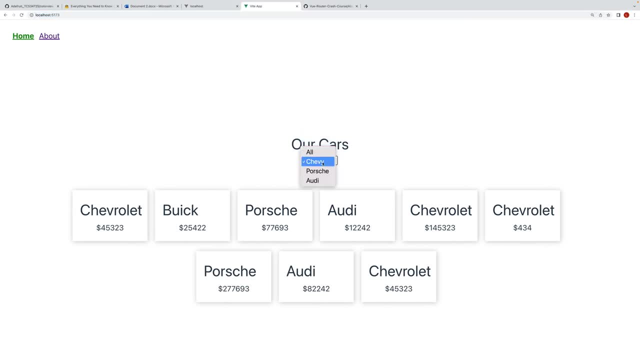 audi, okay. so now we have this right over here, we can obviously select over here. we can obviously select over here. we can obviously select whatever option it is that we want okay, whatever option it is that we want okay, whatever option it is that we want okay. so let's first add that functionality. so 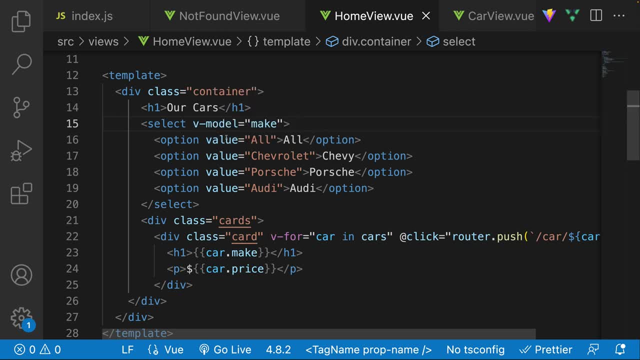 so let's first add that functionality. so, so, let's first add that functionality so that it can actually filter the way that, that it can actually filter the way that, that it can actually filter the way that we want it to. we want it to, we want it to. so anytime that we change this, then we 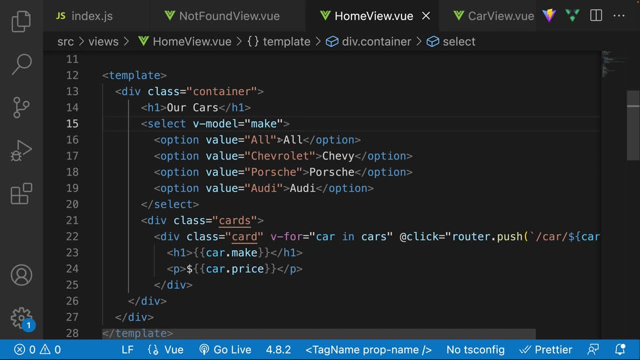 so anytime that we change this, then we, so anytime that we change this, then we want to kind of handle that particular, want to kind of handle that particular, want to kind of handle that particular. change, so over here what happens here. change so over here, what happens here. 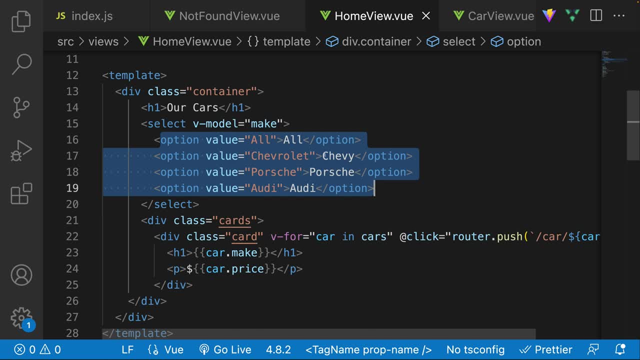 change. so, over here, what happens here when we change this, when we change this, when we change this, is that it goes ahead and it updates is that it goes ahead and it updates is that it goes ahead and it updates the make. so what we can do is we can. 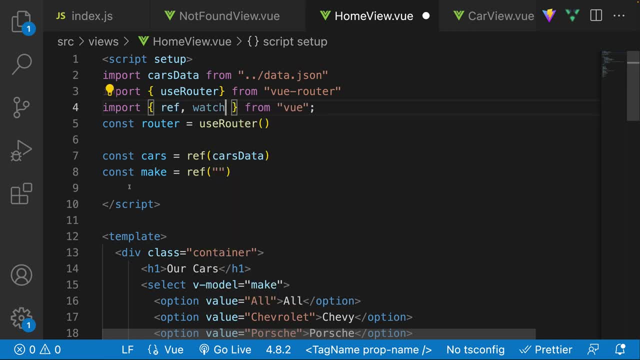 the make. so what we can do is we can the make. so what we can do is we can actually watch for any changes to this, actually watch for any changes to this, actually watch for any changes to this make. so i'm going to say watch and this: 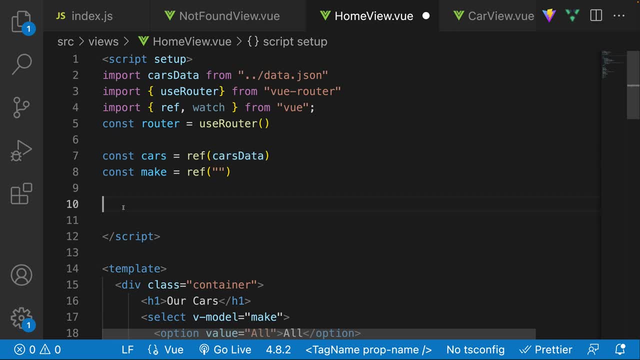 make. so i'm going to say watch and this make. so i'm going to say watch, and this is where we're going to update the cars, is where we're going to update the cars, is where we're going to update the cars state. so we're going to say watch and i 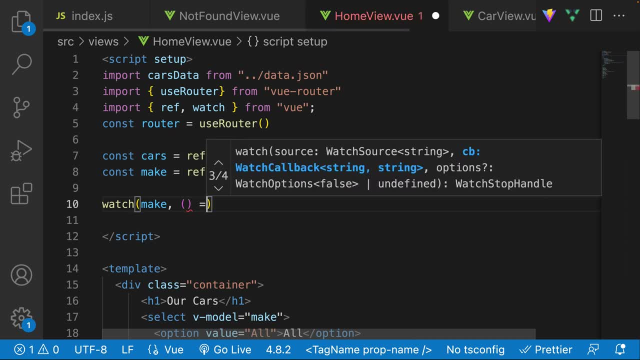 state so we're going to say watch, and i state so we're going to say watch, and i want to watch for the make and anytime want to watch for the make and anytime want to watch for the make and anytime that the make changes, i want to update. 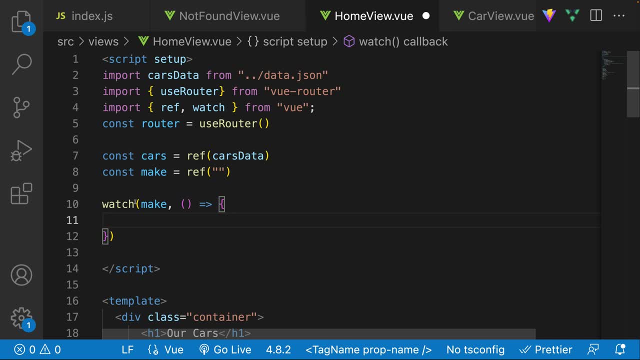 that the make changes. i want to update that the make changes. i want to update the car state, the car state, the car state. so we're going to say here: if so. we're going to say here: if so, we're going to say here: if make, so if make, dot value is not kind of. 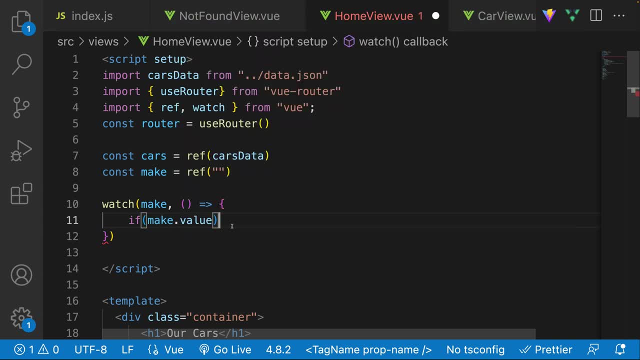 make. so if make dot value is not kind of make, so if make dot value is not kind of empty an empty string, then let's go empty an empty string. then let's go empty an empty string, then let's go ahead and actually update the thing. but 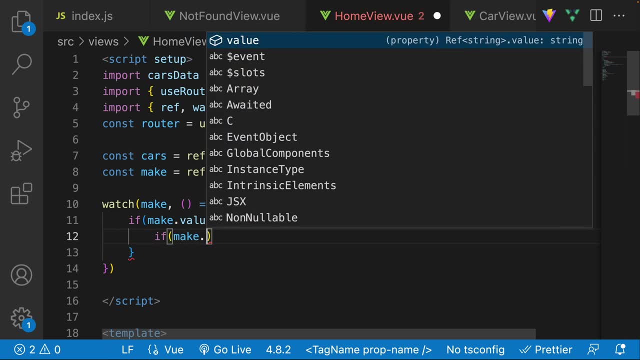 ahead and actually update the thing, but ahead and actually update the thing. but the first thing i want to do is i want. the first thing i want to do is i want. the first thing i want to do is i want to see: okay, if make dot value is equal. 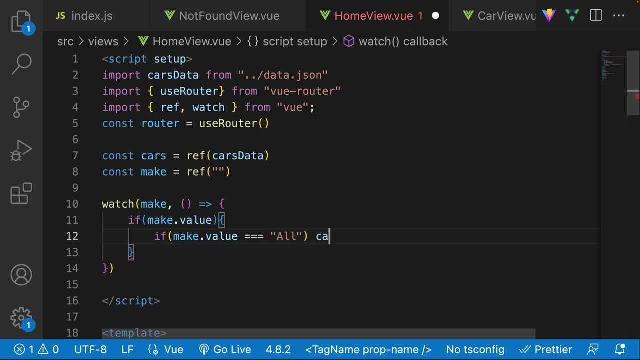 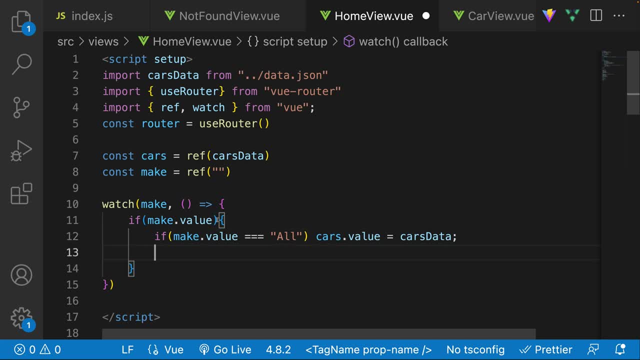 cars dot value, that's going to be equal to the cars data. the cars data. the cars data now. if that's not the case, then what we now? if that's not the case, then what we now? if that's not the case, then what we want to do is we want to filter. so 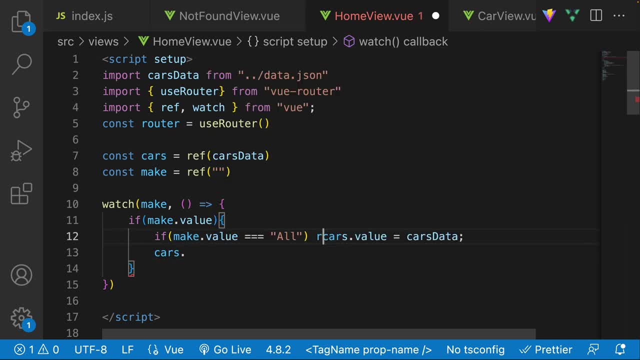 want to do is. we want to filter, so want to do is we want to filter. so we're going to say cars. we're going to say cars. we're going to say cars, dot value over here. we should probably dot value over here. we should probably dot value over here. we should probably return. 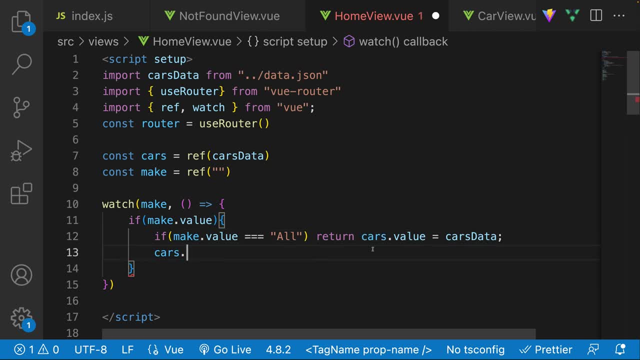 return, return, just return early, just return early, just return early. and over here we're going to say or, and over here we're going to say or, and over here we're going to say or maybe we shouldn't return early, we, maybe we shouldn't return early, we. 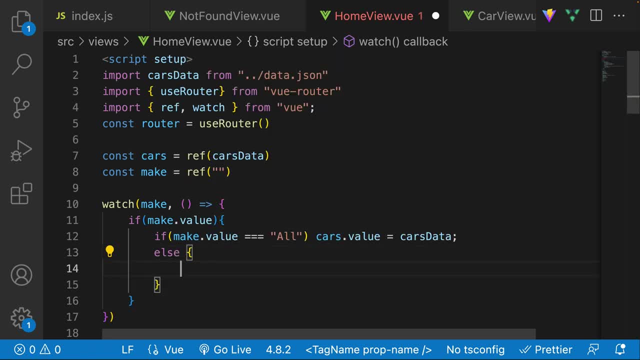 maybe we shouldn't return early. we should add an else clause. that'll be. should add an else clause, that'll be. should add an else clause, that'll be. probably be a little bit better, probably be a little bit better, probably be a little bit better. we're going to say cars, dot, value and we're going to say cars dot value and we're going to say cars dot value and we're going to say that that is going to. we're going to say that that is going to. we're going to say that that is going to be equal to. 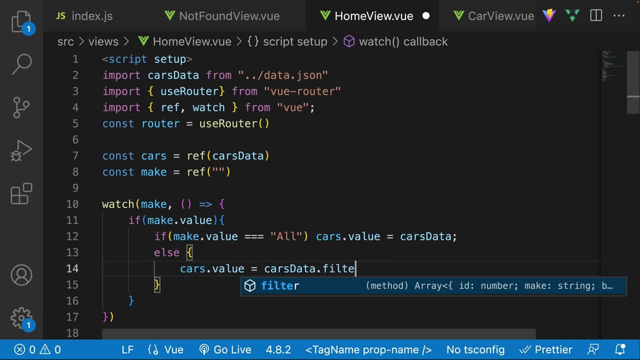 be equal to be equal to, and we're going to say cars data dot and we're going to say cars data dot and we're going to say cars data dot filter and we're going to filter for filter and we're going to filter for filter and we're going to filter for every particular car. let's just call. 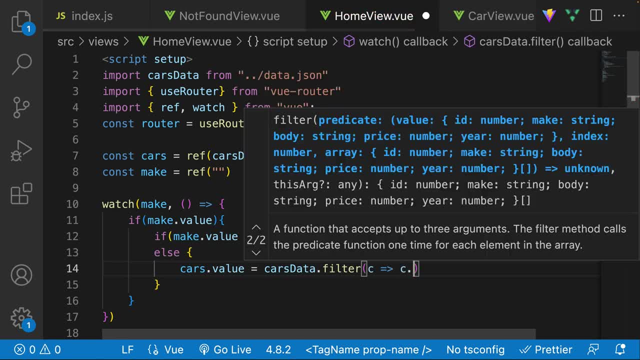 every particular car. let's just call every particular car, let's just call this, this, this c, and we're going to say car dot c and we're going to say car dot c and we're going to say car dot make or c dot make is equal to. 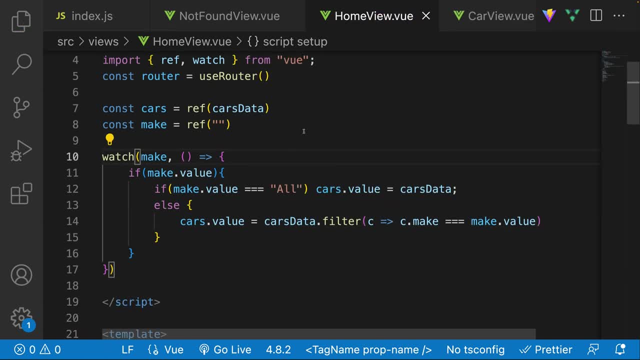 make, or c dot make is equal to make, or c dot make is equal to the make dot value, that's pretty much it. the make dot value, that's pretty much it. the make dot value, that's pretty much it. that's what we're going to have to add. 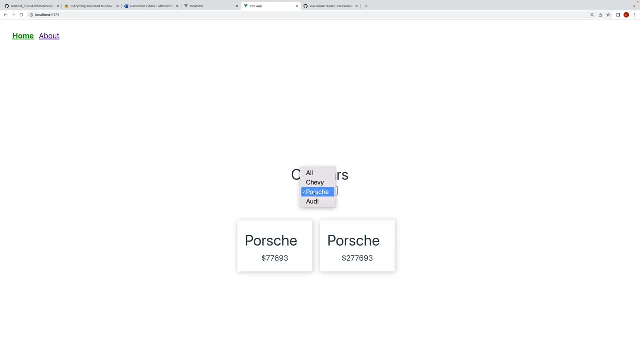 that's what we're going to have to add. that's what we're going to have to add. so now let's say we filter for porsche. so now let's say we filter for porsche. so now let's say we filter for porsche. now we get porsche chevy, we get chevy. 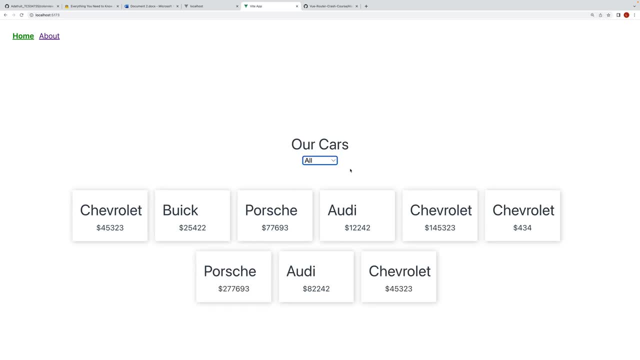 now we get porsche chevy, we get chevy, now we get porsche chevy, we get chevy audi, we get audi, and then all we get audi, we get audi, and then all we get audi, we get audi, and then all we get all. okay, so this is looking pretty good. 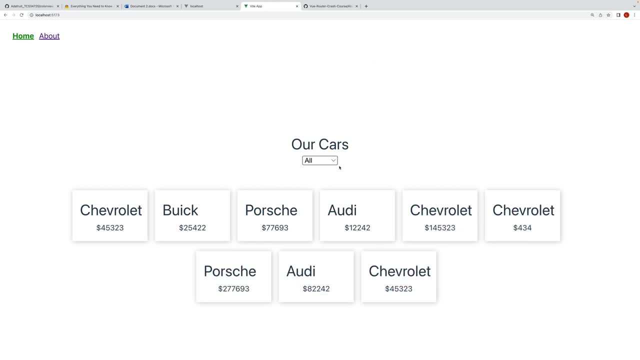 all okay, so this is looking pretty good. all okay, so this is looking pretty good. now let's say that you know i'm a spoiled. now let's say that you know i'm a spoiled. now let's say that you know i'm a spoiled kid and i want my dad to buy me a car. 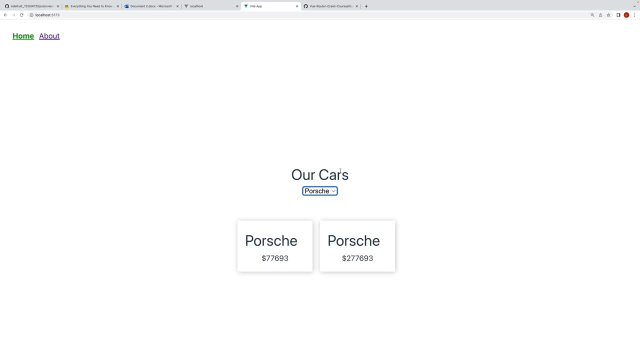 kid and i want my dad to buy me a car. kid, and i want my dad to buy me a car. and i'm very, very spoiled. i want the and i'm very, very spoiled. i want the and i'm very, very spoiled. i want the best of the best. i just want to. i want. 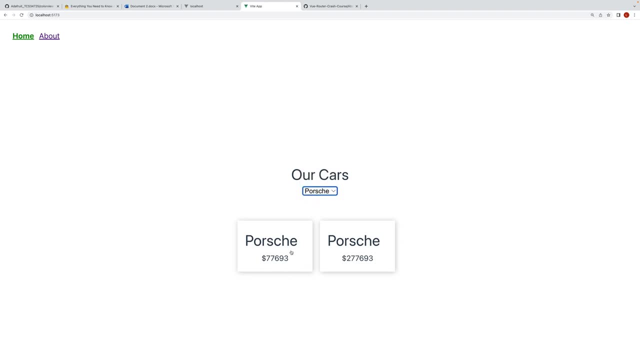 best of the best. i just want to. i want best of the best, i just want to. i want you know the porsches, so i go ahead and you know the porsches, so i go ahead and you know the porsches, so i go ahead and i filter for porsches and i say you. 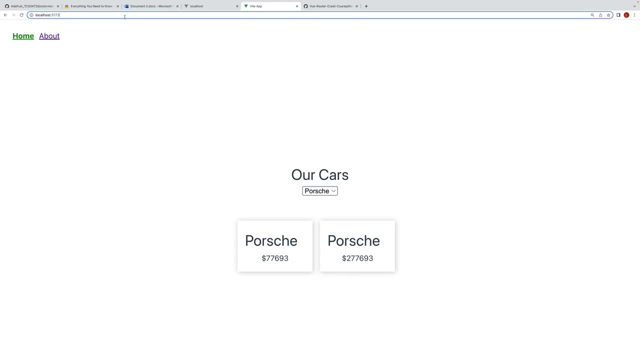 i filter for porsches and i say you, i filter for porsches. and i say you know what i'm happy with one of these? know what i'm happy with one of these? know what i'm happy with one of these two cars? i'm going to send this link to: 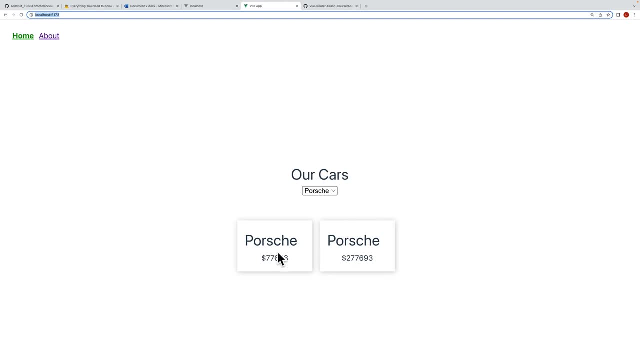 two cars. i'm going to send this link to two cars. i'm going to send this link to my dad. so this link over here to my dad, my dad, so this link over here to my dad, my dad, so this link over here to my dad. and just buy one of these two cars i. 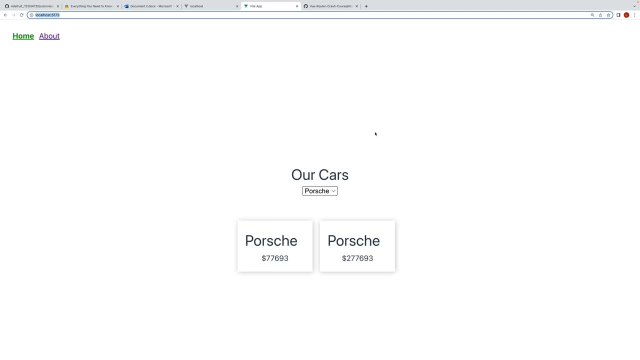 and just buy one of these two cars. i and just buy one of these two cars. i don't care, preferably this car over here, don't care, preferably this car over here, don't care, preferably this car over here. that's three hundred thousand dollars, that's three hundred thousand dollars. 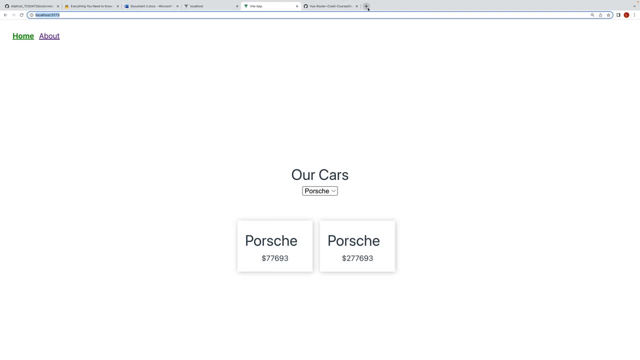 that's three hundred thousand dollars. so i copy the link and i send it to my. so i copy the link and i send it to my. so i copy the link and i send it to my dad. my dad then gets the link, and then dad. my dad then gets the link, and then. 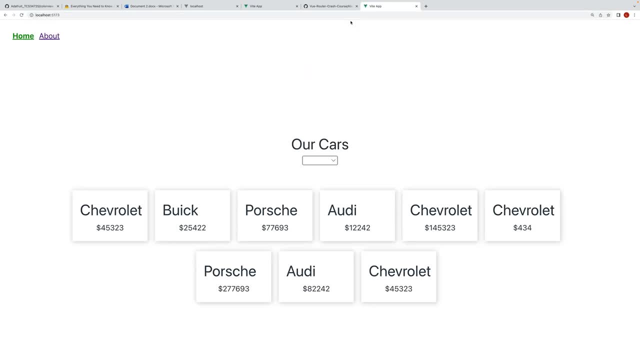 dad, my dad, then gets the link and then he pastes it, he pastes it, he pastes it, and then you can see here that well this, and then you can see here that well this, and then you can see here that well this. right here i get all of the filtering. 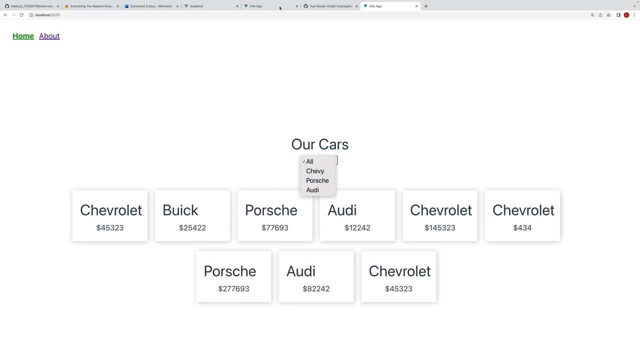 right here i get all of the filtering. right here i get all of the filtering options. so you can see it doesn't options. so you can see. it doesn't options. so you can see it doesn't default to the porsche, which is what i default to the porsche, which is what i. 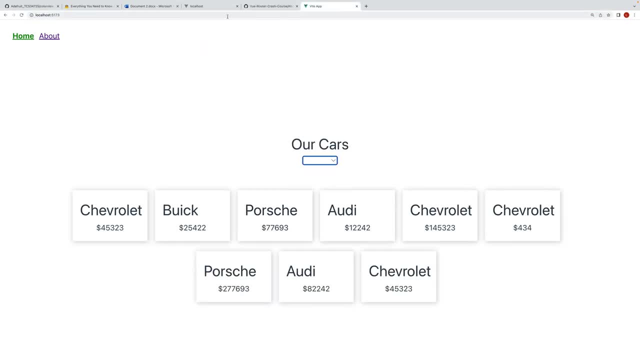 default to the porsche, which is what i had initially. so my dad is like, oh my, had initially. so my dad is like, oh my, had initially. so my dad is like, oh my, my kid. oh, he's not that spoiled anymore, kid. oh, he's not that spoiled anymore. 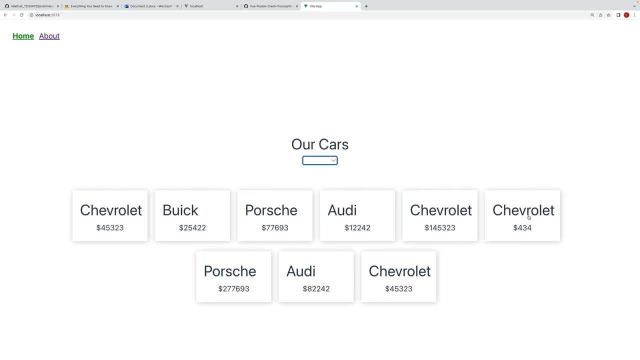 kid. oh, he's not that spoiled anymore. he doesn't. he doesn't want a nice car. i'm, he doesn't. he doesn't want a nice car. i'm, he doesn't. he doesn't want a nice car. i'm just gonna buy them this 400 and. 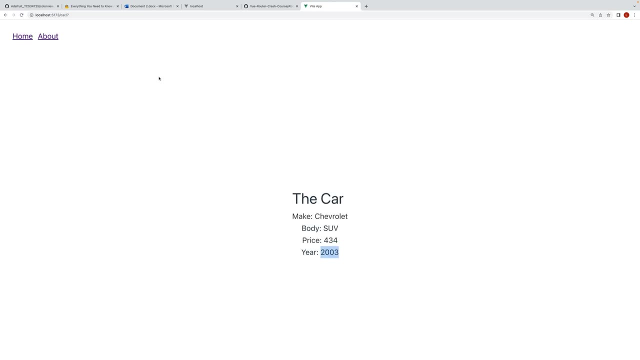 just gonna buy them this 400, and just gonna buy them this 400, and i'm gonna buy them this really old chevy. i'm gonna buy them this really old chevy. i'm gonna buy them this really old chevy. that's 2003, so so this is what i'm. 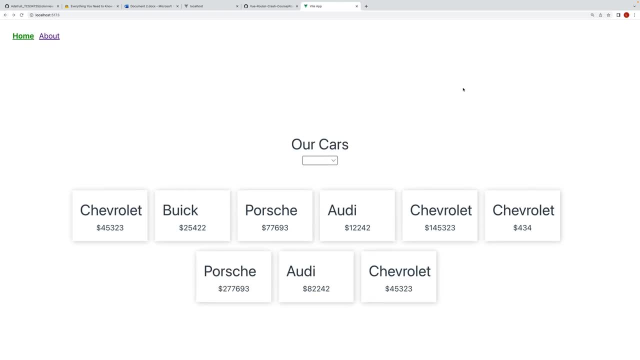 that's 2003. so so this is what i'm. that's 2003, so so this is what i'm gonna buy him because he doesn't care. he gonna buy him because he doesn't care. he gonna buy him because he doesn't care. he. he's a very, you know, nice kid, but in 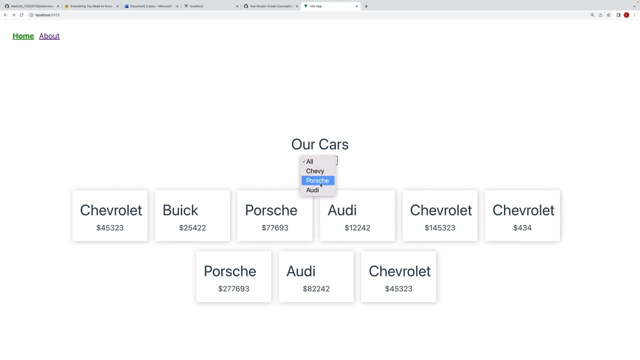 he's a very you know nice kid, but in he's a very you know nice kid, but in reality, you know, i i wanted the porsche reality. you know i i wanted the porsche reality. you know i i wanted the porsche, and that's because i went ahead and i. 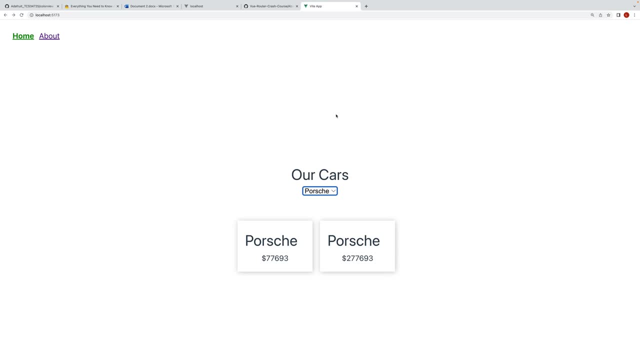 and that's because i went ahead and i, and that's because i went ahead and i filtered for this and i sent him the url filtered for this and i sent him the url filtered for this and i sent him the url, so you can see that this could cause. 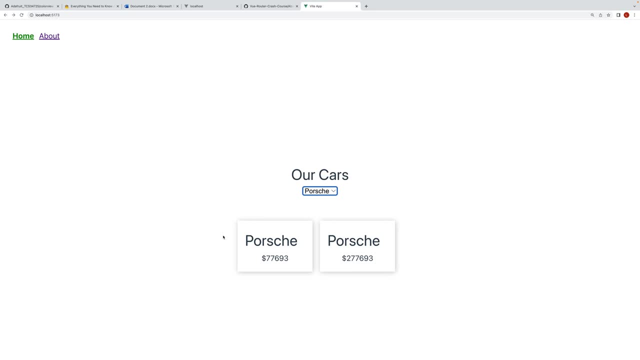 so you can see that this could cause. so you can see that this could cause some potential issues. so is there a way, some potential issues. so is there a way, some potential issues. so is there a way that we can actually somehow save this, that we can actually somehow save this? 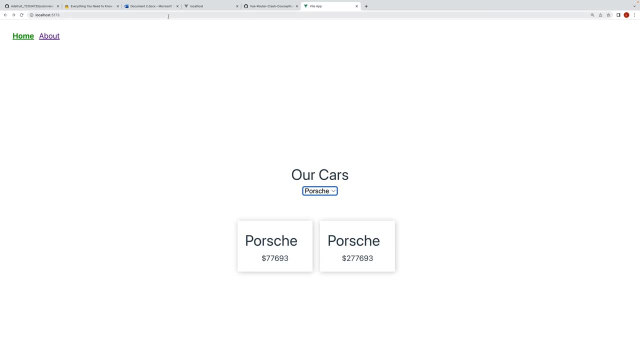 that we can actually somehow save this filter information inside of the url, filter information inside of the url filter information inside of the url itself itself itself, and we can actually do that with query and we can actually do that with query and we can actually do that with query parameters. 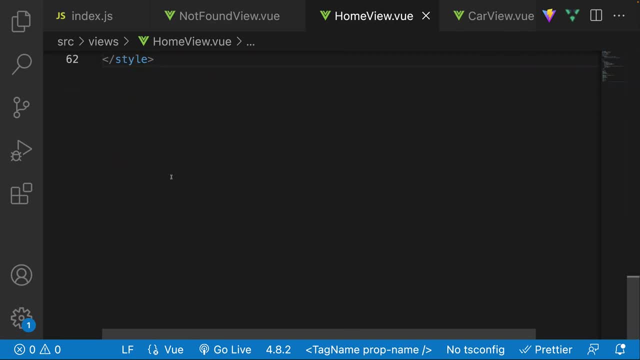 parameters, parameters. so if you're actually unfamiliar with, so, if you're actually unfamiliar with, so, if you're actually unfamiliar with query parameters: they're just parameters. query parameters, they're just parameters. query parameters, they're just parameters that we can add to our path, that we can add to our path. 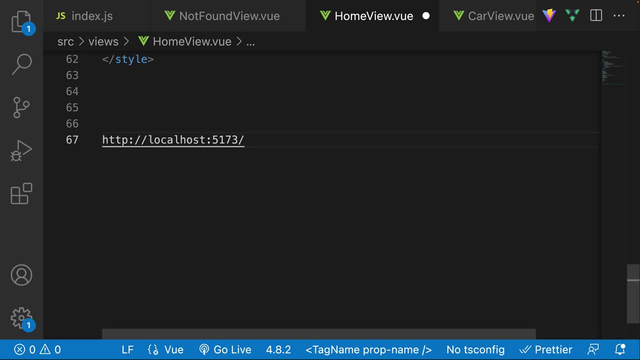 that we can add to our path. so right now we're on slash cars, or so right now we're on slash cars, or so right now we're on slash cars, or maybe we're on slash home, right? maybe we're on slash home, right, maybe we're on slash home, right. so what we can actually do is, instead of 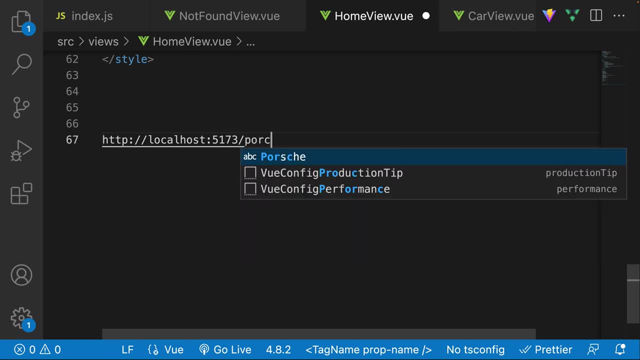 so what we can actually do is instead of. so what we can actually do is, instead of adding another path like the make is adding another path, like the make is adding another path, like the make is porsche, or whatever, what we can do is we porsche or whatever. what we can do is we. 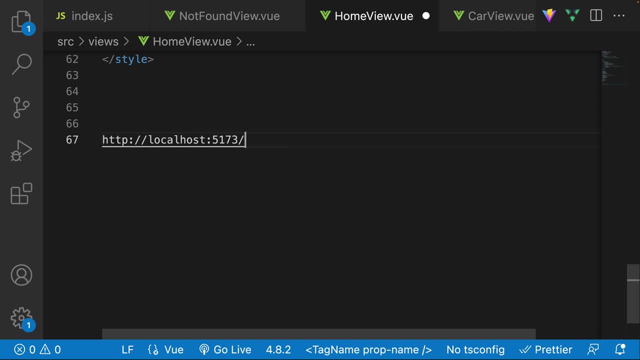 porsche or whatever. what we can do is: we can just append as many can just append as many can just append as many variables as well as their values keys, variables as well as their values keys, variables as well as their values, keys, and as well as their values as possible. 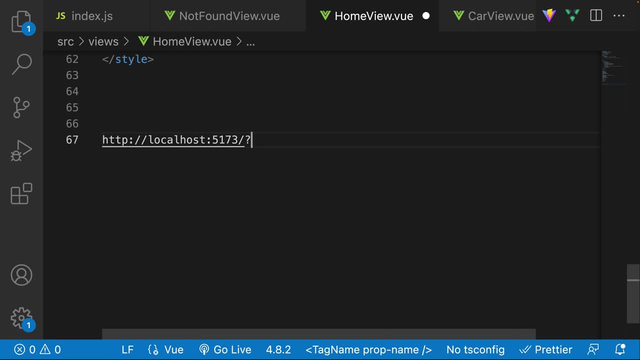 and as well as their values as possible, and as well as their values as possible to the path. and we do that very simply to the path, and we do that very simply to the path, and we do that very simply by adding a question mark and then over. 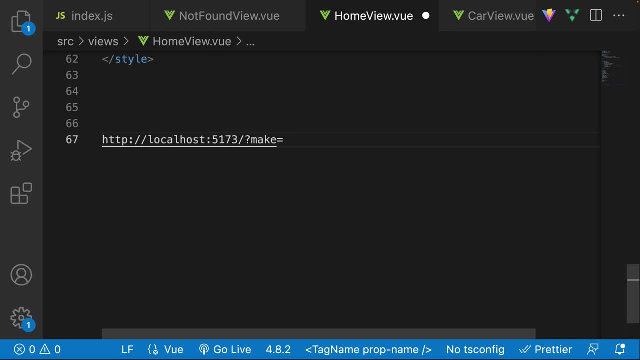 by adding a question mark, and then over by adding a question mark, and then over here we can say something like make, and here we can say something like make, and here we can say something like make, and then we can say that that is going to. then we can say that that is going to. 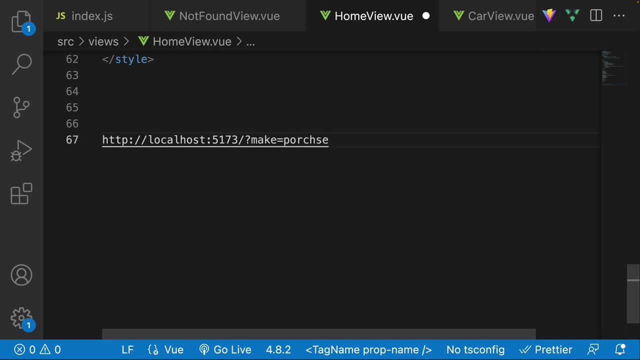 then we can say that that is going to be equal to porsche. and then if you want be equal to porsche, and then if you want be equal to porsche, and then if you want to add another thing, i can just say: to add another thing, i can just say: 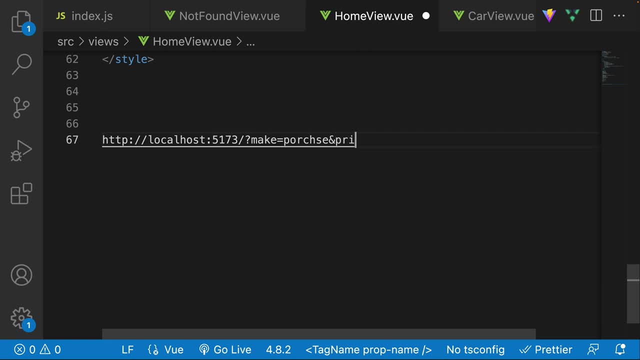 to add another thing. i can just say: you know price is equal to, or maybe you know price is equal to, or maybe you know price is equal to, or maybe maybe something like min price, maybe something like min price, maybe something like min price, and then that is going to be equal to i. 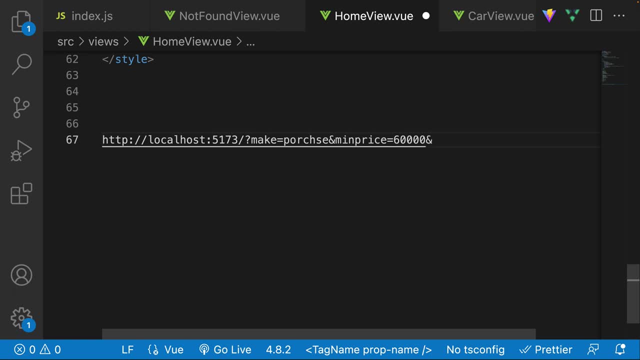 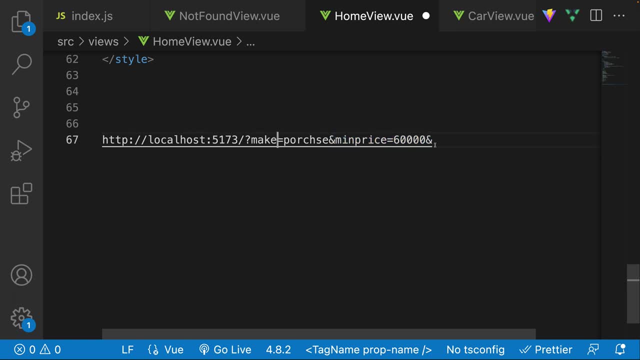 think of them as variables, that we are appending to our, that, we are appending to our, that, we are appending to our url, and so this is actually the best url, and so this is actually the best url, and so this is actually the best thing that we can do. so what i want to 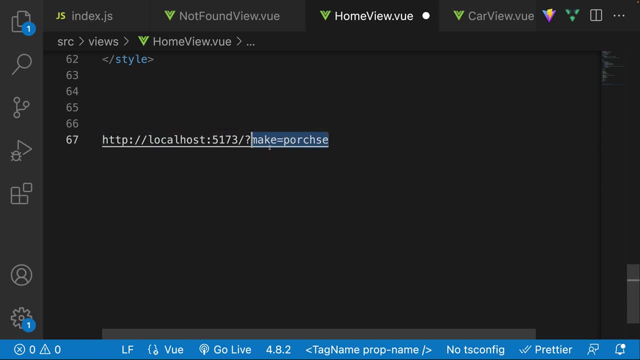 thing that we can do. so what i want to thing that we can do, so what i want to do is: i want to add do is. i want to add do is. i want to add a query parameter where the make is, a query parameter where the make is. 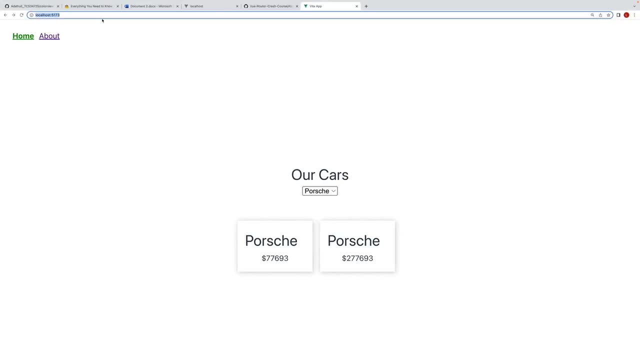 a query parameter where the make is equal to porsche, and that way, when they equal to porsche, and that way, when they equal to porsche, and that way when they go ahead and actually copy this, then go ahead and actually copy this, then go ahead and actually copy this, then we're going to go ahead and actually 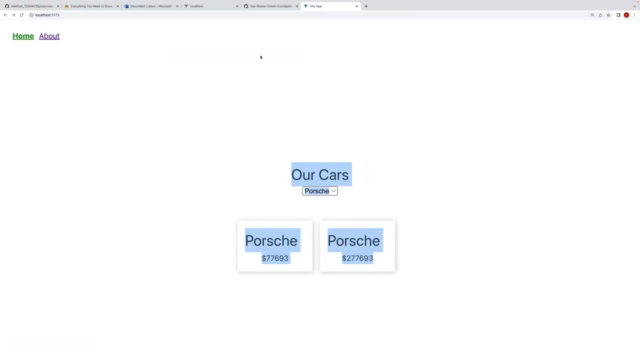 we're going to go ahead and actually we're going to go ahead and actually update. they're going to see exactly that update. they're going to see exactly that update. they're going to see exactly that. hey, this is the porsche that we want this. hey, this is the porsche that we want this. 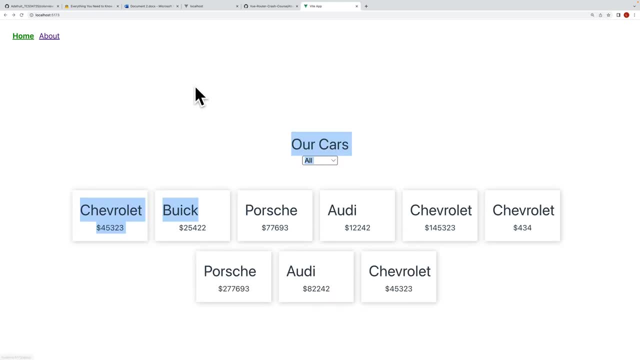 hey, this is the porsche that we want. this is the. this is the type of cars that is the. this is the type of cars that is the. this is the type of cars that we want. i hope that makes sense, so let's we want. i hope that makes sense, so let's. 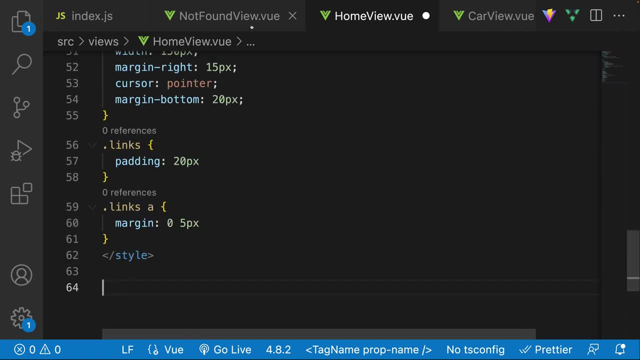 we want. i hope that makes sense. so let's go ahead and actually add this query. go ahead and actually add this query. go ahead and actually add this query parameter any time that we make this parameter, any time that we make this parameter, any time that we make this particular change. 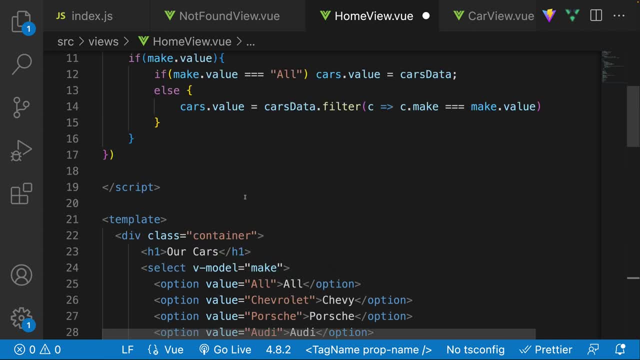 particular change, particular change. so let's go over here and what we're. so let's go over here and what we're. so let's go over here and what we're going to do is we're going to add a. going to do is we're going to add a. 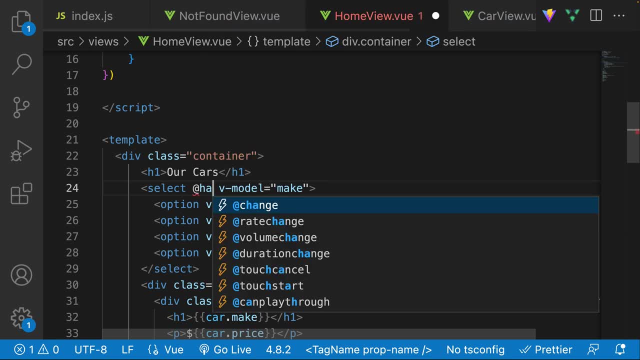 going to do is we're going to add a handle change, handle change, handle change. so we're going to say at handle. so we're going to say at handle. so we're going to say at handle change. so handle change or sorry. this is change. so handle change or sorry. this is. 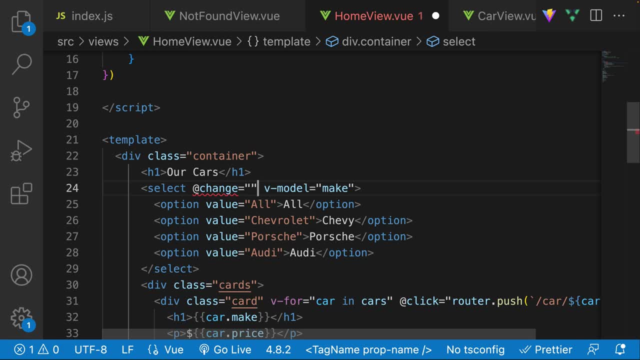 change, so handle change, or sorry, this is going to be going to be going to be at change and we're going to call a at change and we're going to call a at change and we're going to call a handle change, function, handle change, function, handle, change function. so handle change, like so. so i'm going 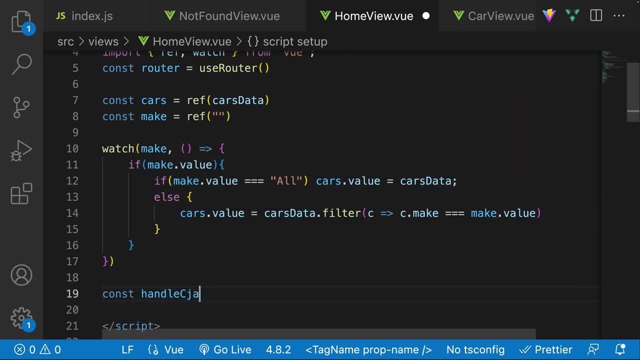 so handle change like so. so i'm going so handle change like so. so i'm going to go ahead and to go ahead and to go ahead and create this function called handle change, create this function called handle change, create this function called handle change, and this function all it is going to do. 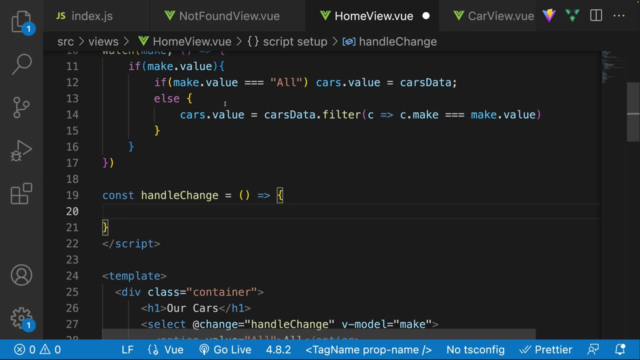 and this function. all it is going to do and this function. all it is going to do is just grab the make and add a query. is just grab the make and add a query. is just grab the make and add a query parameter to our path, parameter to our path. 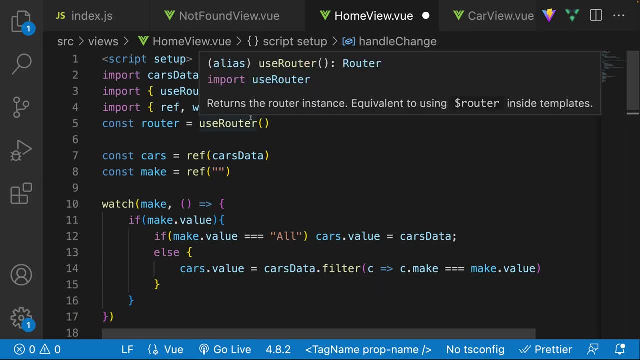 parameter to our path. so let's go over here. and in order to so, let's go over here. and in order to so, let's go over here, and in order to actually actually actually mutate our query parameters, let's mutate our query parameters. let's mutate our query parameters. let's remember we're going to need to utilize 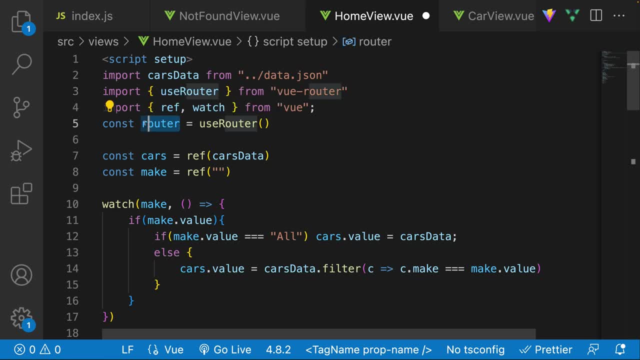 remember we're going to need to utilize. remember we're going to need to utilize the use router, so not use route. use the use router, so not use route. use the use router, so not use route use router. and luckily we already have our router and luckily we already have our. 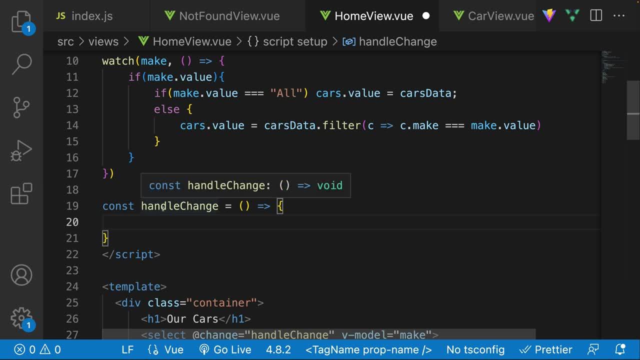 router and luckily we already have our router, router, router. so very simply, what we can actually do, so very simply, what we can actually do, so very simply, what we can actually do here is actually here, is actually here, is actually push a query parameter so we can say: 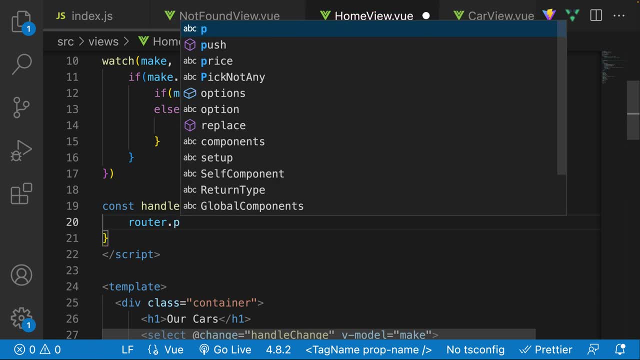 push a query parameter, so we can say: push a query parameter, so we can say router, and then i can say router, and then i can say router, and then i can say dot, push, dot, push, dot, push, and over here i can go ahead and actually, and over here i can go ahead and actually. 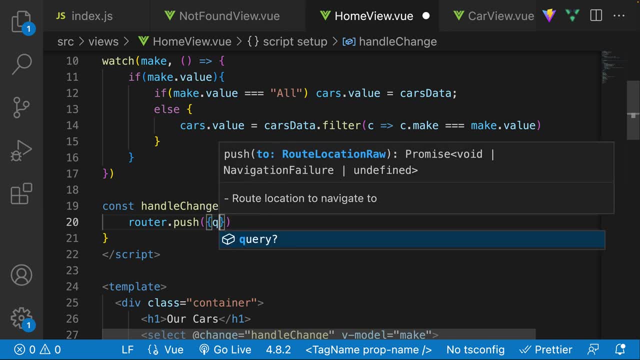 and over here, i can go ahead and actually invoke this, invoke this, invoke this, and instead of passing in a path, i'm, and instead of passing in a path, i'm, and instead of passing in a path, i'm going to pass in an object. going to pass in an object. 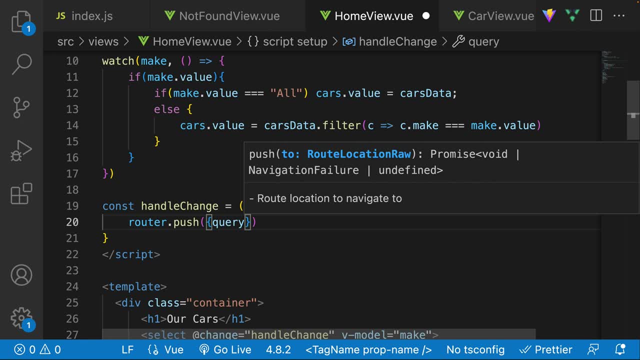 going to pass in an object where we have a query, and then i'm going where we have a query, and then i'm going where we have a query and then i'm going to define, to define, to define all of the different key value pairs. so all of the different key value pairs, so 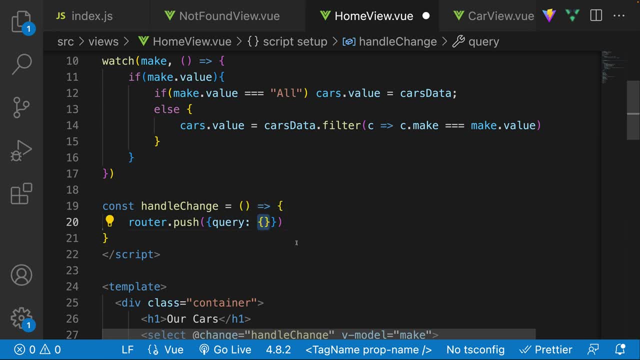 all of the different key value pairs. so, remember we can have as many query, remember we can have as many query. remember we can have as many query parameters as possible. we can add them parameters as possible. we can add them parameters as possible. we can add them inside of this object. 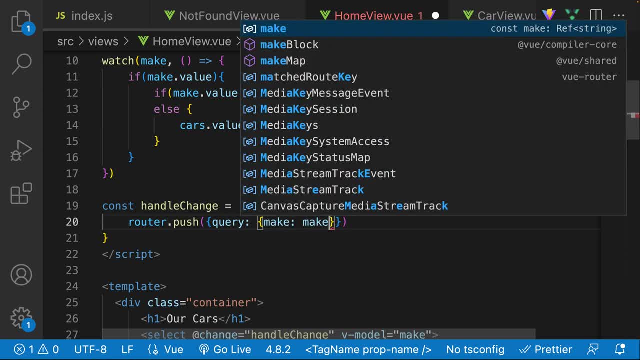 inside of this object, inside of this object now, i only want to add one which is going now. i only want to add one which is going now. i only want to add one which is going to be the make to be, the make to be, the make. i'm going to say this is going to be the. 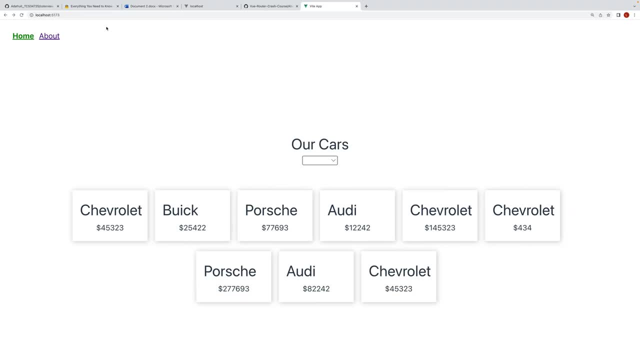 i'm going to say this is going to be the. i'm going to say this is going to be the: make dot value, make dot value, make dot value. so now, if i were to, i'm going to go. so now, if i were to, i'm going to go. 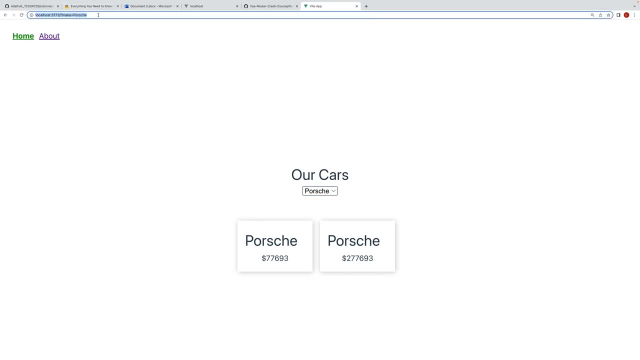 so now, if i were to, i'm going to go ahead and go to ahead, and go to ahead and go to porsche and i were to save this. you can, porsche, and i were to save this. you can, porsche, and i were to save this. you can see here. 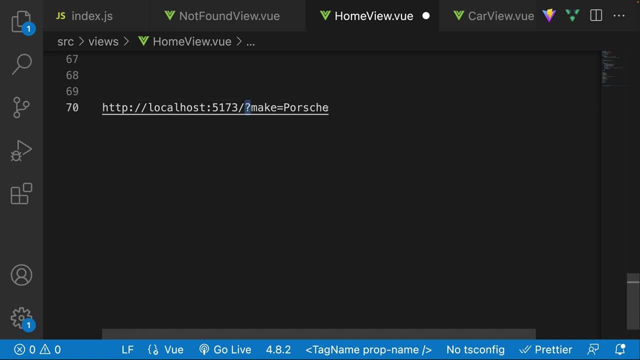 see here, see here that this is how my path looks like. so that this is how my path looks like. so that this is how my path looks like. so it's going to be like. it's going to be like. it's going to be like slash make, slash, porsche, but again, i 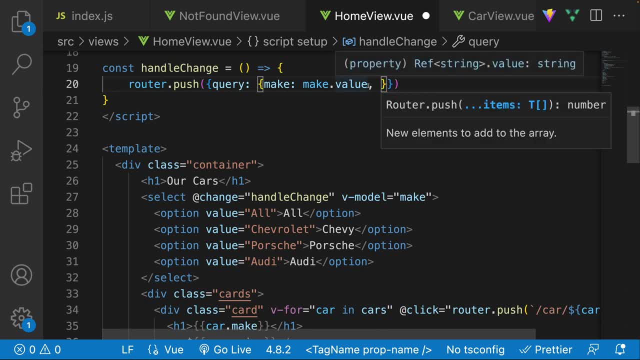 slash, make slash porsche. but again i slash, make slash porsche. but again i could have just as easily added more so could have just as easily added more so could have just as easily added more so so i could have added, so i could have added, so i could have added: you know, banana is equal to yellow, or? 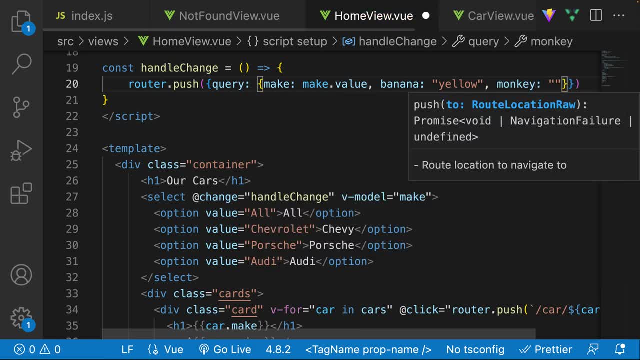 you know banana is equal to yellow, or you know banana is equal to yellow, or um monkey is equal to um monkey is equal to um monkey is equal to um banana. i don't know something like um banana. i don't know something like um banana. i don't know something like that. so i could have just as easily. that, so i could have just as easily that, so i could have just as easily added more. and now this time if i were added more, and now this time, if i were added more, and now this time if i were to click on this, to click on this. 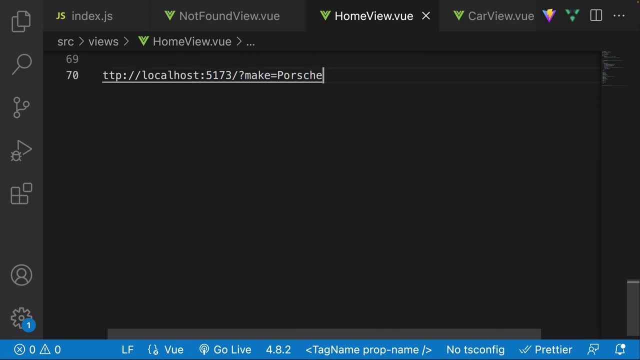 to click on this. you can see that this is how the query. you can see that. this is how the query. you can see that this is how the query parameters look like. parameters look like parameters look like: so something like that now, of course. so something like that, now, of course. so something like that. now, of course, this doesn't really make much sense to this, doesn't really make much sense to this, doesn't really make much sense to me, so we're just going to kind of stick me. so we're just going to kind of stick. 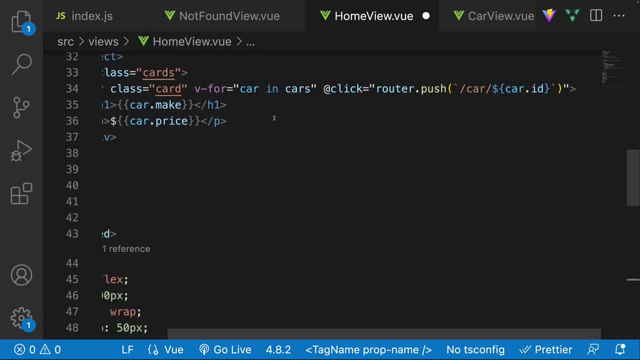 me. so we're just going to kind of stick with what we have over here, with what we have over here, with what we have over here. okay, so, let us let me just remove this. okay, so, let us let me just remove this. okay, so, let us let me just remove this. i'm going to remove that for now. i'm going to remove that for now. i'm going to remove that for now. and there we go, nice and saved, okay, so, and there we go, nice and saved, okay so, and there we go, nice and saved, okay, so now we have added. now we have added. 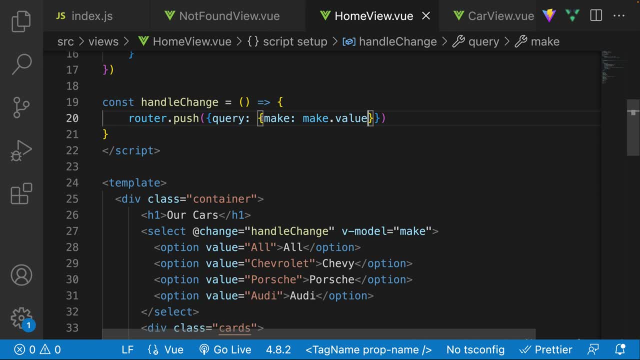 now, we have added this query parameter. so now this query parameter, so now this query parameter. so now, what is the next step? well, the next step. what is the next step? well, the next step. what is the next step? well, the next step is as soon as this component mounts. 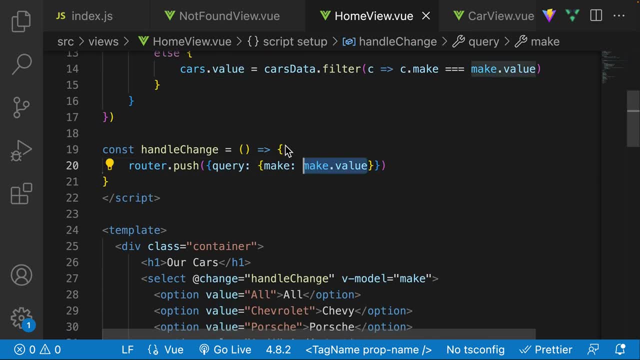 is as soon as this component mounts, is as soon as this component mounts. what i want to do is i want to grab the. what i want to do is i want to grab the. what i want to do is i want to grab the query parameter if we have it in there. query parameter if we have it in there and if we do have it in there, such as if and if we do have it in there, such as if and if we do have it in there, such as if it's a porsche, it's a porsche. 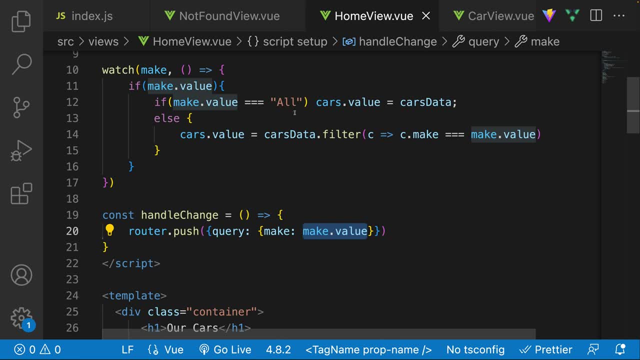 it's a porsche. that i want to do is just i want to. that i want to do is just i want to. that i want to do is just i want to, right away, just kind of filter for what. right away, just kind of filter for what. 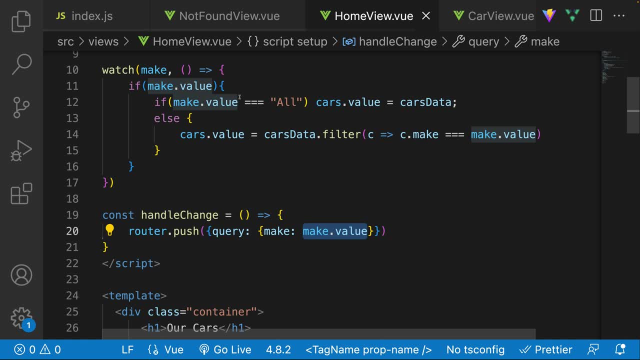 right away, just kind of filter for what we have. we have, we have. so i want to go ahead and grab the query. so i want to go ahead and grab the query. so i want to go ahead and grab the query, parameter, parameter parameter, and then i'm going to go ahead and assign. 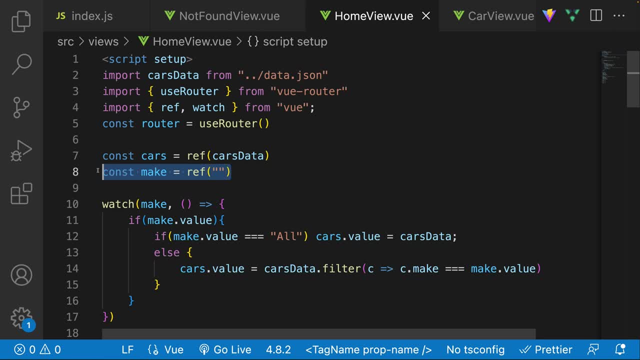 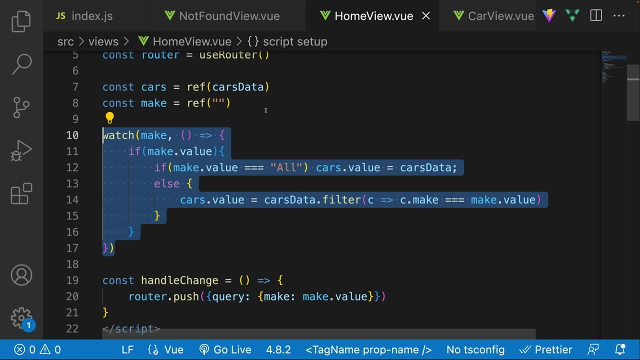 and then i'm going to go ahead and assign, and then i'm going to go ahead and assign it to it, to it to: if we have a value inside of our query, if we have a value inside of our query, if we have a value inside of our query parameter. 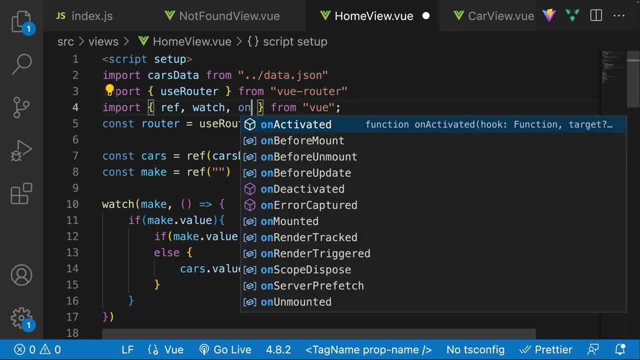 parameter parameter. so i'm going to go over here and i'm so i'm going to go over here and i'm so i'm going to go over here and i'm going to call a on going to call a on going to call a on mounted and let's go over. 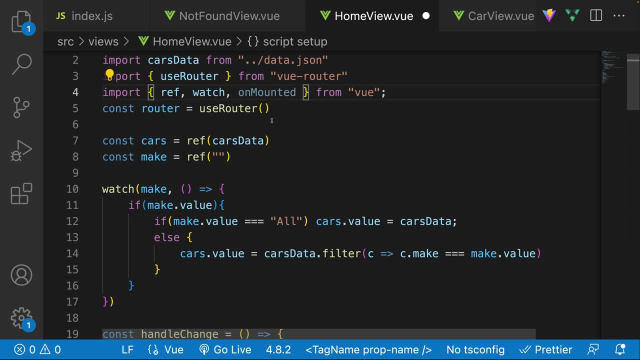 mounted and let's go over mounted and let's go over here and we're going to call this here and we're going to call this here and we're going to call this, let's just call it. let's just call it, let's just call it right here. so we're going to say on. 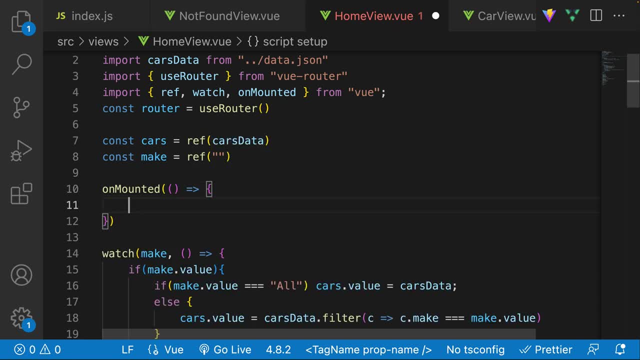 right here. so we're going to say on, right here, so we're going to say on mounted, mounted, mounted, and i want to basically call this and i and i want to grab whatever values in, and i want to grab whatever values in and i want to grab whatever values in the query parameter and update it to. 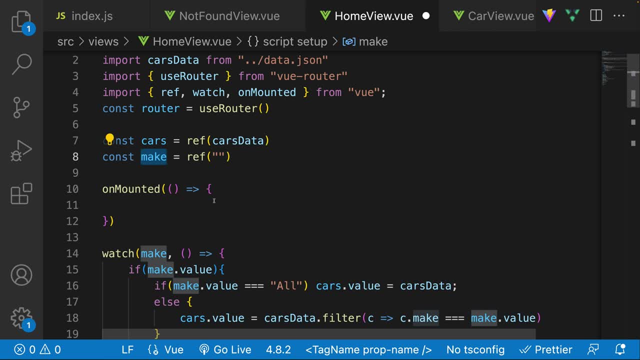 the query parameter and update it to the query parameter and update it to our state now. this presents a little bit our state now. this presents a little bit our state now. this presents a little bit of an issue. how are we going to get of an issue? how are we going to get? 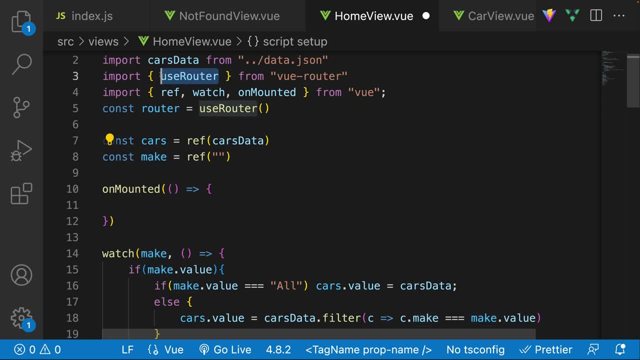 of an issue: how are we going to get access to the query parameter? access to the query parameter, access to the query parameter? well, you guessed it, instead of using. well, you guessed it, instead of using. well, you guessed it, instead of using use router, we're going to use use route. 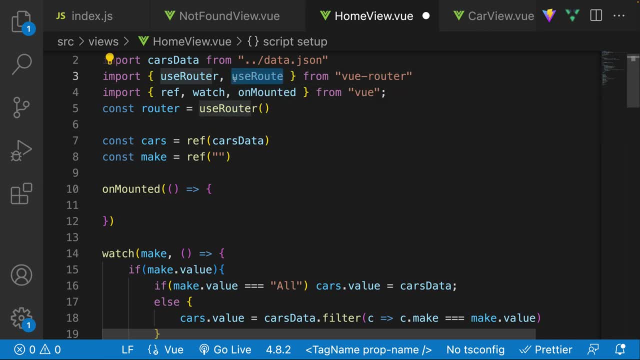 use router, we're going to use use route. use router, we're going to use use route. so anytime you want to get information, so anytime you want to get information. so anytime you want to get information about our particular uh path, our, about our particular uh path, our. 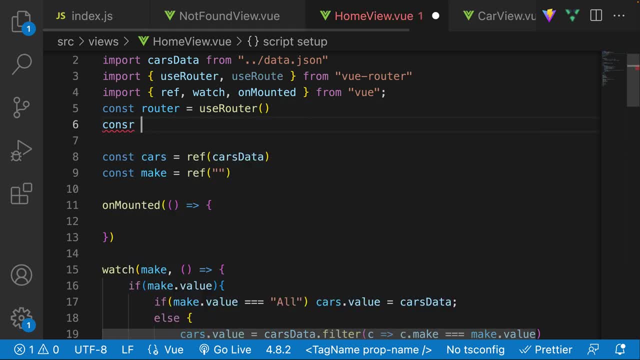 about our particular uh path, our particular route. we're going to use the particular route. we're going to use the particular route. we're going to use the use route composable. so we're going to use route composable. so we're going to use route composable, so we're going to say const. 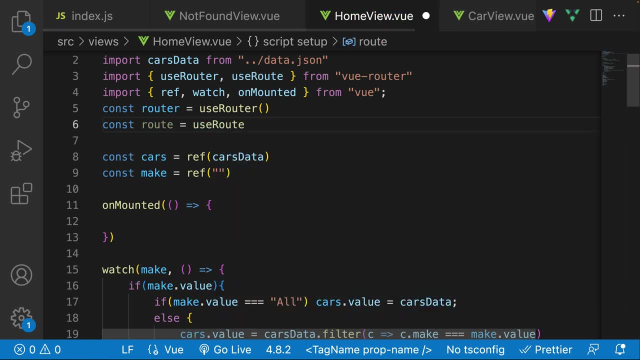 say const, say const, use route. we're going to say equal to use route. we're going to say equal to use route. we're going to say equal to use route and we're going to go ahead: use route. and we're going to go ahead: use route. and we're going to go ahead and invoke it and then, over here, now, if 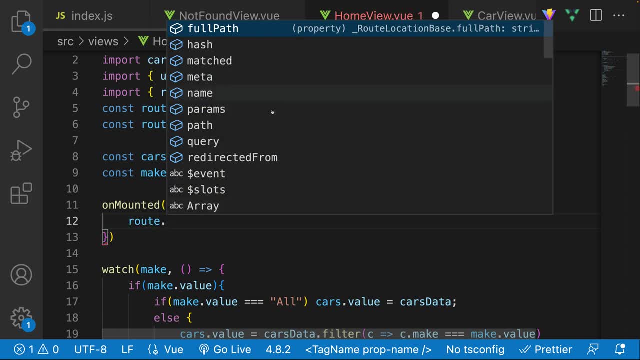 and invoke it. and then over here now, if and invoke it, and then over here now, if i were to say route, i were to say route, i were to say route, route dot. you can see, here we actually route dot. you can see, here, we actually route dot. you can see, here we actually can get the query parameters by. 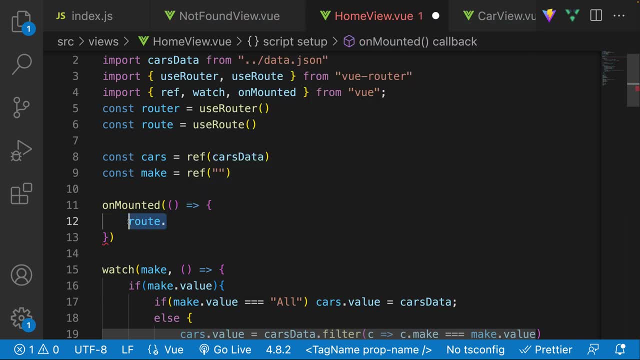 can get the query parameters by. can get the query parameters by utilizing: utilizing- utilizing- query right over here. so what i'm going query right over here, so what i'm going query right over here. so what i'm going to do now is i'm going to very simply, 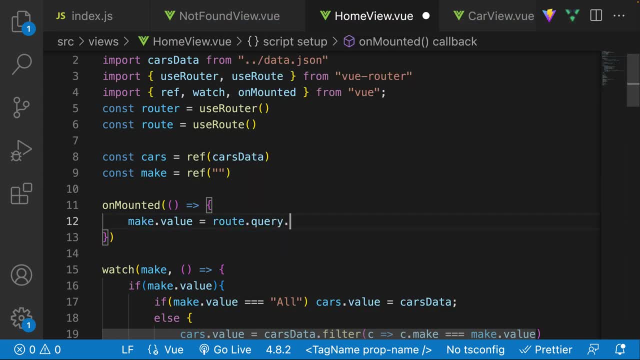 to do now is i'm going to very simply to do. now is i'm going to very simply say: say, say, make dot value is equal to route dot. make dot value is equal to route dot. make dot value is equal to route dot. query, query, query, and then dot, uh, and then this is going. 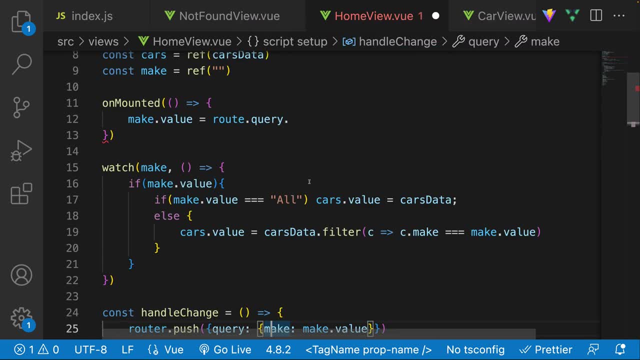 and then dot uh, and then this is going and then dot uh and then this is going to be to be: to be uh called whatever key value. we uh called whatever key value, we uh called whatever key value. we provided which is going to be make, provided which is going to be make. 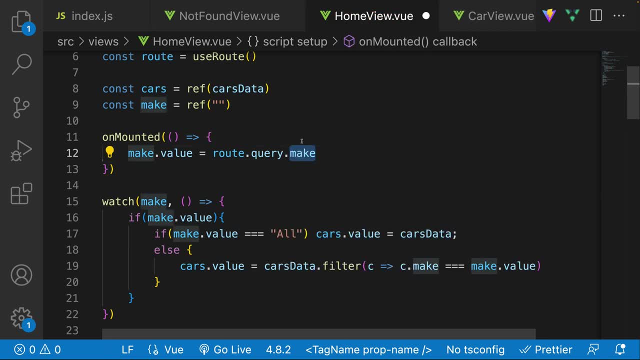 provided, which is going to be make now. if it's not there, it's just going now. if it's not there, it's just going now. if it's not there, it's just going to be to be to be completely empty. however, if it is there, completely empty. however, if it is there, 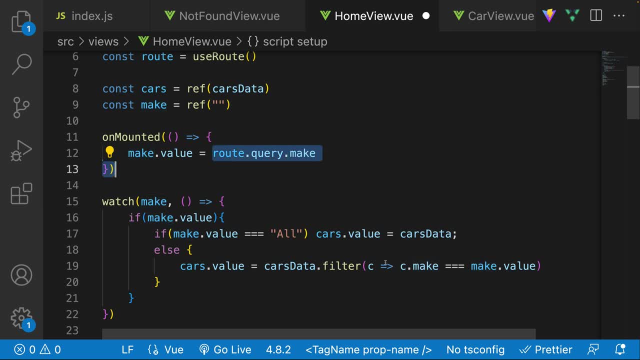 completely empty. however, if it is there, then then then you know it'll, it'll show it'll be, you know it'll, it'll show it'll be, you know it'll, it'll show it'll be. whatever it is that we have it in, whatever it is that we have it in, 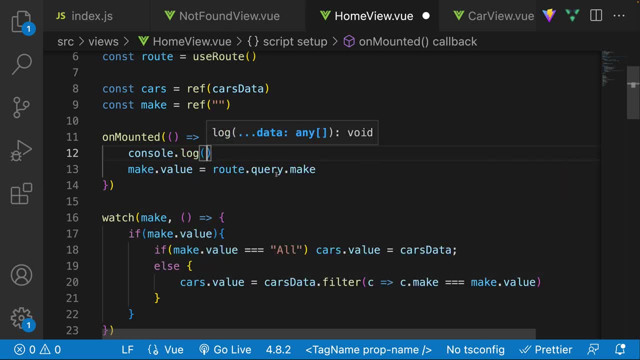 whatever it is that we have it in. so let me just quickly consolelog. so let me just quickly consolelog. so let me just quickly consolelog the route query, just uh, the route query, just uh, the route query, just uh. prove this to you. so right now i'm. 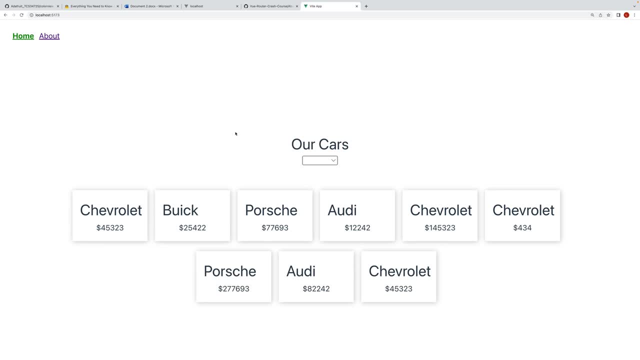 prove this to you. so, right now, i'm prove this to you. so right now, i'm going to go home, going to go home, going to go home. so let's go home. and now, if i were to, so let's go home. and now, if i were to, 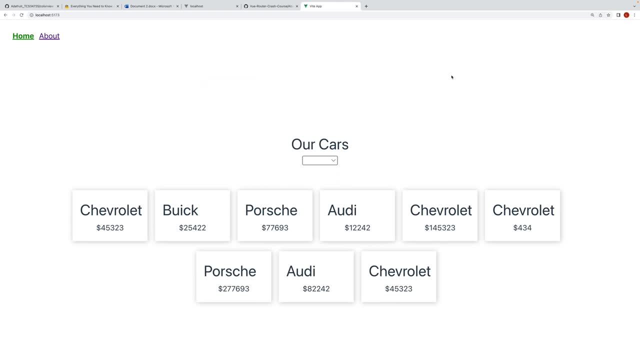 so let's go home. and now, if i were to, let's just quickly inspect here. let's just quickly inspect here. let's just quickly inspect here. just look at the console so you can see. just look at the console so you can see. just look at the console so you can see. it is an object here and there is. 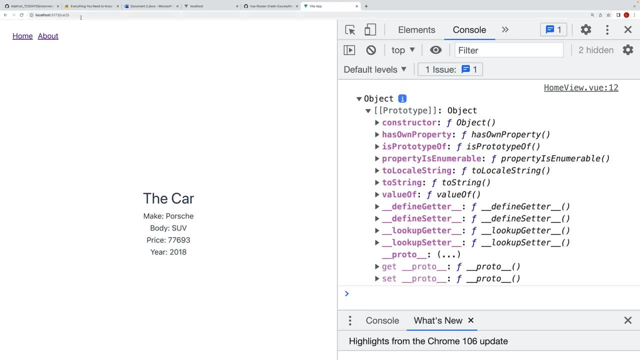 it is an object here and there is. it is an object here and there is nothing in there. so now if i were to nothing in there, so now if i were to nothing in there, so now if i were to click on, click on, click on, let's say, let's go back here and let's. 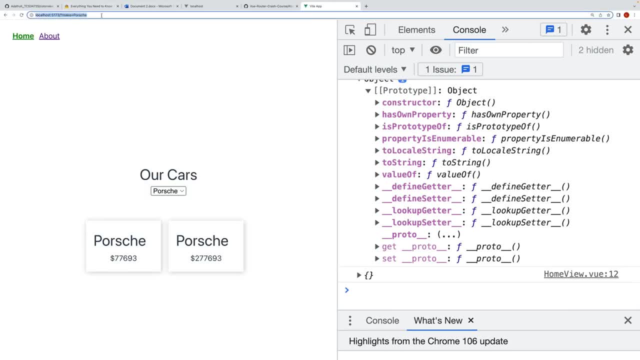 let's say: let's go back here and let's: let's go to porsche. so now you can see we have go to porsche. so now you can see we have go to porsche. so now you can see we have a query parameter, a query parameter. 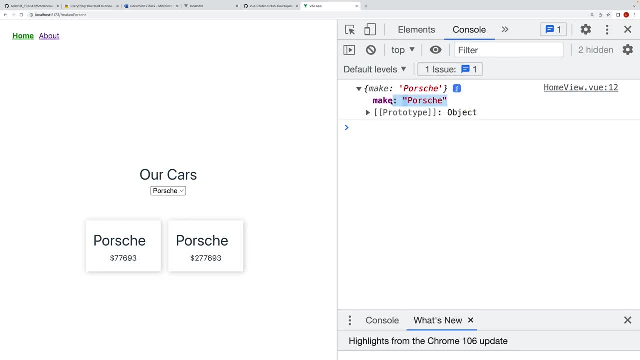 a query parameter and i'm going to see that now we have a and i'm going to see that now we have a and i'm going to see that now we have a, make, make, make of porsche. so also what we can do here is of porsche. so also what we can do here is. 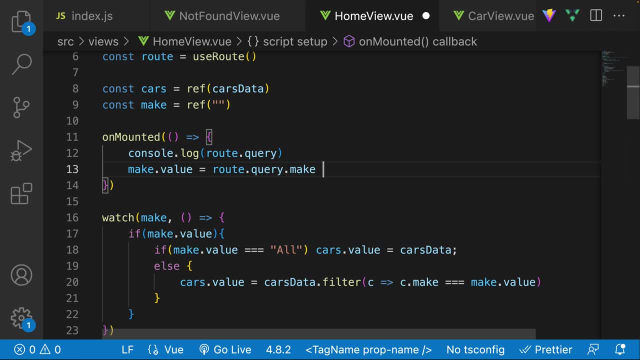 of porsche. so also, what we can do here is very simply just check if we have a make. very simply just check if we have a make. very simply just check if we have a make, so we can say something like that or an. so we can say something like that or an. 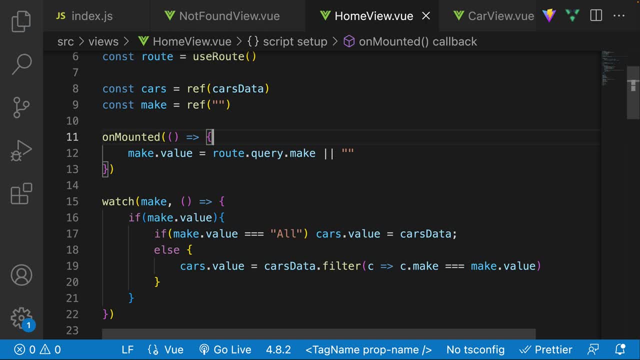 so we can say something like that: or an empty string, something like that empty string, something like that empty string, something like that. all right, so that's pretty much all it is all right. so that's pretty much all it is all right. so that's pretty much all it is that we need to do so now. 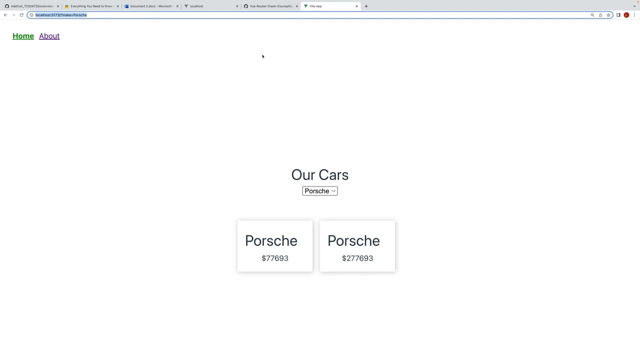 that we need to do so now that we need to do so now. the spoiled kid can actually copy this. the spoiled kid can actually copy this. the spoiled kid can actually copy this url and then we can give it to the dad url and then we can give it to the dad. 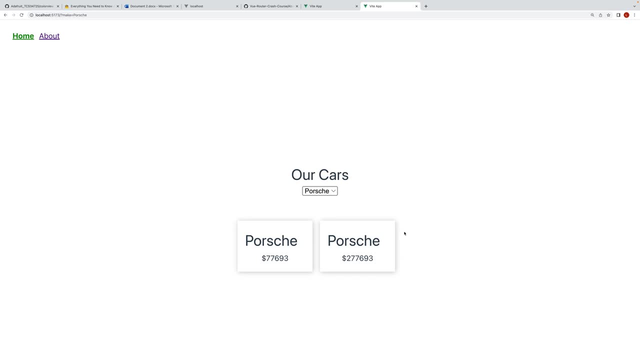 url and then we can give it to the dad and the dad can have exact access to it and the dad can have exact access to it. and the dad can have exact access to it. then he's like, oh crap, come on now i. then he's like, oh crap, come on now i. 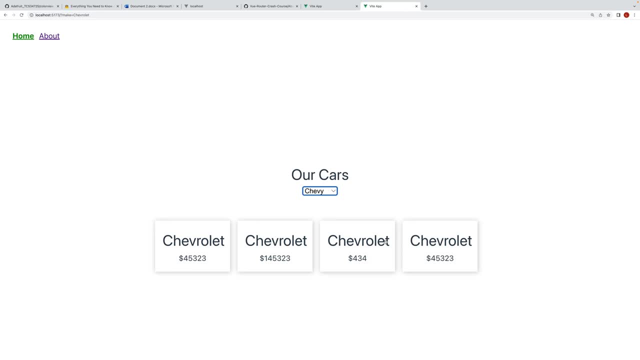 then he's like: oh crap, come on now. i gotta go buy him a porsche, oh that sucks. gotta go buy him a porsche, oh that sucks. gotta go buy him a porsche, oh that sucks, i'm gonna then. then then the dad is, i'm gonna then. then. then the dad is. 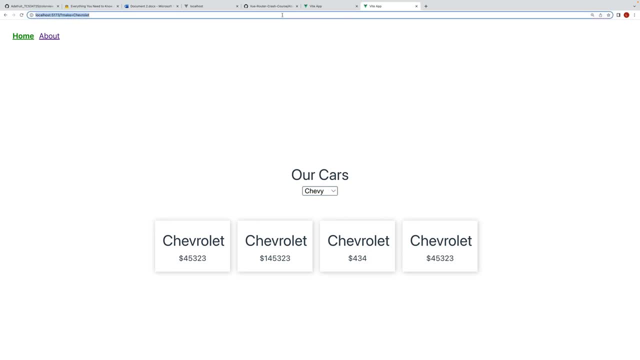 i'm gonna then, then, then the dad is gonna be like, gonna be, like, gonna be like. hey, what if i buy you one of these cars? hey, what if i buy you one of these cars? hey, what if i buy you one of these cars? and he's gonna copy this url. 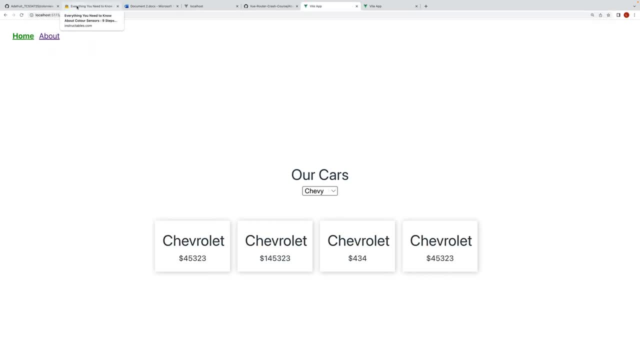 and he's gonna copy this url. and he's gonna copy this url, then the kid's gonna get it, and then then the kid's gonna get it, and then then the kid's gonna get it, and then he's gonna go ahead and paste it, and he's gonna go ahead and paste it, and. 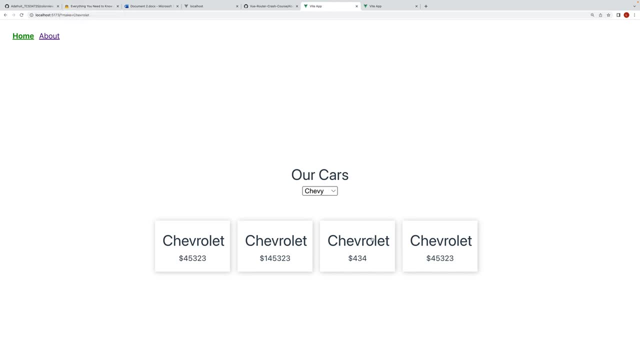 he's gonna go ahead and paste it and he's be like he's be like. he's be like dad, stop being such a prick. i don't want dad stop being such a prick. i don't want dad stop being such a prick. i don't want a car like this. give me a porsche, you. 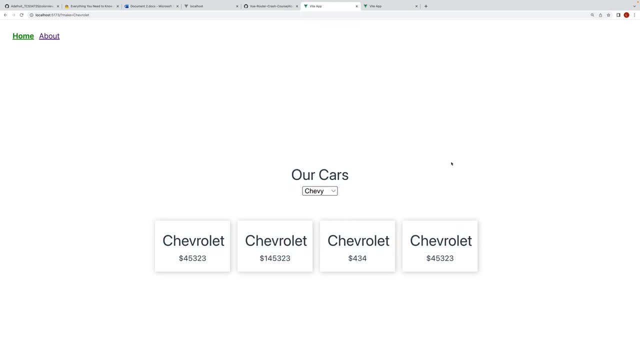 a car like this: give me a porsche you. a car like this: give me a porsche, you guys get the point, guys get the point, guys get the point. okay, so that's, uh, that's pretty much it. okay, so that's, uh, that's pretty much it. 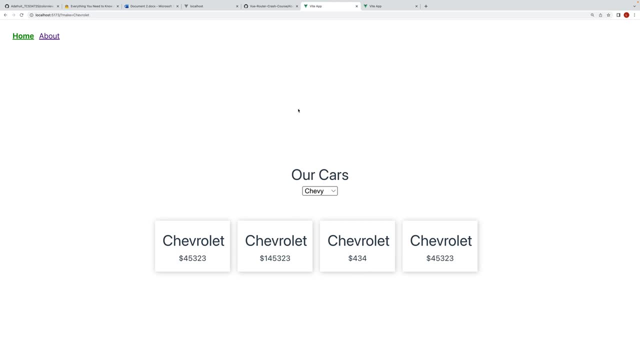 okay, so that's uh, that's pretty much it. that's kind of one of the more advanced, that's kind of one of the more advanced. that's kind of one of the more advanced: uh features, uh features, uh features. so another thing that i want to talk: 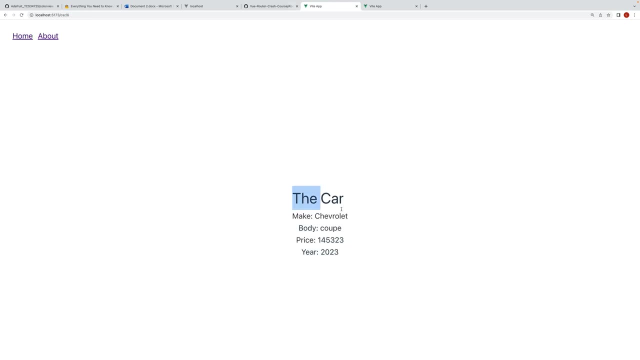 so another thing that i want to talk, so another thing that i want to talk about about, about is nested routes. so let's go over: here is nested routes. so let's go over: here is nested routes. so let's go over here, to this uh page right over here. 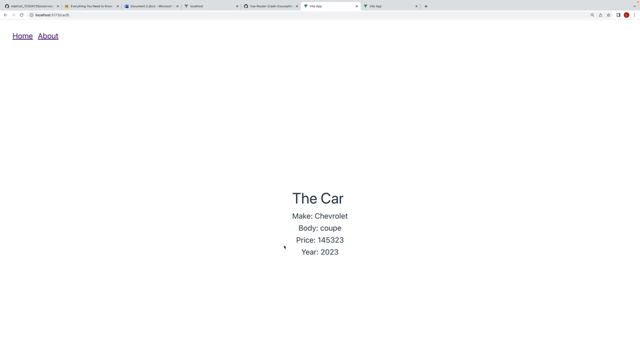 to this uh page right over here, to this uh page right over here, and let's say we also want. so let's say, and let's say we also want. so let's say, and let's say we also want. so let's say someone's interested in a particular car. 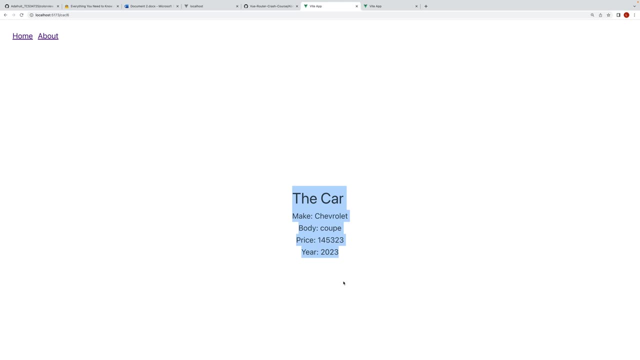 someone's interested in a particular car. someone's interested in a particular car, and if they're interested in a car, what? and if they're interested in a car, what? and if they're interested in a car, what we want to do, we want to do, we want to do is we want to um. 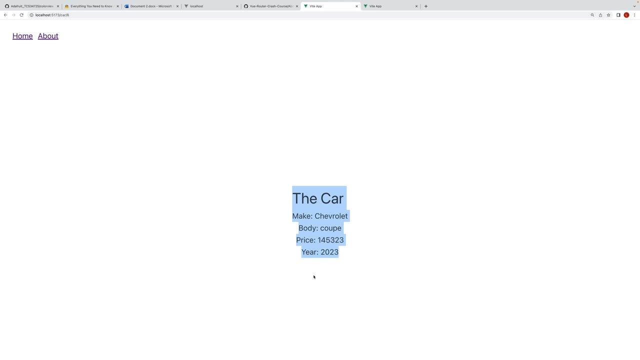 is we want to um is we want to um. you know, you know, you know, have them click a button to either have them click a button to either have them click a button to either contact a dealer or contact the contact a dealer, or contact the contact a dealer or contact the manufacturer. you know they can call. 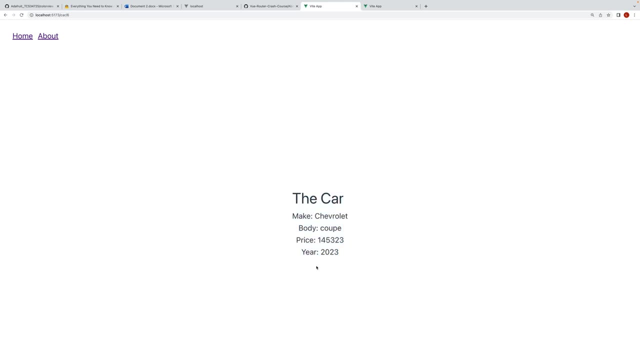 manufacturer. you know they can call manufacturer. you know they can call contact either or contact either, or contact either or so. however, what we want to do is we want so. however, what we want to do is we want so. however, what we want to do is we want to render this component right below. 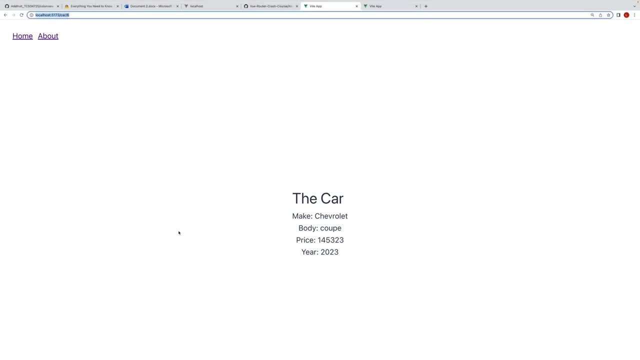 to render this component right below, to render this component right below here. but we only want to render this here. but we only want to render this here. but we only want to render this component if you hit a specific path component. if you hit a specific path component, if you hit a specific path. so, for example, 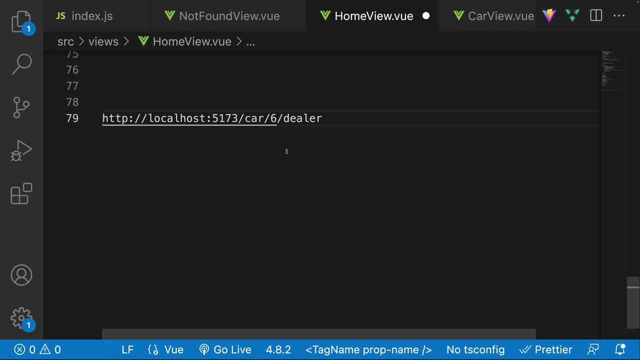 so for example. so, for example, let's say over here, let's say: if you go, let's say over here. let's say, if you go, let's say over here, let's say, if you go to slash dealer, then right on this page. to slash dealer, then right on this page. 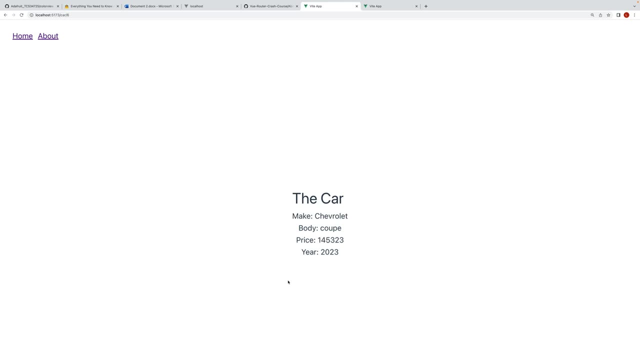 to slash dealer, then right on this page, not on the home page on this page. right, not on the home page on this page. right, not on the home page on this page. right below this, right over here. we want to. below this, right over here, we want to. 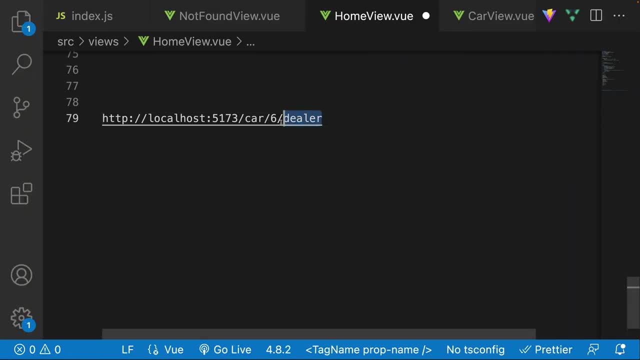 below this, right over here, we want to render the dealer's information, render the dealer's information, render the dealer's information. but if you go to slash, but if you go to slash, but if you go to slash- manufacturer, manufacturer, manufacturer, something like that- then again right on. 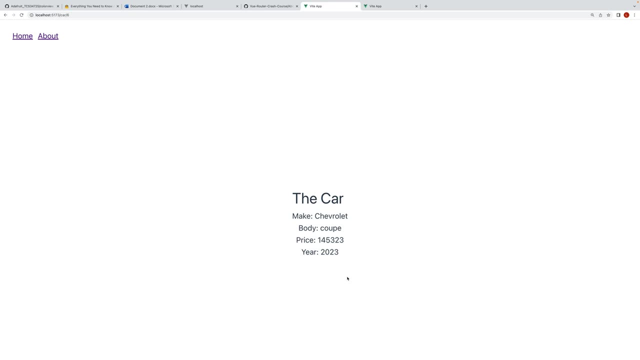 something like that, then again right on something like that, then again right on this page. i want to render the this page, i want to render the this page. i want to render the manufacturer's uh uh application. manufacturer's uh uh application. manufacturer's uh uh application information. so i want to render a. 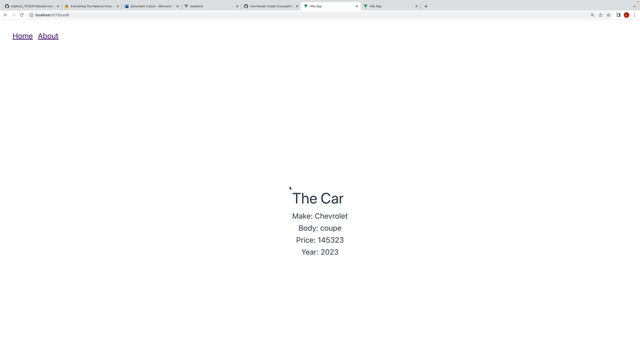 information. so i want to render a information, so i want to render a different component, but it's actually different component, but it's actually different component, but it's actually nested within this car view component, nested within this car view component, nested within this car view component. so now, what we're going to do is we're 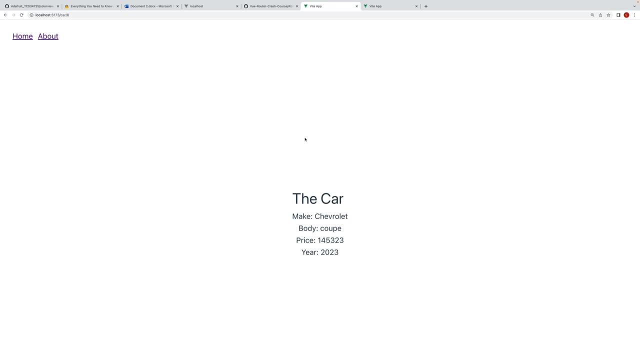 so now, what we're going to do is we're. so now, what we're going to do is we're actually going to talk about nested, actually going to talk about nested, actually going to talk about nested, components, which is kind of an. components, which is kind of an. 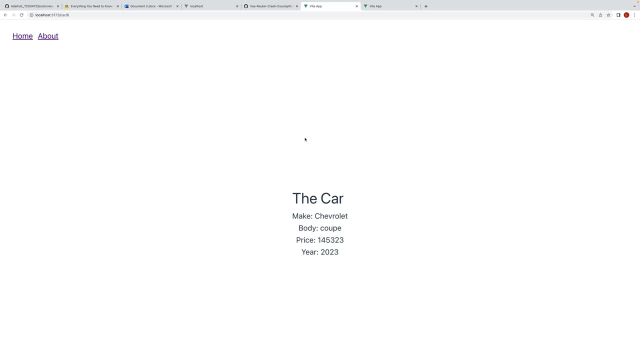 components, which is kind of an interesting and cool feature. interesting and cool feature. interesting and cool feature, so to define nested components. we're so to define nested components. we're so to define nested components. we're going to have to define that inside of, going to have to define that inside of. 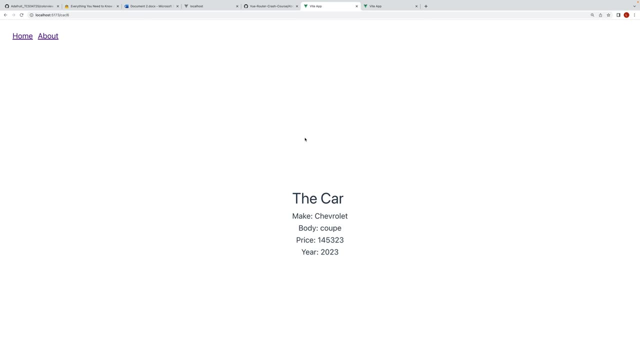 going to have to define that inside of our main dot, our main dot, our main dot js file, or sorry, not in our mainjs js file, or, sorry, not in our mainjs js file, or sorry, not in our mainjs file. it's actually going to be inside of. 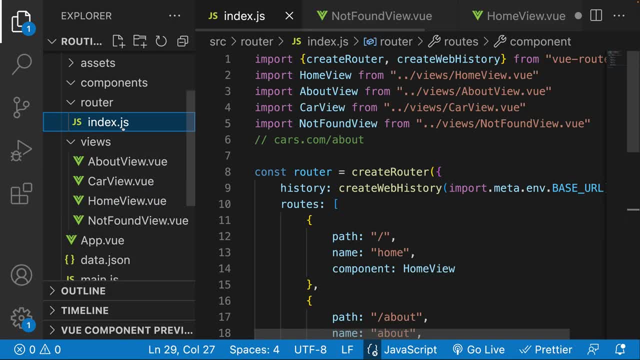 file. it's actually going to be inside of file. it's actually going to be inside of our router file. so let's go over here our router file. so let's go over here our router file. so let's go over here and instead of our router index, we're. 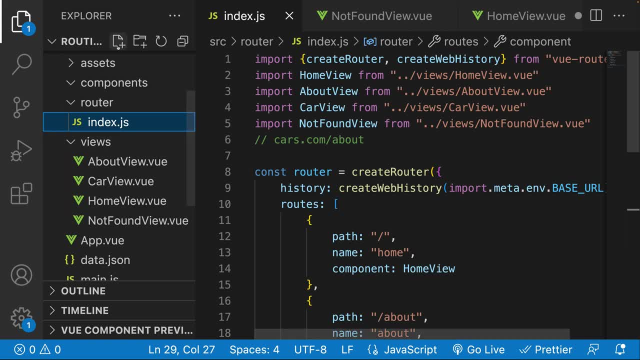 and instead of our router index, we're, and instead of our router index, we're going to define, going to define, going to define our new nested rules. so i'm going to go: our new nested rules. so i'm going to go, our new nested rules. so i'm going to go over here. 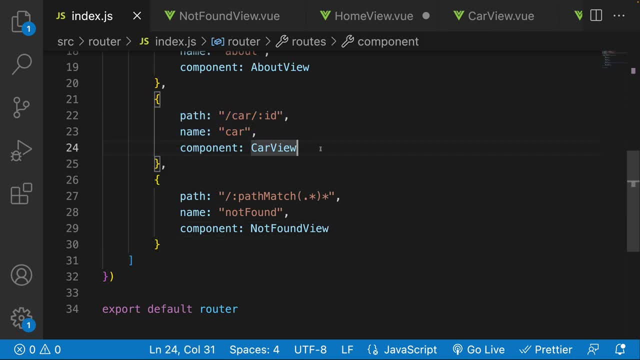 over here, over here, and let's go to the car view and over, and let's go to the car view and over, and let's go to the car view and over here. what i'm going to define here, what i'm going to define here, what i'm going to define are some children. so i'm going to say: 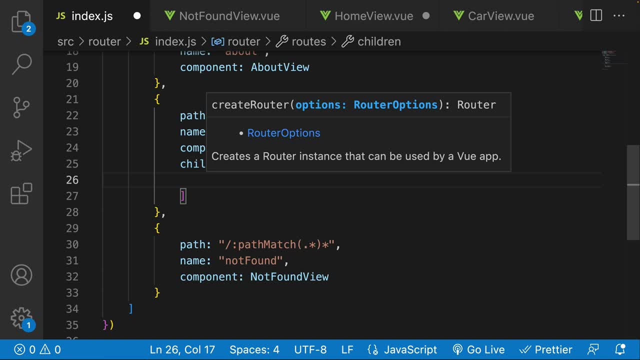 are some children. so i'm going to say: are some children? so i'm going to say children, and this is going to be children, and this is going to be children and this is going to be an array and this is going to have kind an array and this is going to have kind. 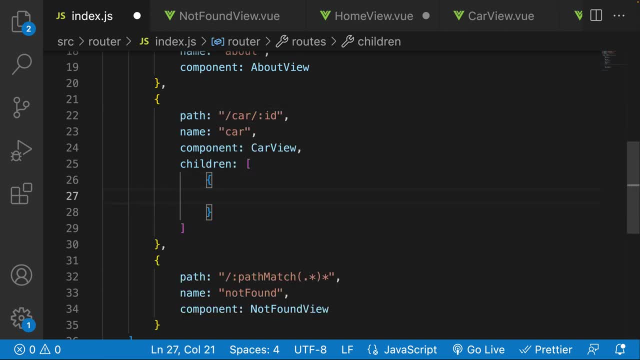 an array and this is going to have kind of these similar stuff that we have here, of these similar stuff that we have here, of these similar stuff that we have here. so i'm going to say so, i'm going to say so, i'm going to say an object, and this i'm going to say path. 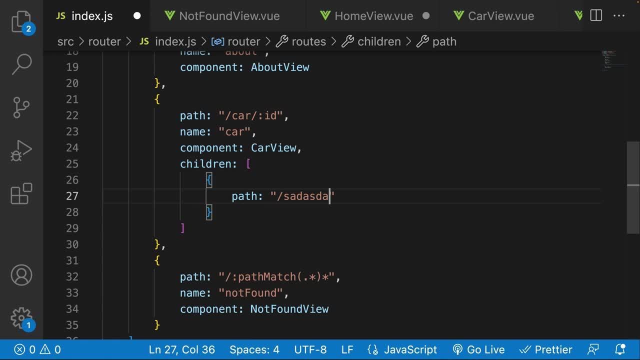 an object, and this i'm going to say: path an object, and this i'm going to say: path like so, but instead of providing slash like so, but instead of providing slash like so, but instead of providing slash, something we're going to say very, something we're going to say very. 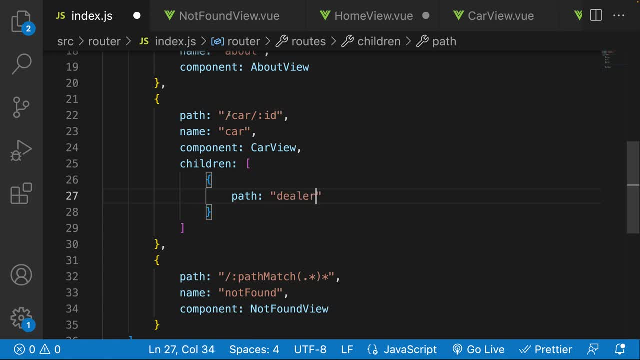 something we're going to say very simply: the path is going to be dealer. simply, the path is going to be dealer. simply, the path is going to be dealer and it's going to understand that this and it's going to understand that this and it's going to understand that this is going to append this path over here. 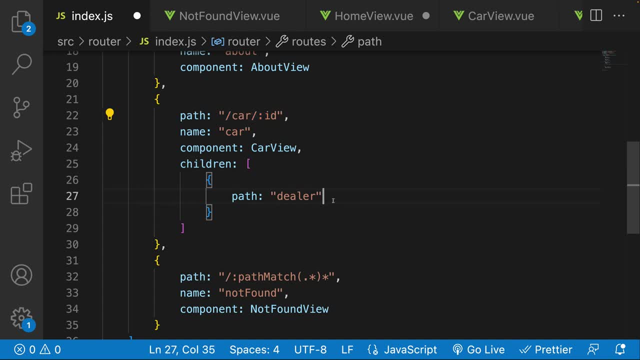 is going to append this path over here, is going to append this path over here. so it's going to be slash car, slash id. so it's going to be slash car, slash id. so it's going to be slash car, slash id, slash dealer? and if that's the case, what? 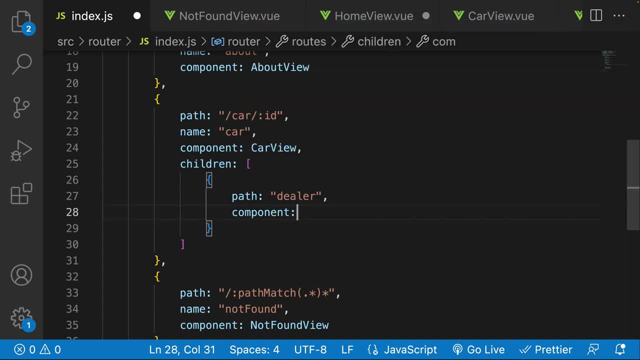 slash dealer? and if that's the case, what slash dealer? and if that's the case, what i want to do is: i want to render, i want to do is. i want to render, i want to do is. i want to render the dealer components. so i'm going to say: 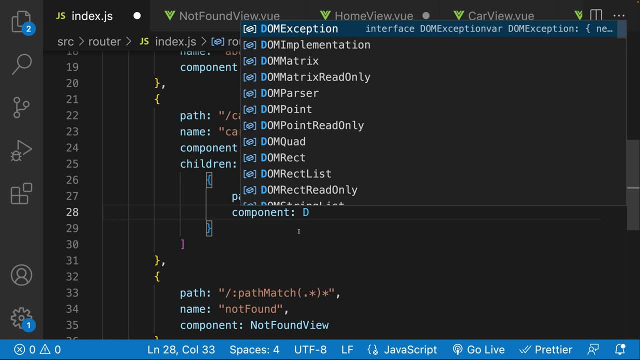 the dealer components. so i'm going to say the dealer components. so i'm going to say dealer, dealer. oh my goodness the dealer, oh my goodness the dealer, oh my goodness the. i can't see anything dealer view. i can't see anything dealer view. i can't see anything dealer view, components. and we can, of course, do the. 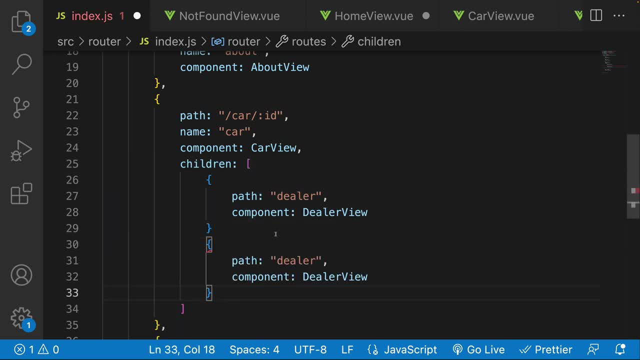 components, and we can of course do the components, and we can of course do the exact same thing now, exact same thing now, exact same thing now over here, so we can call this over here, so we can call this over here, so we can call this the menu. 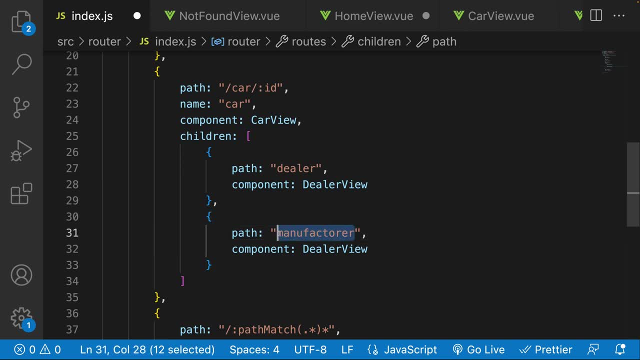 the menu, the menu: fact, fact, fact, sure, sure, sure. i'm going to copy this because it's. i'm going to copy this because it's. i'm going to copy this because it's kind of a hard word to spell, kind of a hard word to spell. 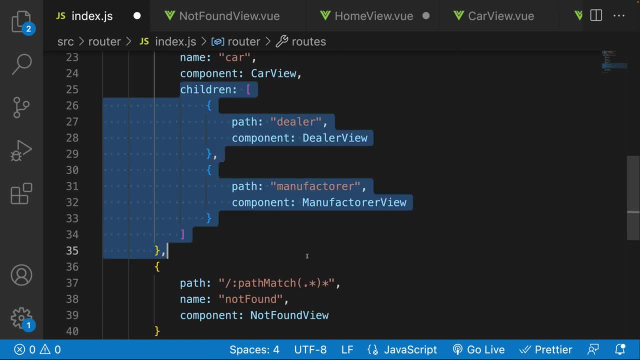 kind of a hard word to spell. and there we go- manufacturer, so this is. and there we go- manufacturer, so this is. and there we go- manufacturer, so this is how we can actually add children, so how we can actually add children, so how we can actually add children. so let's go ahead and i'm going to get rid. let's go ahead and i'm going to get rid. let's go ahead and i'm going to get rid of this for now. let's go ahead and just of this for now. let's go ahead and just of this for now. let's go ahead and just quickly create these components. so i'm 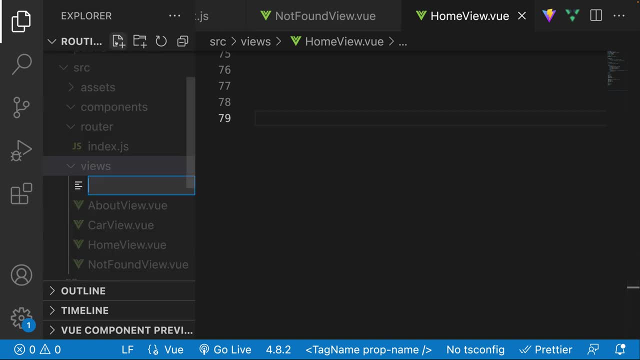 quickly create these components. so i'm quickly create these components. so i'm gonna gonna gonna uh go to the views and we're going to uh go to the views and we're going to uh go to the views and we're going to create a, create a. 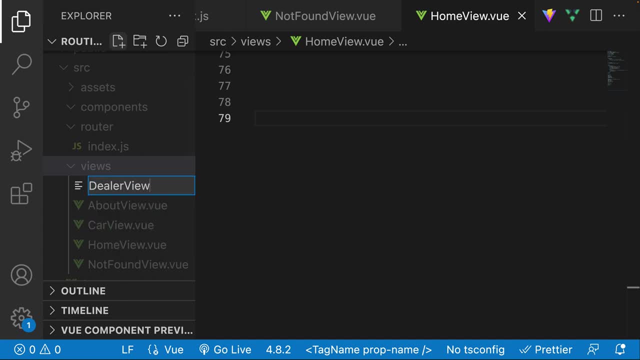 create a dealer dealer view, dealer dealer view, dealer dealer view, dot view and, very simply, we're just dot view and very simply, we're just dot view and very simply, we're just going to create a template with a div, going to create a template with a div. 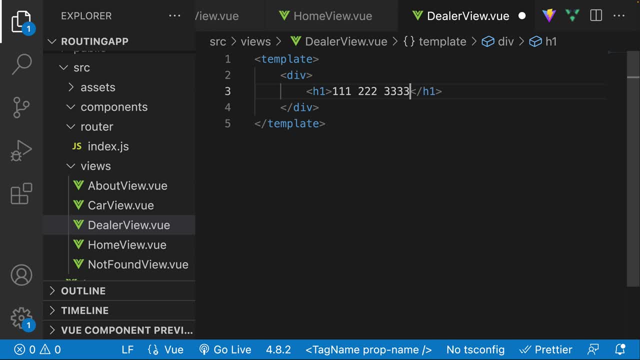 going to create a template with a div, with an h1, with an h1, with an h1, and this is the dealer's information. and this is the dealer's information. and this is the dealer's information. that's his. that's his number and over. that's his. that's his number and over. 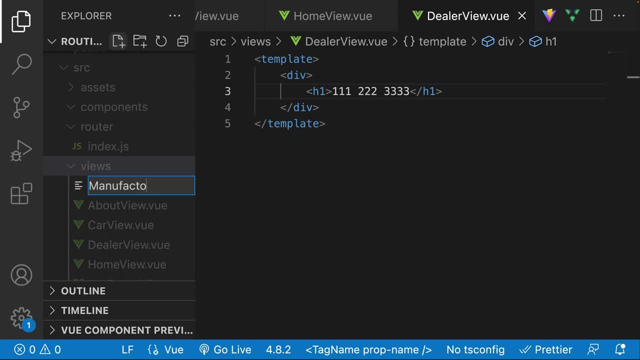 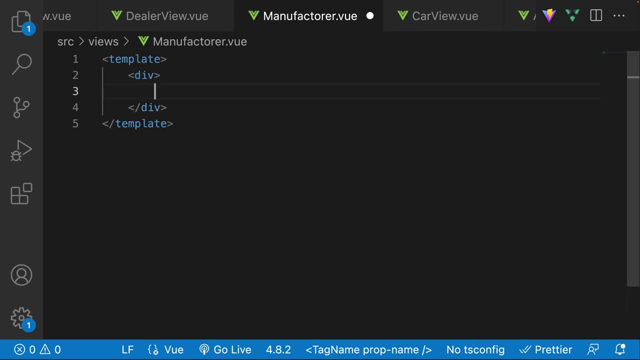 that's his, that's his number, and over here, here, here, we can say manufacturer, we can say manufacturer, we can say manufacturer, dot view, dot, view, dot, view, and this one very again very simply, and this one very again very simply, and this one very again very simply. template div. 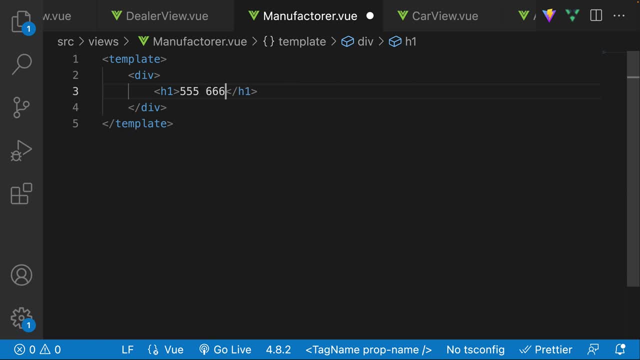 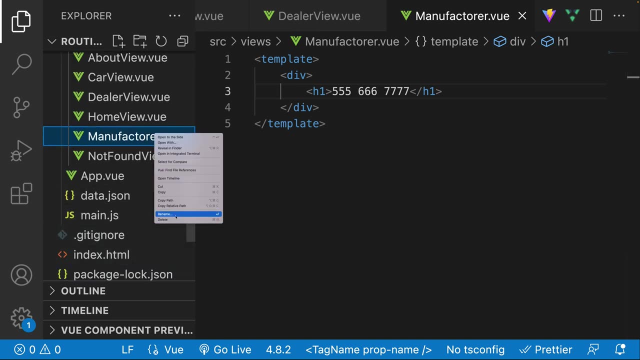 template- div. template, div. and uh, let's have an h1, and this is his. and uh, let's have an h1, and this is his. and uh, let's have an h1, and this is his. information, information, information. all right, so now what we need to do. 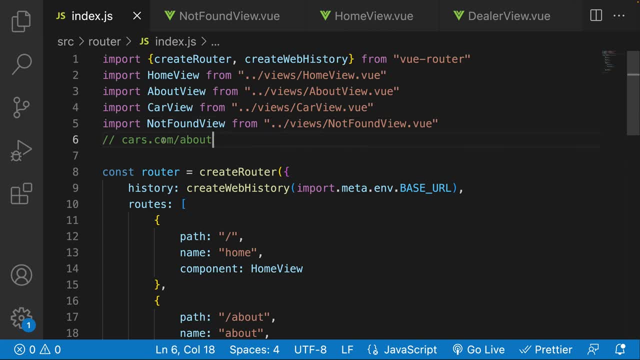 all right, so now what we need to do? all right, so now what we need to do is very simply actually import that inside, is very simply actually import that inside, is very simply actually import that inside of our indexjs file, of our indexjs file, of our indexjs file. so i'm going to say import manufacturer. 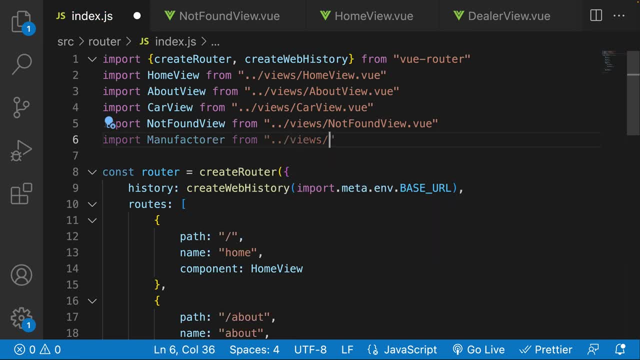 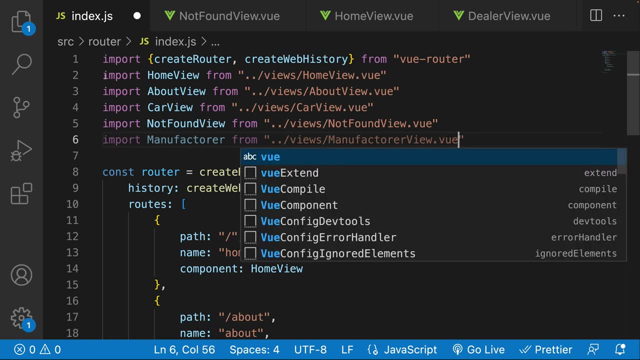 so i'm going to say import manufacturer. so i'm going to say import manufacturer from. we're going to say from. we're going to say from. we're going to say views, and then manufacturer views and then manufacturer views, and then manufacturer view, view, view, dot view. all right, so that's the. 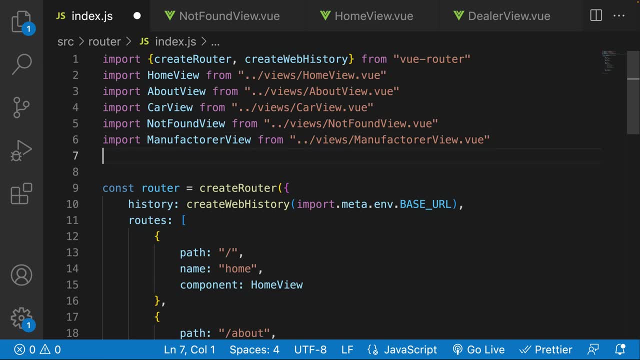 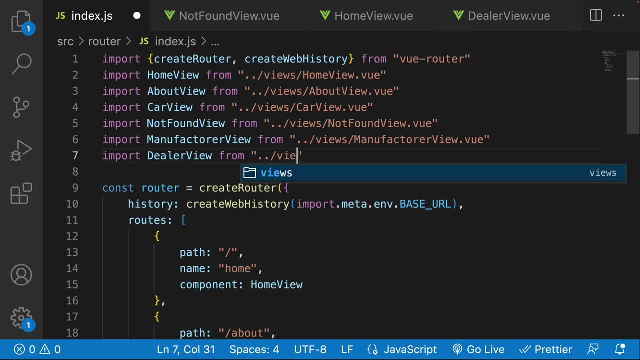 dealer view, dealer view and we're going to import that from and we're going to import that from and we're going to import that from views, and then over here we're going to views and then over here we're going to views and then over here we're going to say: 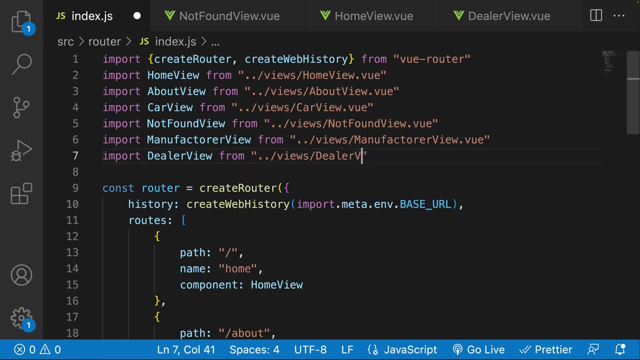 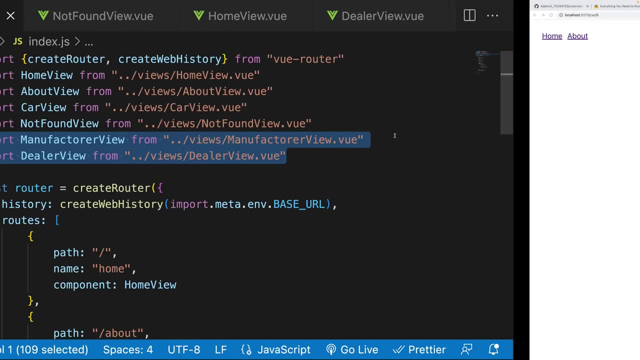 say say dealer, dealer, dealer view view view, dot view like so okay, dot, view like so okay, dot view like so okay. so this is looking pretty good to me, so this is looking pretty good to me. so this is looking pretty good to me. uh, so now, uh, so now. 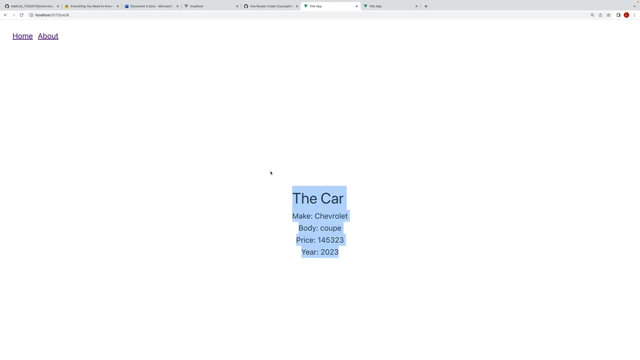 uh, so now. so now, what we can do here, if you. so now, what we can do here, if you. so now, what we can do here. if you refresh, you can see that everything is refresh. you can see that everything is refresh. you can see that everything is fine. however, of course, what we're doing, 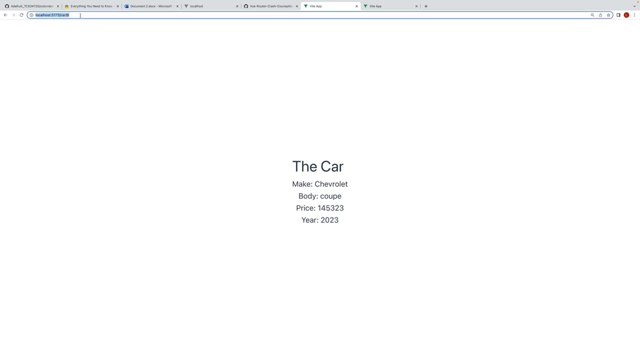 fine. however, of course, what we're doing? fine, however, of course, what we're doing is we're not um, we're not showing this. is we're not um, we're not showing this. is we're not um, we're not showing this. but now, if i, let's say, i go to 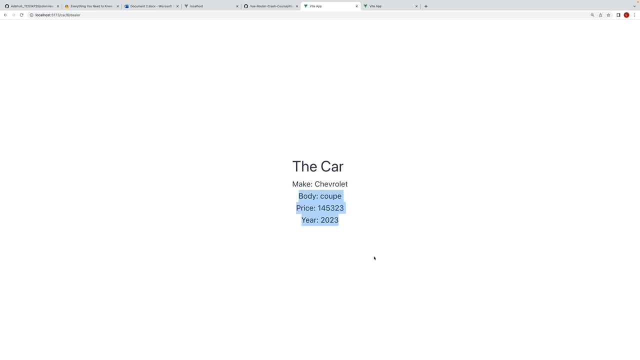 but now if i let's say i go to, but now if i let's say i go to dealer, dealer, dealer, i still don't show it, so that's kind of, i still don't show it, so that's kind of, i still don't show it. so that's kind of weird, what's going on? 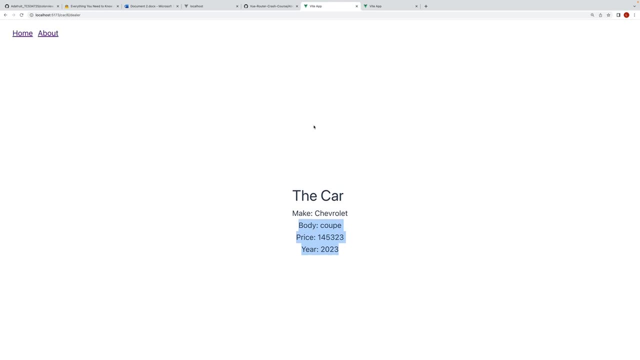 weird what's going on. weird what's going on. well, we're actually forgetting the step. well, we're actually forgetting the step. well, we're actually forgetting the step of defining where we want to render this, of defining where we want to render this, of defining where we want to render this component inside of the home view. 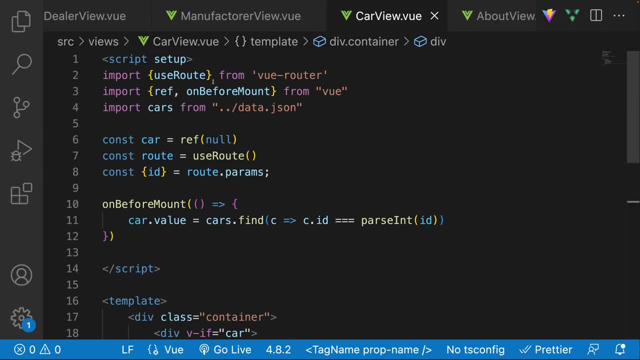 component inside of the home view component, inside of the home view component, or sorry inside of the car component, or sorry inside of the car component, or sorry inside of the car view component. so what we're actually view component, so what we're actually view component, so what we're actually going to need to utilize. 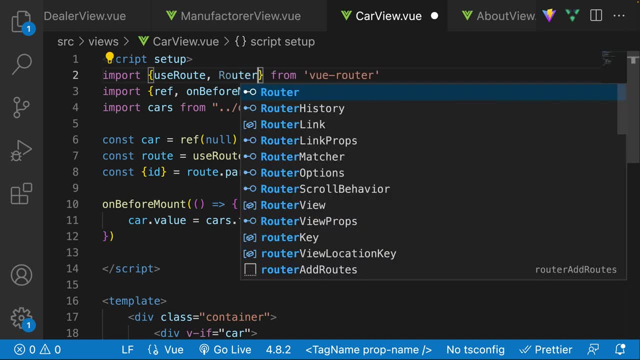 going to need to utilize. going to need to utilize is the router view component. so router is the router view component. so router is the router view component. so router view view view. so over here, so i'm going to say that i. so over here, so i'm going to say that i. 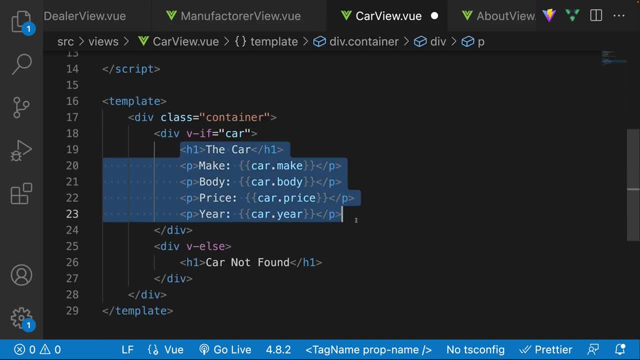 so over here. so i'm going to say that i want to render, want to render, want to render this. let's say right below this, let's say right below this, let's say right below all of this. so i'm going to say: right, all of this. so i'm going to say right. 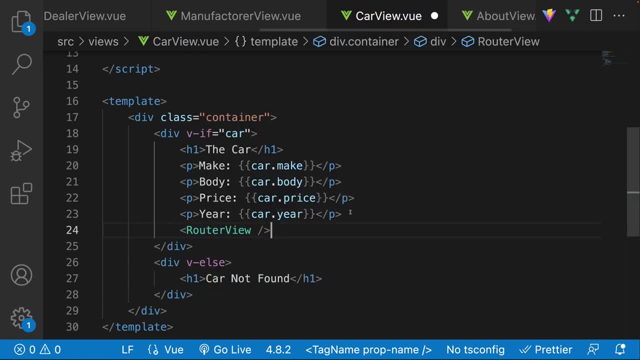 all of this. so i'm going to say, right over here, i want to render the over here, i want to render the over here, i want to render the router view component. so go ahead and router view component. so go ahead and router view component. so go ahead and save that. 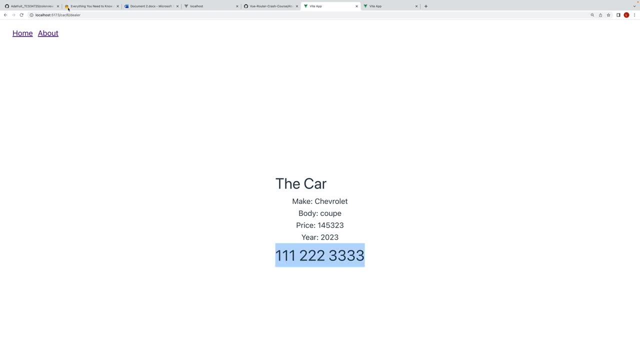 save that, save that, and now, right away, you can see we, and now, right away, you can see we, and now, right away, you can see, we actually get, actually get, actually get our dealer information and over here, our dealer information and over here, our dealer information and over here we can now change this to. 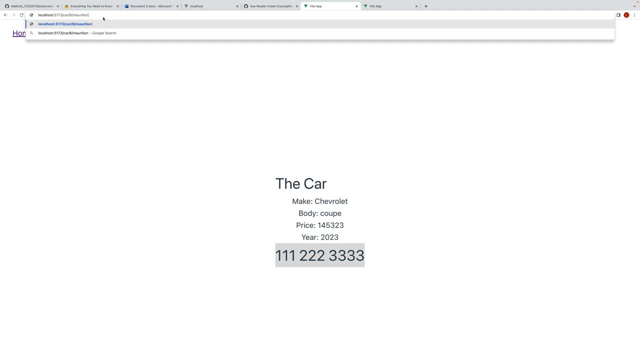 we can now change this to: we can now change this to: manufacturer: manufacturer. and i misspelled it incorrectly and i misspelled it incorrectly and i misspelled it incorrectly. menu, menu, menu- fact, fact, fact charrer. we're getting a not found page. 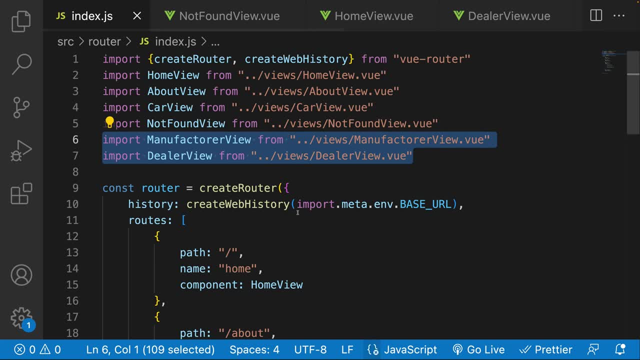 let's see how i spelled it inside of. let's see how i spelled it inside of. let's see how i spelled it inside of: here, here, here, so the indexjs file, so the indexjs file, so the indexjs file. just copy that. just copy that. 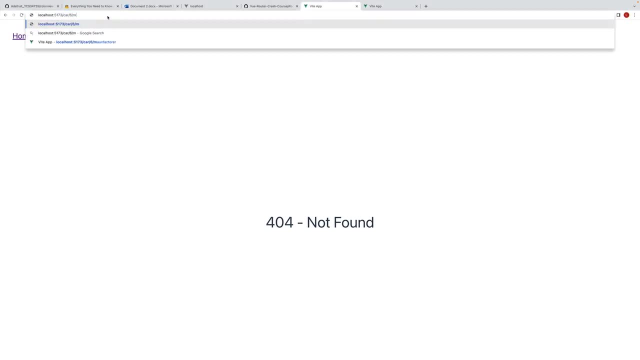 just copy that. so i'm going to say, copy that in and now you can see, now we copy that in and now you can see, now we copy that in and now you can see, now we get the manufacturer information, get the manufacturer information, get the manufacturer information. some styling differences, but whatever. 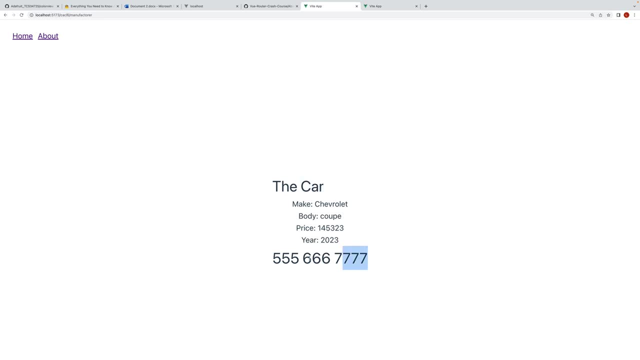 some styling differences, but whatever, some styling differences, but whatever, that's fine, that's fine, that's fine, okay. so that's pretty much all it is okay. so that's pretty much all it is okay. so that's pretty much all it is. that's how we can actually incorporate. 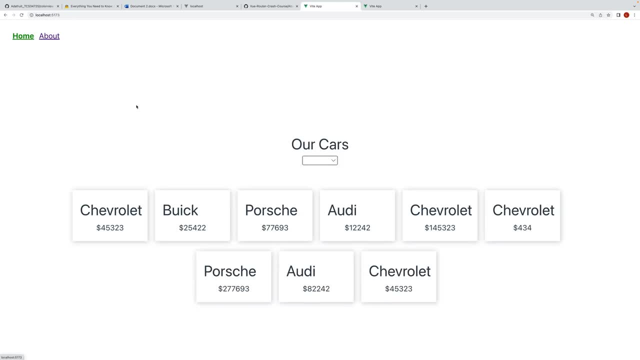 that's how we can actually incorporate. that's how we can actually incorporate nested routes into our app, now, of course. nested routes into our app, now, of course. nested routes into our app, now, of course, it would be nice to, instead of actually, it would be nice to, instead of actually, 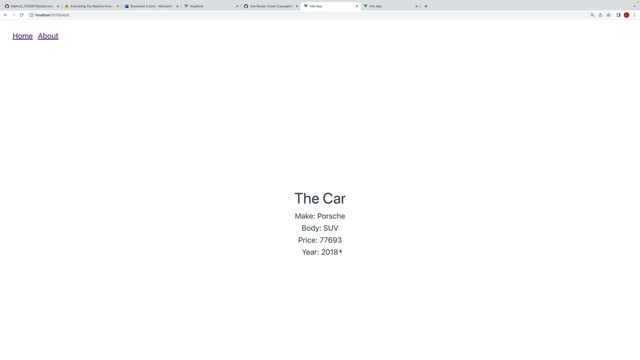 it would be nice to, instead of actually typing in dealer or manufacturer, we can typing in dealer or manufacturer, we can typing in dealer or manufacturer, we can have a button there. but, honestly, for now, have a button there. but honestly, for now, have a button there. but honestly, for now, i think that's a okay. you guys probably. 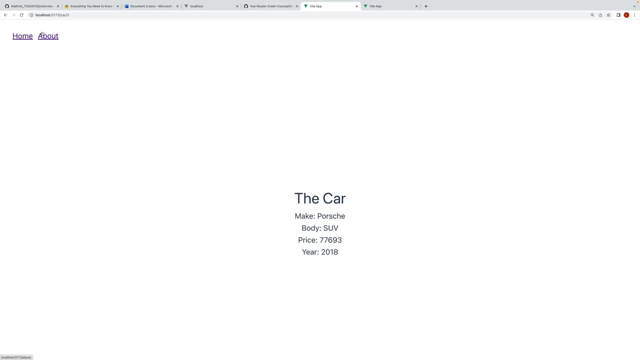 i think that's a okay, you guys probably. i think that's a okay, you guys probably get the point, get the point, get the point okay. so there is one more thing that i okay. so there is one more thing that i okay. so there is one more thing that i want to discuss and that is: uh, let's say 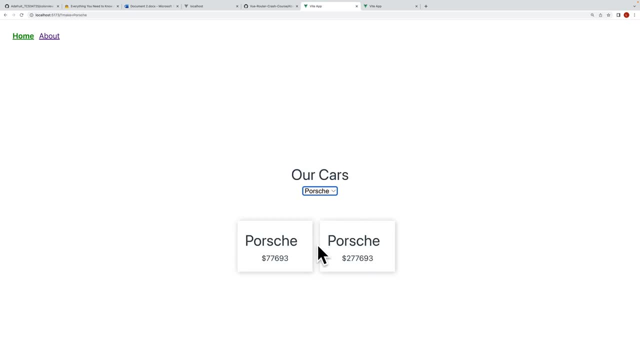 want to discuss, and that is uh, let's say, want to discuss, and that is uh, let's say, i go over here and i select a porsche, i go over here and i select a porsche, i go over here and i select a porsche, and i may be interested in both these. 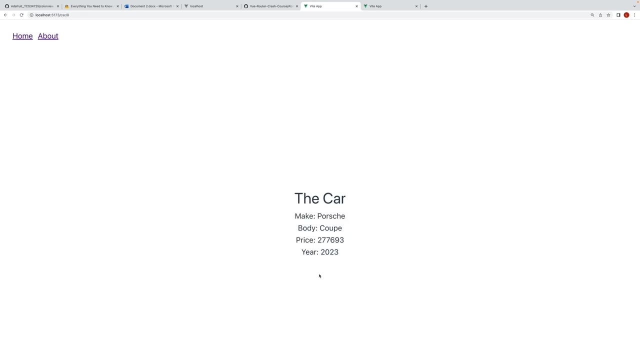 and i may be interested in both these. and i may be interested in both these porsches, porsches, porsches. and i select this porsche, and then i'm, and i select this porsche, and then i'm, and i select this porsche, and then i'm like, okay, let's go back. and if i were to, 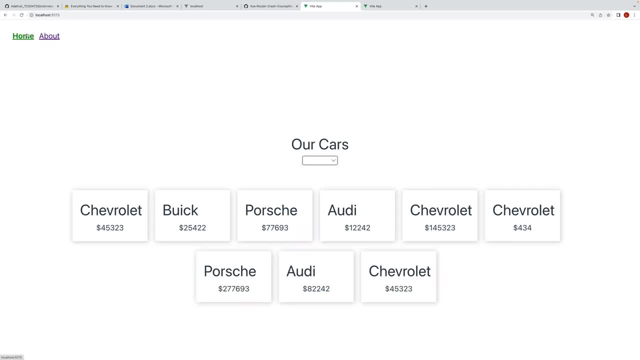 like, okay, let's go back. and if i were to like, okay, let's go back. and if i were to go, let's say i were to go back over here, go, let's say i were to go back over here, go, let's say i were to go back over here to go to home. you can see that i get. 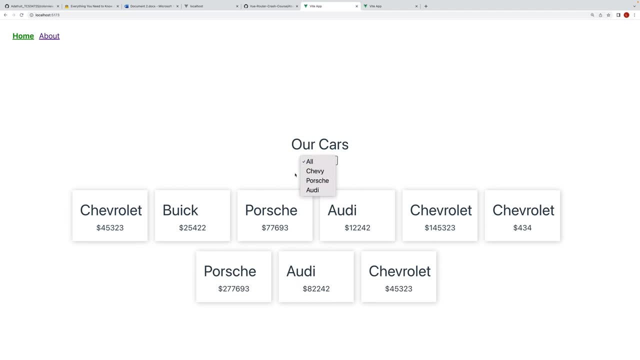 to go back over here to go to home. you can see that i get to go back over here to go to home. you can see that i get redirected to the page with the kind redirected to the page with the kind redirected to the page with the kind of the initial state, without the query. 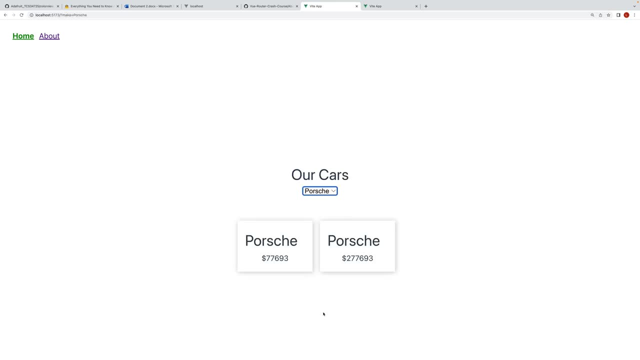 of the initial state without the query of the initial state, without the query parameter. so i think it'd be nice to parameter. so i think it'd be nice to parameter. so i think it'd be nice to have a kind of go back button. that's, have a kind of go back button. that's. 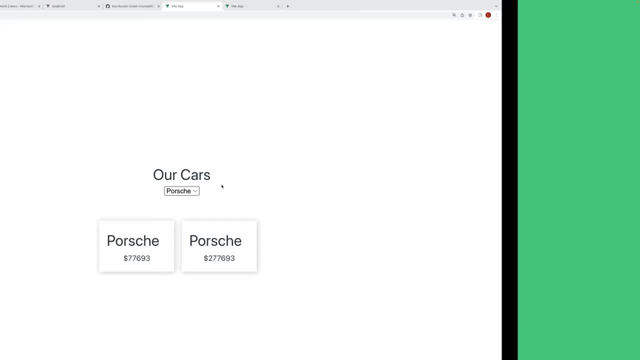 have a kind of go back button that's going to go back to the previous page. going to go back to the previous page, going to go back to the previous page, no matter what it was, no matter what it was, no matter what it was. so over here we can actually do that. 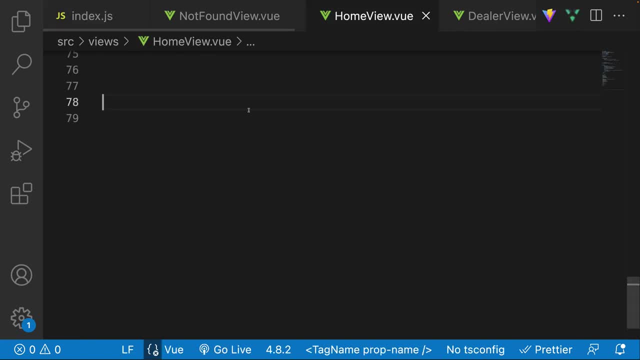 so over here we can actually do that. so over here we can actually do that relatively easily. let's go to our home relatively easily. let's go to our home relatively easily. let's go to our home- view, view, view and let's go over and let's go over. 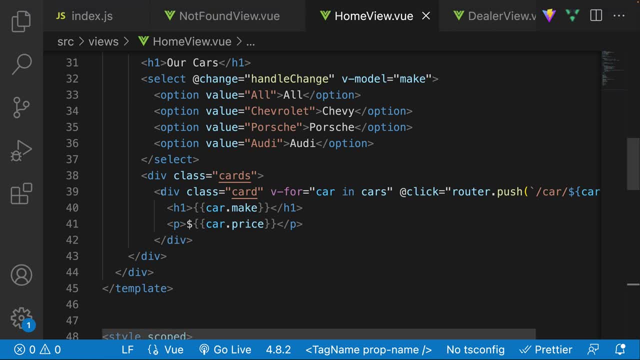 and let's go over here. now we're going to add a go back here. now we're going to add a go back here. now we're going to add a go back button, button, button. so let's add a button that'll allow us. so let's add a button that'll allow us. 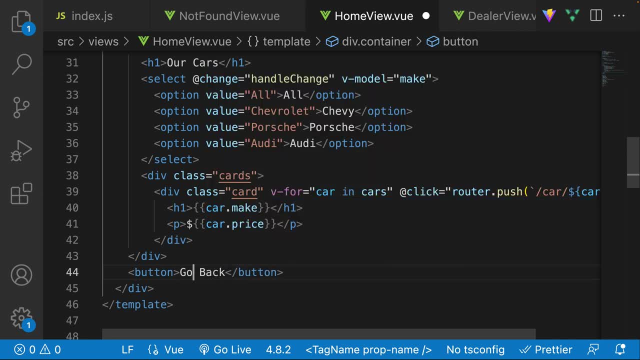 so let's add a button that'll allow us to go back, and i want it to go back to, to go back, and i want it to go back to, to go back, and i want it to go back to the previous page, the previous page, the previous page now, in order for it to go back to the 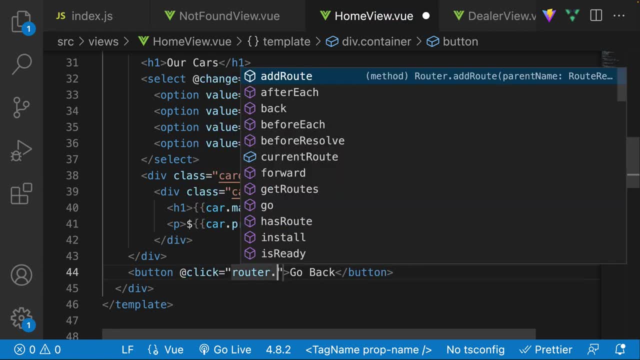 now, in order for it to go back to the now, in order for it to go back to the previous page, we're going to have it previous page. we're going to have it previous page. we're going to have it. click, click, click. we're going to use the router and then we're going to use the router and then we're going to use the router and then, very simply, there's actually a function. very simply, there's actually a function. very simply, there's actually a function here called back, and it's going to just here called back, and it's going to just here called back and it's going to just go back to the previous page, that we go back to the previous page, that we go back to the previous page, that we were on, so it's just going to go ahead. were on, so it's just going to go ahead. 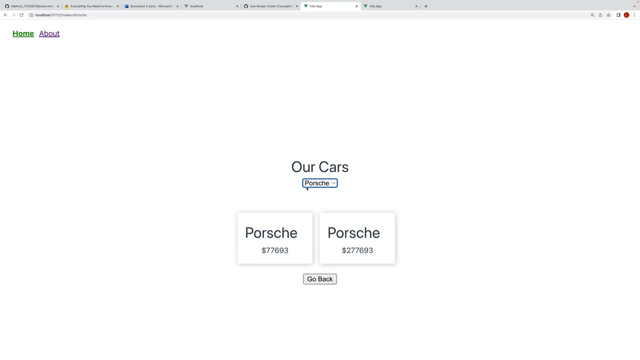 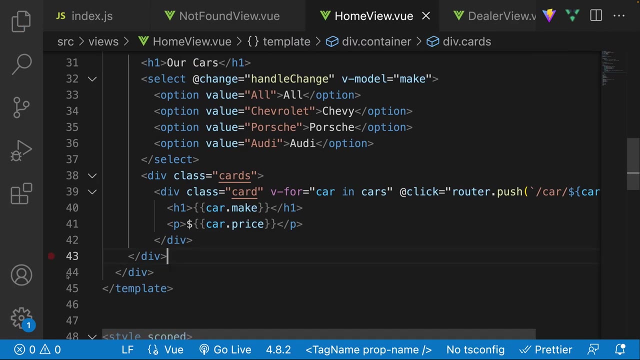 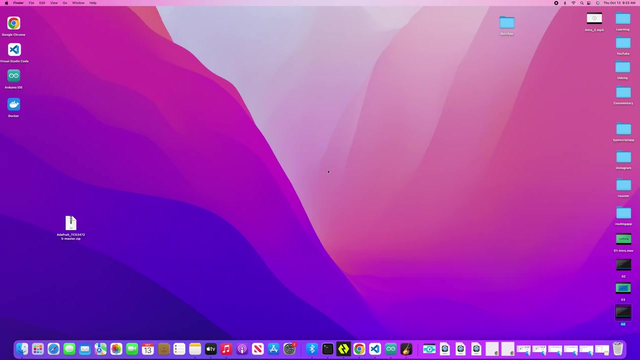 were on. so it's just going to go ahead and kind of remember that and kind of remember that and kind of remember that. so now let's say i am, so now let's say i am. so now let's say i am at this go back button. so now, when i go, 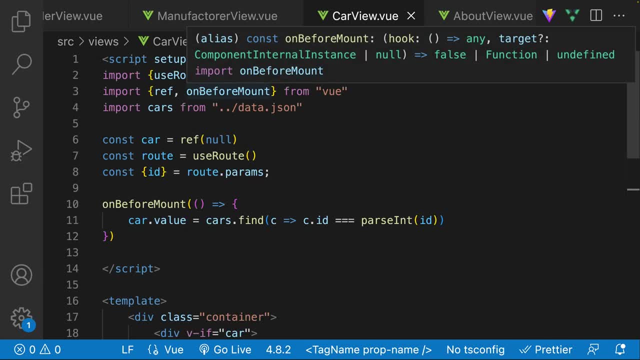 at this go back button. so now when i go at this go back button, so now when i go back, back, back, it doesn't work because we need to have. it doesn't work because we need to have. it doesn't work because we need to have the router. we're not using that here. 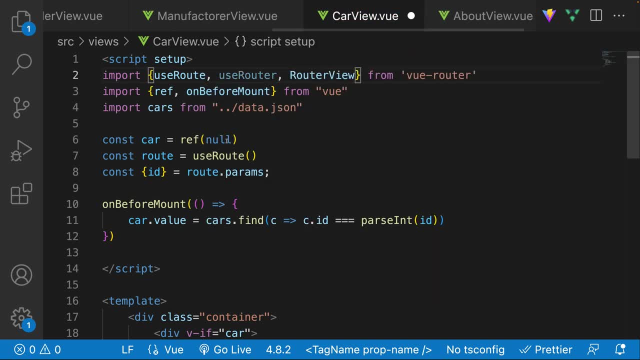 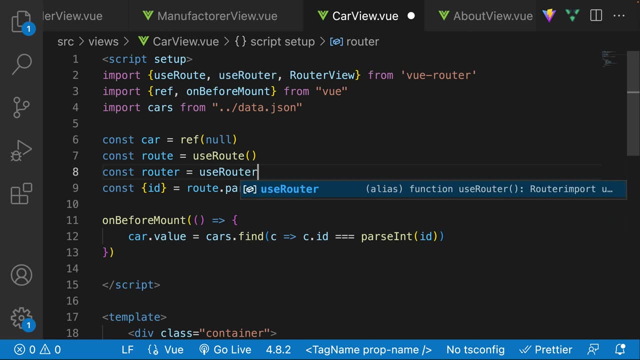 the router, we're not using that here. the router, we're not using that here. so we're going to say use. so we're going to say use. so we're going to say use router. and over here we're going to const: router, use router, router, use router. 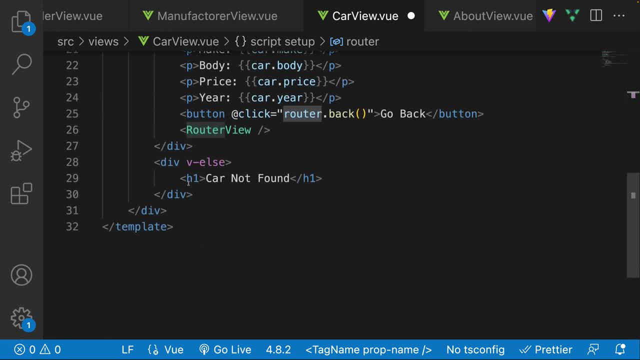 router, use router, and there we go okay, and there we go okay, and there we go okay, and over here, that's pretty much all it, and over here, that's pretty much all it, and over here, that's pretty much all it is that we need to do. 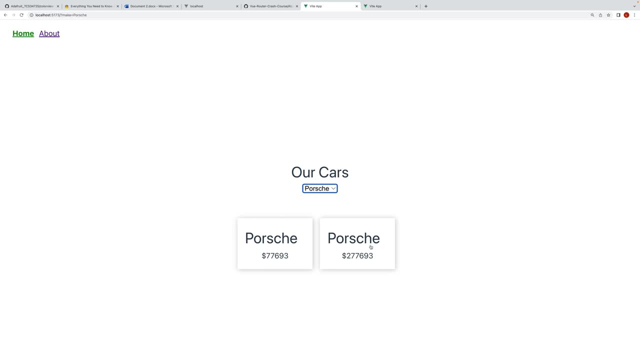 is that we need to do? is that we need to do? so? let's just go home. okay, i select for. so let's just go home. okay, i select for. so let's just go home. okay, i select for porsche. i changed my query parameter: porsche. i changed my query parameter. 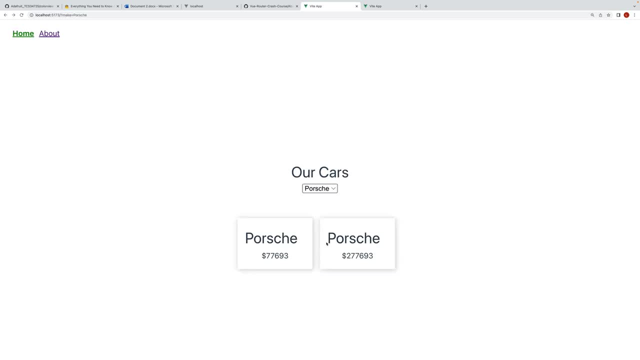 porsche. i changed my query parameter. i'm interested in this porsche. i go back. i'm interested in this porsche. i go back. i'm interested in this porsche. i go back. i can go back. i can go back. i can go back. the last thing that i promised to discuss. 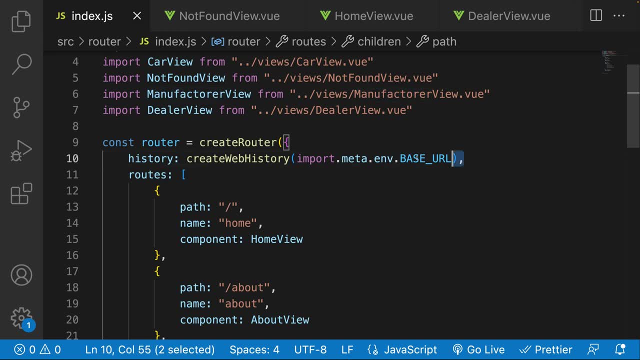 the last thing that i promised to discuss. the last thing that i promised to discuss is this, right over here, the history mode. is this, right over here, the history mode? is this, right over here, the history mode? so which is this right here? so which is this right here? 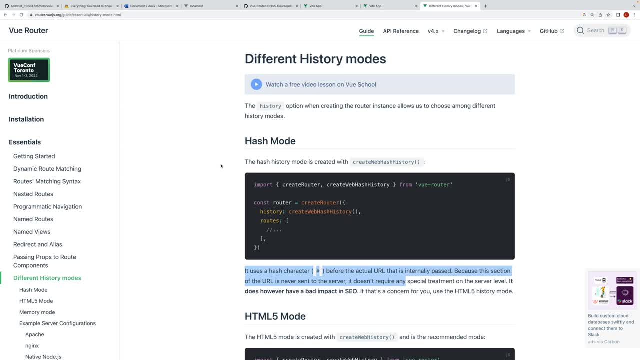 so which is this right here? so the history mode is very simply just so. the history mode is very simply just so. the history mode is very simply just kind of, kind of kind of a different outline of defining our, a different outline of defining our, a different outline of defining our different paths. 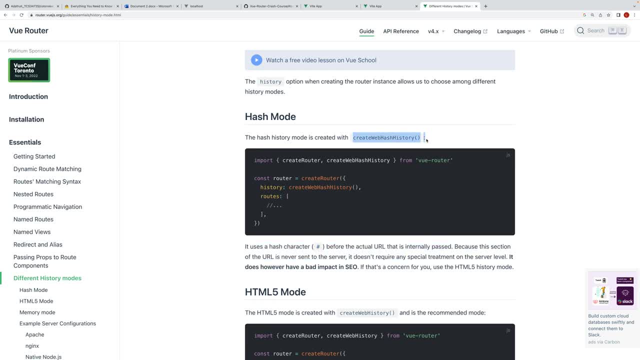 different paths, different paths. so we utilize the web history mode, but so we utilize the web history mode. but so we utilize the web history mode. but we could have also utilized the web hash. we could have also utilized the web hash. we could have also utilized the web hash history mode. 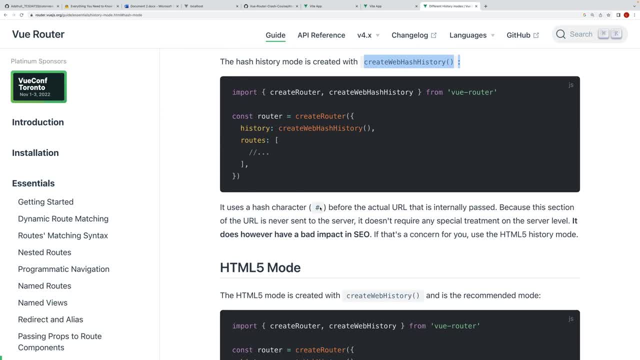 history mode. history mode, so it would look something like this, and so it would look something like this, and so it would look something like this. and what this does is it adds a hash before. what this does is it adds a hash before. what this does is it adds a hash before the url. 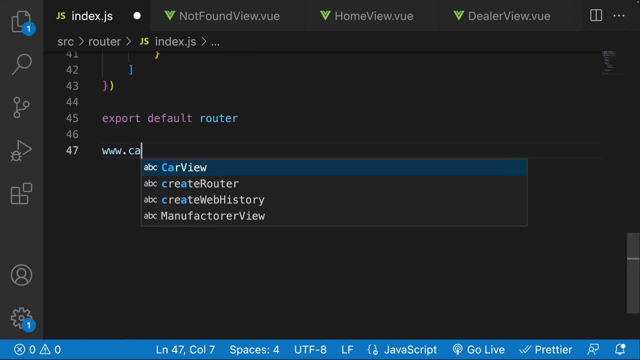 the url. the url, so it would look something like this. we so it would look something like this. we so it would look something like this: we would have would have would have wwwcarscom and then over here, wwwcarscom, and then over here, wwwcarscom and then over here, instead of having maybe slash car. 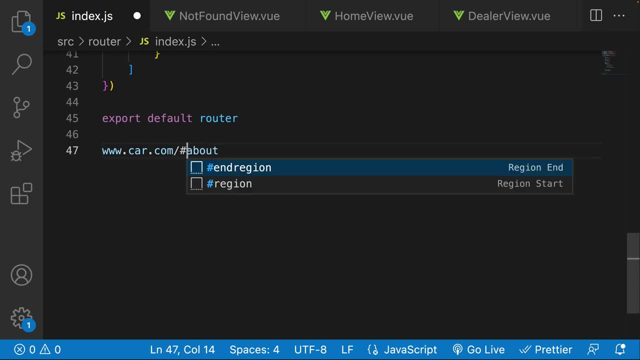 instead of having maybe slash car, instead of having maybe slash car or slash about, we would have a hash or slash about, we would have a hash or slash about we would have a hash right over here. so it'll be hash right over here. so it'll be hash. 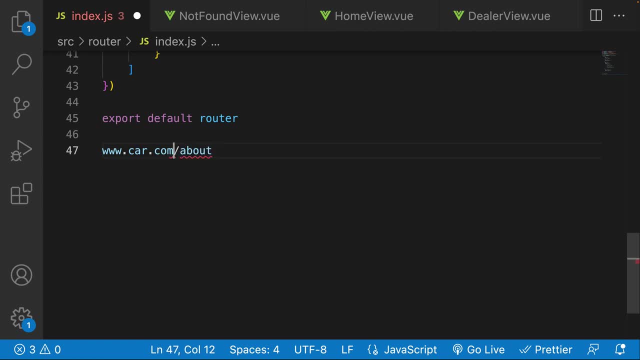 right over here. so it'll be hash and then about, and then, or sorry it and then about, and then, or sorry it and then about, and then or sorry. it would be like this would be like this, would be like this: hash, like this right here, hash about. 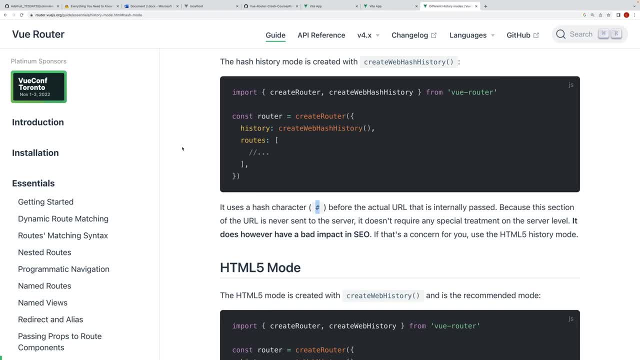 hash like this right here, hash about. hash like this right here, hash about, and then slash car and then slash, and then slash car, and then slash, and then slash car and then slash whatever. so we would always have whatever. so we would always have whatever. so we would always have this hash and, honestly, to me this doesn't. 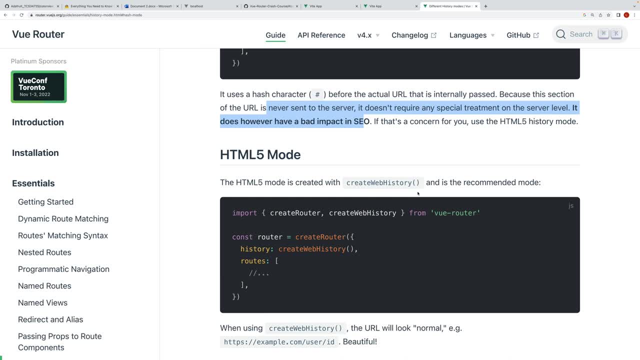 this hash and, honestly to me, this doesn't this hash and, honestly to me, this doesn't. look, look, look. all too great, and you can see here it's all too great and you can see here it's all too great and you can see here it's not really all too nice for. 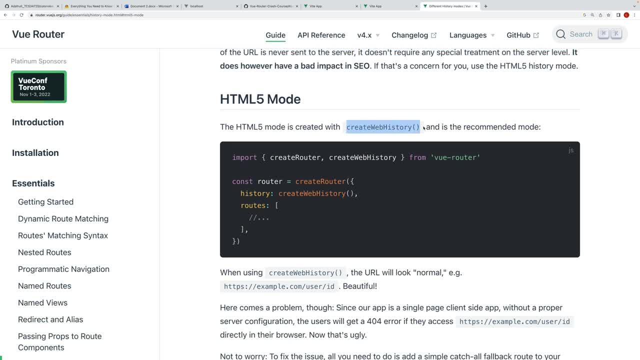 not really all too nice for not really all too nice for seo. so instead, what we're utilizing seo, so instead what we're utilizing seo, so instead what we're utilizing, is this over here which is going to be? is this over here which is going to be? 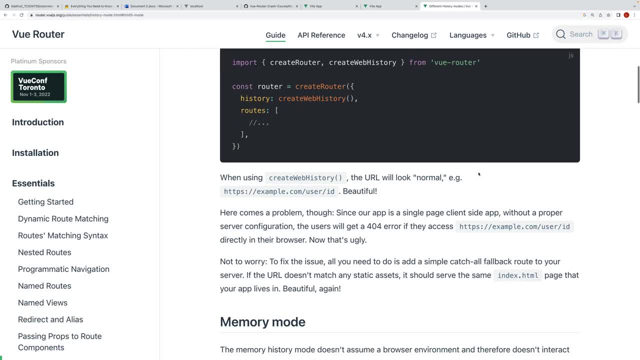 is this over here, which is going to be the web browser history that will allow the web browser history that will allow the web browser history that will allow us to well remove that hash and kind of us to well remove that hash and kind of us to well remove that hash and kind of have this beautiful url, just slash you. 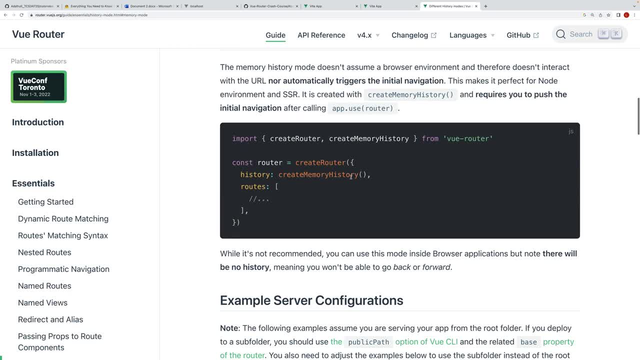 have this beautiful url, just slash you. have this beautiful url, just slash you url slash id. so that's pretty much all url slash id. so that's pretty much all url slash id. so that's pretty much all it is. there's other things more advanced. it is, there's other things more advanced. 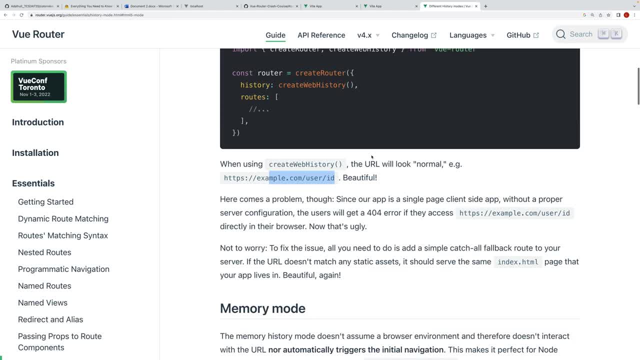 it is. there's other things more advanced features about this, but it's honestly features about this. but it's honestly features about this, but it's honestly not all too important. you can read up not all too important. you can read up not all too important. you can read up about it if you want to. about it if you want to.